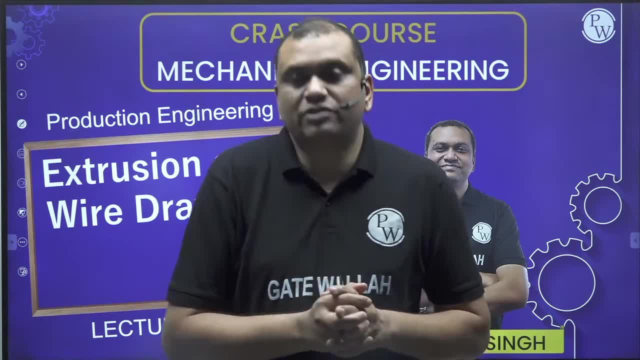 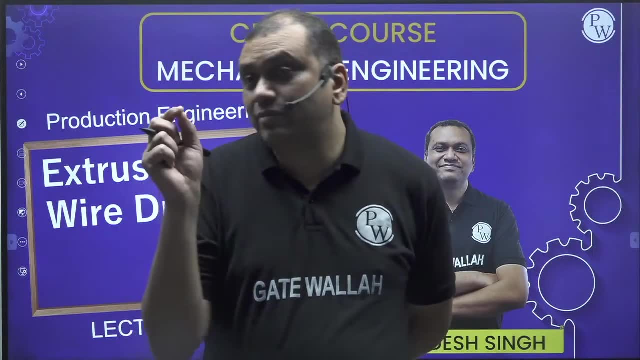 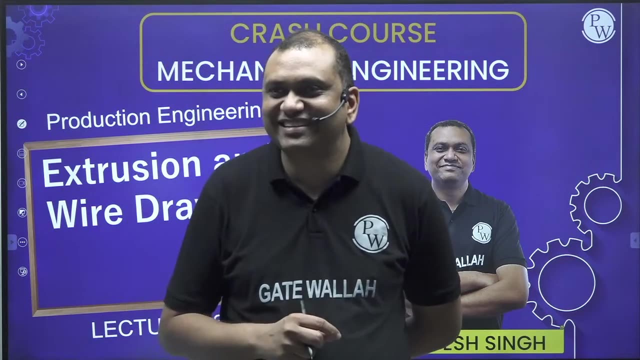 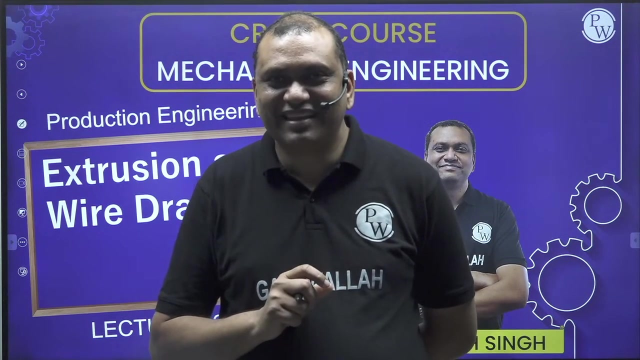 So today we will start with metal forming. Metal forming is the beginning And, brother see, this lecture is very important. Good evening, Hello Sanjit. Hello, This lecture is very important, Not because it is important in the gate, It is important. 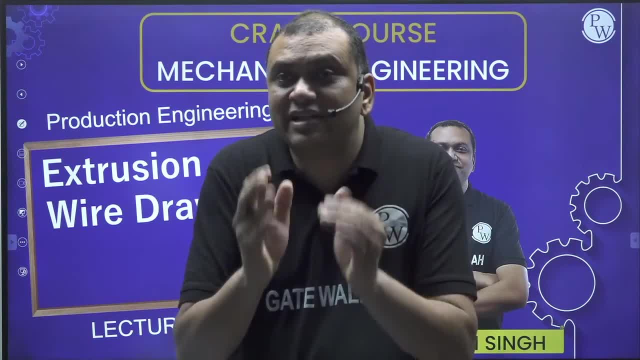 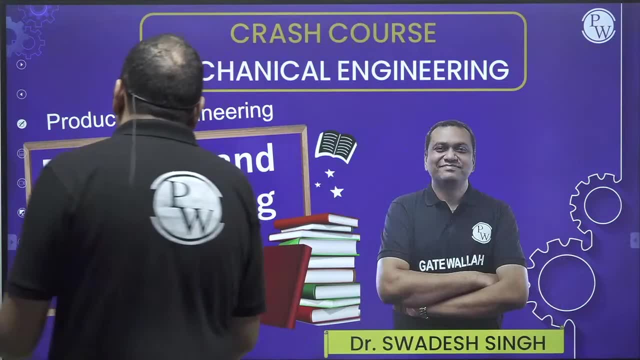 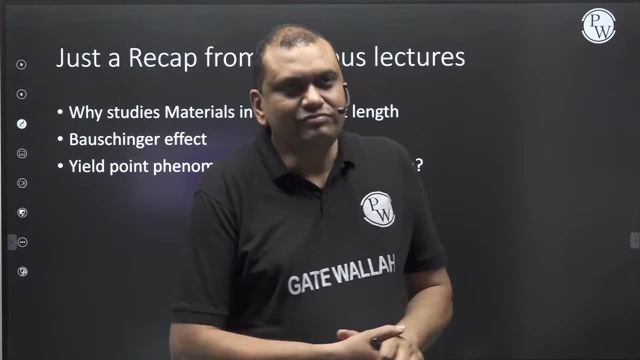 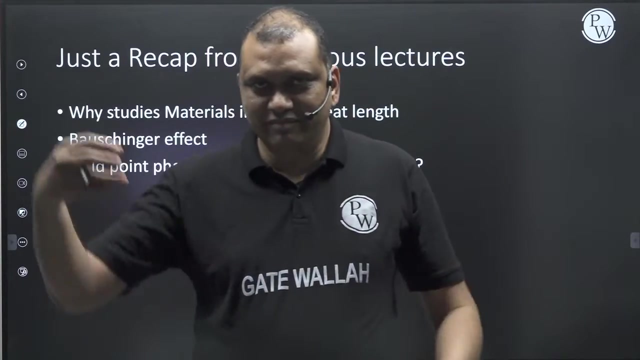 But the rest of the metal forming's fundamental knowledge is there. So in the beginning we will cover exclusion of wire drawing. We will cover exclusion of wire drawing. See some students once again. one more thing: I got hundreds of messages, personal messages. 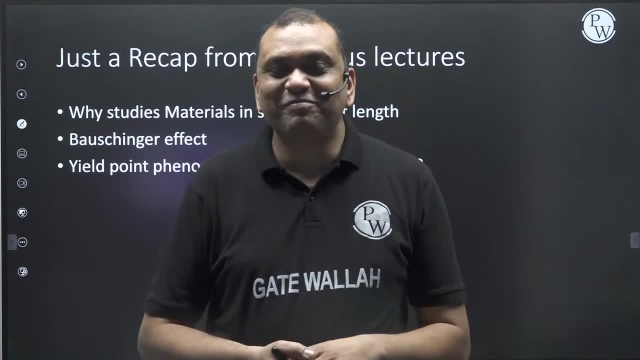 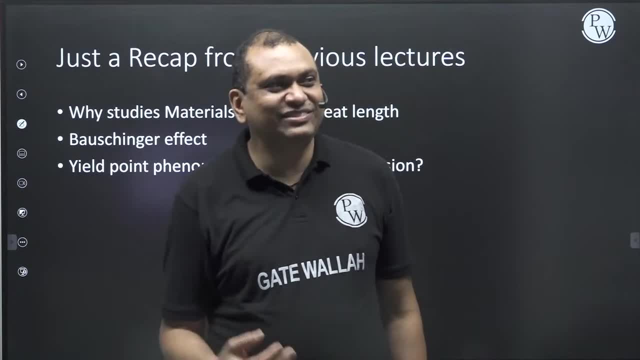 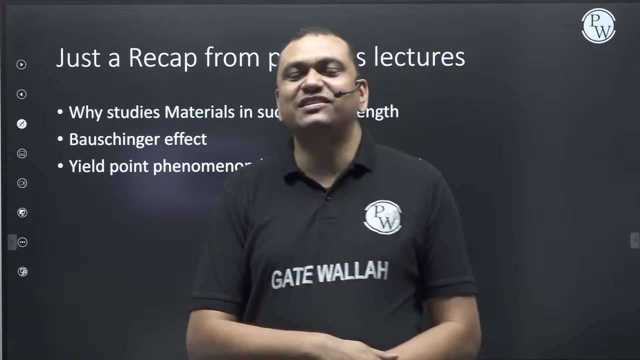 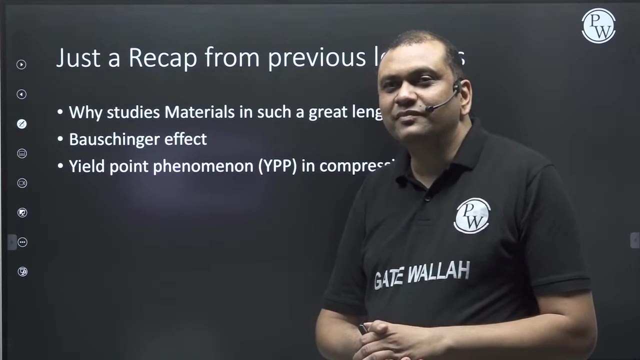 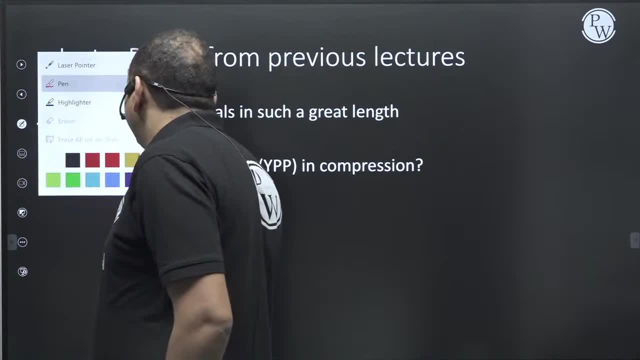 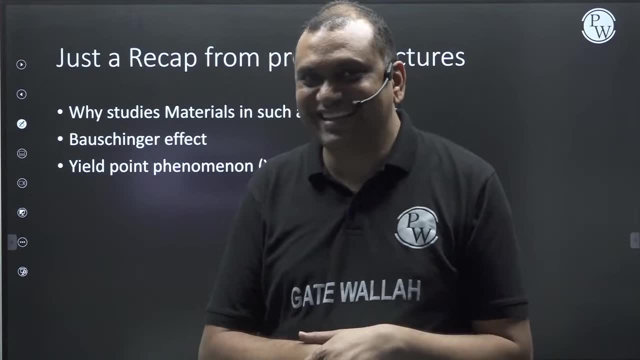 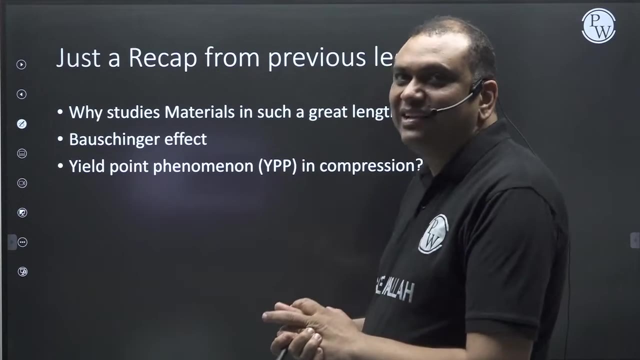 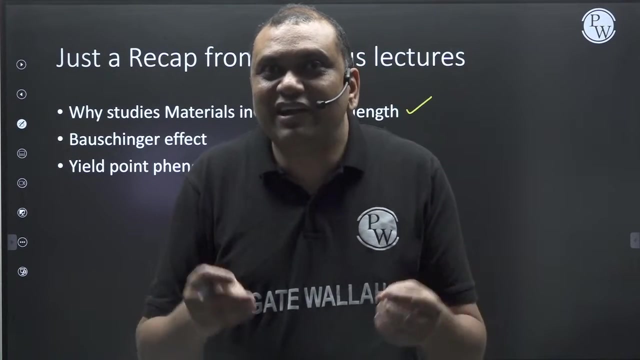 The first message that came to me from one or two students was: Sir, material science comes in 2 numbers in the gate. You have taken 5 lectures on it. Do you know the answer to this? I am addressing this first. If there are no funds for material science, then you can never understand metal forming, welding. 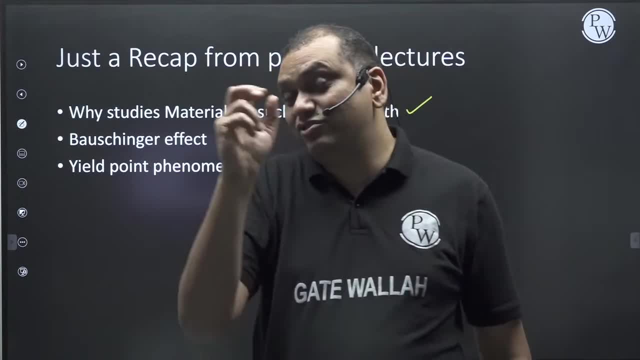 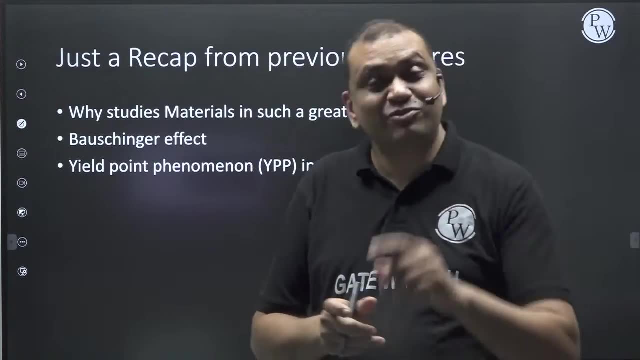 Metal forming and welding can only be understood when you we have seen 4-5 lectures on material science. if you understand that, then you will understand today's lecture on metal forming. So it is very important to develop the foundation of material science. 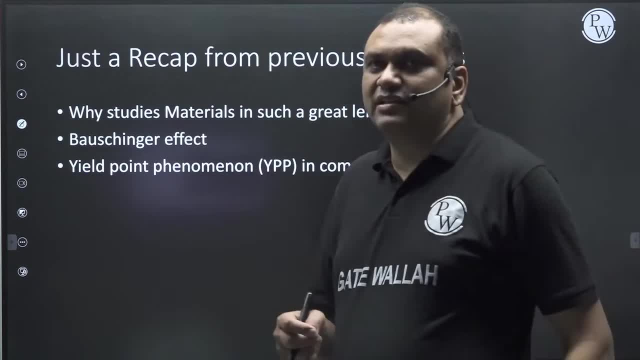 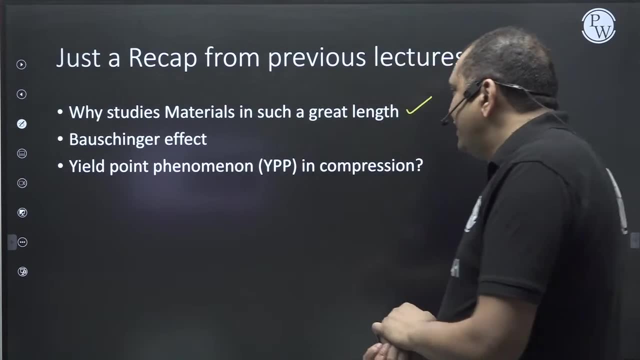 Of course there are 2 marks in the gate and sometimes there are 3 marks and sometimes 1 mark, But if you look at the history of the last 2-3 years then it comes around 2 marks. Now one student asked a question. it was a very good question. 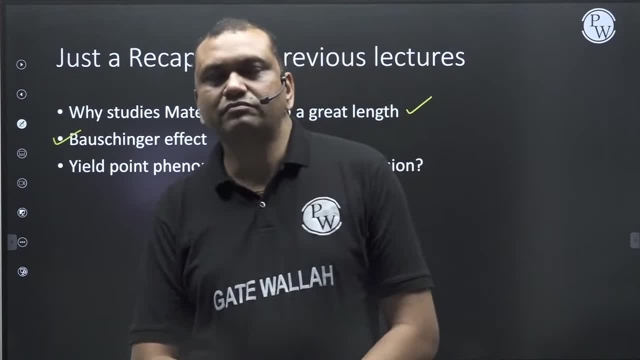 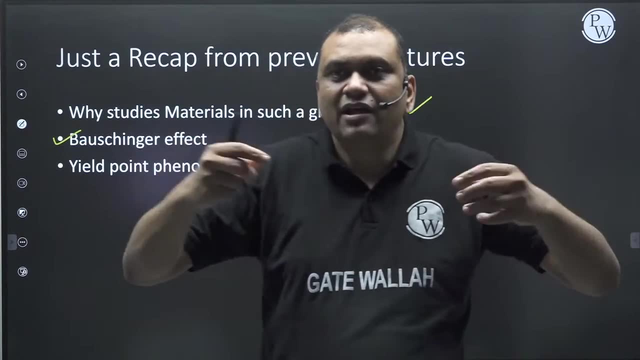 This was my personal question. it was a very good question. Sir you are saying that, Sir you are saying that, Sir you are saying that I have applied a tensile load. We are recapping a little bit. We applied a tensile load. 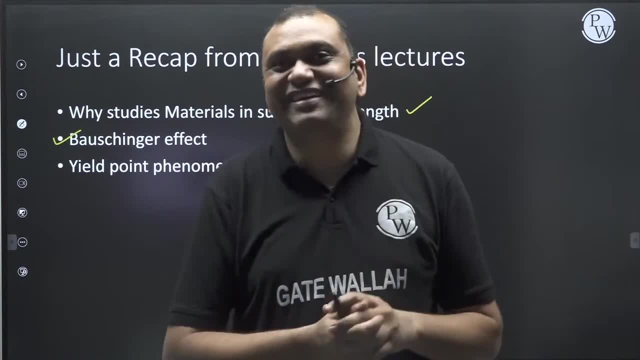 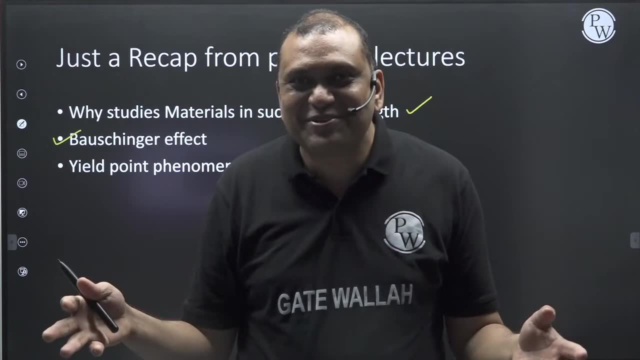 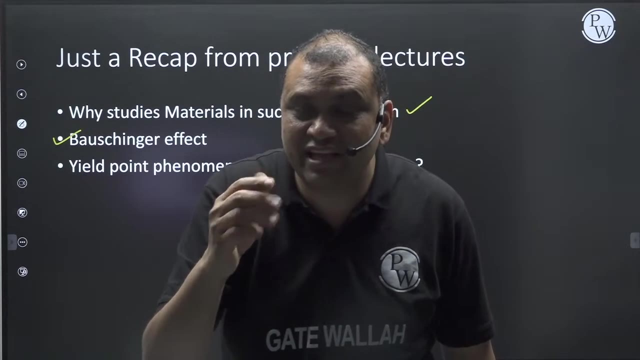 So you're saying that the dislocation is coming out. The grain boundary is found. If I have applied a compressive load suddenly, then what will happen to the material? You applied a tensile load, The dislocation started to move. This means that we are ahead of the yield point. 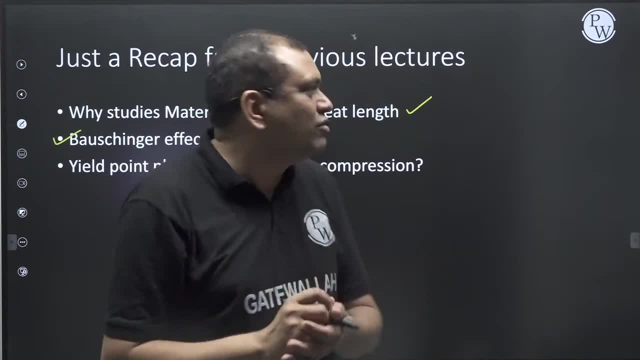 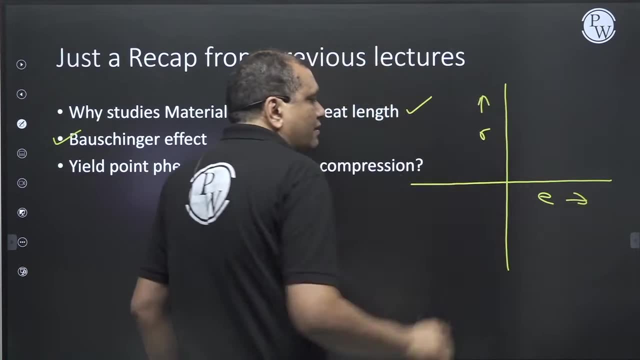 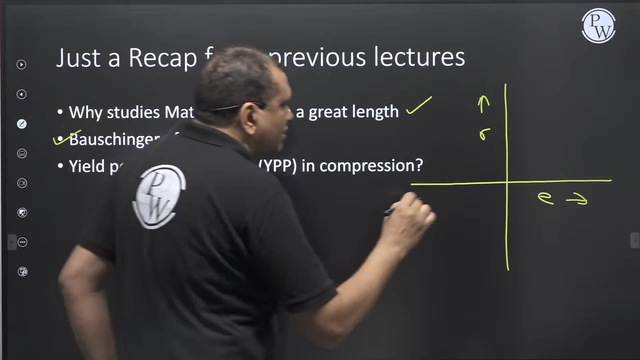 Suddenly you applied a compressive load. if you apply compressive load, then what will happen? so see, this will happen. this is stress-strain diagram. so if we look at stress-strain diagram in tension, then something like this will come: if we look at stress-strain diagram in tension: 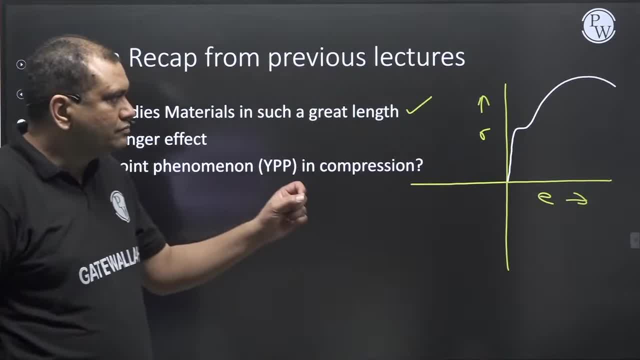 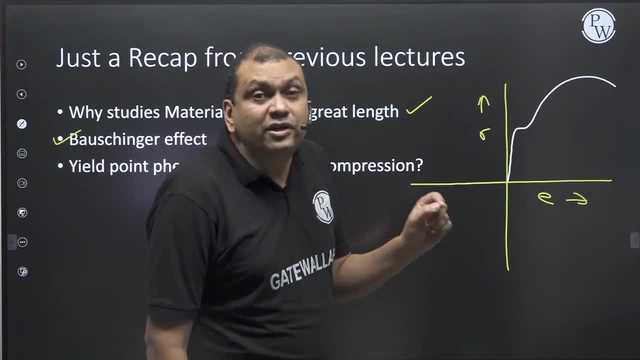 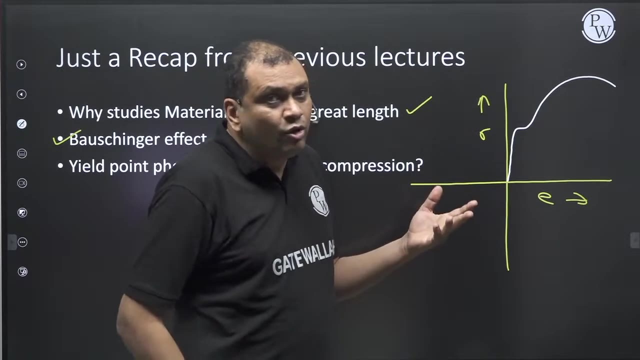 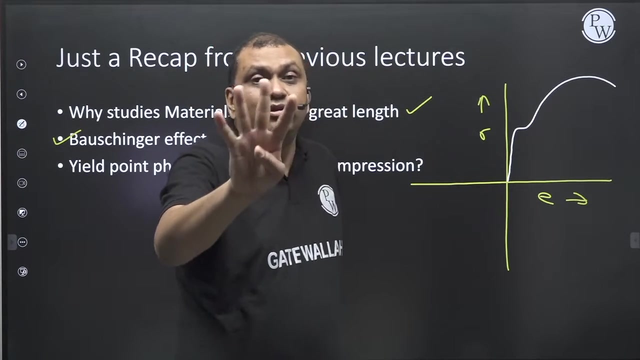 then something like this will come. so when your again I am saying it is very important to have sound fundamentals of material science, forming, welding without forming you can't do material science. today you will realize. and in metal forming, take any set, you will get question number 4. 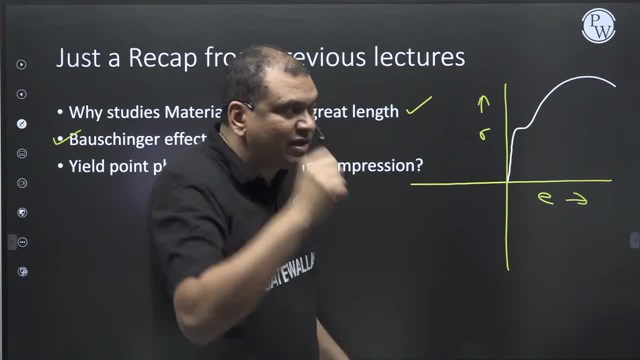 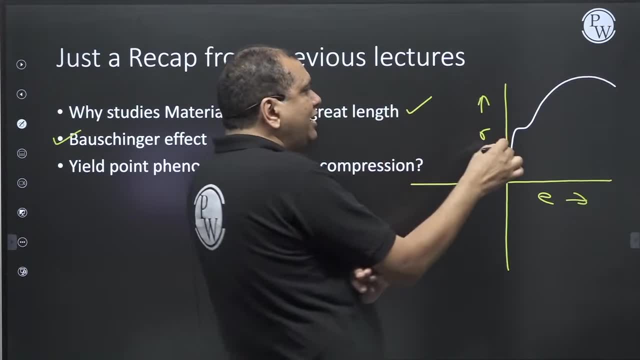 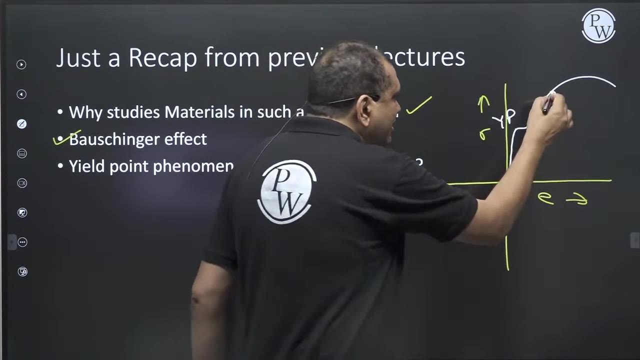 so today you have to be very careful. whatever I am teaching today, you have to be attentive and understand. so see, you have applied so much stress in tension that you are beyond the yield point. that you are beyond the yield point, let us say: till here. you have reached till here in work hardening region. 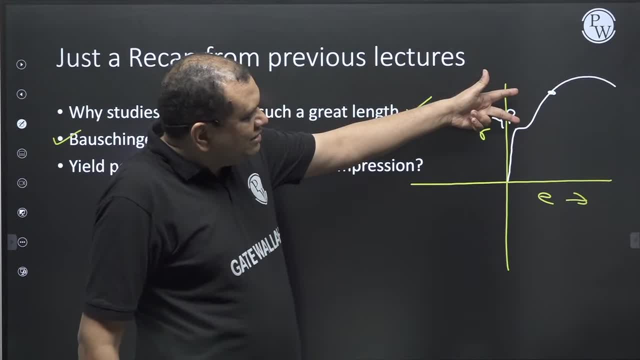 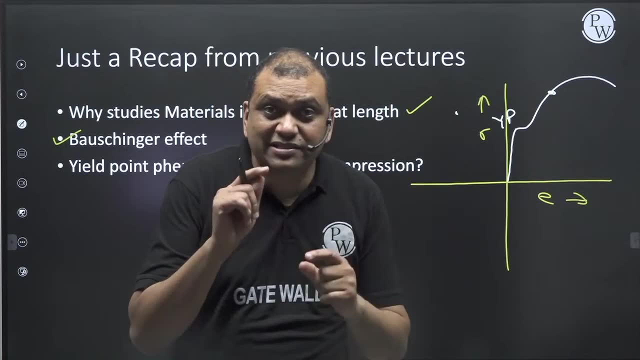 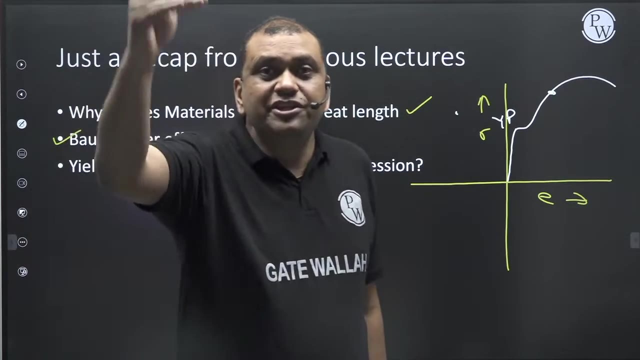 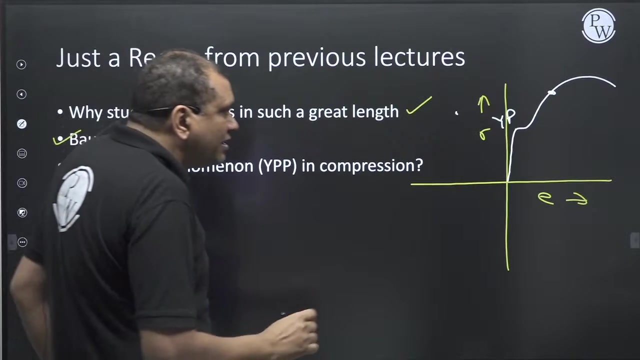 so so much back stress has developed in material. so much back stress develop now. why is it affecting what was its cause? why is it affecting what was its cause? the back stress is coming due to dislocation. pile up at the grain boundary. what did you do? now you suddenly put compression on the load due to tension. 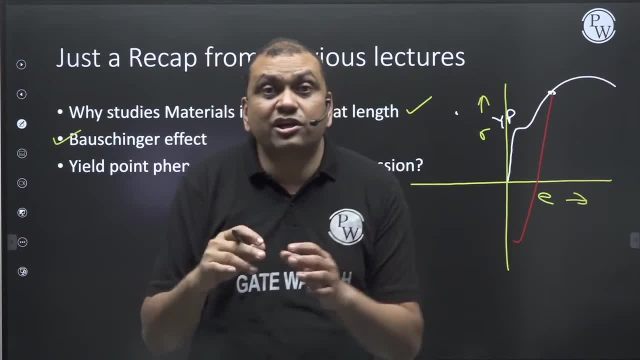 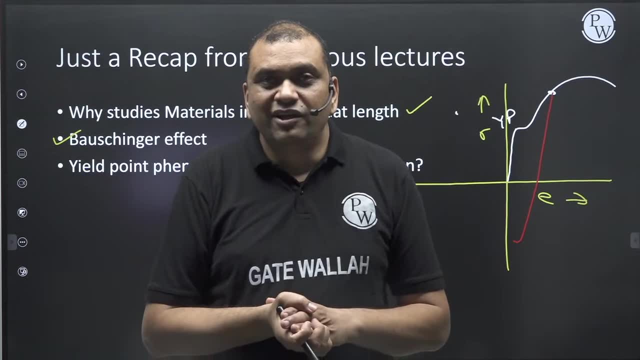 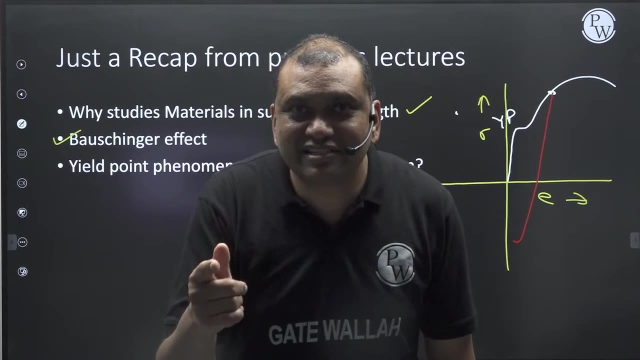 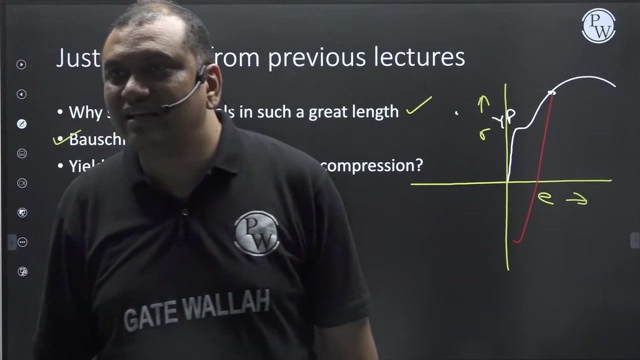 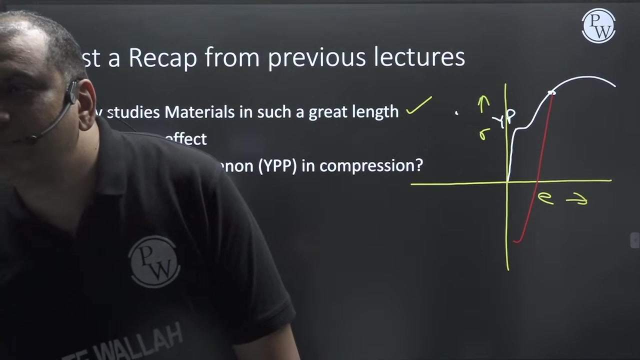 earlier it was in tension. suddenly there is a stress reversal and you started putting compression. so do you know what will happen? dislocation suddenly start moving in the opposite direction. dislocation: your lecture is coming in place of geotech class. I don't know what is this. 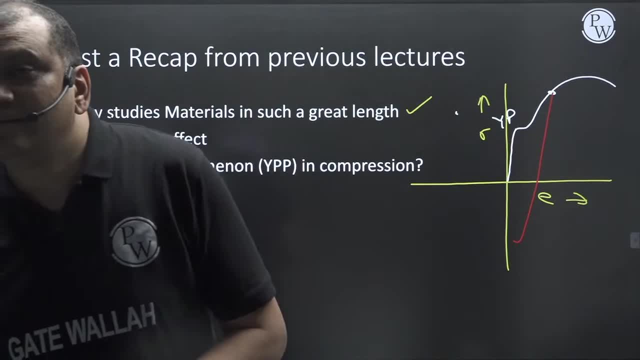 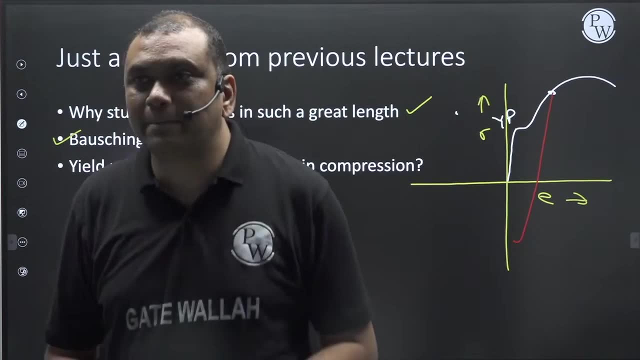 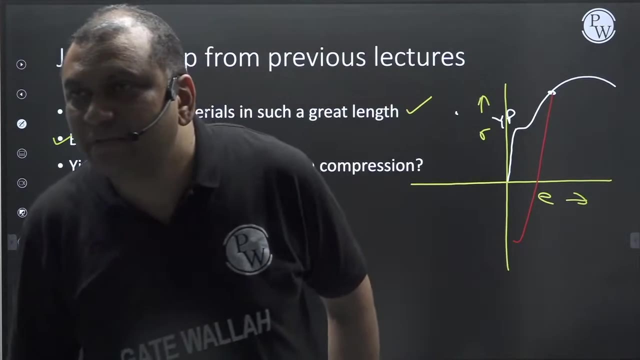 I don't know what is this actually? how can this happen? hey, all of you don't know what is this. you are basically mechanical, right, because there seems to be some link issue here. please see back end people. can you respond to the chat? 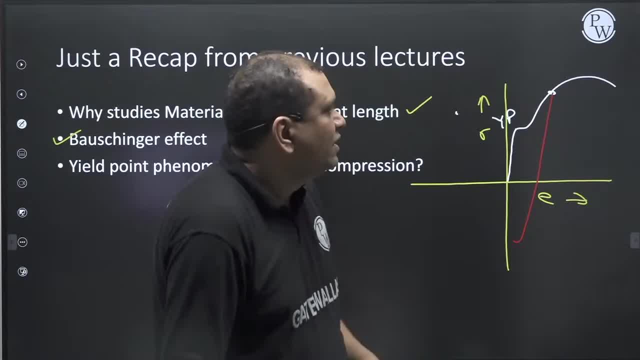 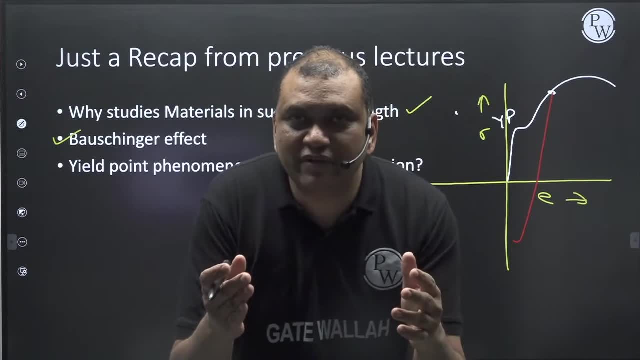 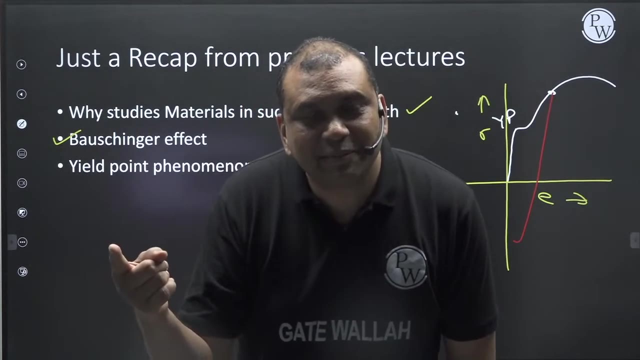 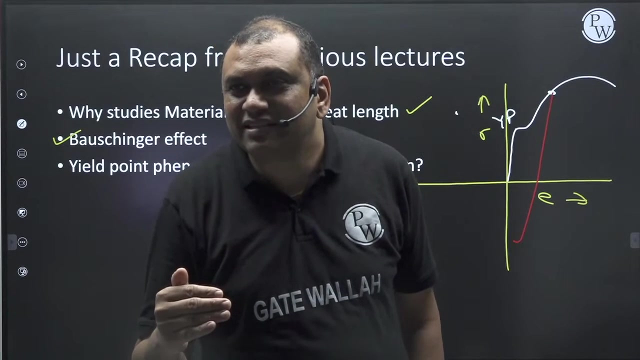 because this is also coming in geotechnical. please see that. so see you suddenly put compression so the dislocation start moving in the opposite direction. dislocation started moving in the opposite direction, so the back stress now starts supporting the movement of dislocation. back stress starts suddenly moving in the opposite direction. 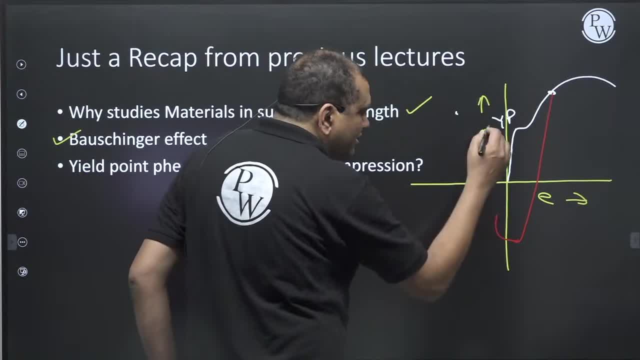 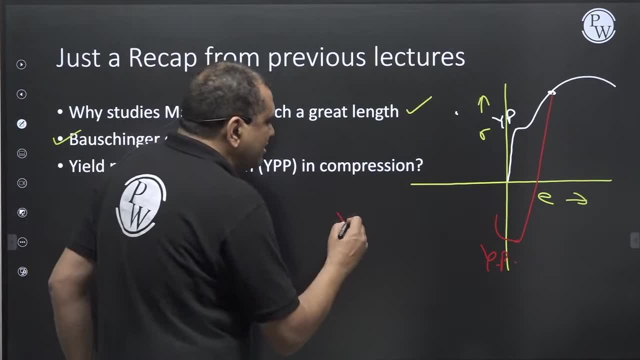 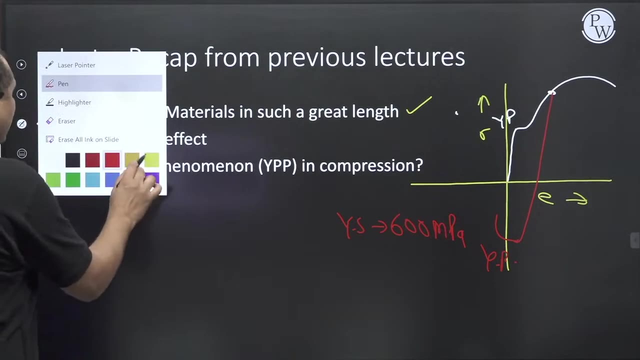 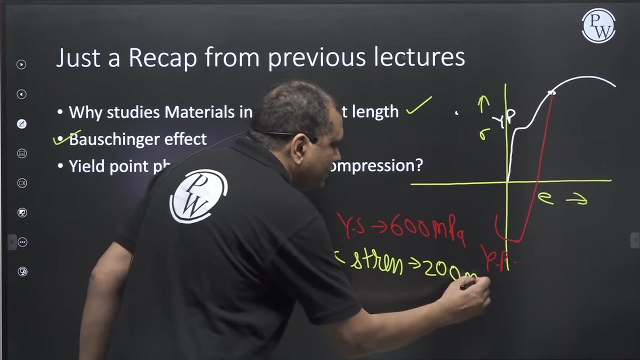 so its yield point in compression will appear prematurely. what does this mean? let us say yield strength in compression was 600 MPa and the back stress which was developed, the back stress which was developed, that is 200 MPa. so your yield point will come on 400 MPa. 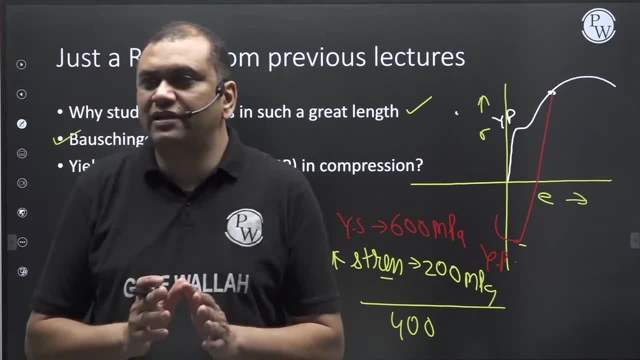 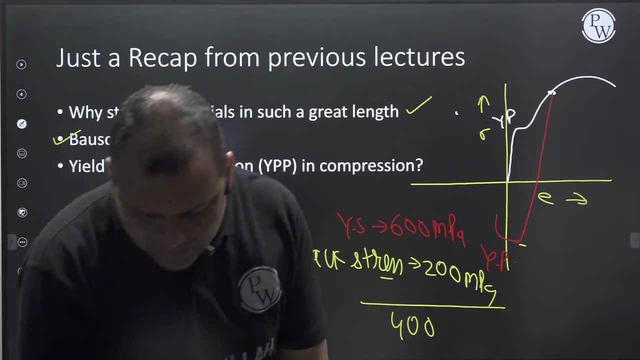 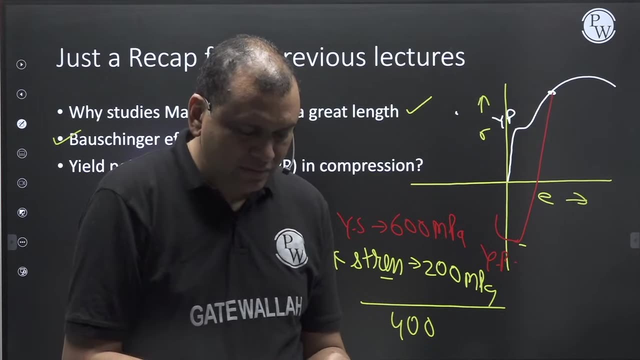 it will come on 400 MPa. it will come on 400 MPa if your yield add on 400 MPa. that is this particular value. so the back stress is now 80 MPa. if your yield point is 800 MPa, then the back stress is now 10 MPa. 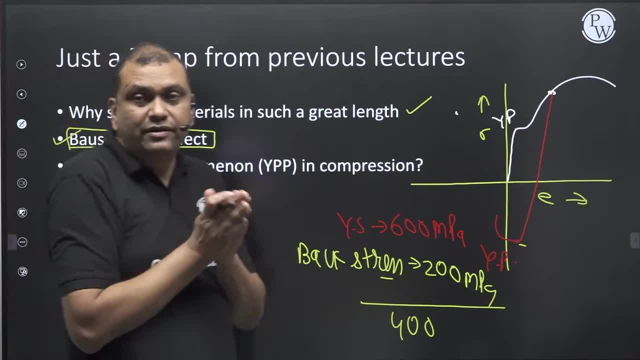 so the back stress is now 100 MPa and the front stress is now 80 MPa. for the back stress, if the front stress is now 20 MPa, then the back stress is now 100 MPa. So this is the second case. 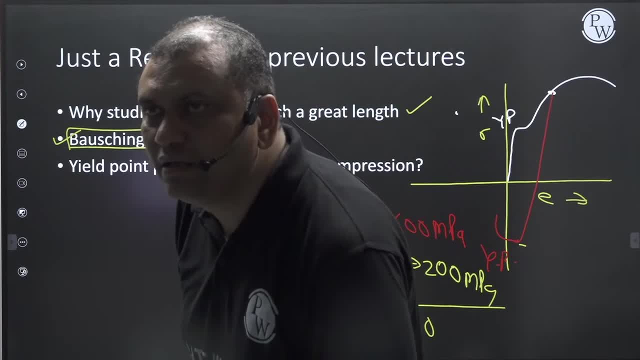 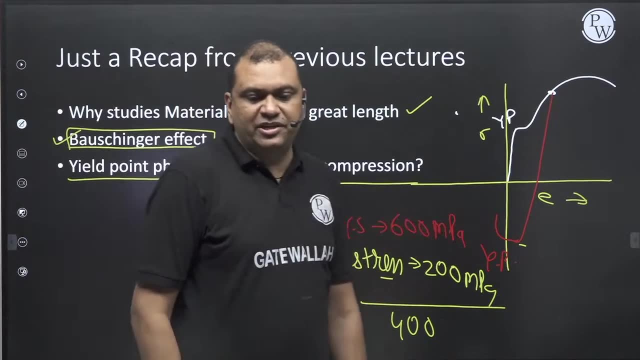 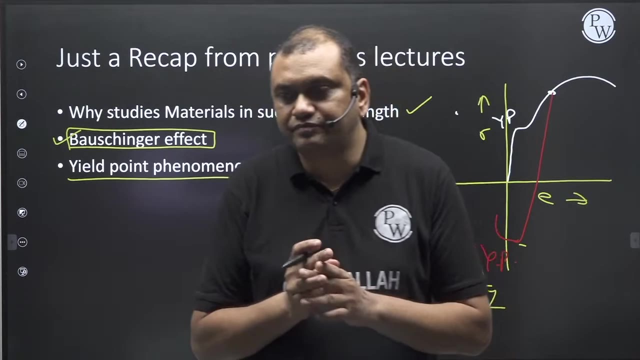 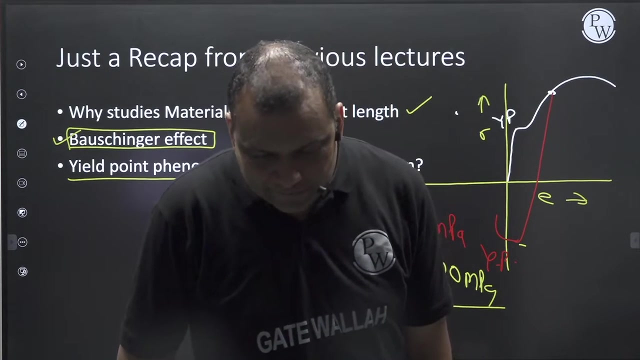 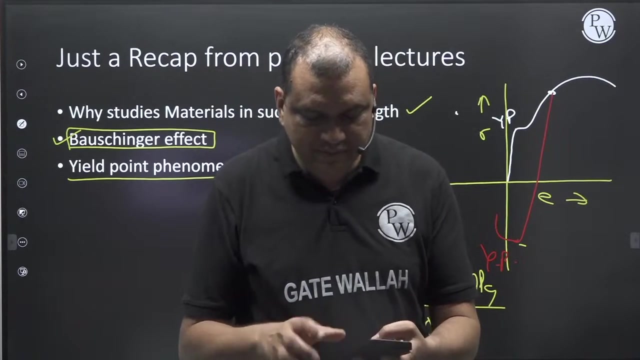 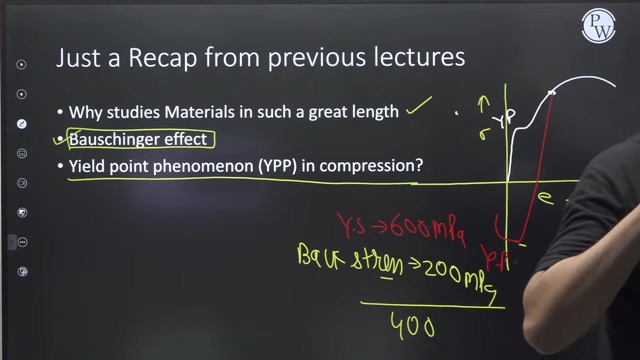 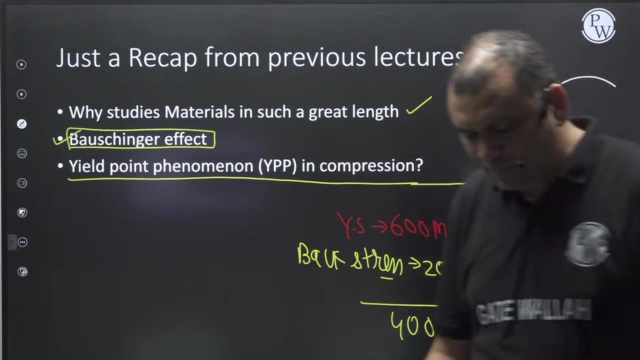 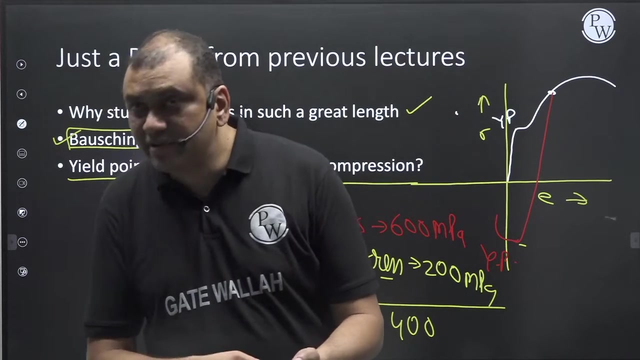 This was your second doubt, wasn't it? Now the third question. this question was asked by many students. This third question was asked by many students. We haven't seen the yield point phenomenon in tension. Just, I will pause it for one minute, You have to see, because I am trying to call my back-end person. 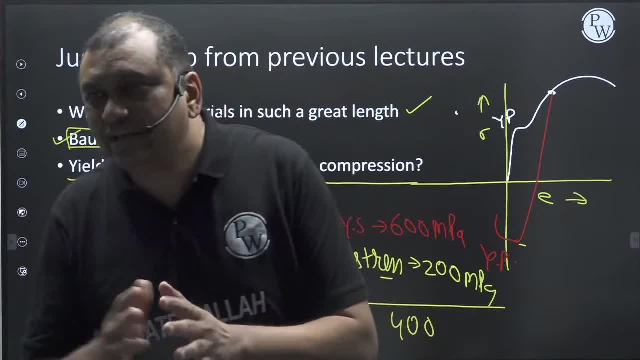 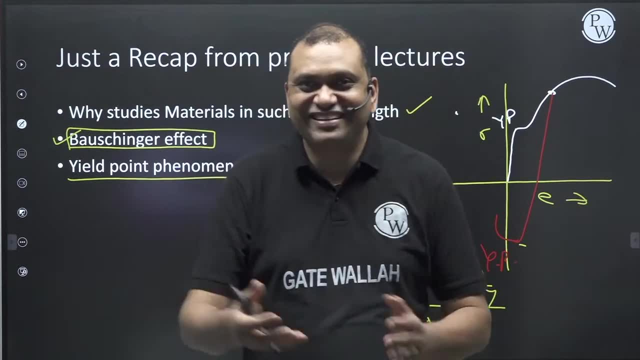 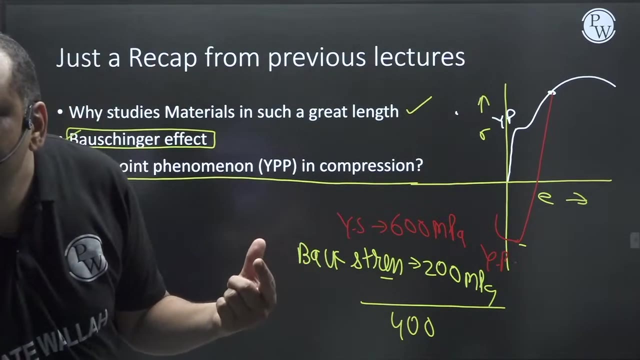 His phone is engaged, So I think they will correct it. just wait for two minutes, Because you are also our students. You are also our children. Now, this question was asked by many students. That Yield point phenomenon is a phenomenon. We have seen the yield point phenomenon in tension. 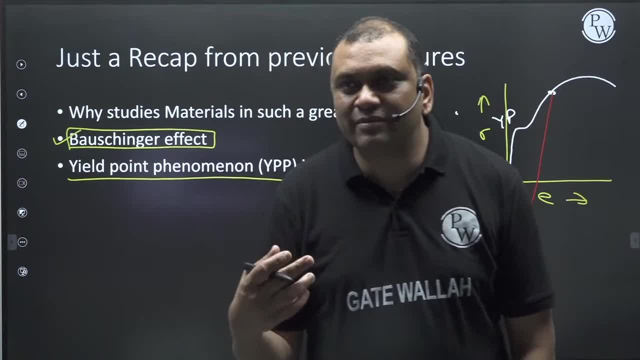 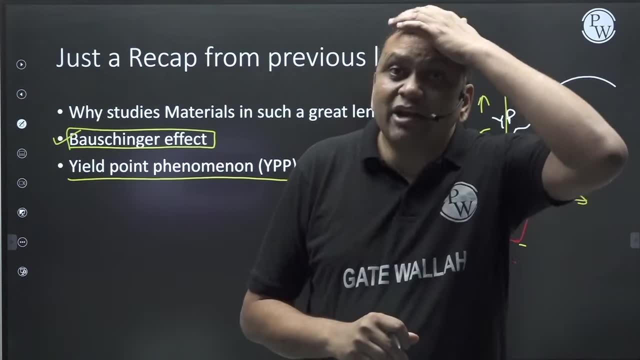 What will come in compression? In fact, some students were telling, Sir, our teacher has taught that There will be a yield point phenomenon in compression as well. I asked them to ask in which book it is written: Yield point phenomenon will not come in compression at all. 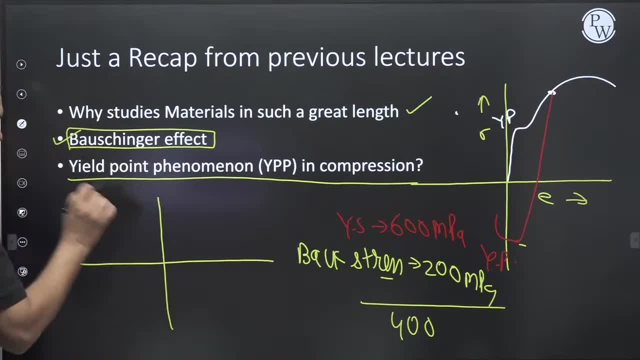 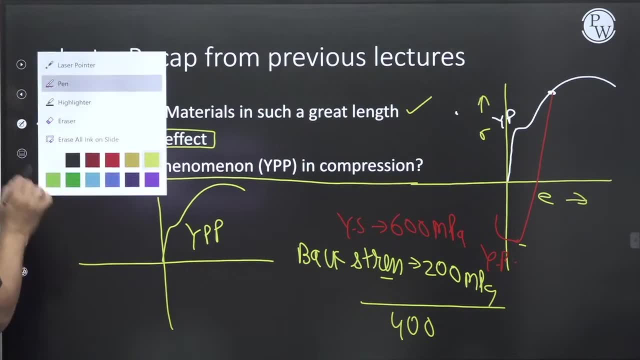 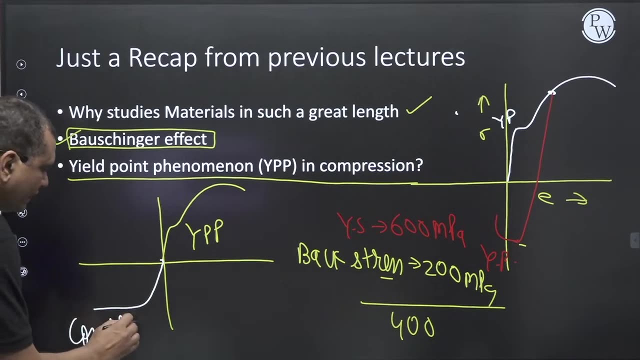 Because its mechanism is a little different. The way your yield point phenomenon came, Let us say in tension, The curve in our compression, It will be a little different. Something like this: Compression In compression, Because the failure in compression is due to buckling, Half planes are coming out. 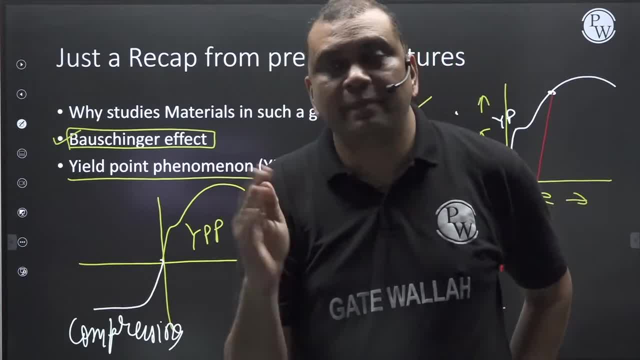 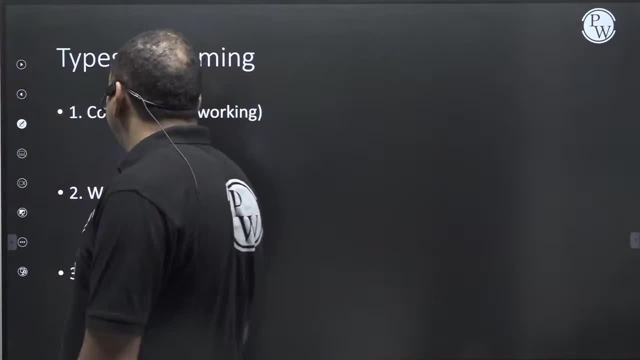 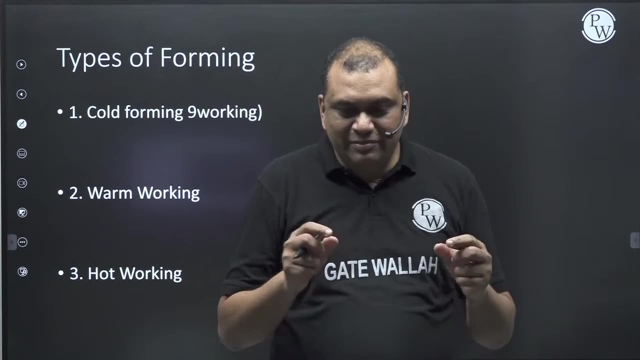 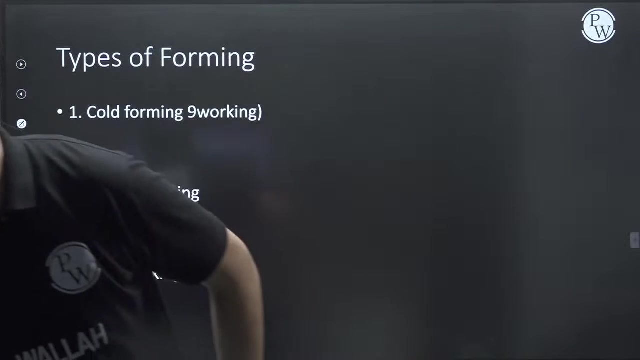 So you have to keep in mind that The yield point phenomenon, It will never come in compression. Alright, that was the discussion. Some questions Now forming, Okay, Okay, once again, I will request you all: You Be a little attentive today. You be a little attentive today. This is a little bit in RK engineers. 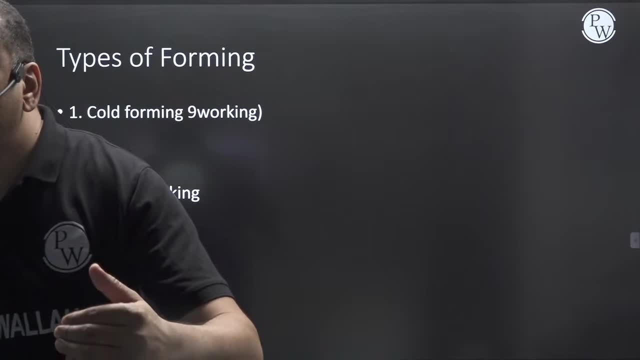 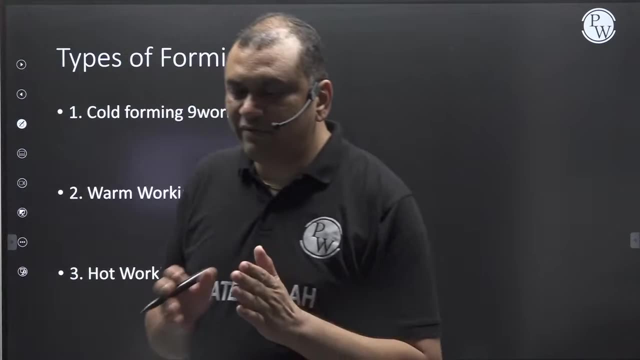 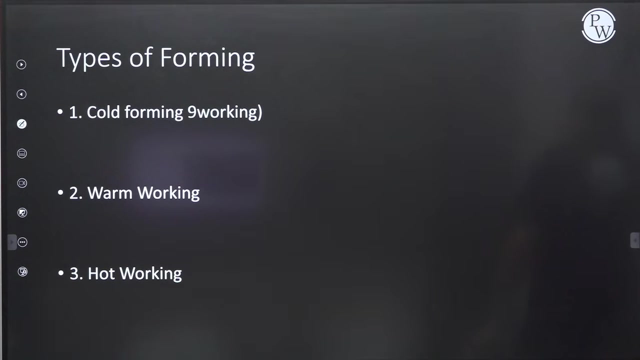 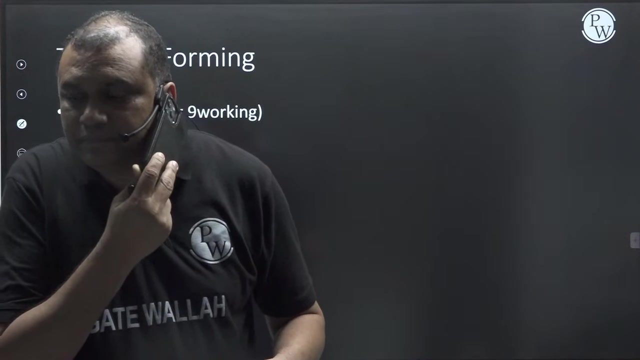 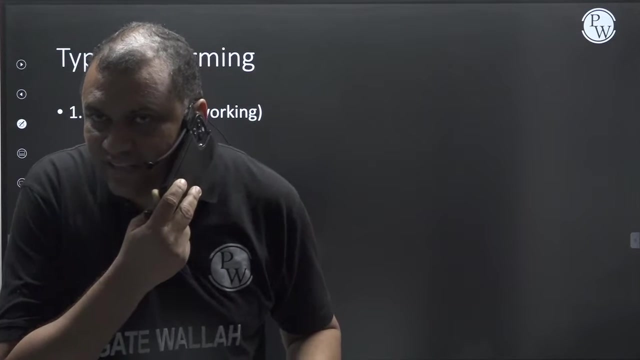 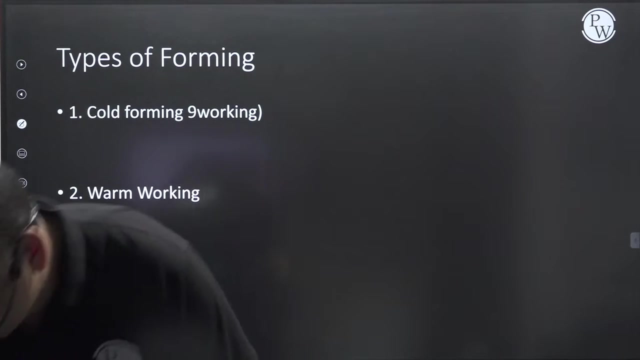 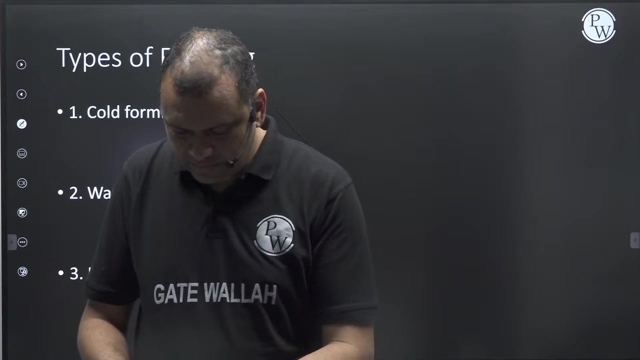 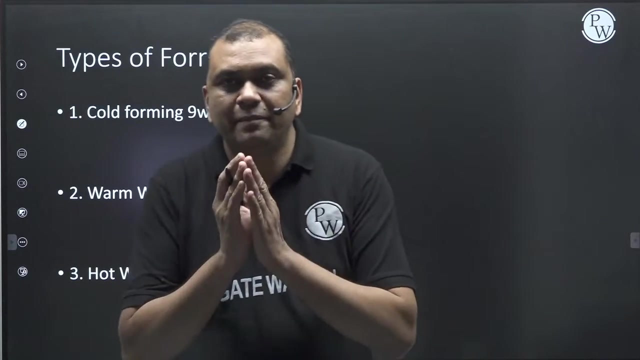 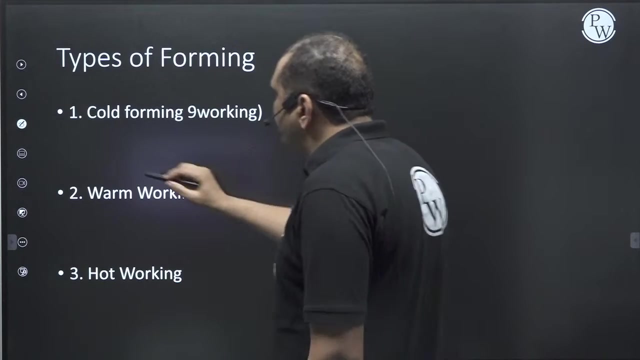 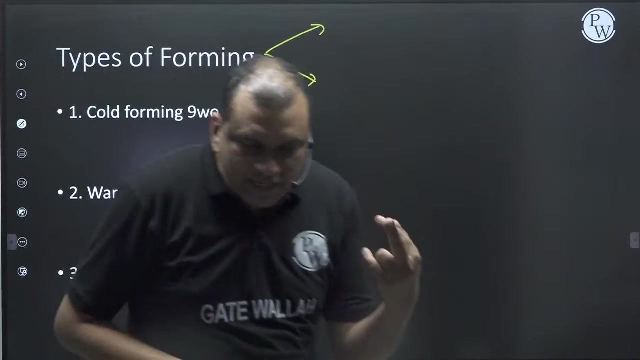 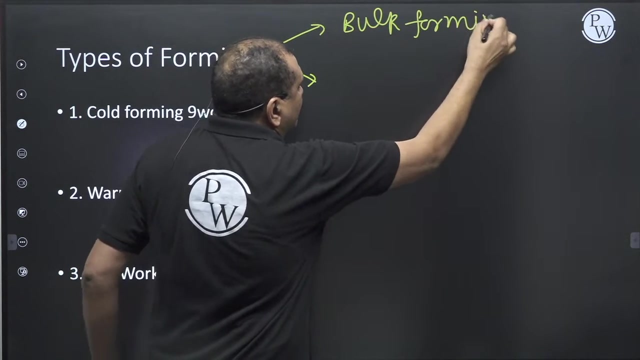 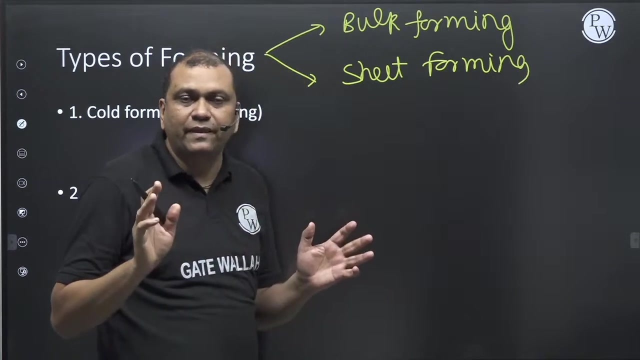 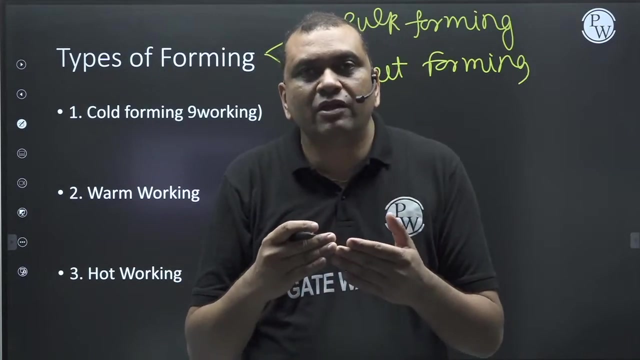 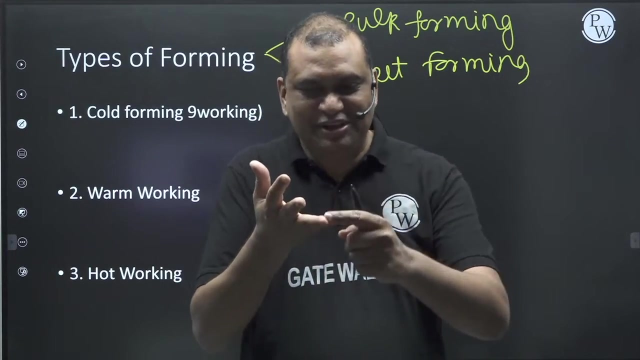 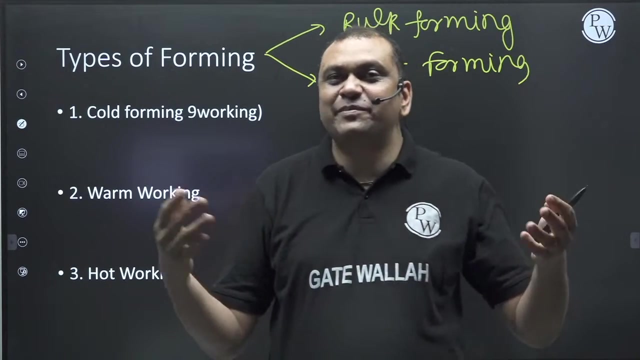 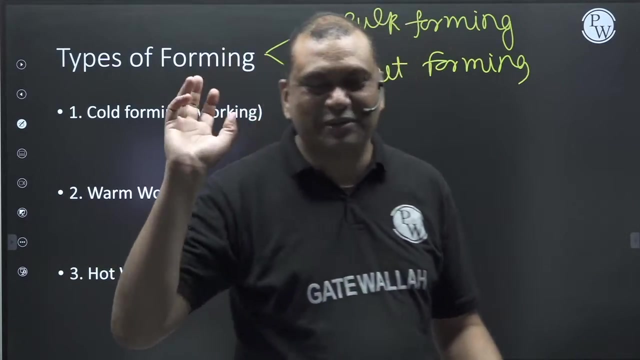 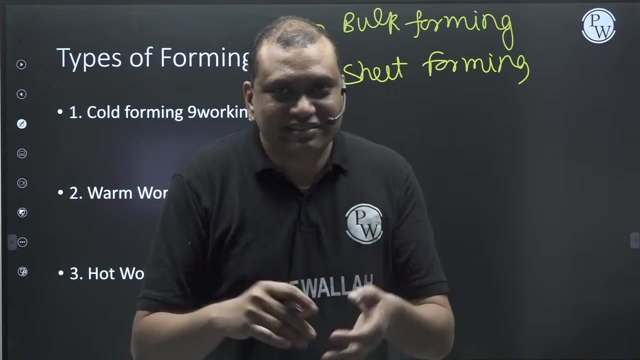 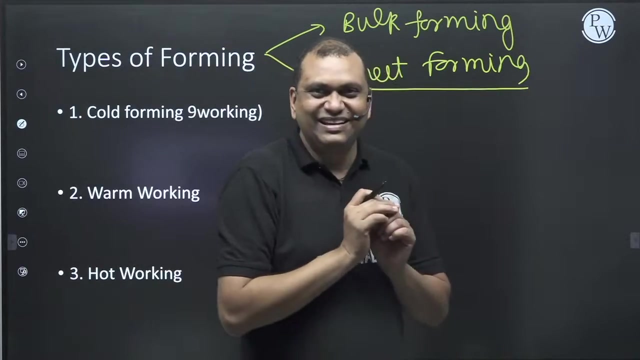 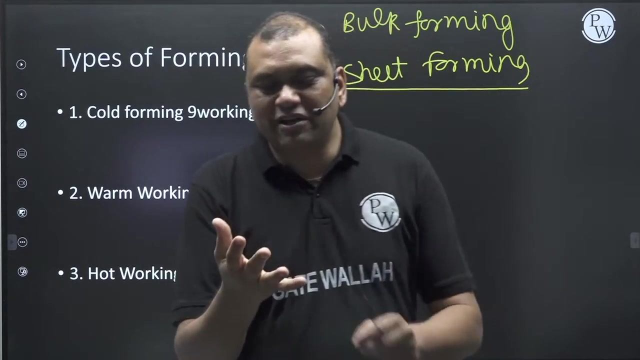 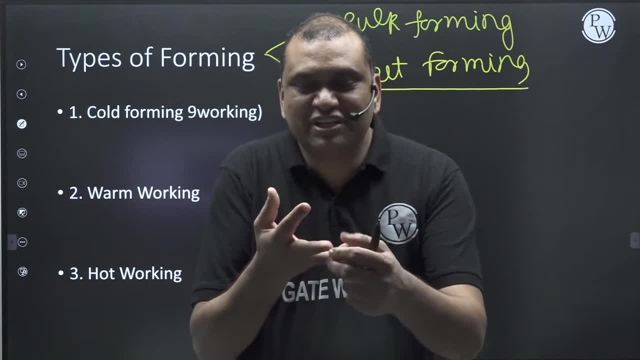 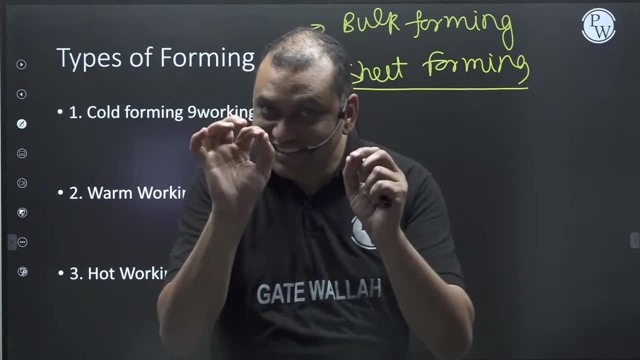 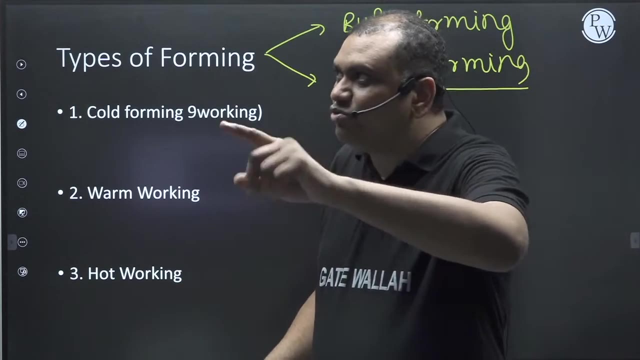 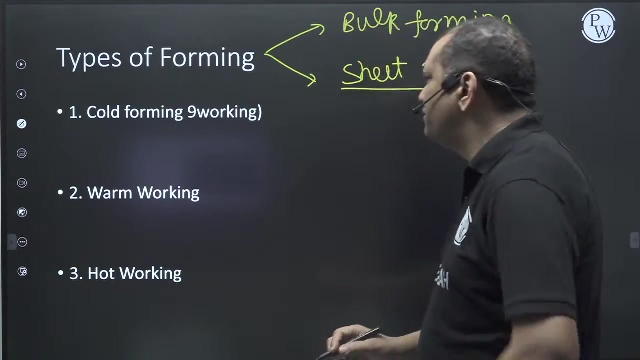 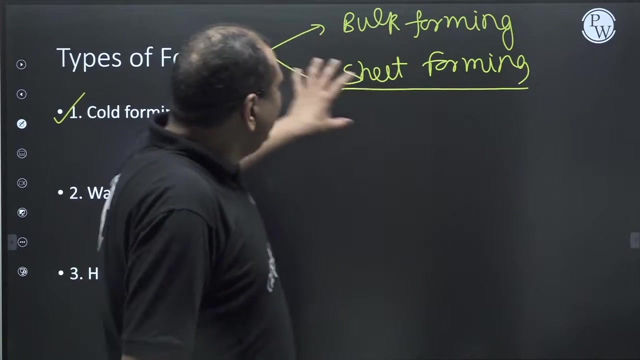 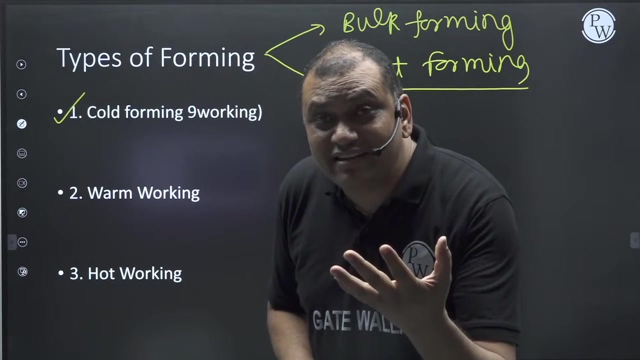 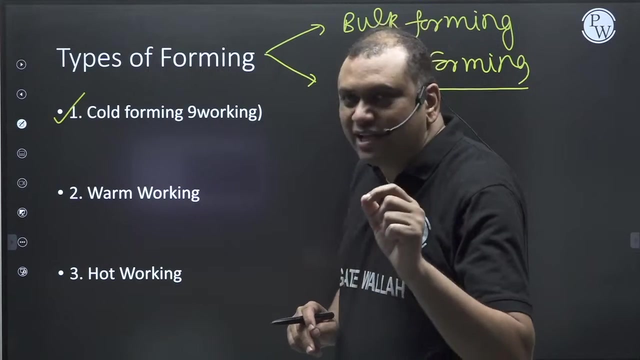 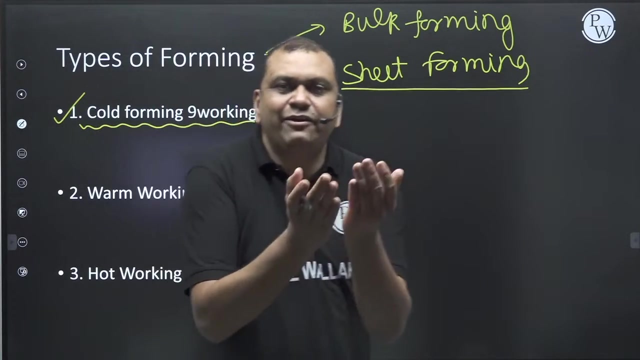 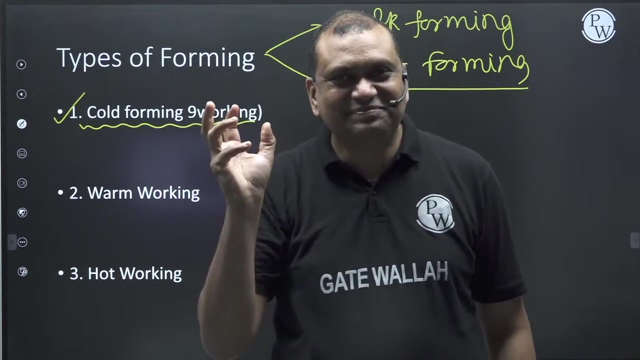 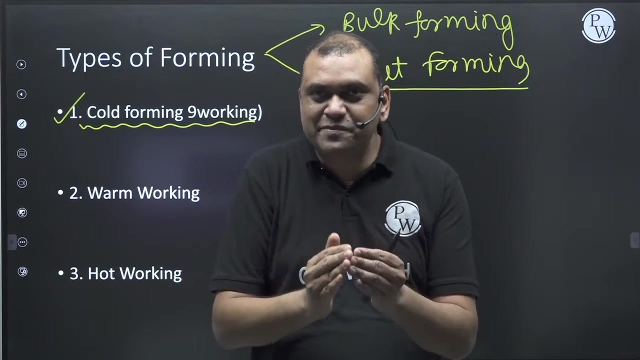 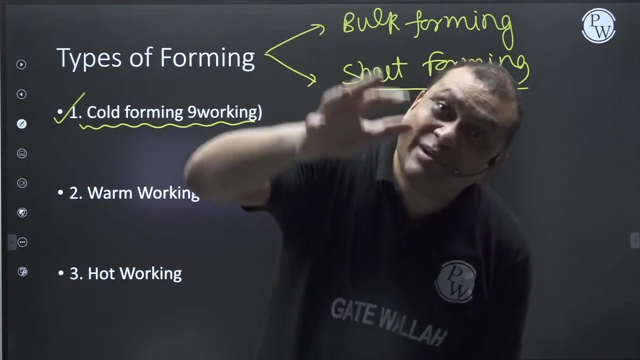 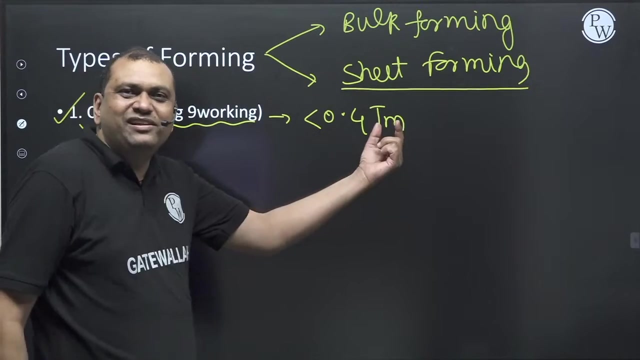 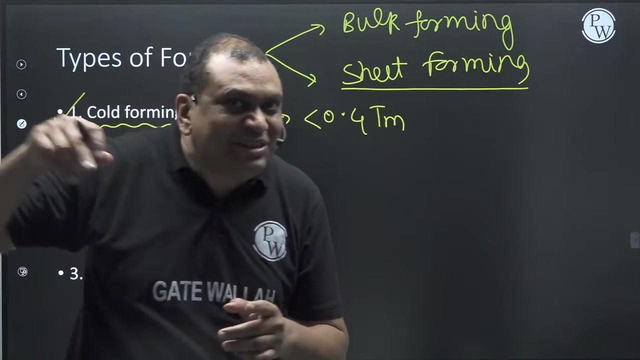 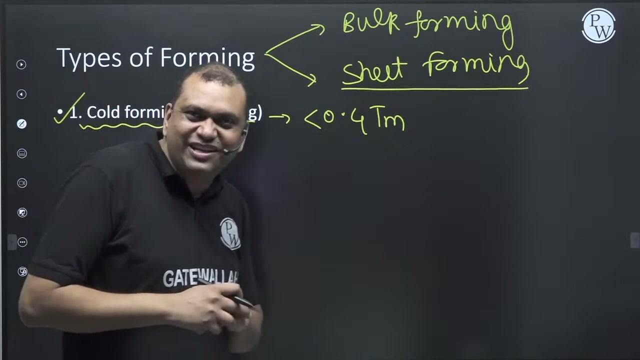 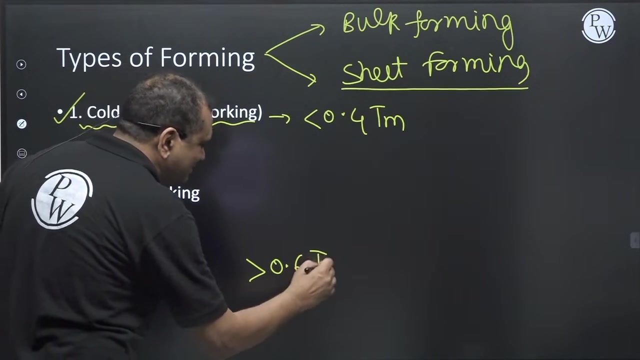 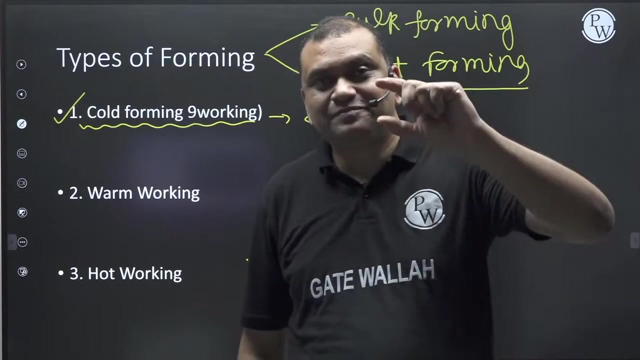 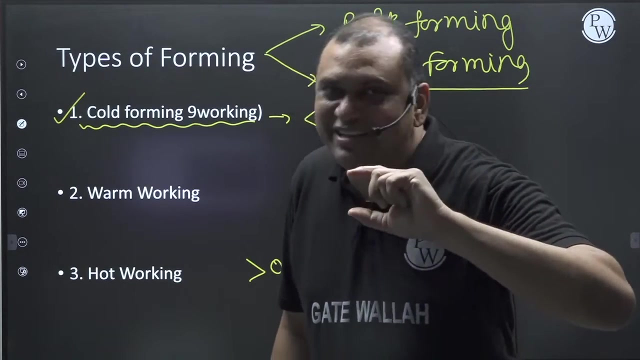 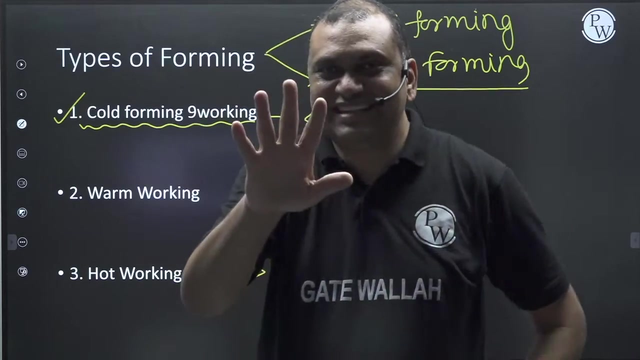 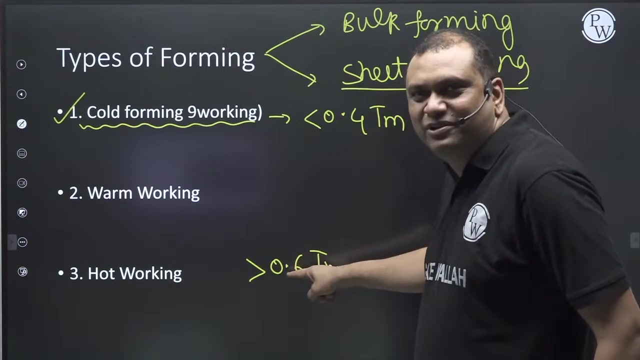 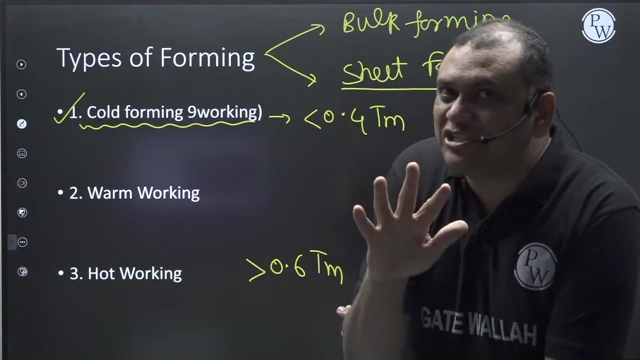 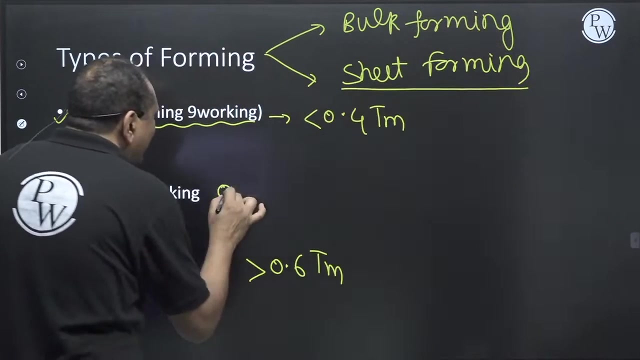 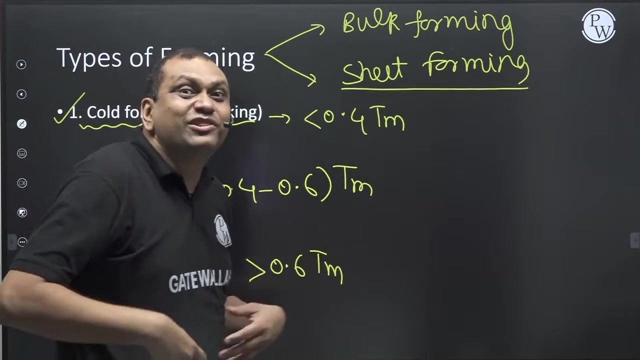 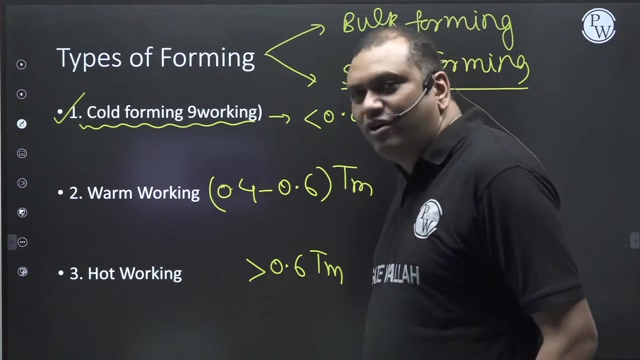 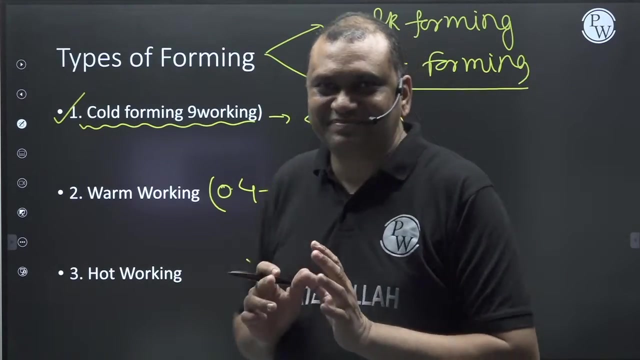 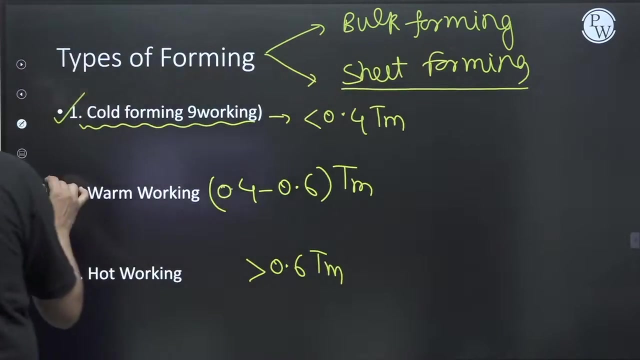 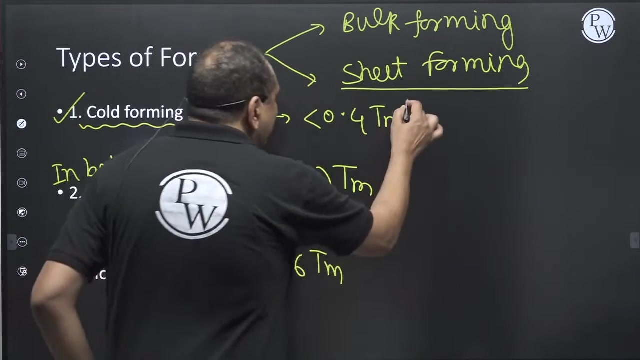 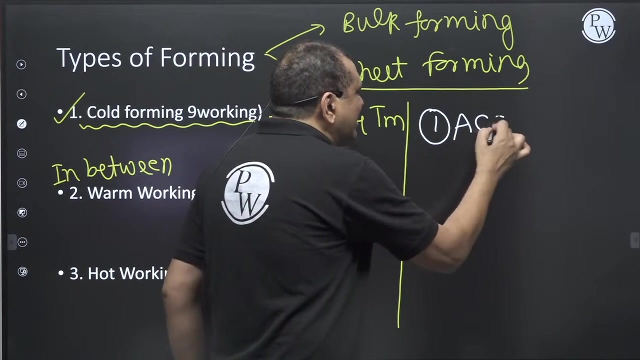 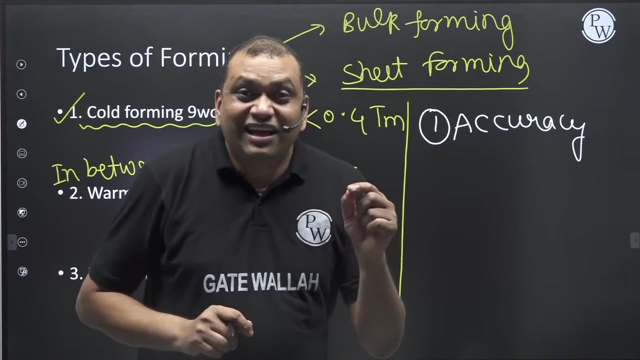 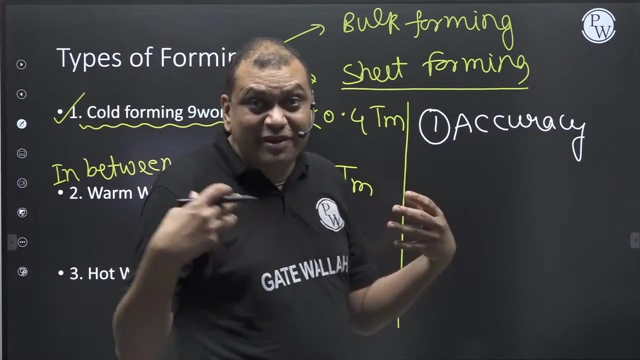 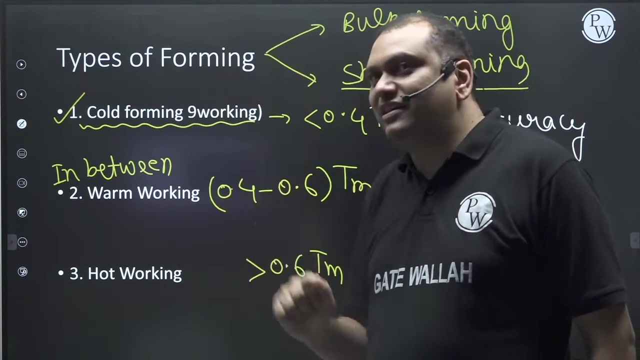 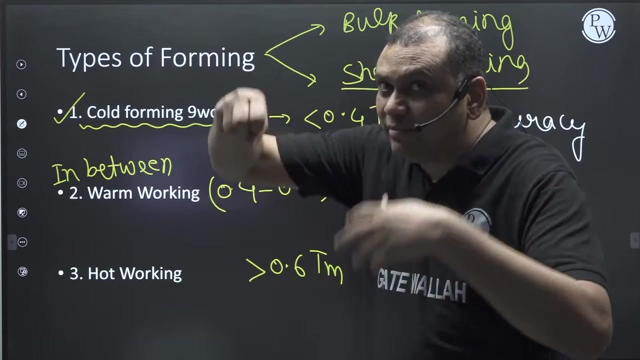 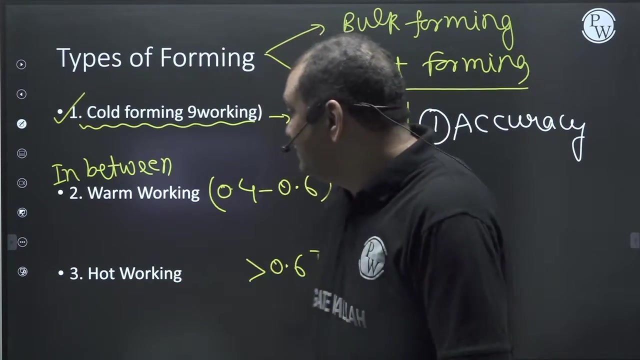 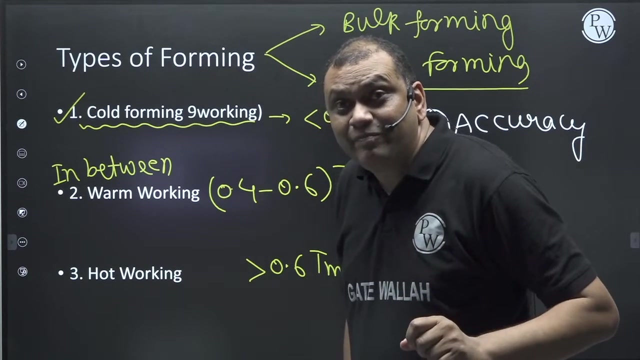 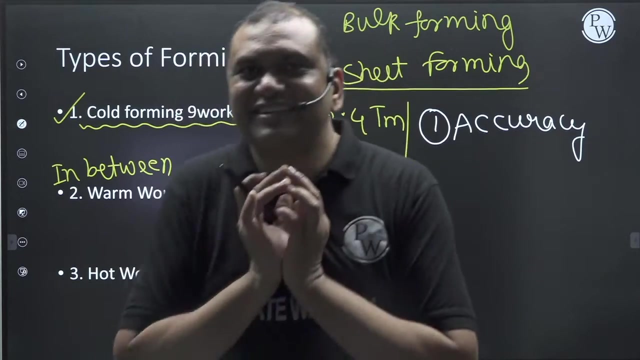 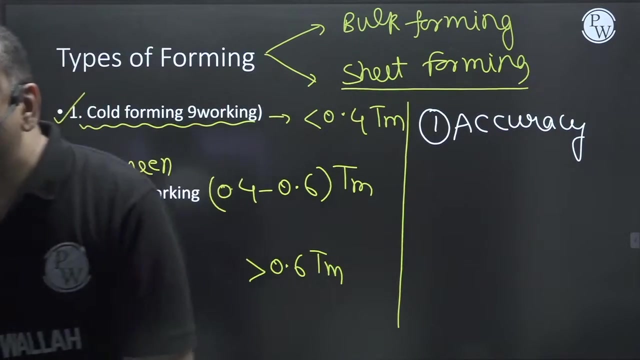 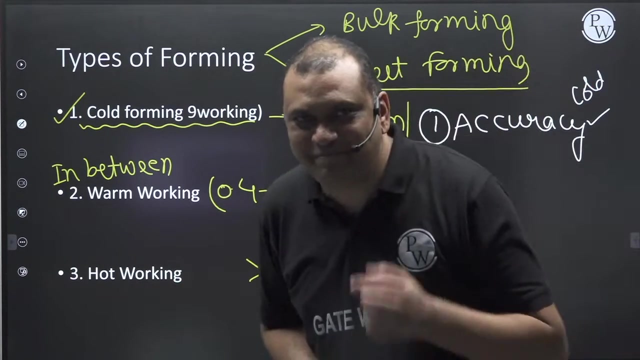 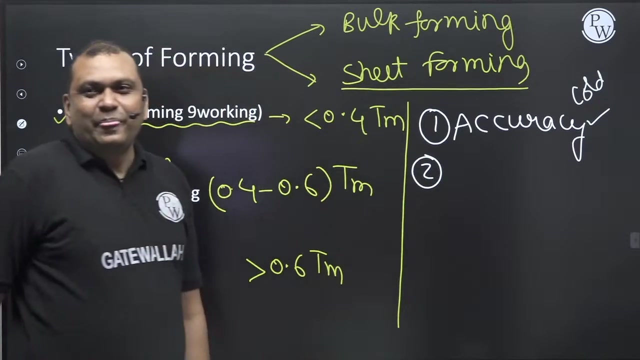 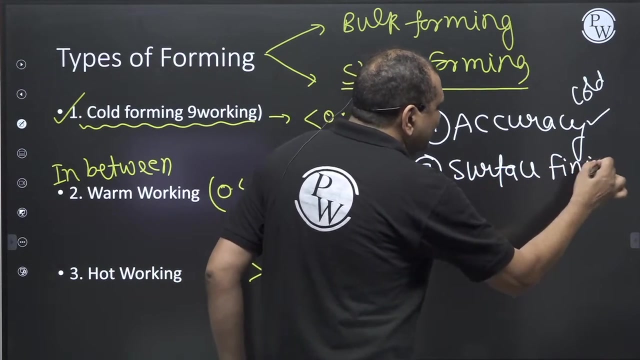 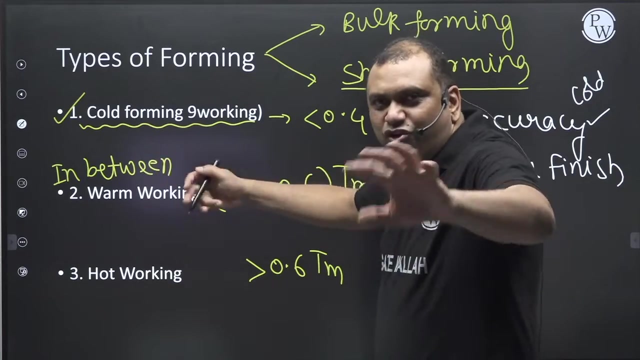 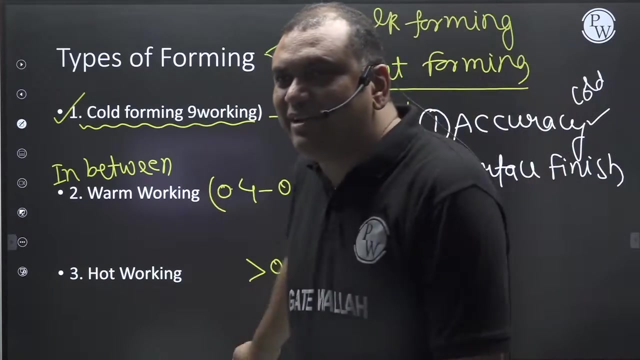 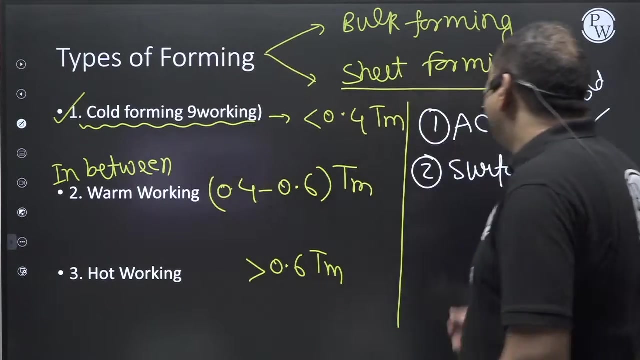 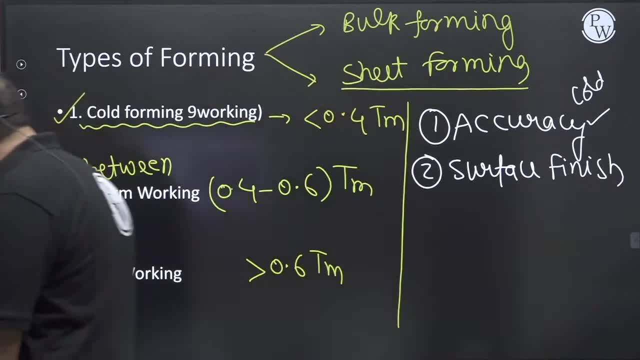 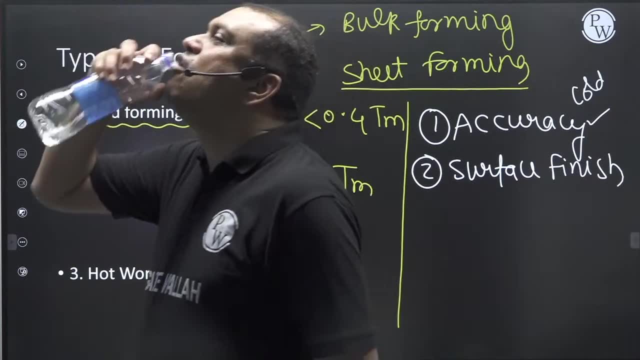 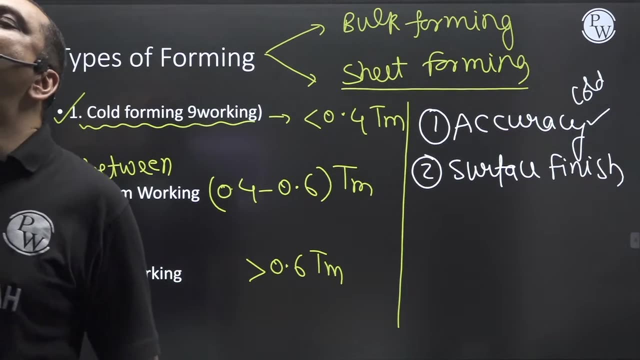 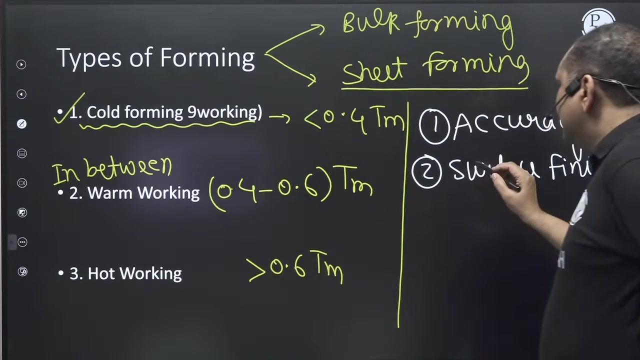 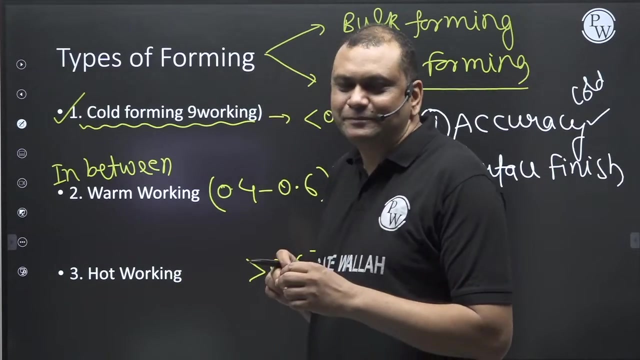 Thank you, Thank you. surface finish, which I am writing- you can write in the chat box because I am seeing that some of you are really brilliant- or Ashok. the surface finish will be bad in hot working. surface finish will be bad in hot working. do you know why? 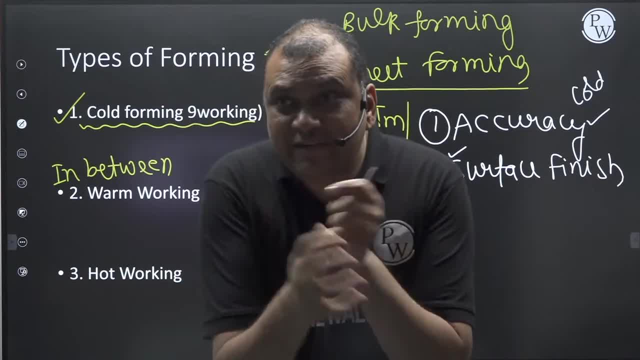 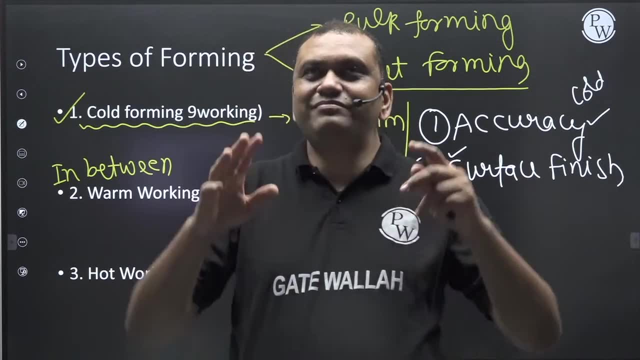 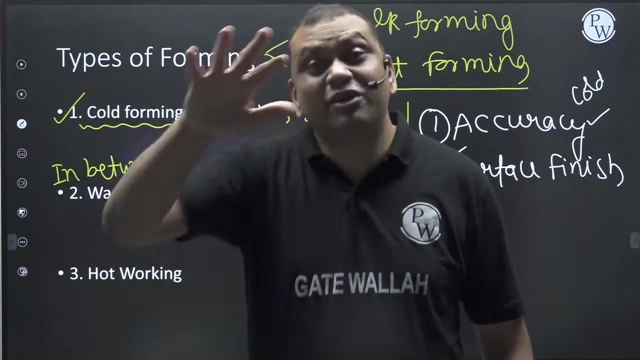 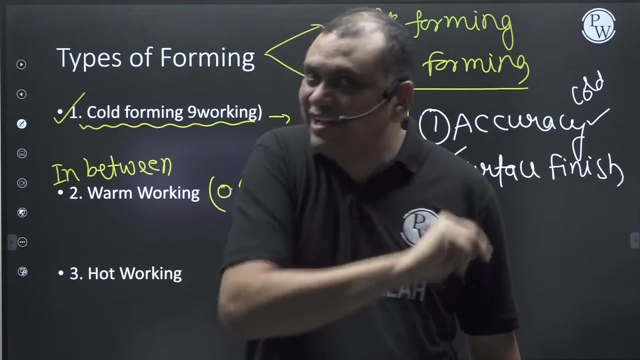 the surface of our work piece at high temperature, the hot working surface. in hot working the surface of the work piece becomes oxidized. oxide forms over the surface of the work. so oxide is a foreign element. oxide is a foreign element. so when our work piece comes at room temperature, 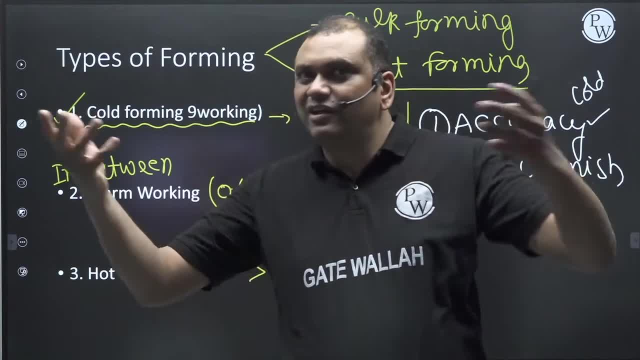 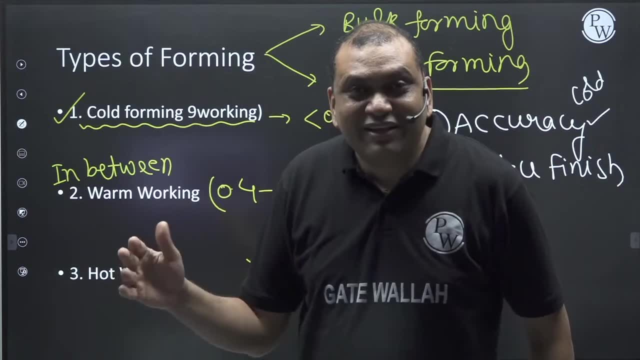 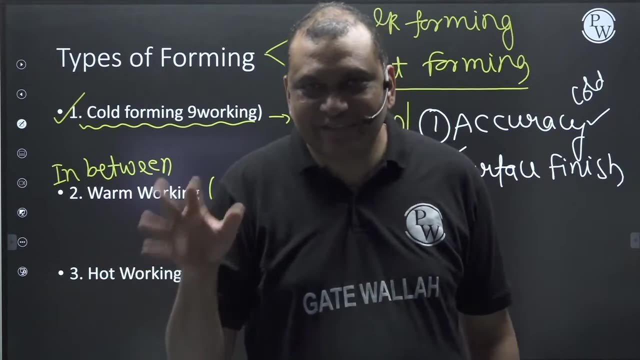 then the oxide around the work piece will fly away. it will be removed automatically because it is a different material, and when the oxide goes away, then the outer surface will become rough. the outer surface will become rough. so in which way does our surface finish get better? 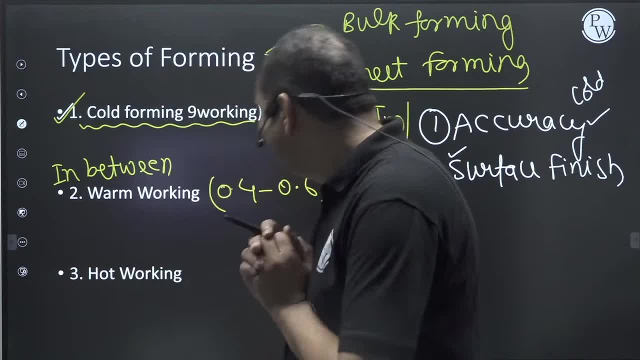 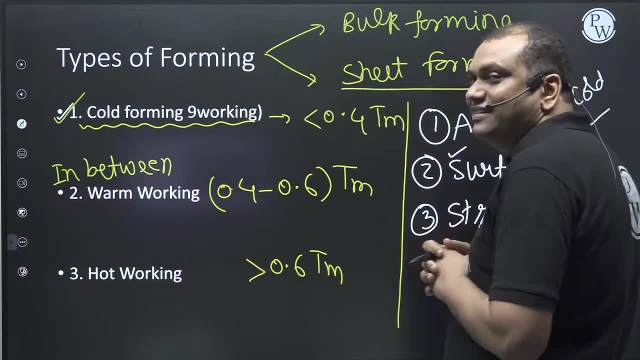 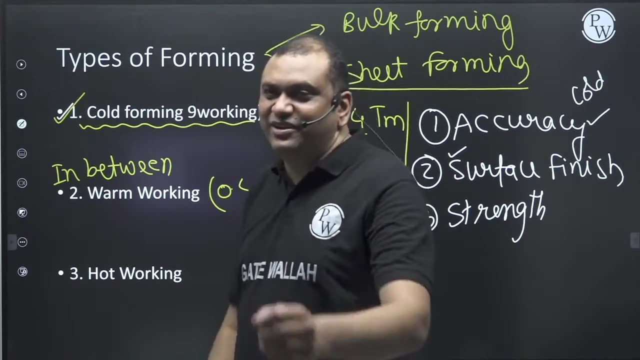 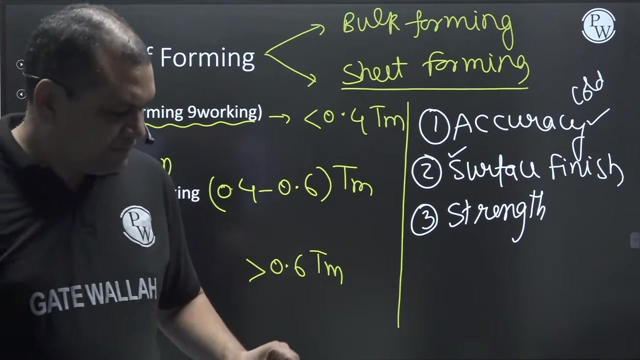 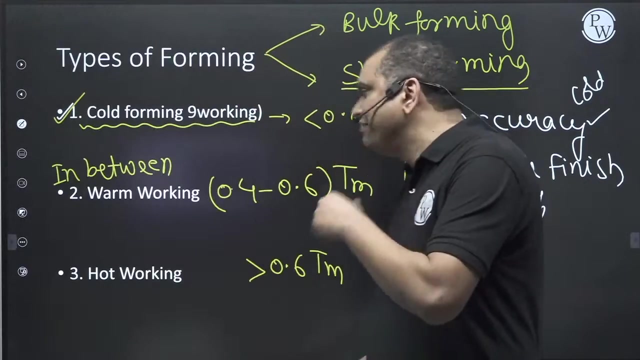 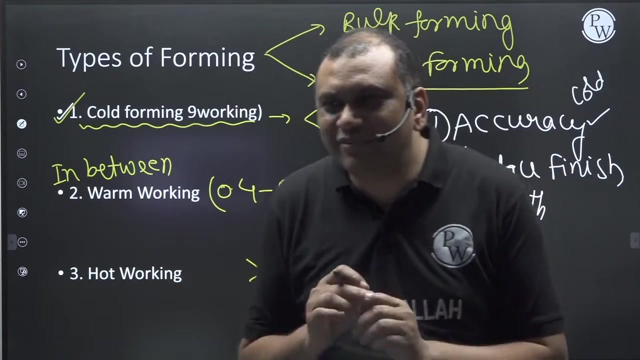 in cold working, isn't it next, strength, strength, in which working, the strength of the product will be better, in which the strength of the product will be better, the strength will be better, very good- in cold working. in cold working, there will be dislocation, pile up. 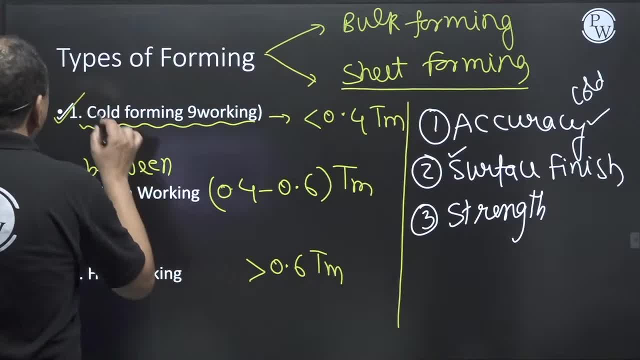 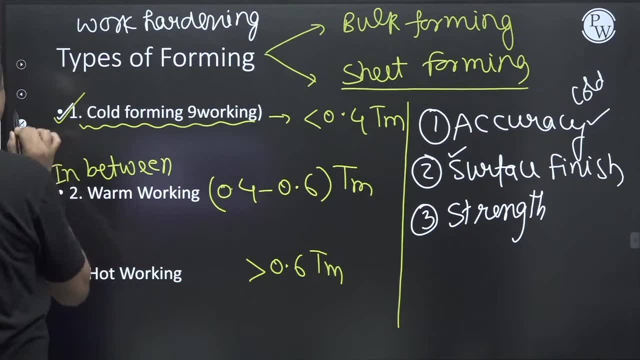 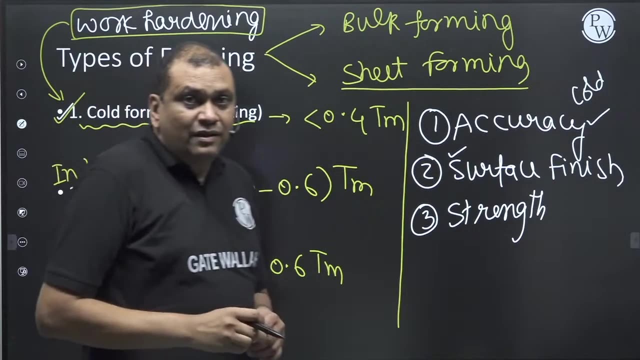 you can also say this in English: there will be work hardening. there will be work hardening, excessive work hardening. there will be excessive work hardening in the cold working. what happens? because of excessive work hardening? the product will be stronger. all of you are correct. 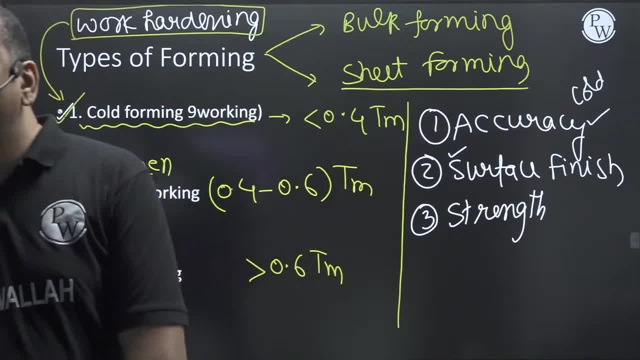 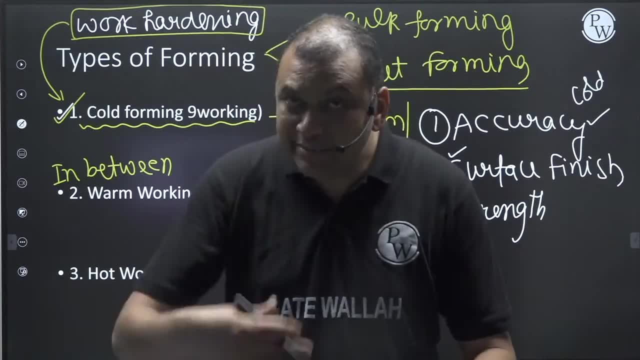 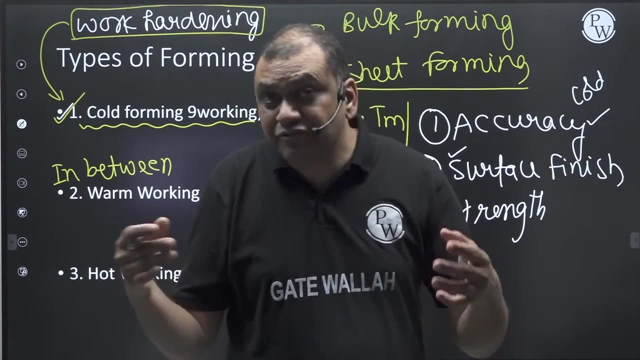 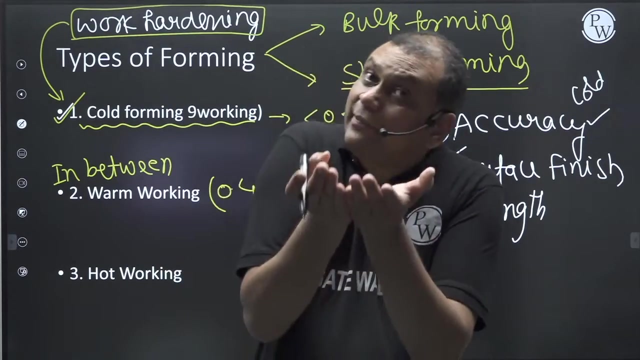 very good. Anshu Jayesh, Aditya Harsh. everybody is correct in that what happens in hot working- there was a discussion in material science as well- as you are forming by the plastic deformation, there will be dislocation, pile up, but because the temperature is above the recrystallization temperature, 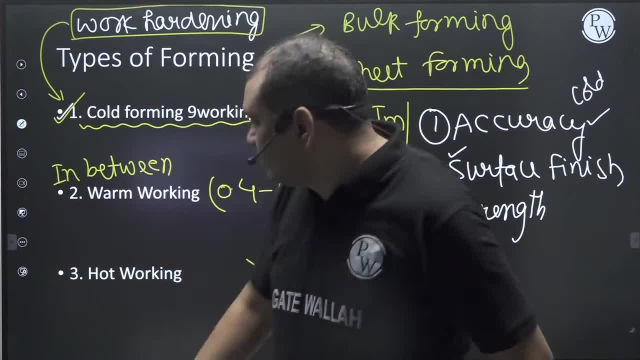 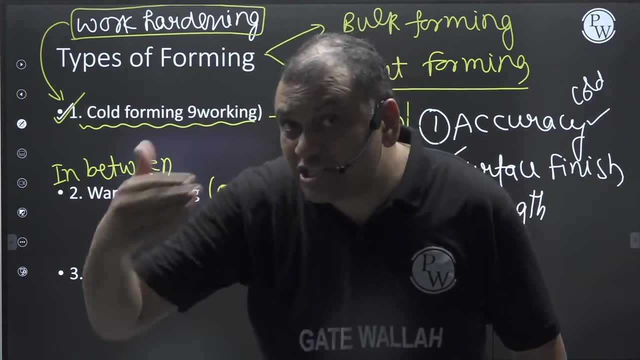 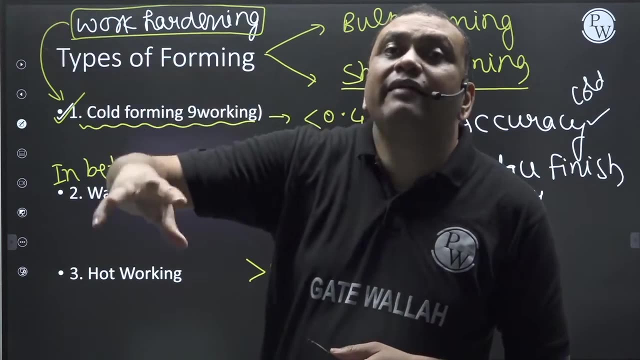 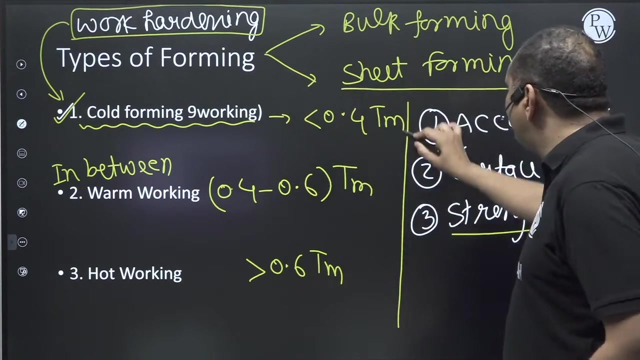 because our temperature is in hot working, recrystallization is above the temperature. so due to recrystallization, new crystals will be formed and the dislocation on the grain boundary- they will die out. they will die out. so there will be strength in cold working. 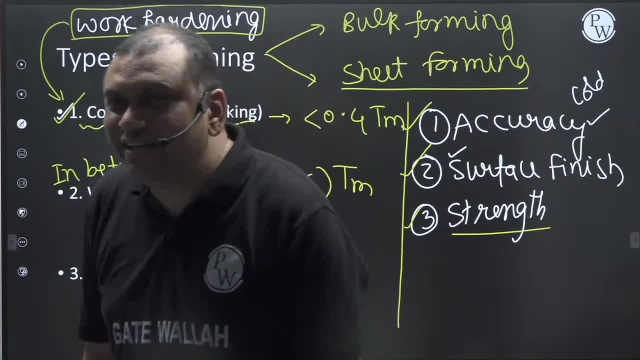 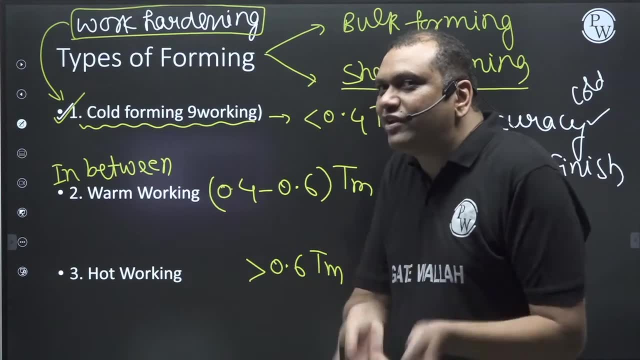 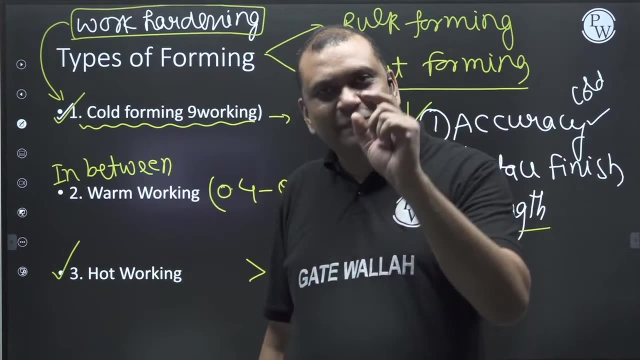 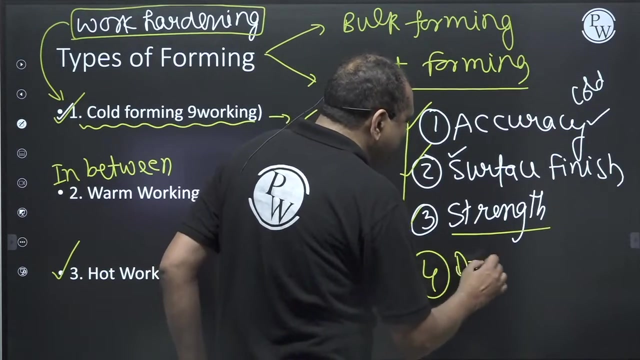 so whatever option you have seen, all are cold working, everything is cold working. so why are we using hot working? we are using cold working only. why do we use hot working? hot working: there is an advantage in one place drawing force. drawing force will be minimum in hot working. 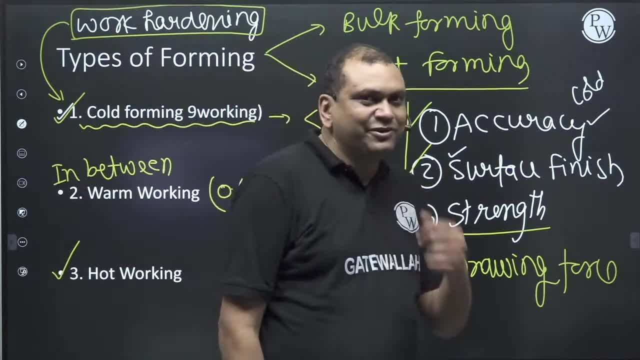 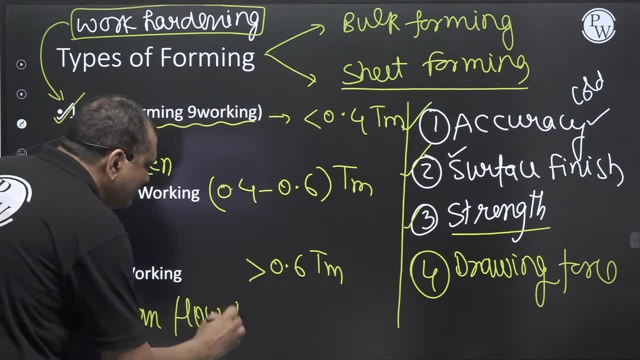 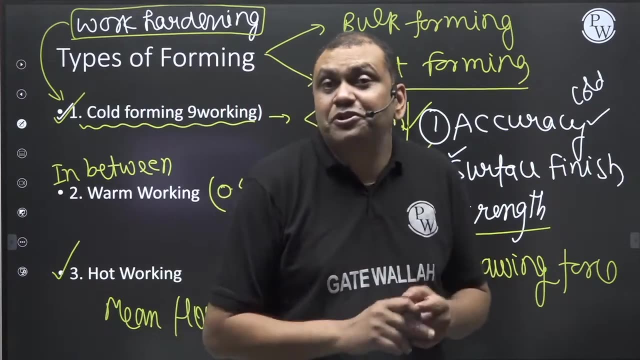 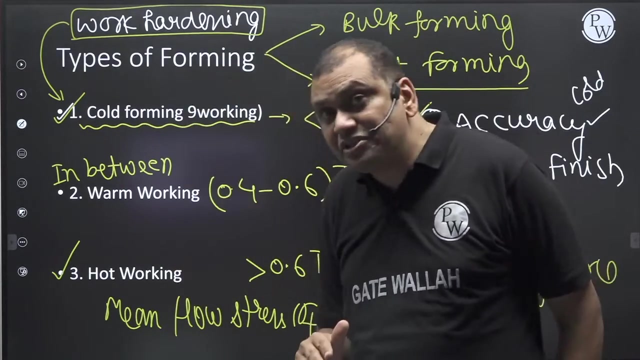 drawing force will be minimum in hot working. do you know why there is something called mean flow stress? there is something called mean flow stress, sigma fm. by increasing the temperature, mean flow stress decreases, like we had studied in last two last lecture. stress strain diagram at different temperature. 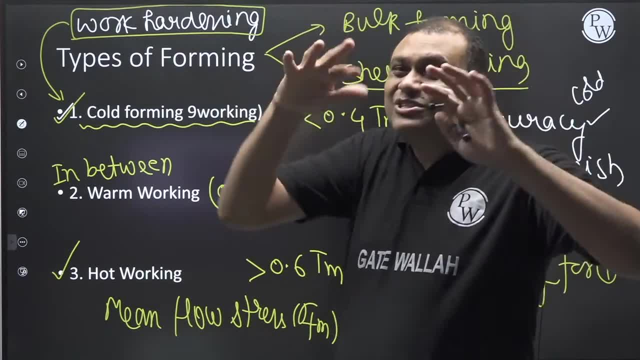 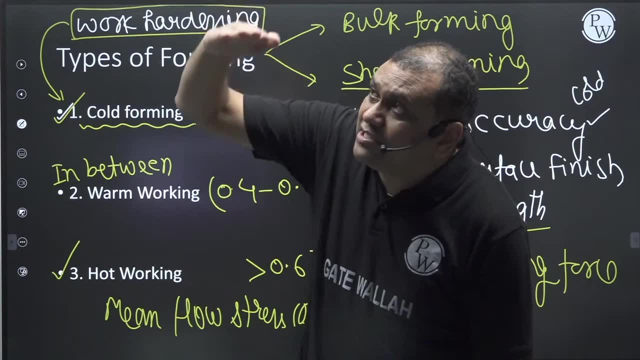 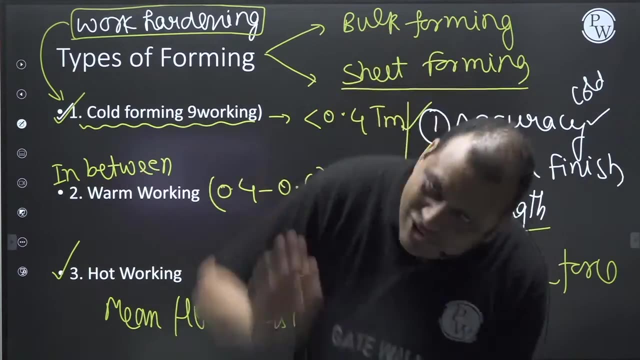 so we had studied there. if suppose there is no chromium? if there is no chromium then our stress strain curve will keep. coming down means yield strength and ultimate tensile strength. both will decrease and if both decrease then the average flow stress will decrease and due to that 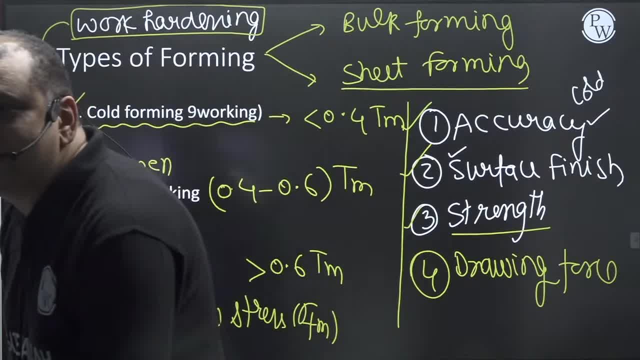 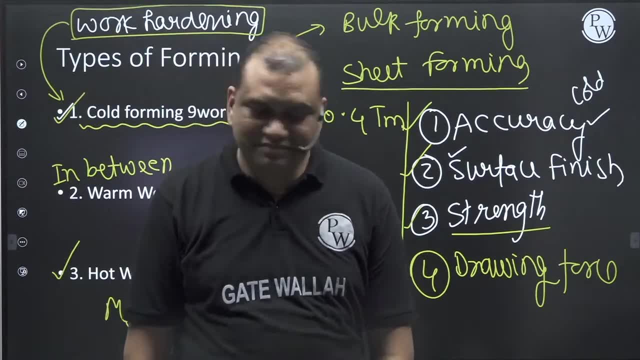 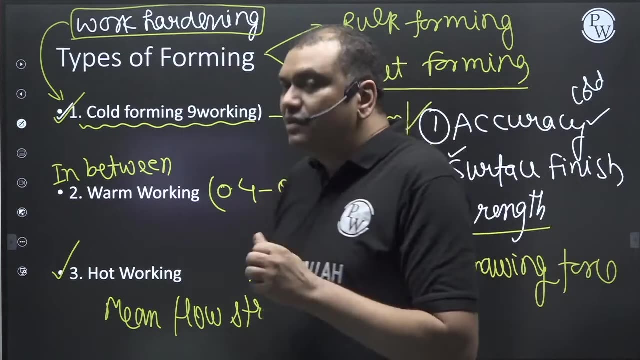 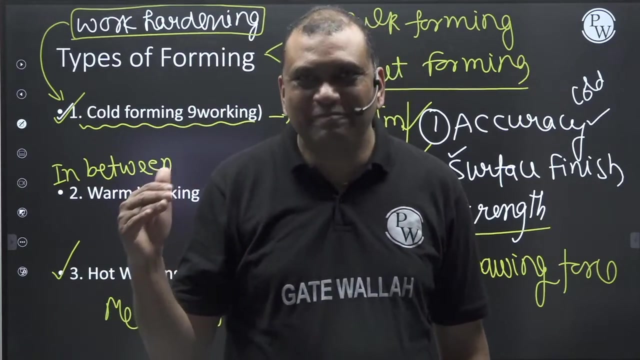 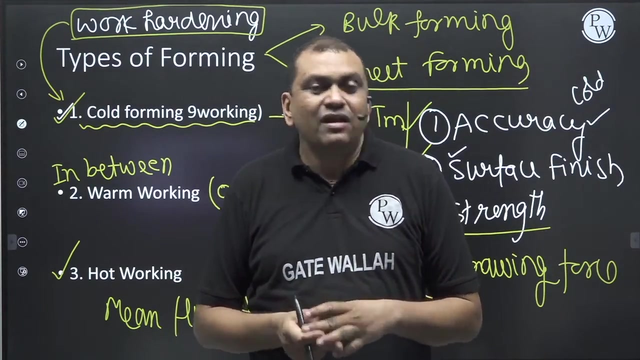 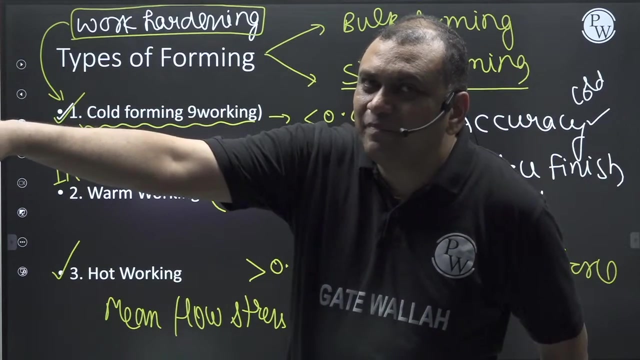 drawing force will be less. drawing force will be less. new grain formation will take place in the. there is no chromium, also plate formation. you will have more. there are more, many more. you can learn all this in the next class. ok, bye, bye, it will be treated as a different grain. 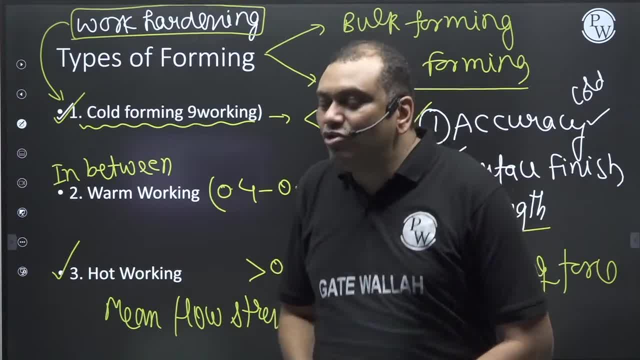 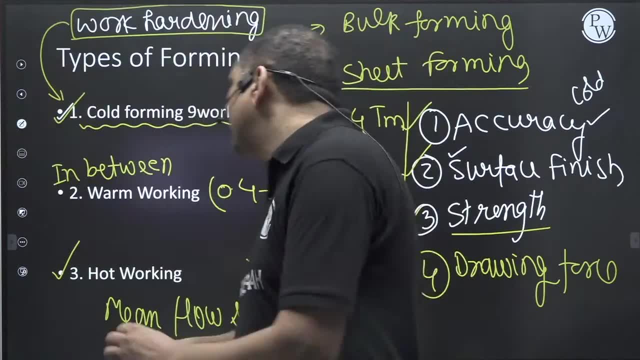 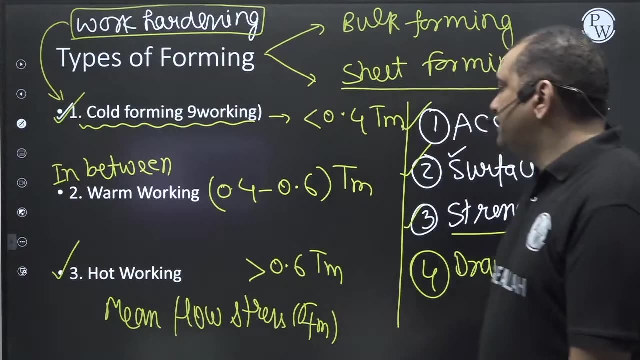 but if you talk about grain growth, it will be in hot forming. in cold working. wherever there is an excessive dislocation, pileup, that will be treated as a different grain. this was your answer. so cold working, warm forming and hot working: Lucifer death if our material is brittle. 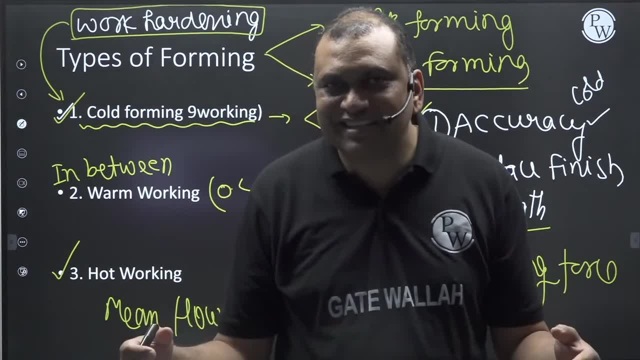 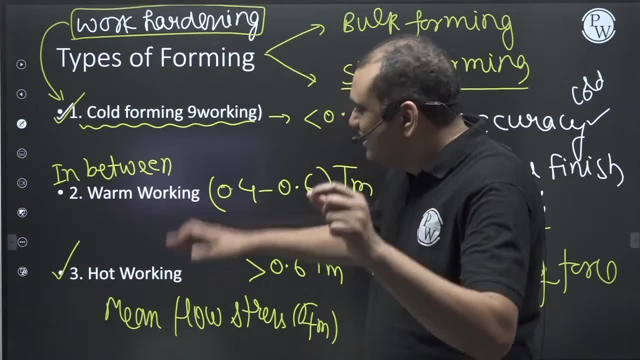 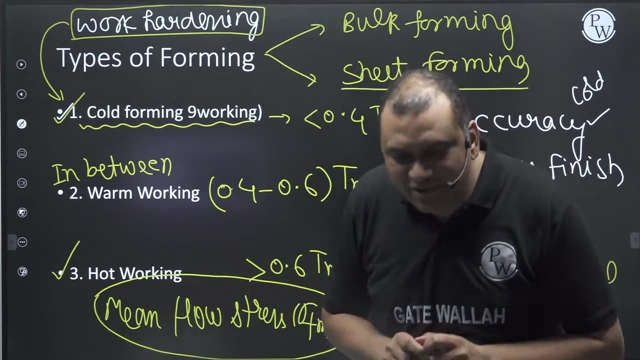 we do a special thing for that. I will tell you after an hour. I will not tell you now. now see what is the advantage of cold working? the biggest advantage of hot working is it reduces the mean flow stress, and by reducing the mean flow stress you will get less force. 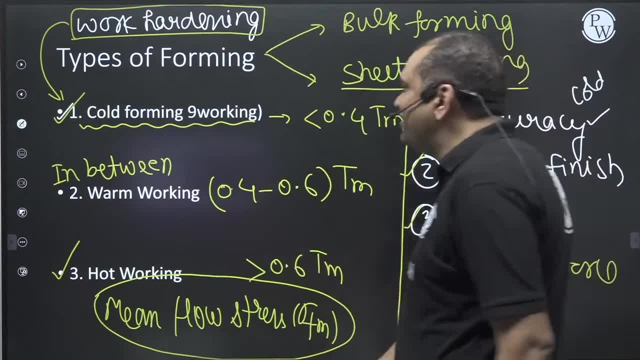 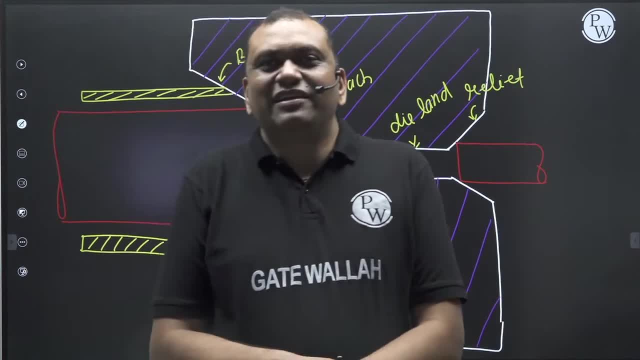 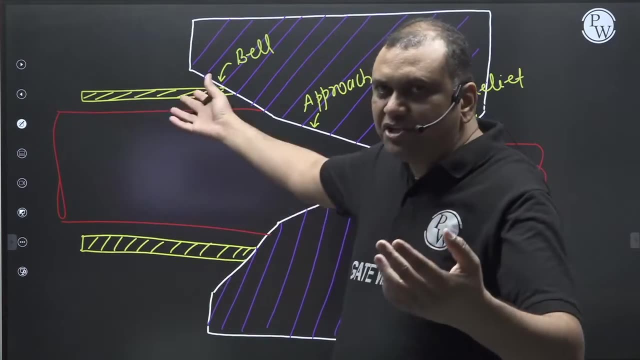 ok, anyway, I will give you all the slides later. I am uploading them on my app, so let's start. let's get into the theory. you must be sitting with a pen and paper. you can write whatever you want. this sheet is uploaded as a pdf. let's discuss the theory. 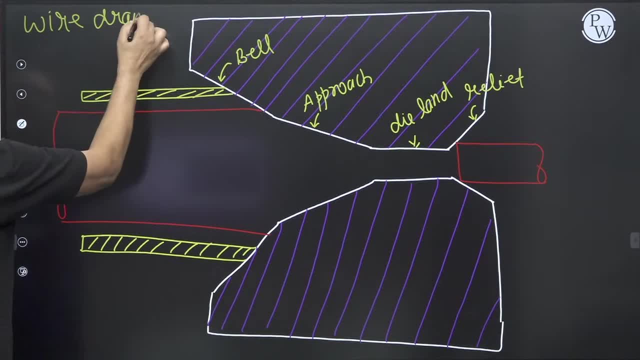 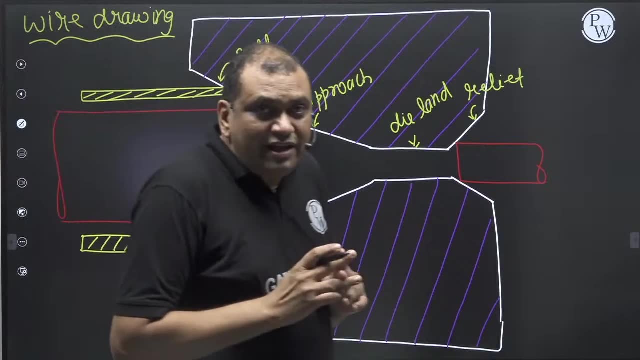 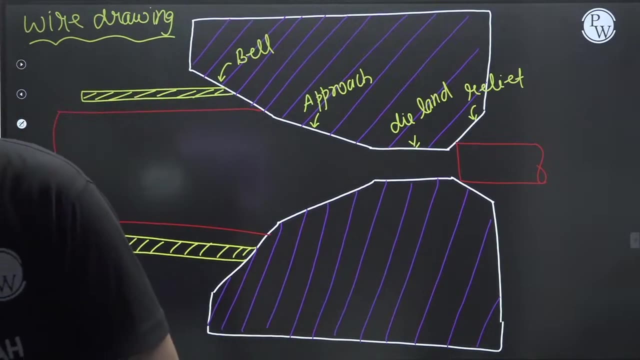 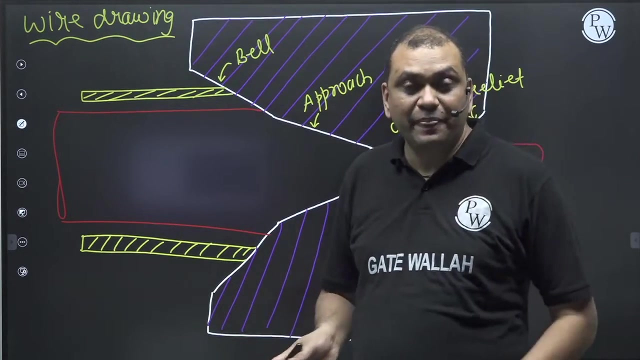 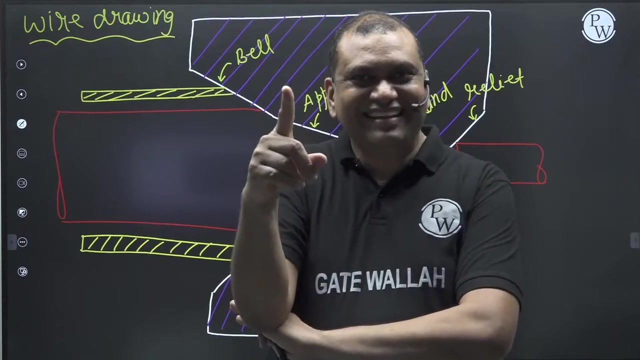 wire drawing. let's discuss the theory: wire drawing and extrusion as far as principle is concerned. as far as principle is concerned, wire drawing and extrusion are exactly same mathematical principle, the principle behind metal forming. I will talk about that. so wire drawing and extrusion are same. 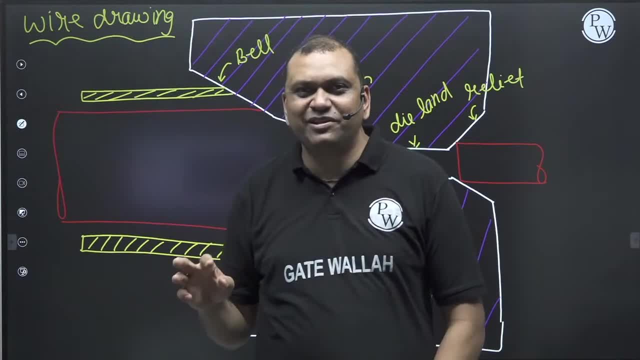 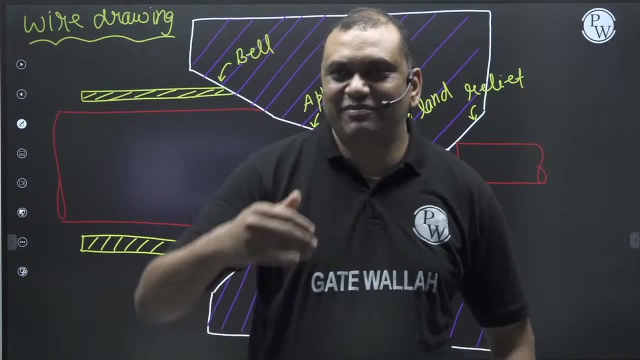 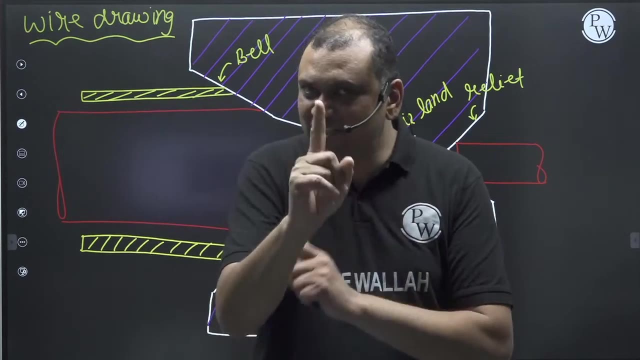 do you know one thing: close your chat box for 10 minutes. listen to me what I am saying, because actually some students are. I will tell you that you are free to write in chat box. write everything. I will answer in chat box, but for 10 minutes. 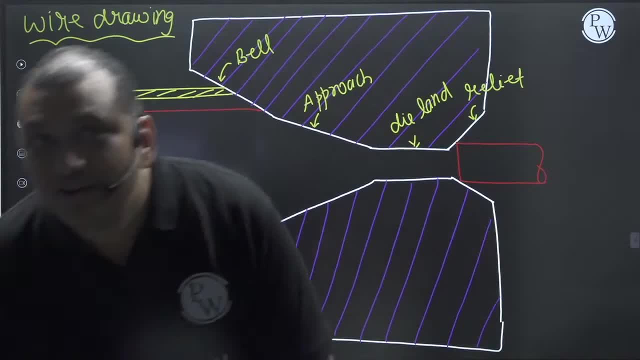 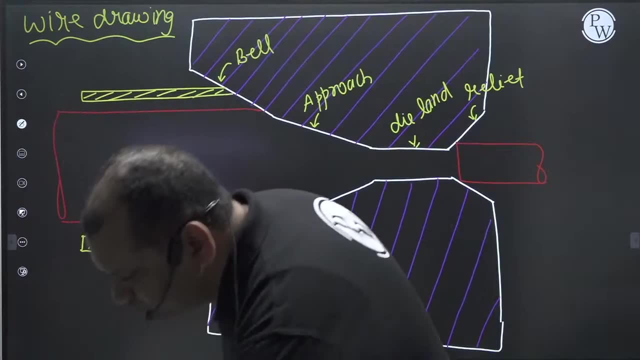 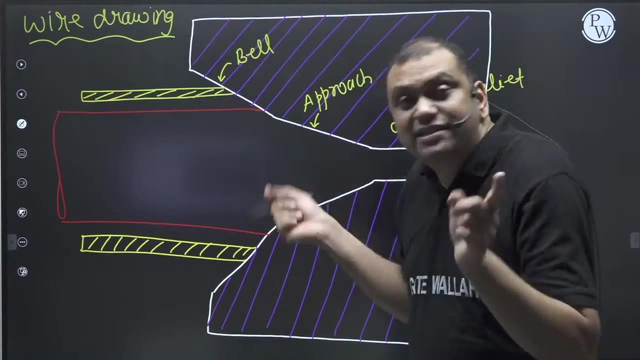 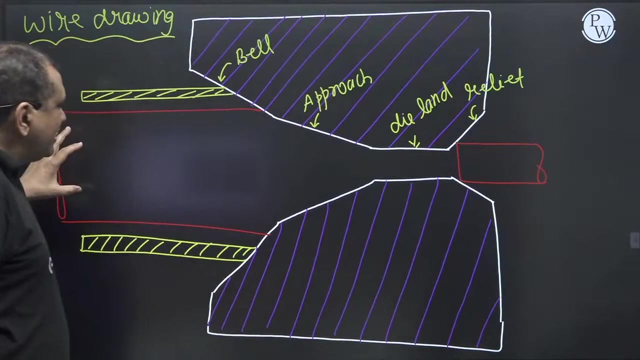 wait a little and drink some water. as far as principle is concerned, wire drawing and extrusion are exactly same. what is wire drawing? what is wire drawing? what is wire drawing? it is a process of decreasing the incoming cross section area of wire. let us say 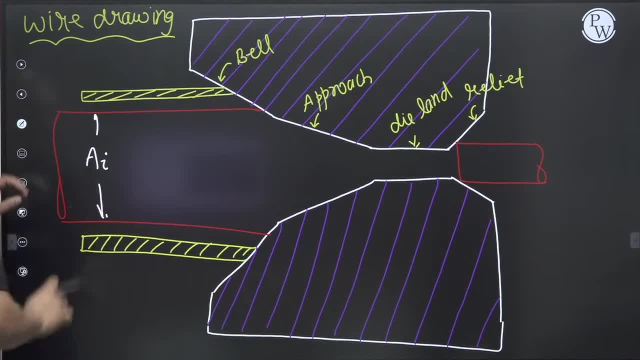 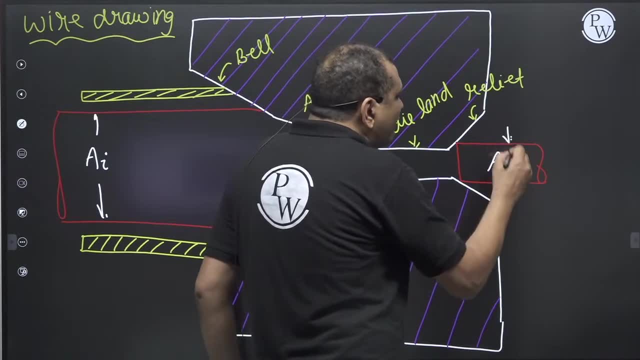 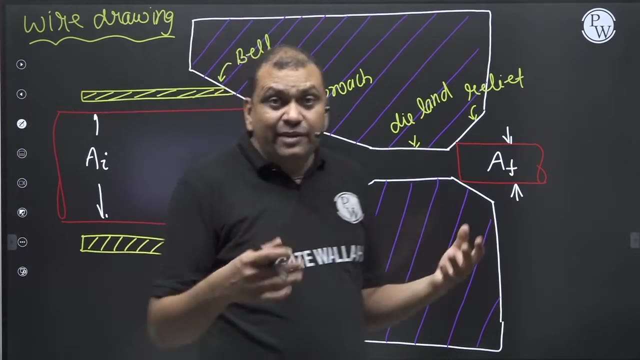 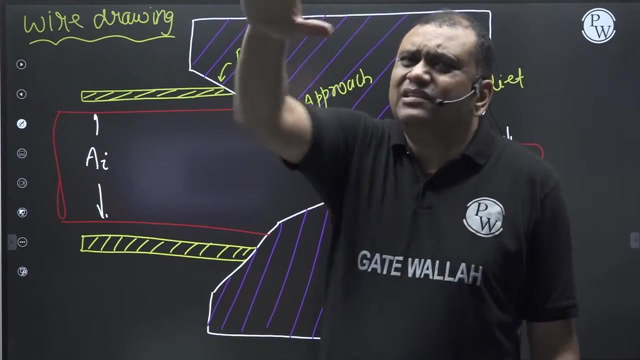 Ai is the incoming area of wire which is of red color, which is the wire which is going inside the die and Af is outgoing area of wire, outgoing area of wire. so generally, before wire drawing the raw material was sent by some other company. generally, the raw materials 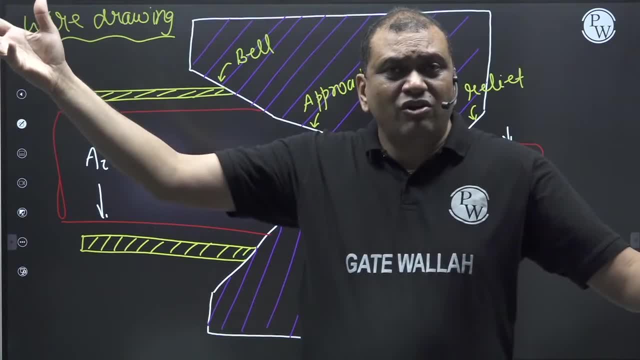 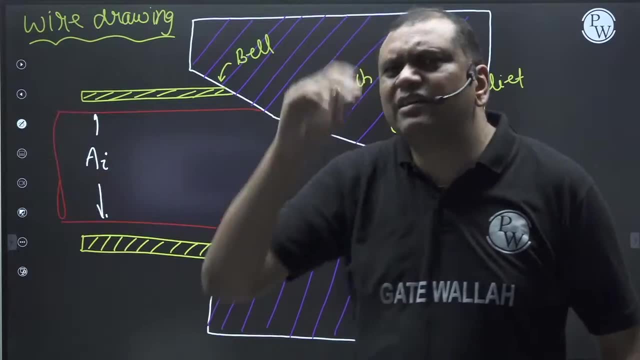 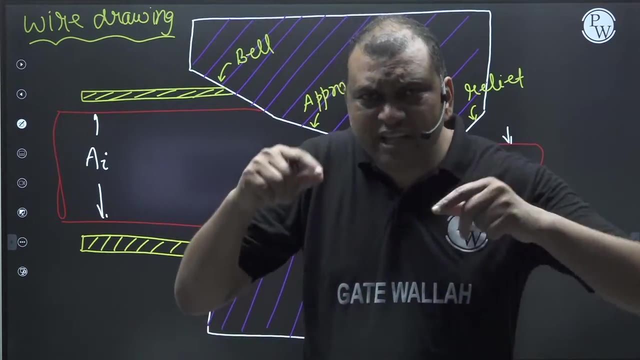 are stored in open and the material is lying like this for weeks. it comes from somewhere. when we do wire drawing, it is around after one month. everything is lying like this, generally in open, so naturally there will be oxide layer formation on it. now see, please, for half an hour. 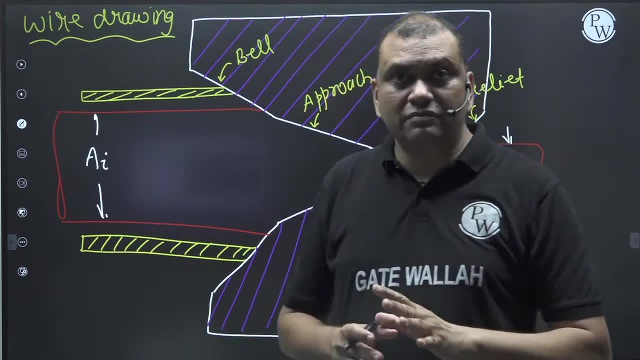 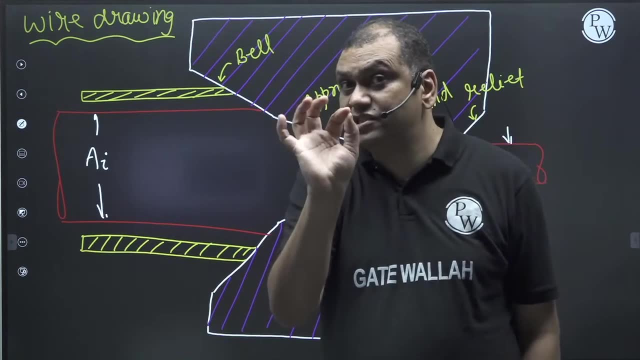 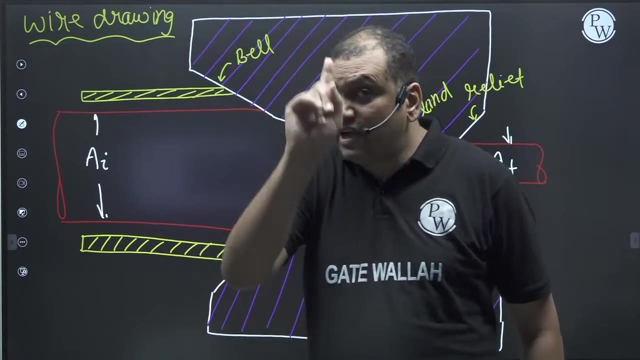 I want your absolute attention. if you understand, then you will find the forming very easy. these are four lectures of forming. take it very seriously. ok, this is crash course. I understand that gate is important for 2023. now for half an hour, look very closely so the material which is stored. 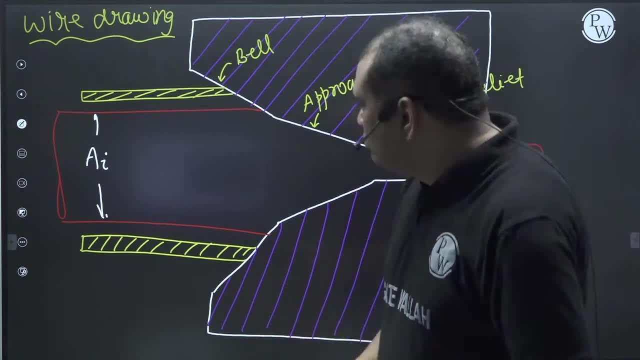 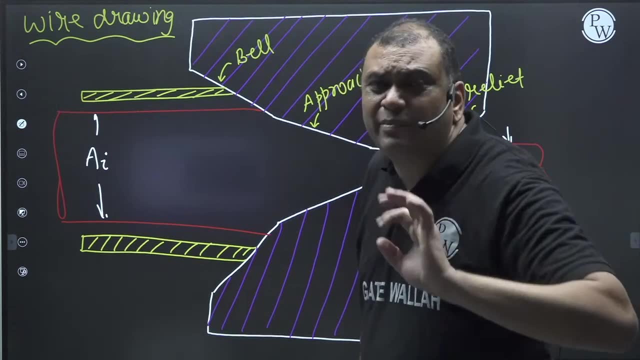 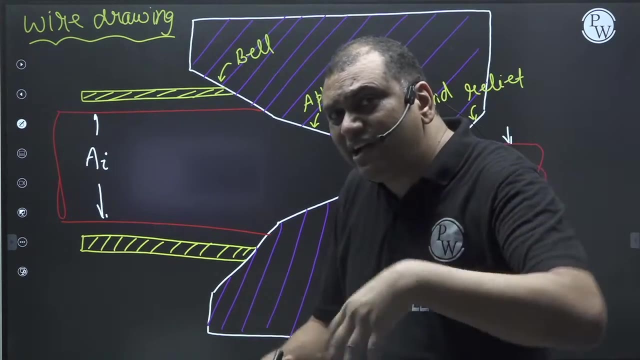 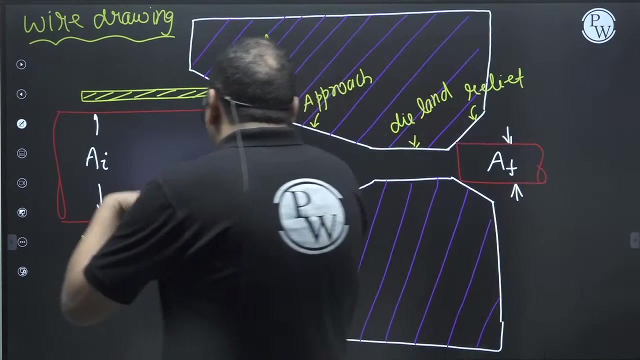 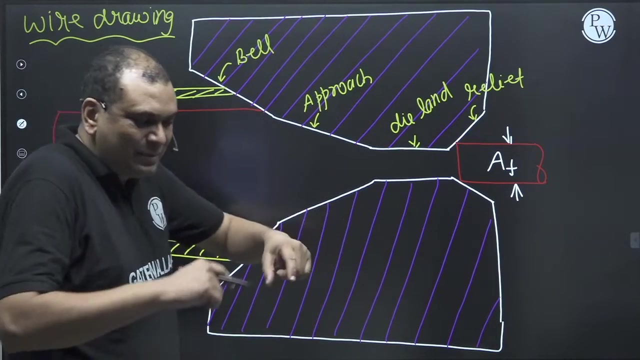 will have oxide on it. so before drawing, we have to remove the oxide from its surface. if you without removing the oxide, if you start drawing it, you, if you start drawing it without removing the oxide, then do you know what will happen during deformation? the wire which is there. 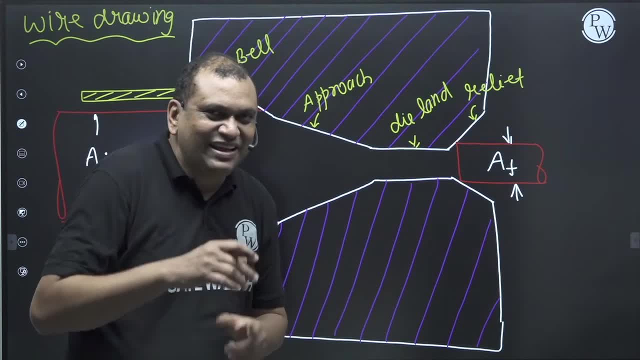 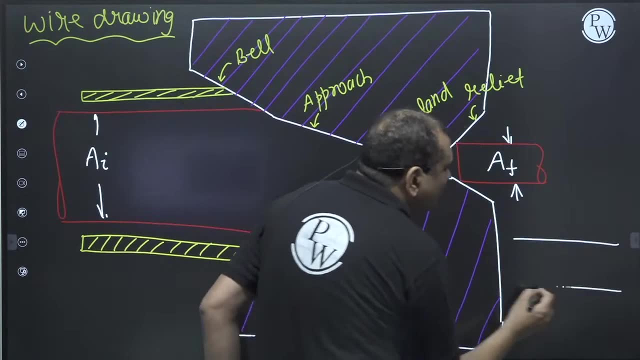 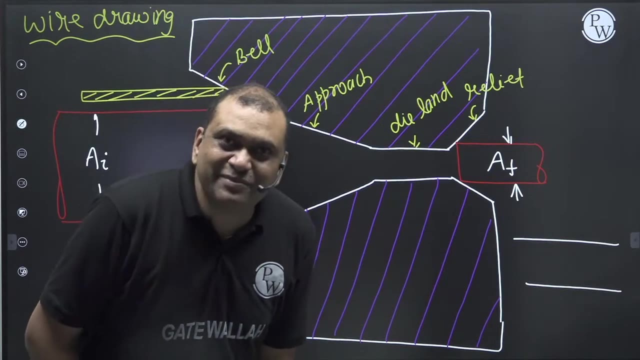 if there was oxide on its surface, it will percolate down and accumulate at the centre. means deformation: the outgoing. this is outgoing wire. so when deformation will happen in die, so oxide is a different material. so it will go towards the centre of the wire because deformation is dying on the wire. 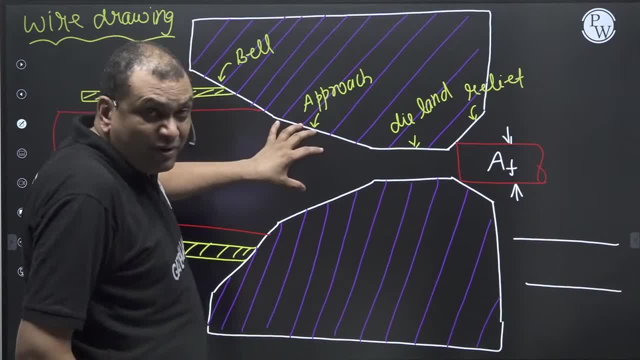 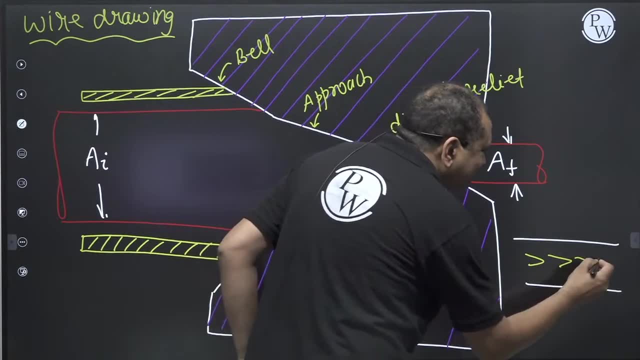 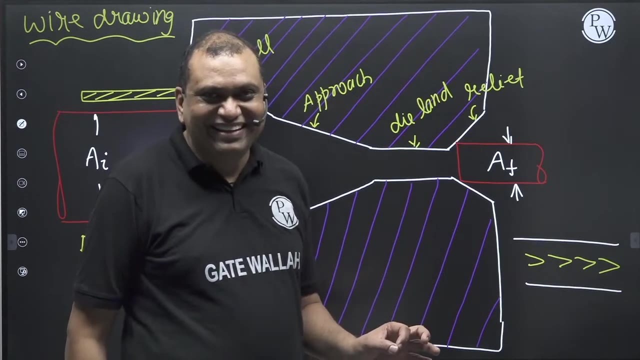 but oxide is not metal, so it is impurity. so it will converge and go towards the centre of the wire. so it will converge and go towards the centre of the wire and it comes in this form, like this: there are some cracks on the centre line. there are some cracks on the centre line. 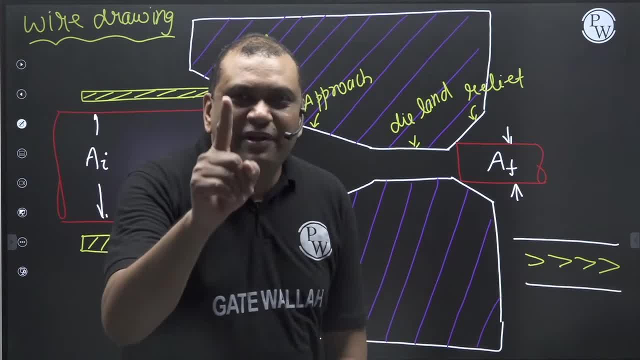 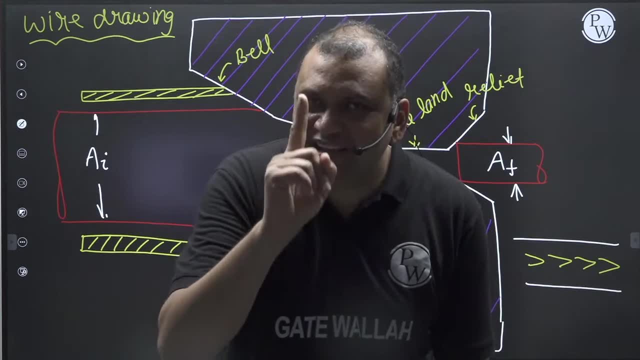 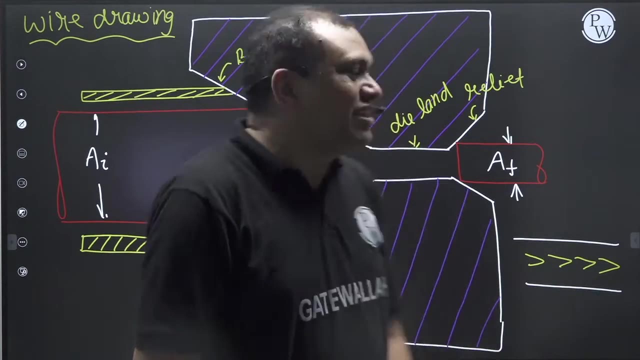 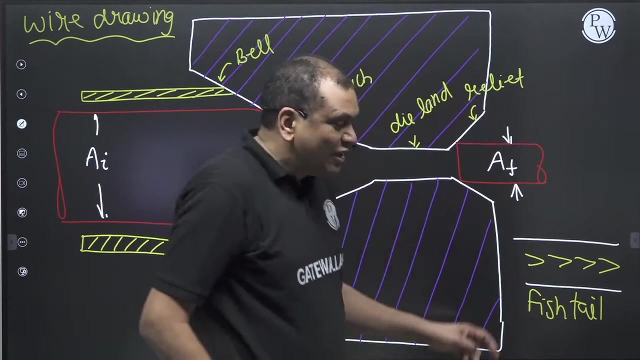 why there are cracks on the centre line? because before drawing and extrusion you, you, before drawing and extrusion, you didn't remove the oxide and this defect is called fish tail. some people eat fish. I don't eat fish, so it looks like a fish tail, so fish tailing. 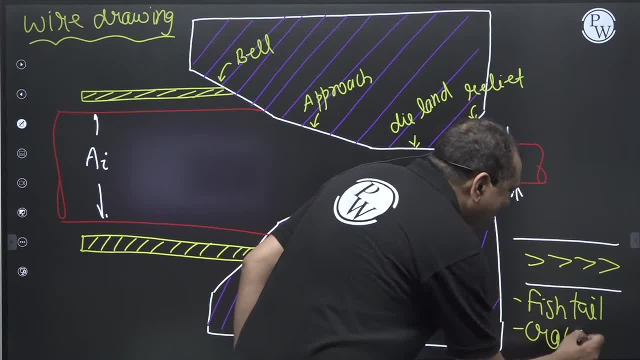 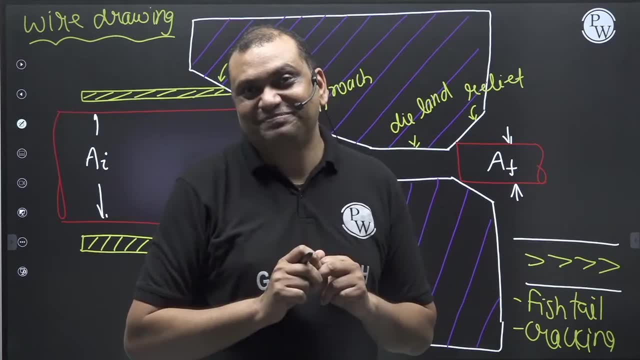 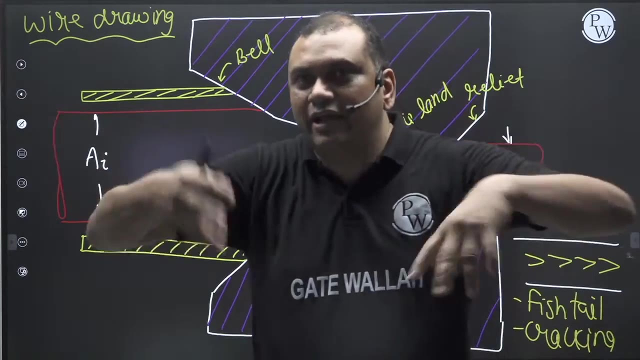 centre line cracking, centre line cracking etc. so it is very important to remove the oxide. so how do I remove the oxide? wire drawing so we do same in extrusion. if great dilute in extrusion then I날anger it. if small wire, how do I remove the oxide? 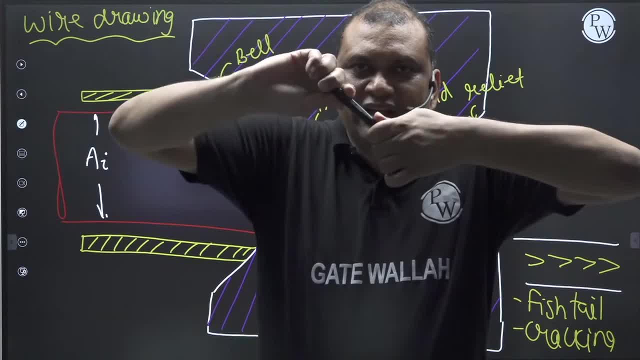 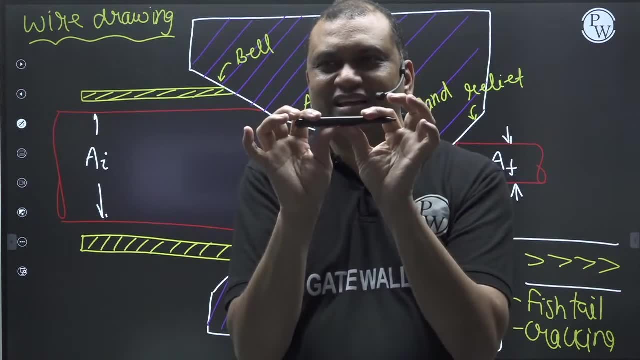 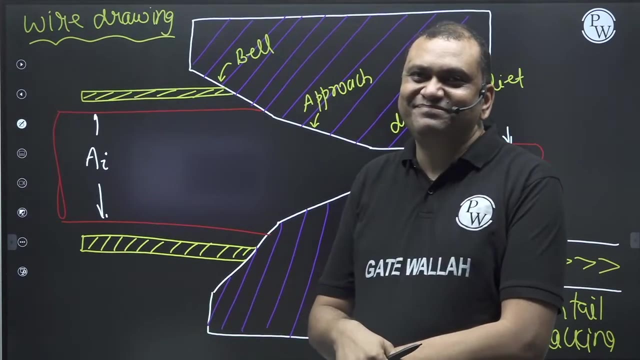 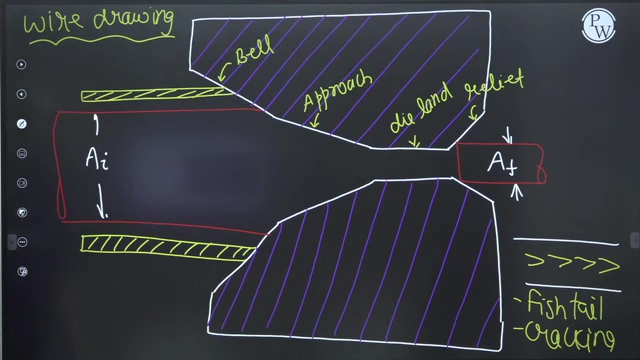 I will twist the wire. either twist or bend, or twist or bend. so what happen? it will remove the oxide on the wire. its will be removed alright, and this is known as pickling process. and after that, the incoming wire: I will dip it in a lubricant. 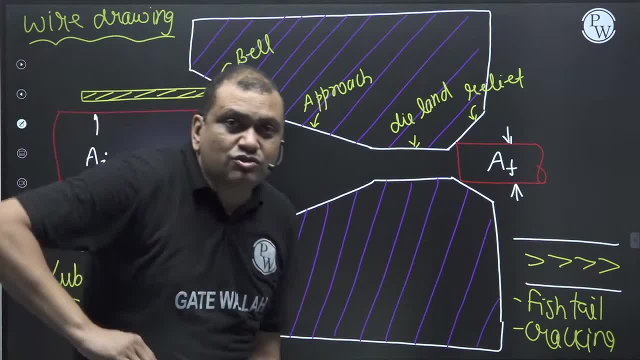 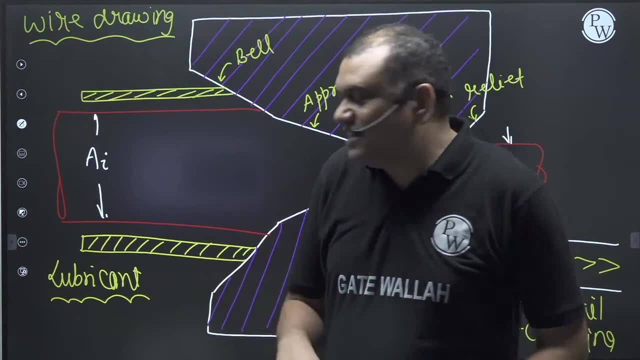 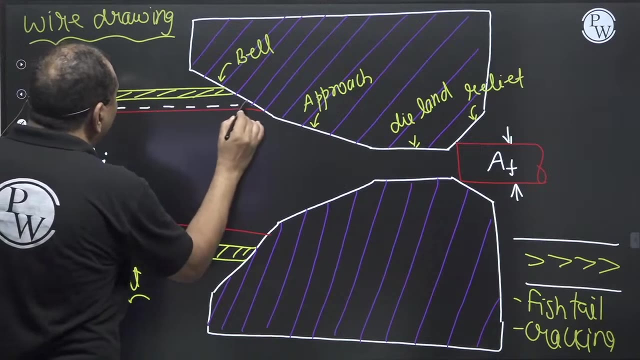 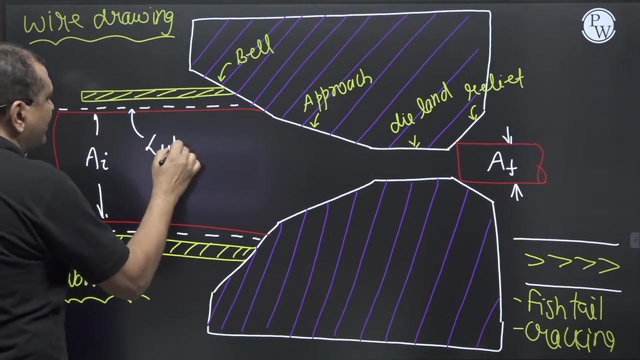 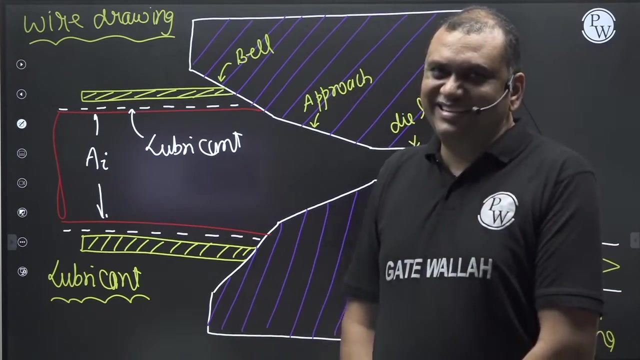 the incoming wire, I will dip it in a lubricant. so what is the purpose of dipping the lubricant that our incoming wire? there will be a thin layer of lubricant over the incoming wire. there will be a thin layer of lubricant over the incoming wire. 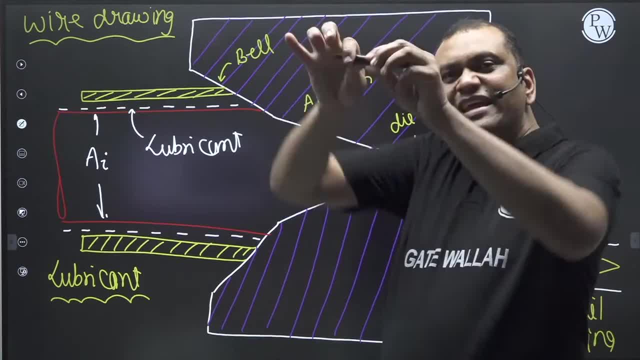 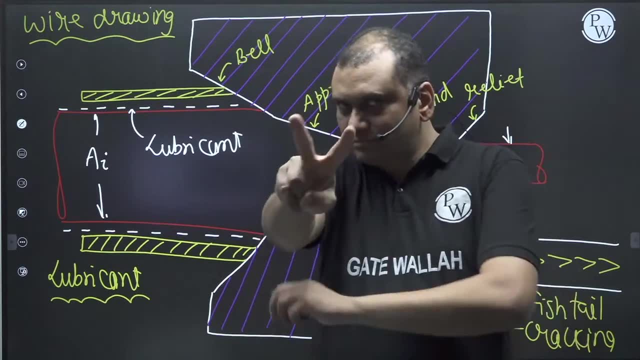 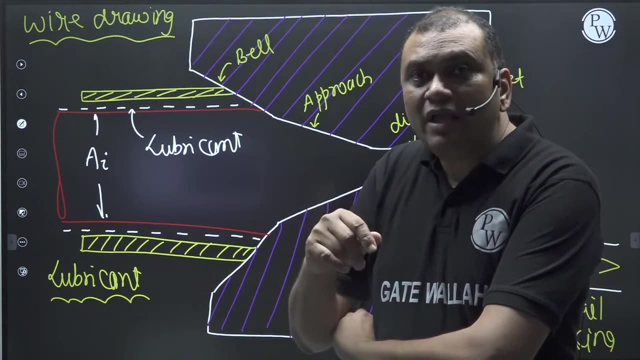 pickling means you have twisted or bent it so that the oxide comes out. after that you have dipped it in a lubricant. there are two types of lubricant. one is liquid lubricant, like there are many oils- vegetable oils, mineral oils- there are many solid lubricant. 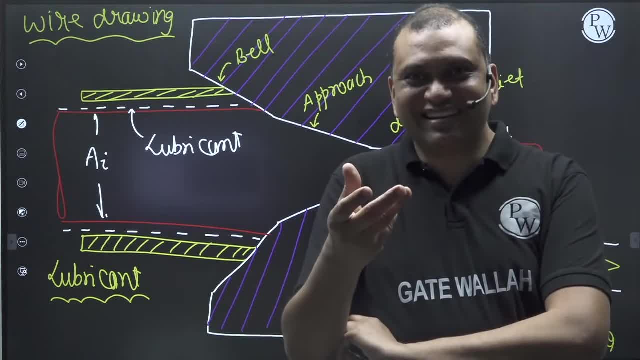 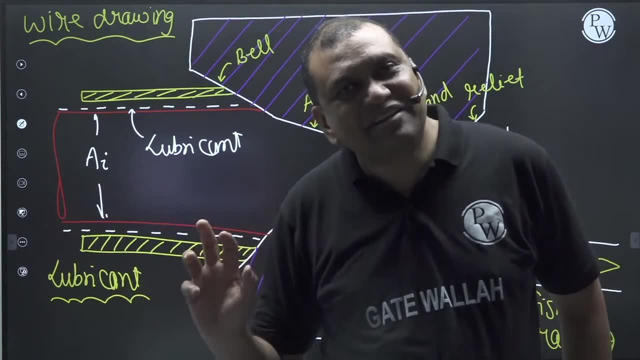 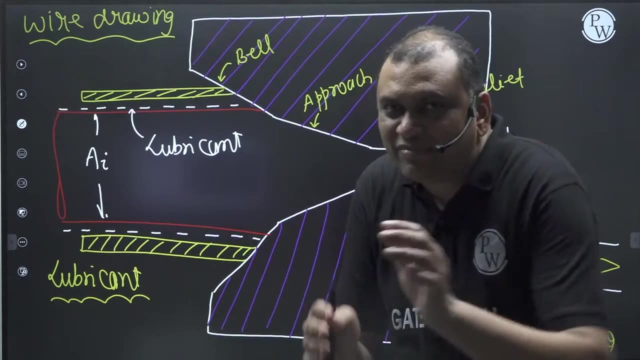 aluminium powder, graphite powder, soap powder. so when we have to give a large reduction, we use solid lubricant. when we have to give a large reduction, we use solid lubricant. if we have to give a small reduction, then I will use liquid lubricant, then I will use liquid lubricant. 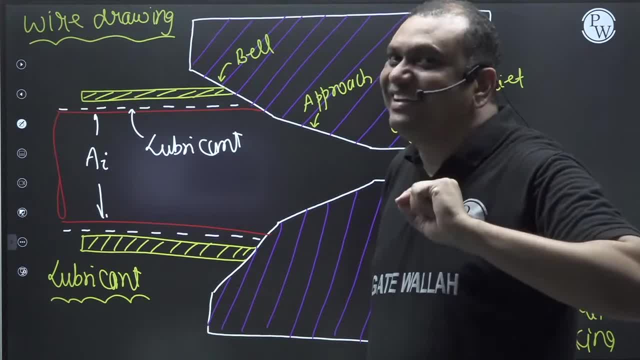 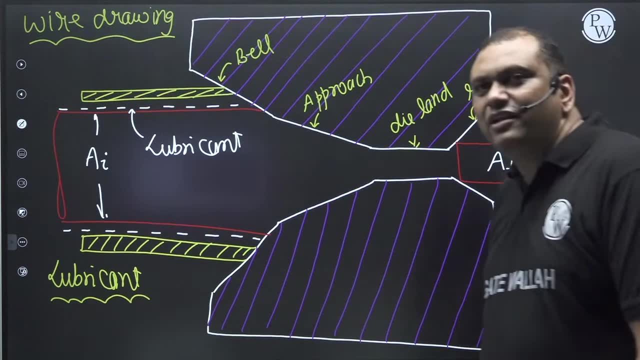 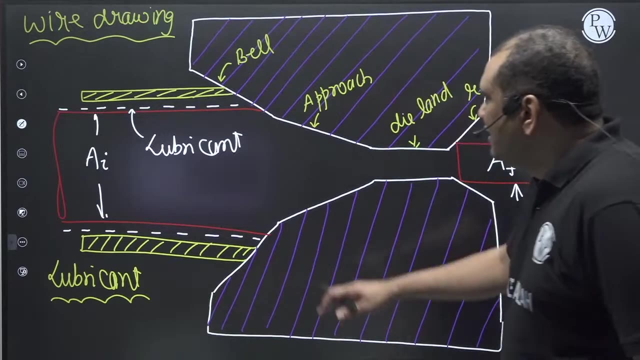 why did we use lubricant? see the internal cracking like fish tailing or internal cracking, tail pipe or tail pipe- all are the same thing. because we are not able to remove oxide and that percolates down and accumulates at the center. and that percolates down and accumulates at the center. 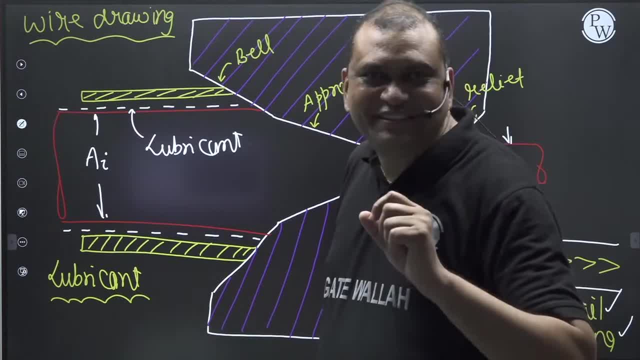 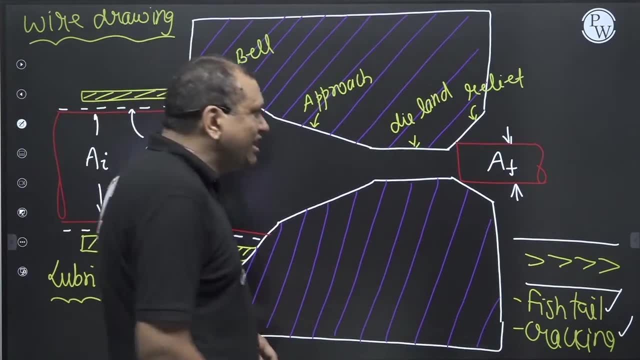 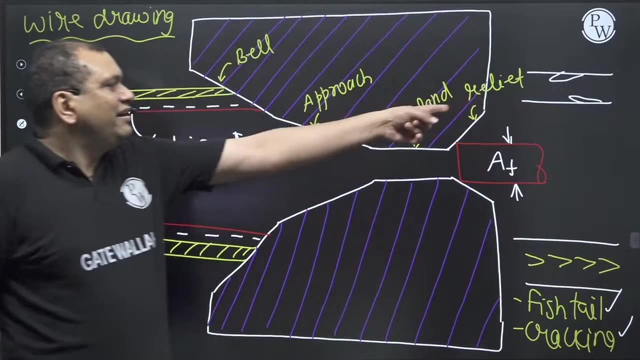 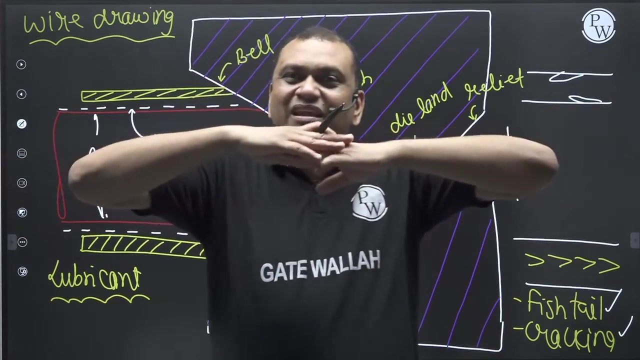 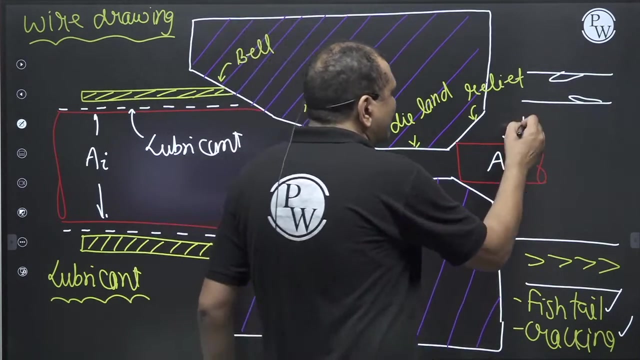 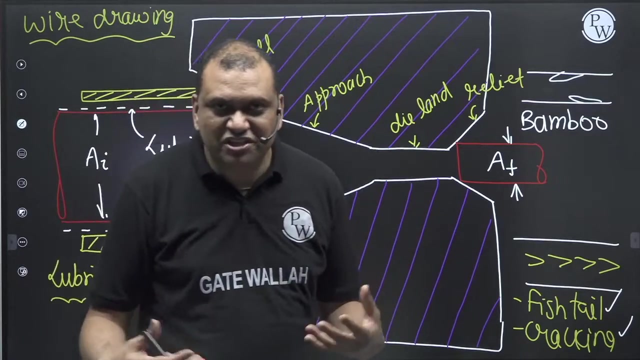 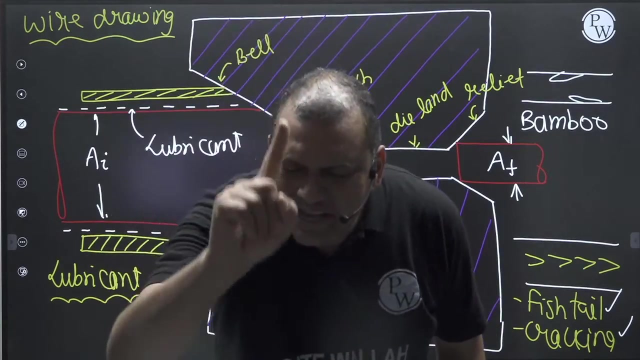 internal crack but suppose lubricant is not proper during the deformation? surface crack. this defect is called bamboo defect. this defect is called bamboo defect. surface crack, surface crack, improper lubrication, central and crack because of improper cleaning of the incoming material. improper cleaning of oxide leads to central and crack improper. 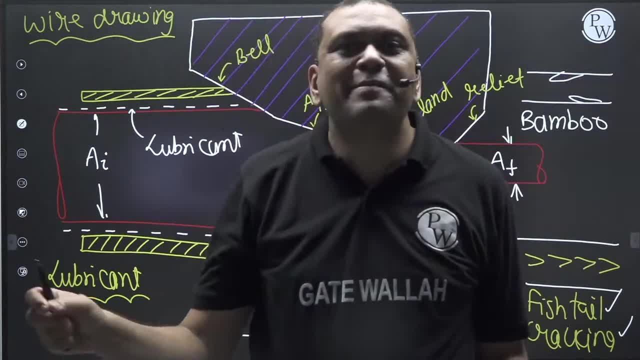 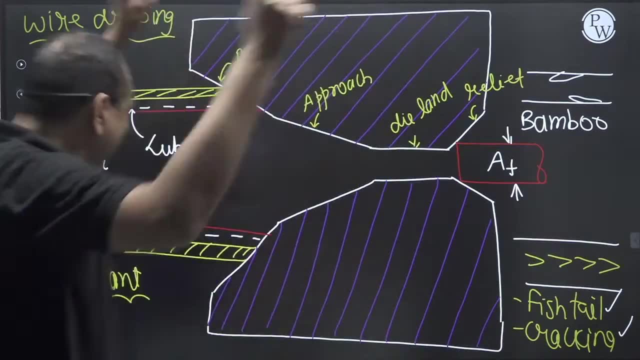 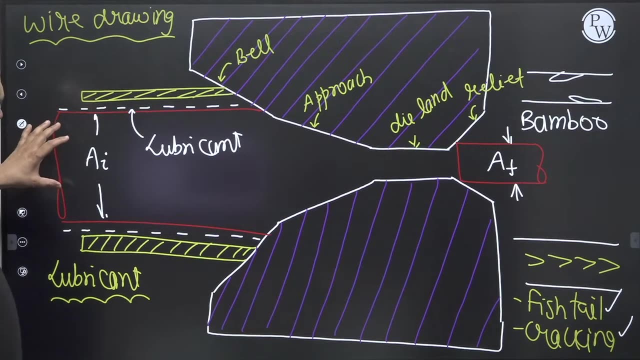 lubrication leads to surface crack that is called bamboo thumb boom, a bamboo bambu bambu. so what they are going to take away? so I've made lubricant. what would be a Tiga was capable of. incoming material will have a thin layer of lubricant over it. okay now, Joe. 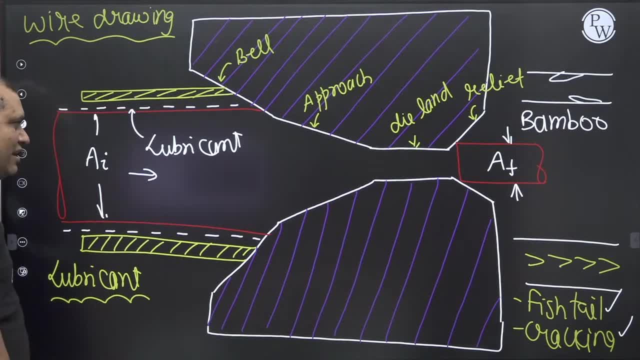 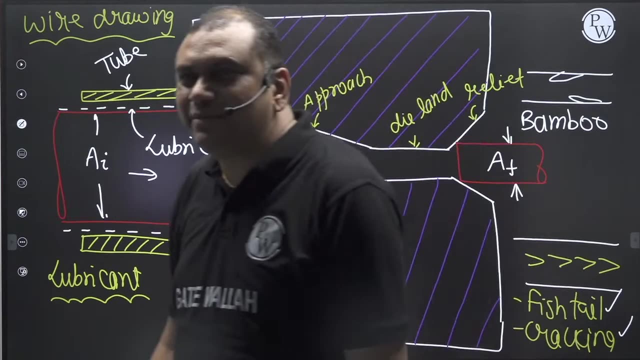 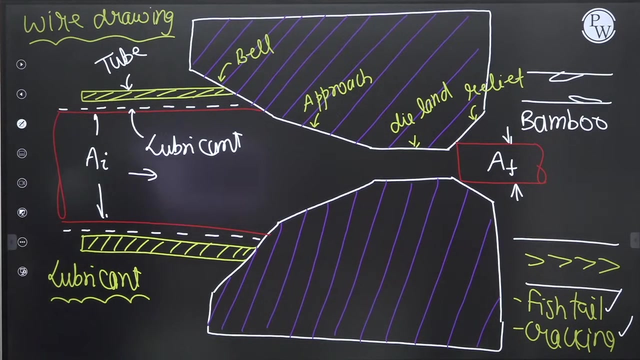 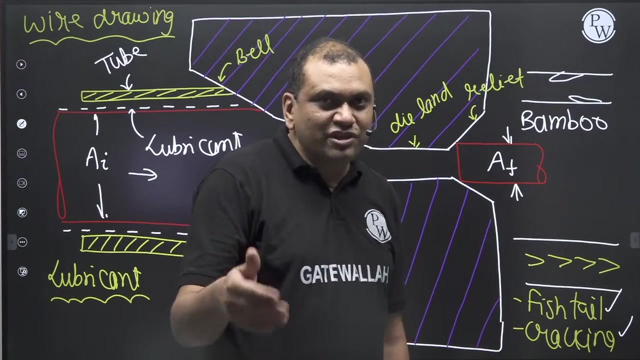 hamara do incoming material here. voila, it is approaching the die with the help of a teal. it is approaching with the help of a teal, amira. now chat box can be active. chat box can be active. no, God of Marana, you are wrong. that's not the way why drawing also can be hot. working X to some can also be. 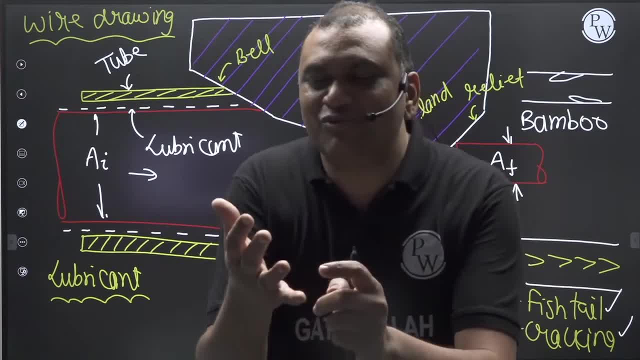 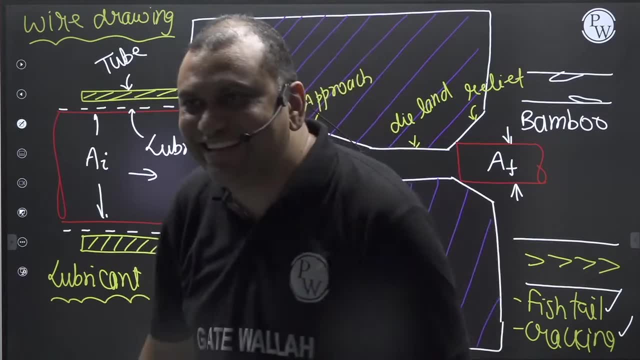 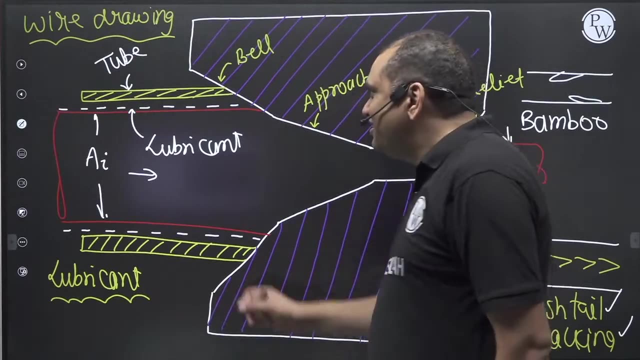 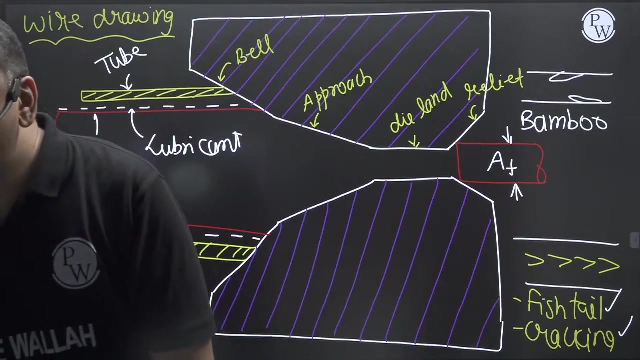 cold, working, X to some can be cold, X to some, warm, X to some, hot, extrusion wire drawing can be cold, cold by drawing, bomb by drawing. and anybody, any champion in the group, any champion in the group, support muhammad. i think you are from kashmir, if i, if i'm not wrong. 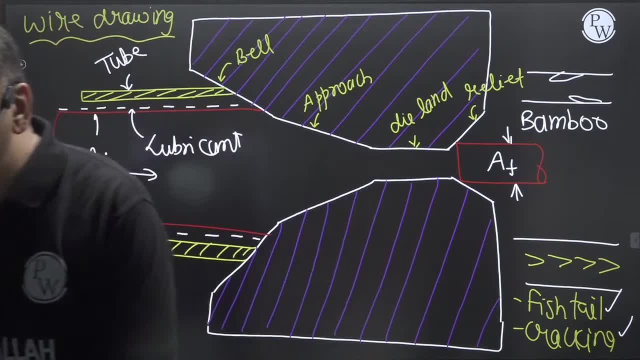 there are five kashmir students, kashmir children from here. guide the material in the bed. also, support two feet properly guiding the wire. support ravi abhishek, ankit pavan. everybody is getting the same answer, but i will tell you your answers are wrong. 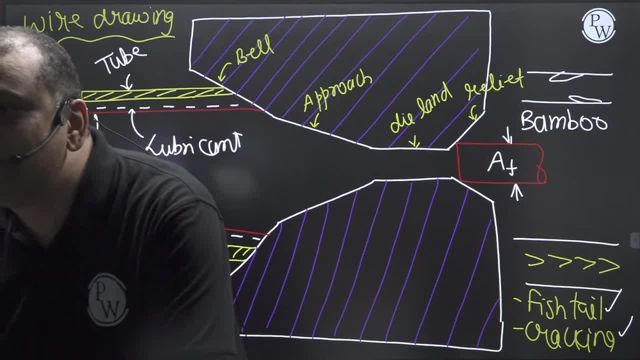 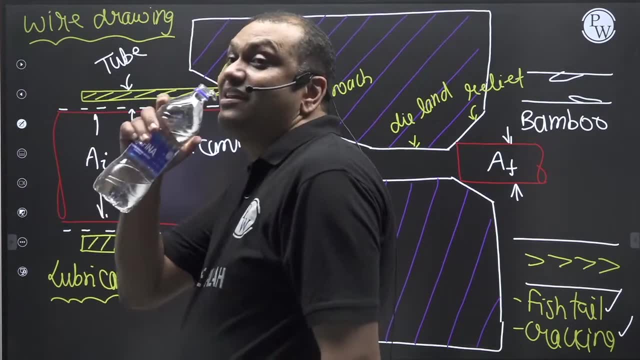 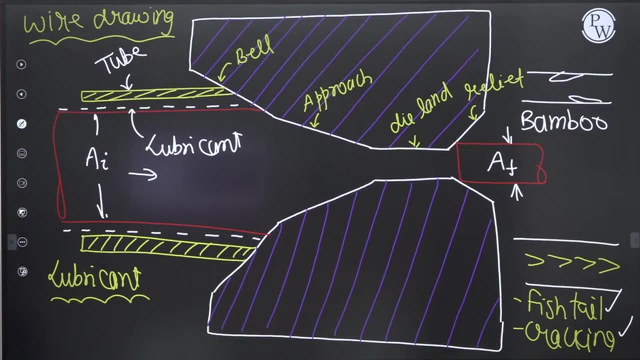 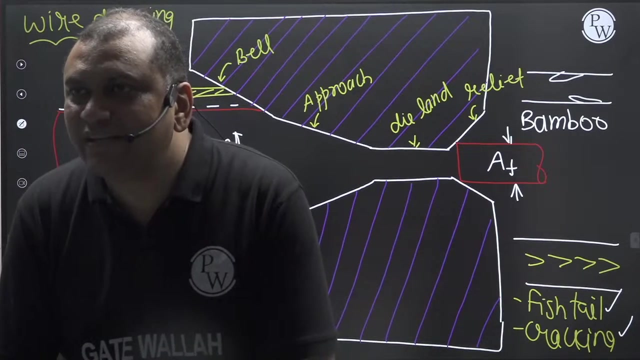 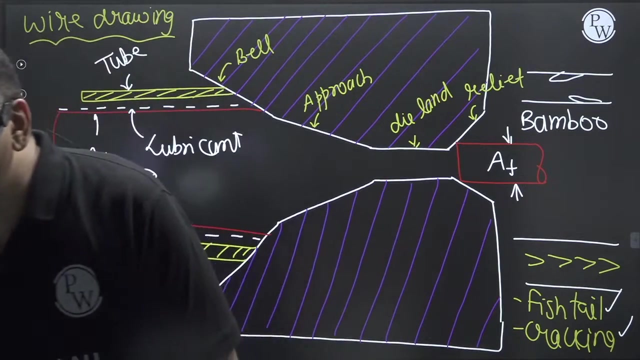 none of the answer is correct. all the answers are wrong, all the, even the fahad harsh. everybody is wrong here. huh, everybody is wrong. no, nira singh, that is also wrong answer, animation wrong. i think nobody will be able to get it. yeah, kashmir. i remember navid from kashmir because you have written to me also. 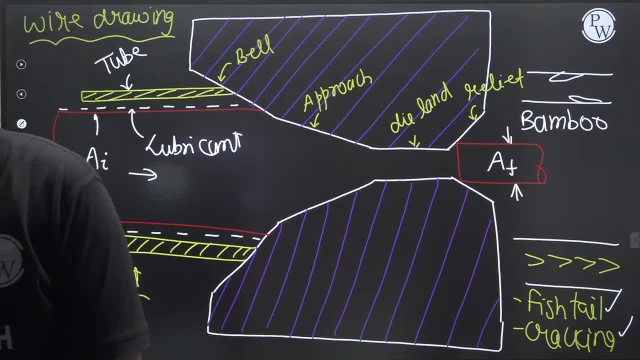 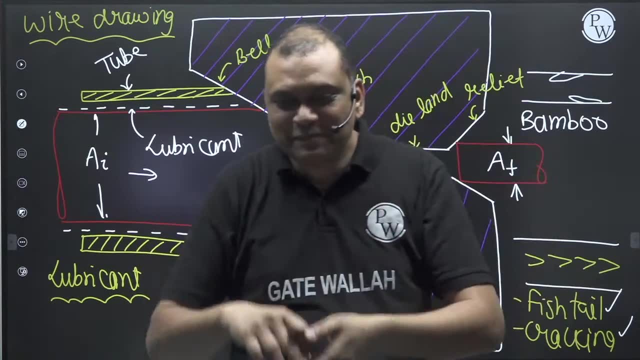 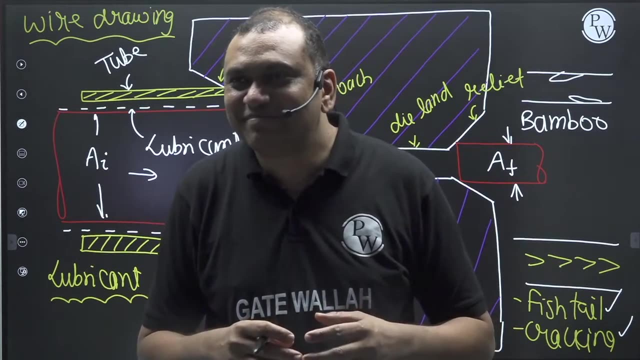 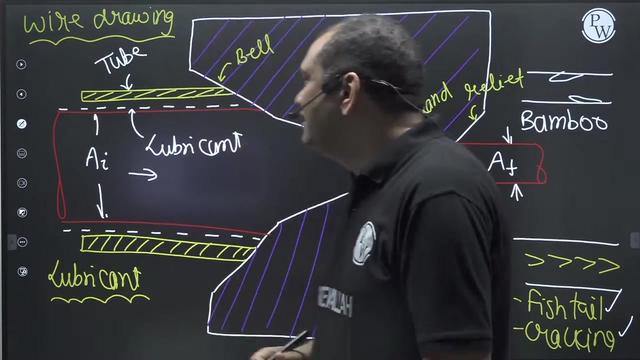 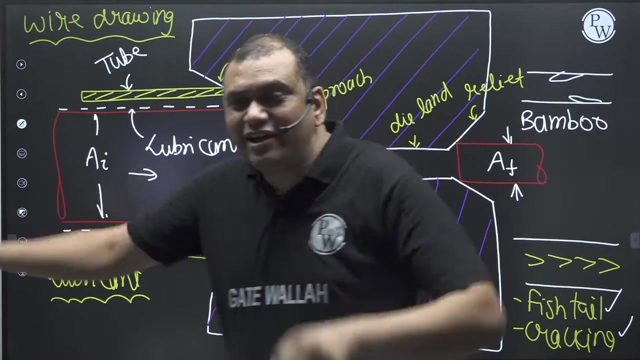 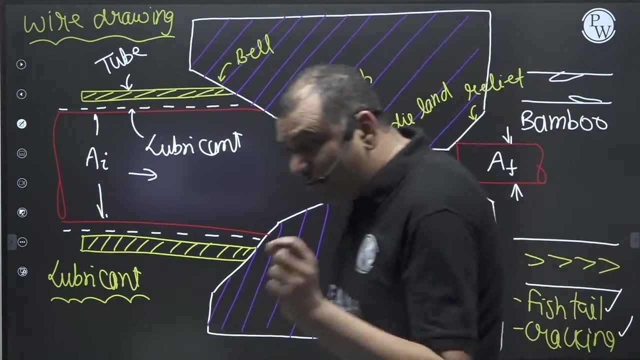 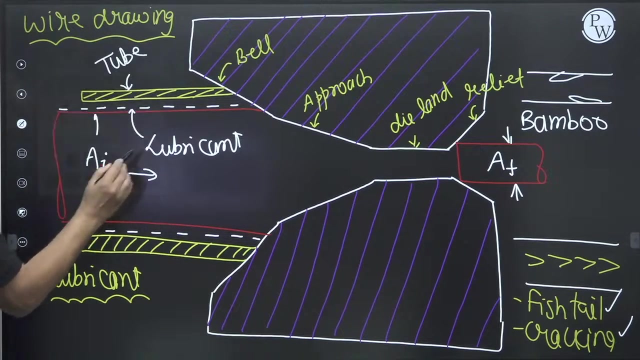 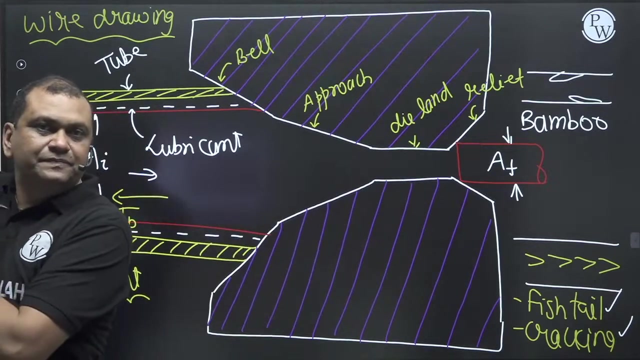 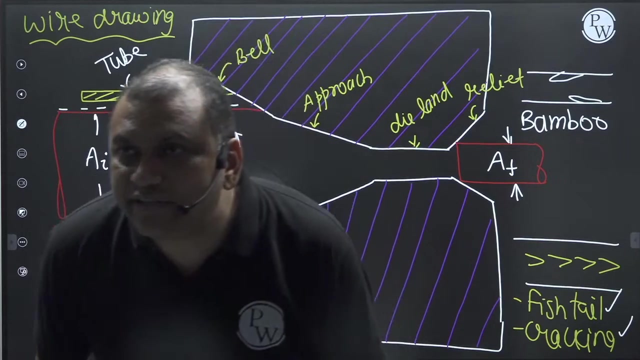 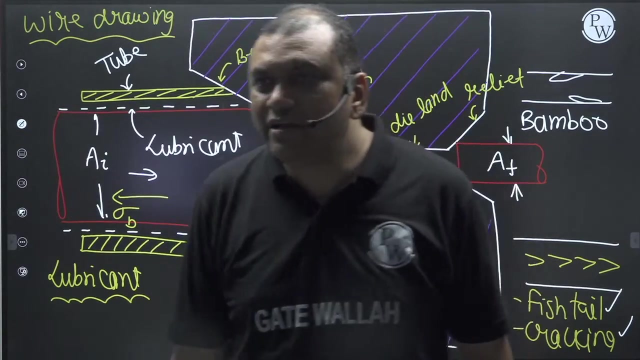 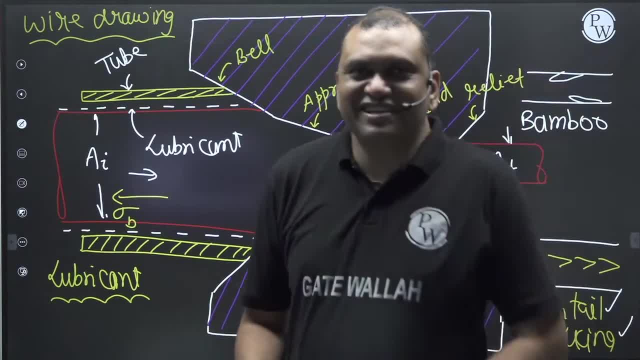 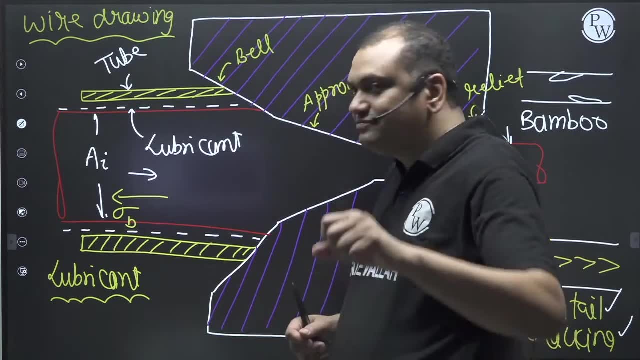 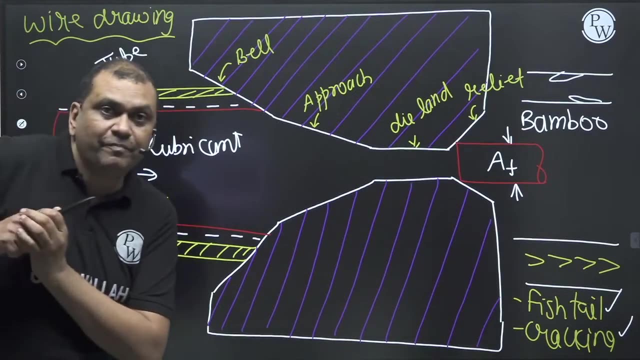 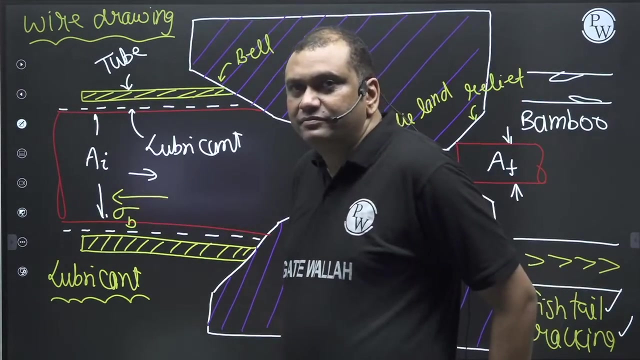 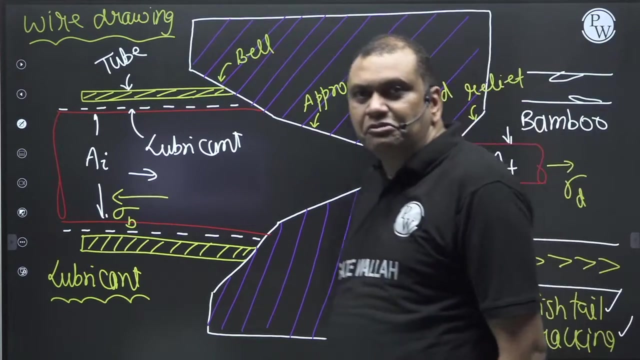 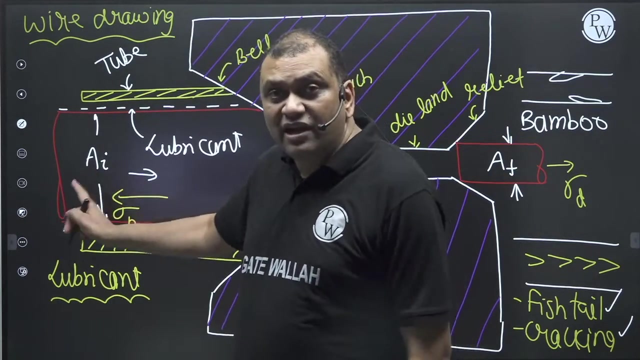 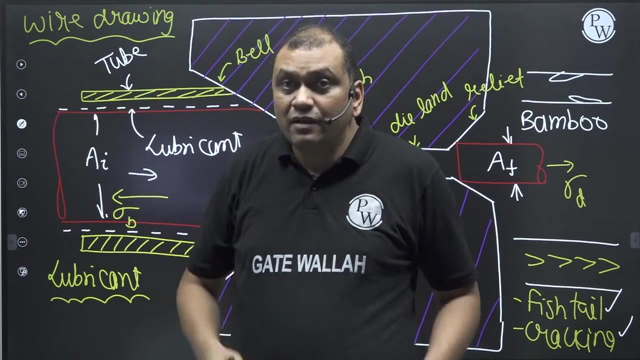 I think you are teachers. to keep the wire straight, we apply the back pull. now what is the purpose of this tube? of course, by providing the back pull, the drawing stresses will increase, means we need more energy to draw. but still, we will apply the back pull so that our incoming material remains straight. 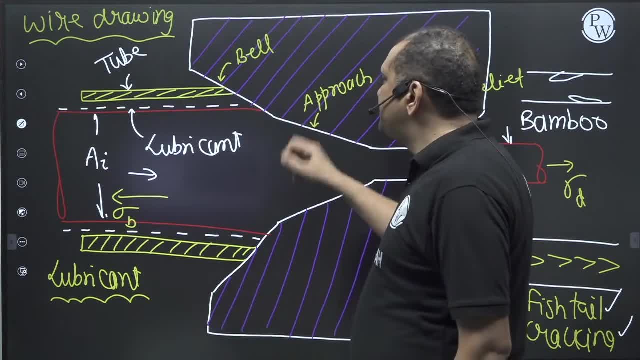 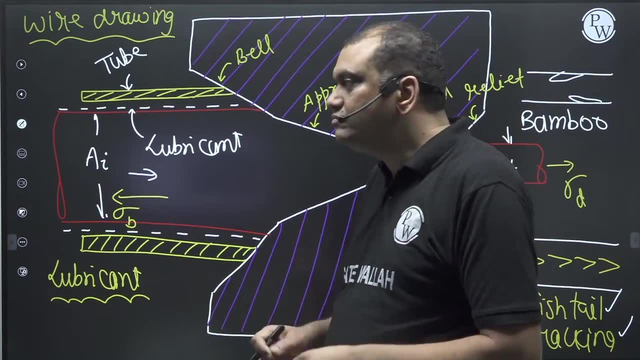 otherwise, you know what will happen: it will damage the belt section of the die. the initial portion of the die will be damaged. the belt section of the die. the initial portion of the die will be damaged. the belt section of the die will be damaged. the belt section of the die. 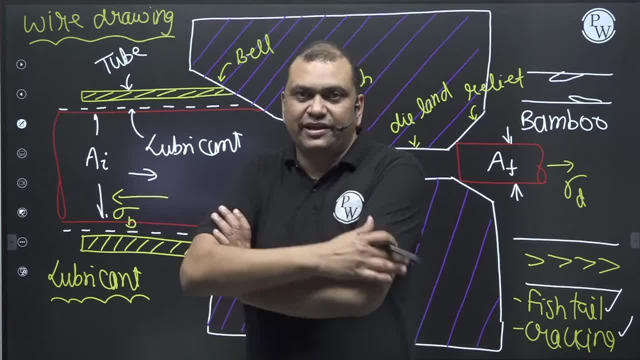 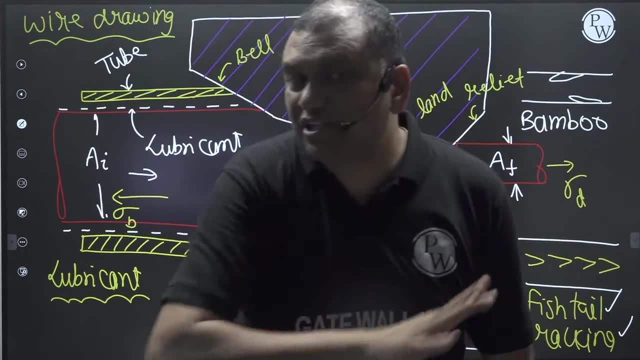 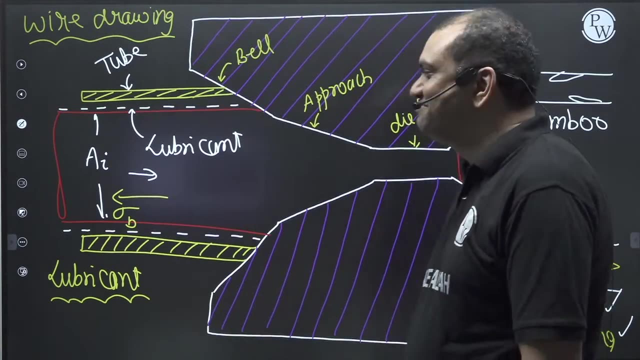 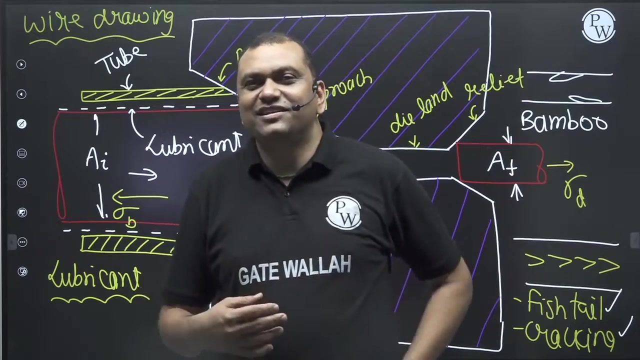 now the question arises: what is the purpose of this tube? the purpose of the tube is pressurized lubrication. the purpose of the tube is pressurized lubrication. how see, many of you are from the village. why? because of the greenery. this is the only thing. 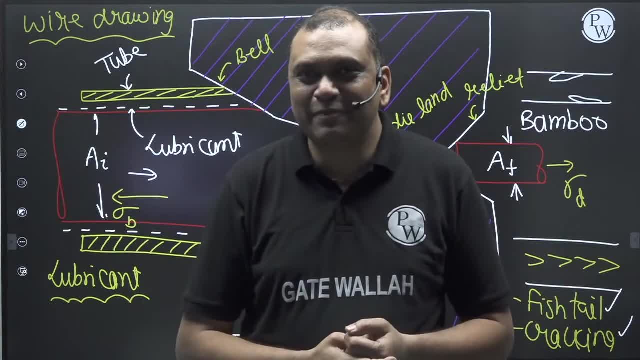 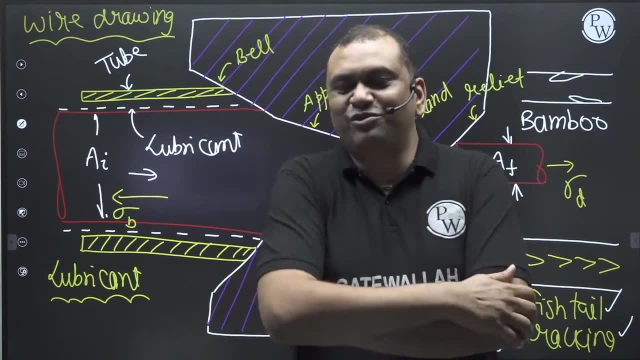 people have all the greenery. this is the only thing. you all are the poor people. you are the poor people who can not afford greenery. please, you are from the village? ok, you must have seen something in the village. we tie the animals. we tie the animals. 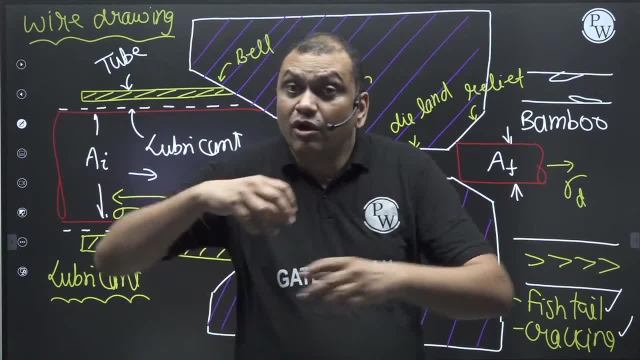 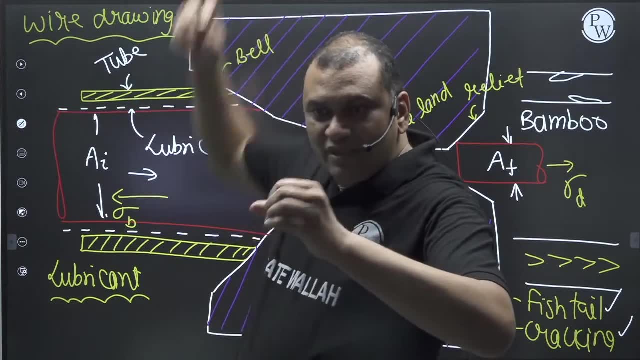 it is a rope of sacred thread. it is a rope of sacred thread and gets wet in the rain. then see the rope. you have to hold it like this and pull it like this, so from here water will come out. You must have seen this phenomenon. the people who are from villages. 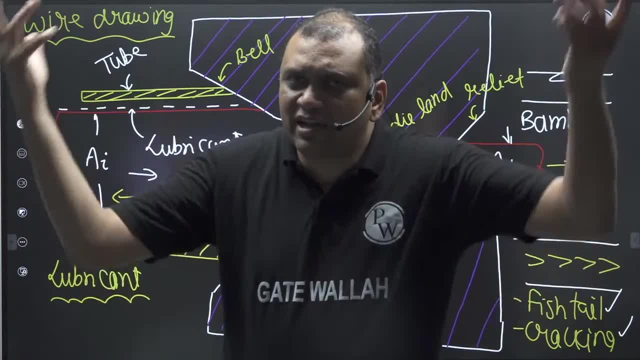 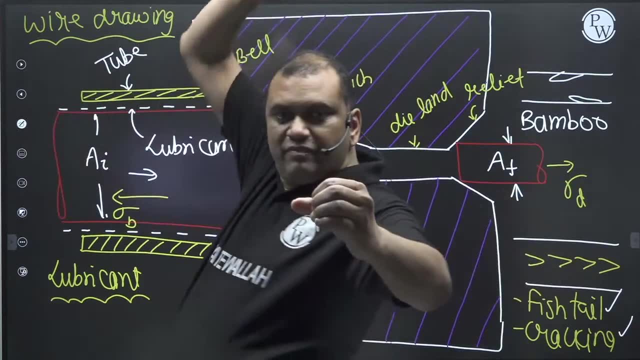 Nowadays it is raining a lot in UP. Floods have come everywhere in Aligarh, Like many people are doing it in Nava, So you must have seen this phenomenon. There is a lot of The same thing will happen here. 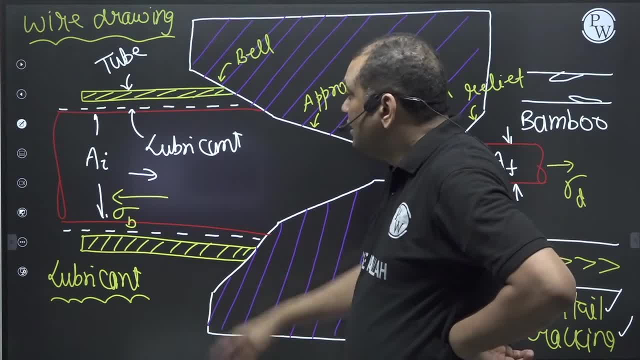 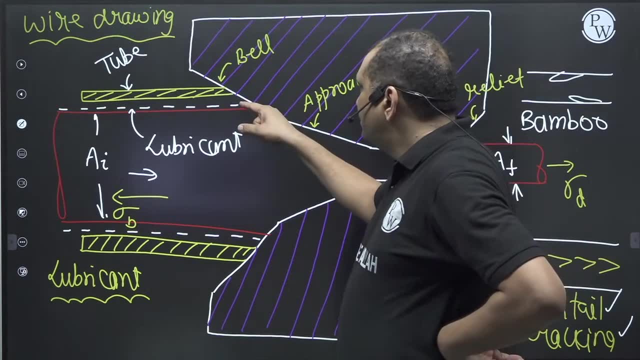 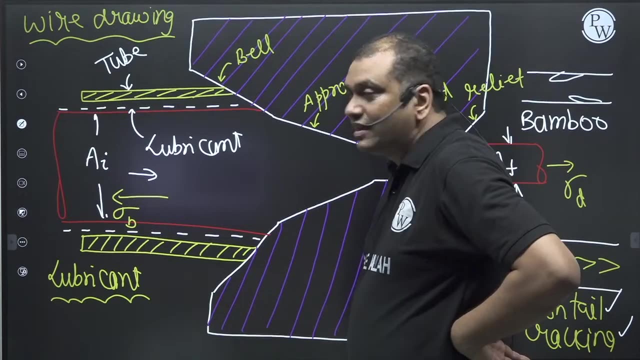 If this is not a tube, Everyone look carefully. If this is not a tube, then when we are pulling the wire forward, So The lubricant will splash. If you provide a tube. If you provide a tube, then see what will happen. 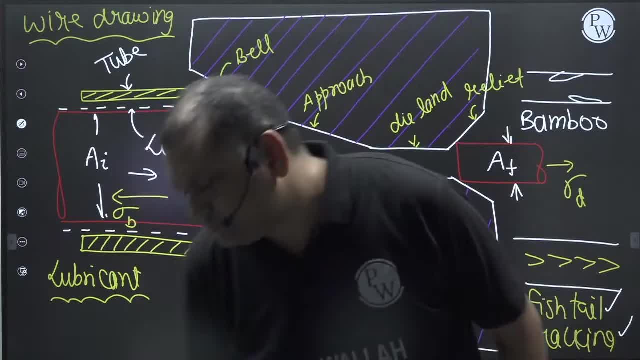 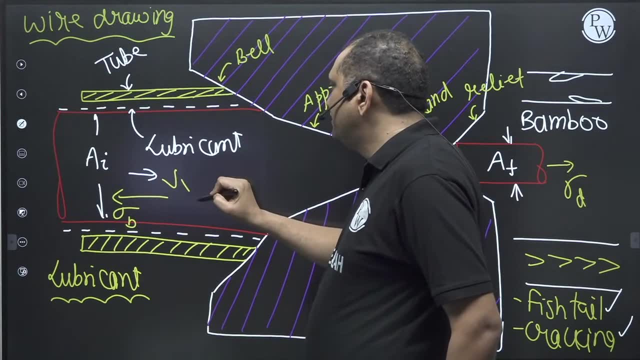 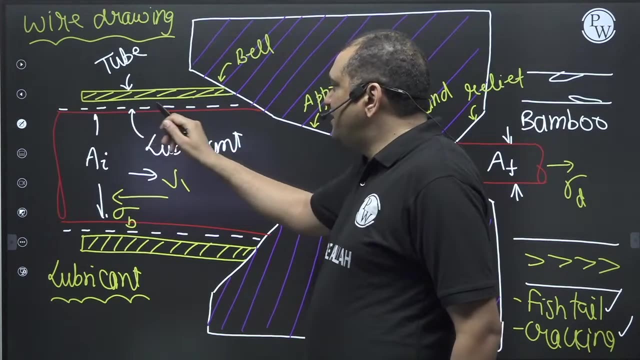 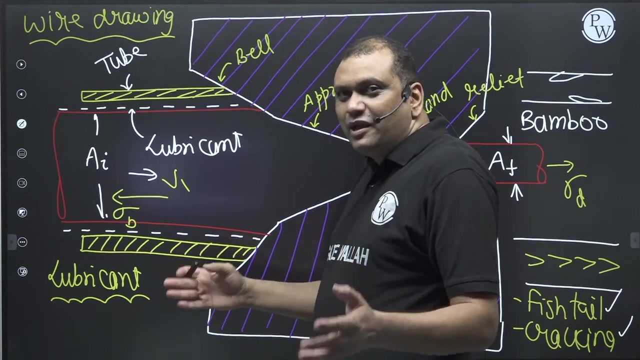 Then see what will happen. This wire is moving, Let us say, velocity V1.. Why Incoming material is moving with velocity V1. So our lubricant that also moves with velocity V1. So our lubricant is also moving with the same velocity. 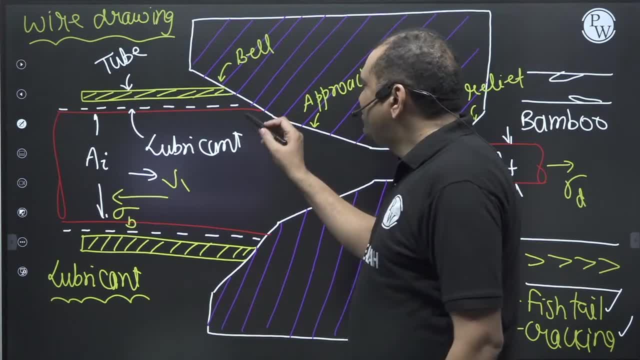 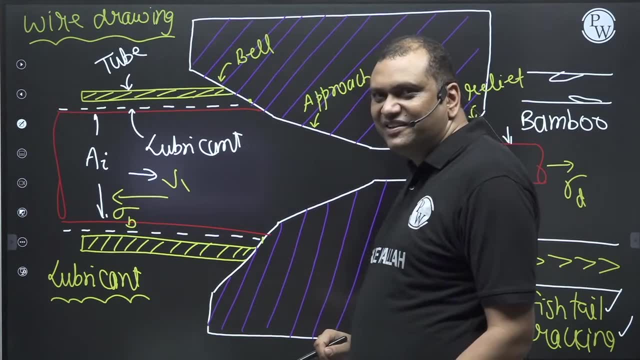 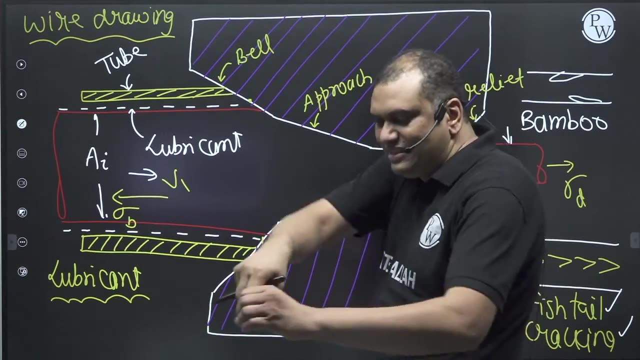 as that of wire. So the lubricant which will hit the belt section. When the lubricant hits the belt section of the die, the lubricant cannot go because it is a tube. The lubricant will not splash Like the puller will splash. 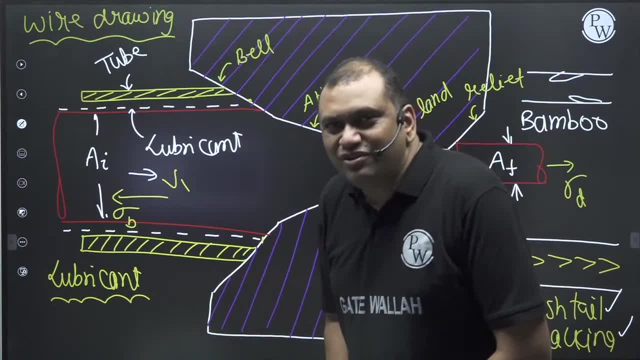 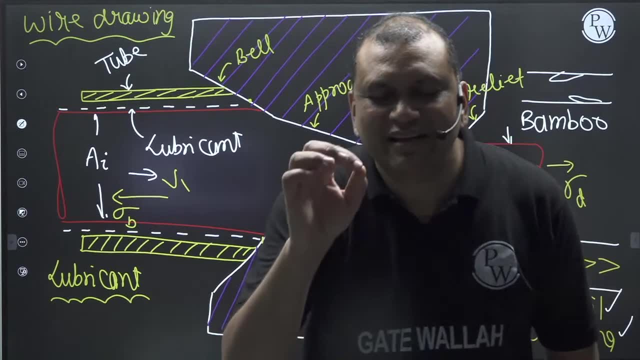 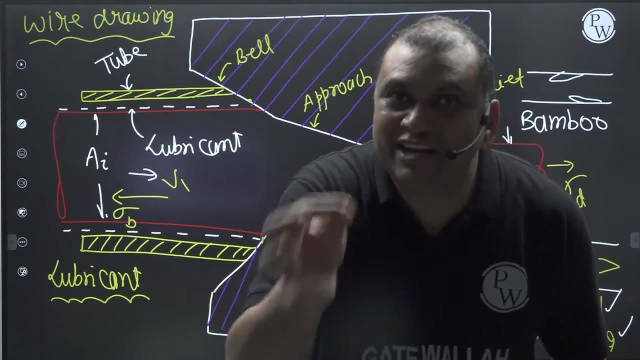 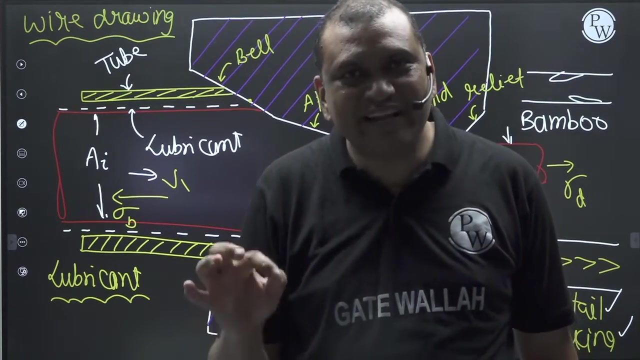 It will not splash because it is a tube. So now see what I am going to say in a sentence. Lubricant cannot be said here, So the momentum of lubricant will be lost. Momentum of lubricant will be lost. Momentum of lubricant will be. 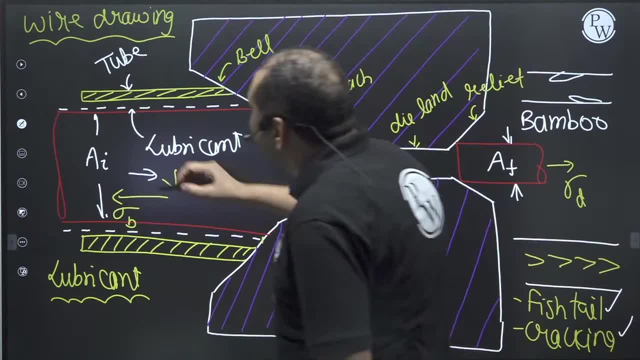 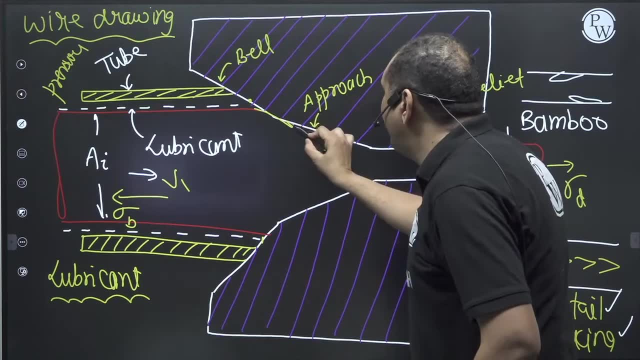 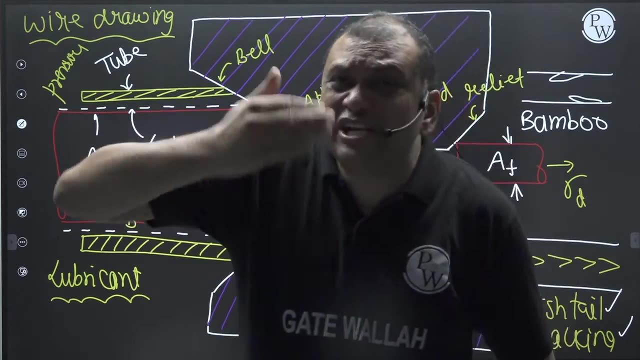 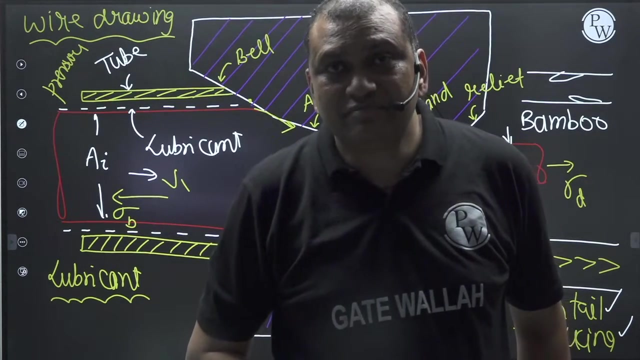 lost, And this will convert into pressure. This will convert into pressure, And this pressure enables the lubricant to enter into the deformation zone. Loss of momentum will convert into pressure, And this pressure enables the lubricant to enter into the deformation zone. So what is the purpose of tube? Pressurized lubrication- What is the purpose of tube? 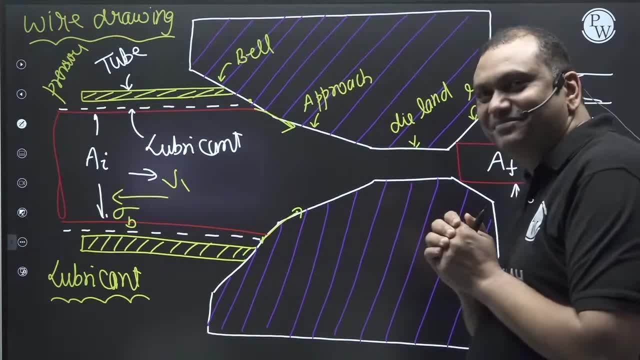 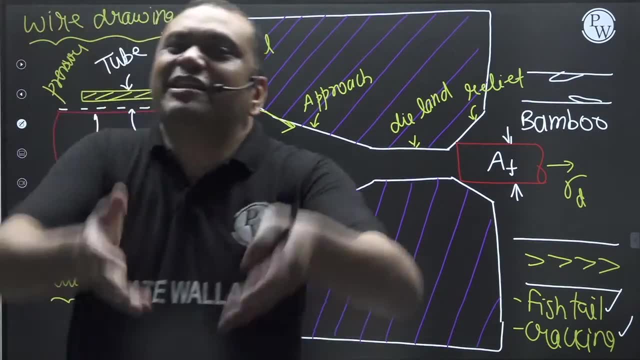 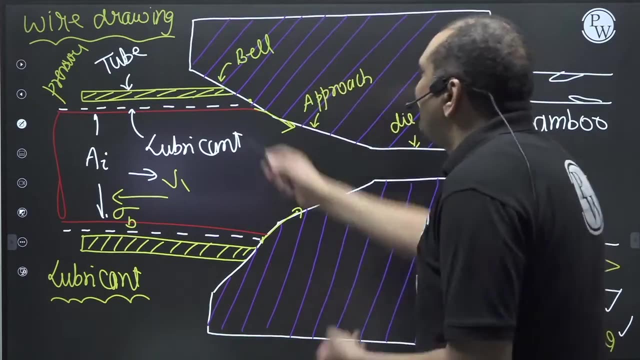 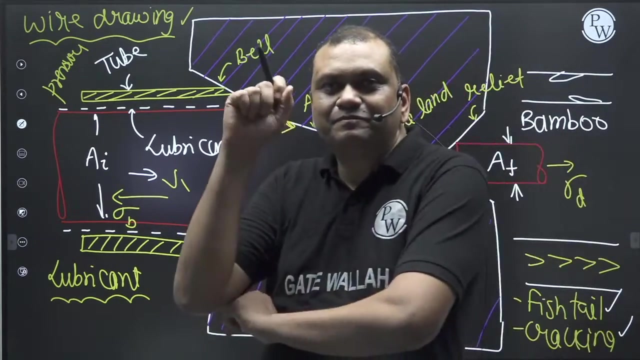 what is pressurized lubrication? is this right or wrong? this is not material science. this is forming. what is wire drawing? he is teaching material science. this is wire drawing. this is heading written. wire drawing comes in forming. you are doing great. now see. 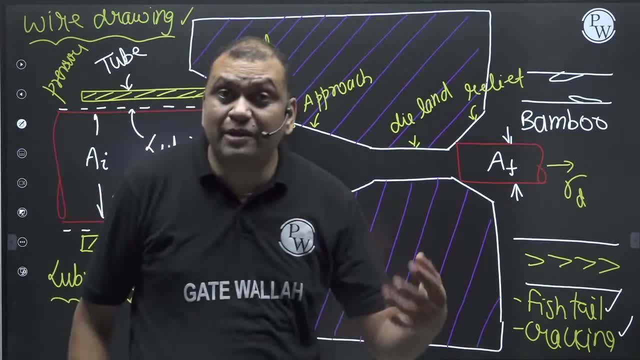 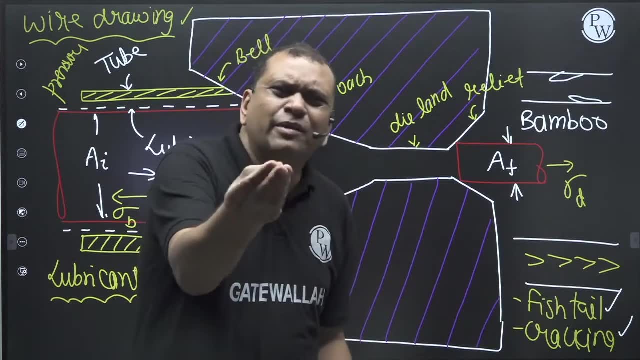 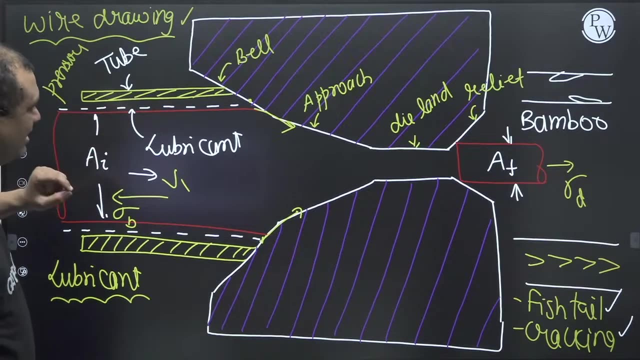 this equation comes in objective, which I am telling you in 2 minutes. it does not come in gate, but actually there are so many PSEs this question is repeated. it is repeated in ES. actually, listen, this is your incoming material. its area is AI. so first, how will you enter in the die? 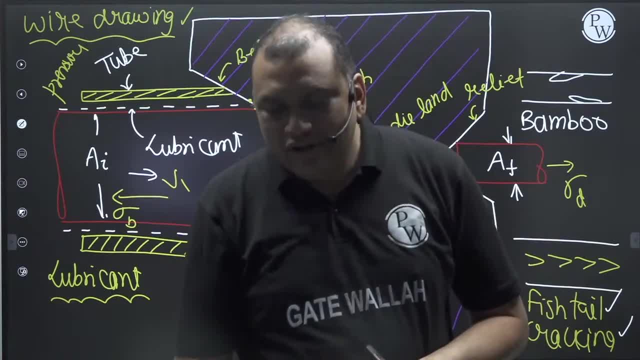 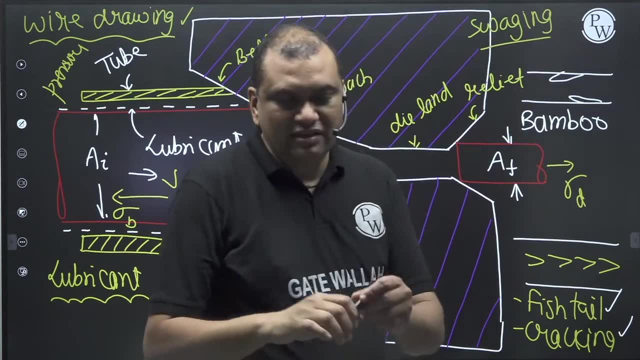 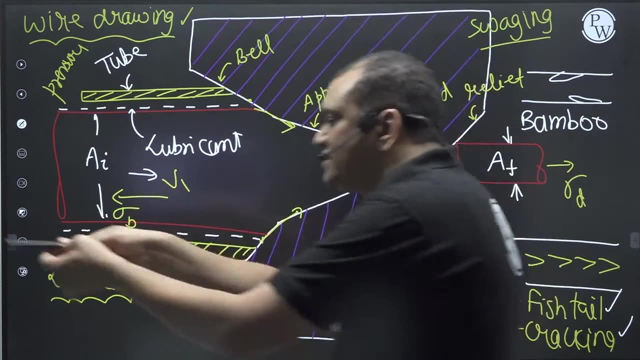 we have to make its diameter small. and how do we make it small? with swaging operation. this is swaging, this is a forging operation. so I have held the tip with a dime and hammered it from all sides, so it will become a tip. now remove this tip from the die. 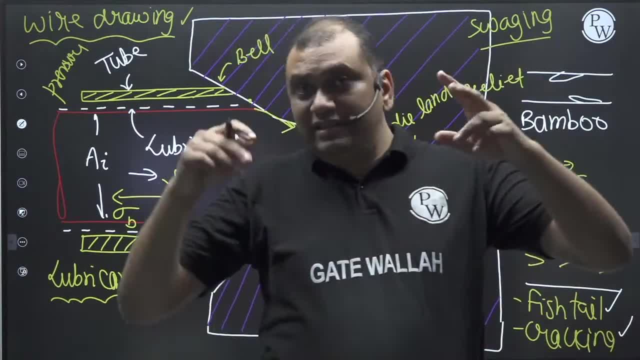 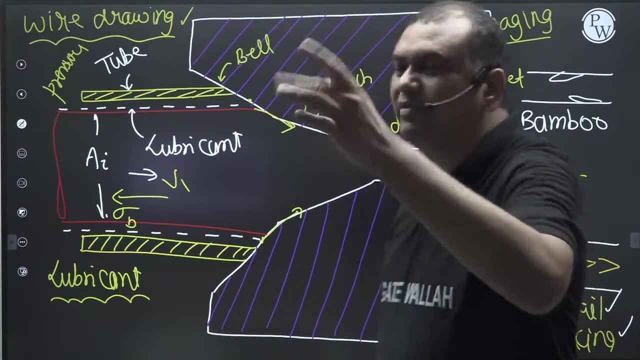 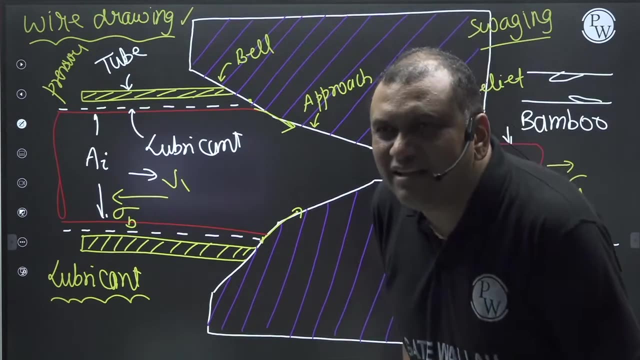 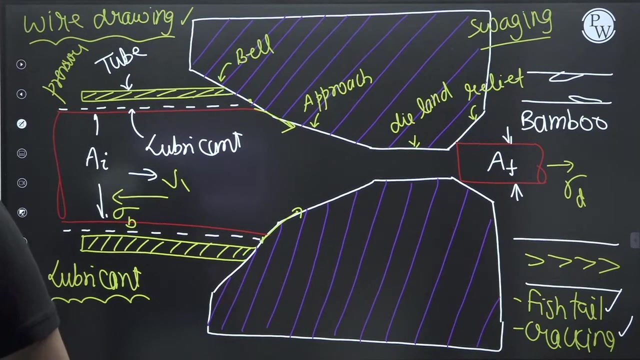 and pull it out like this. so this is how the preparation is done. this is how the drawing starts. this question comes in PSEs. it is repeated in ES also. you have to be careful. now see for different regions. we understand the application. is your brain cool? 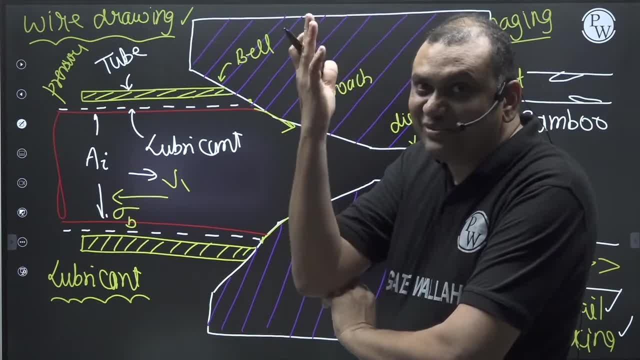 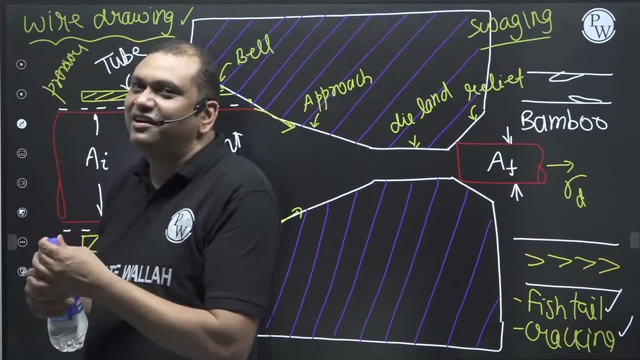 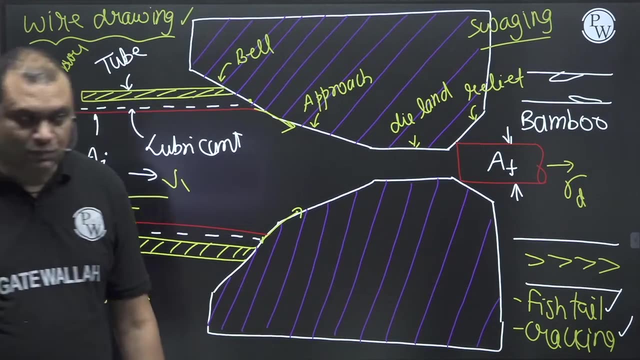 it is raining everywhere in India, so your brain will also be cool. it is very important to have a cool brain for forming and for production. it is very important to have a cool brain. surprisingly, friends, this is a very nice. have a cool brain. there are four ways to build a good brain. 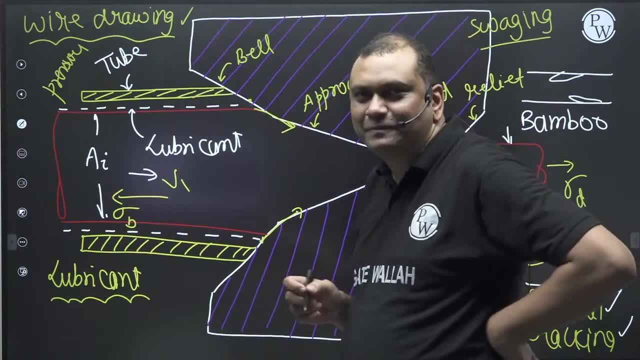 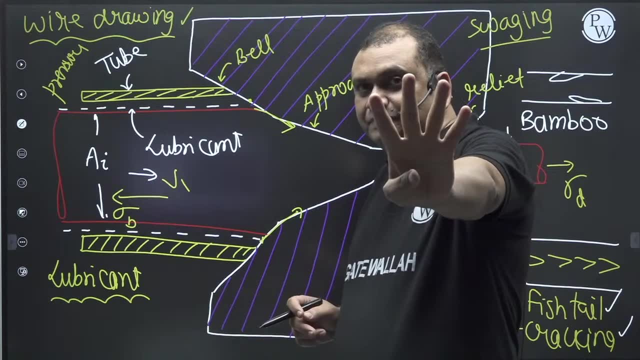 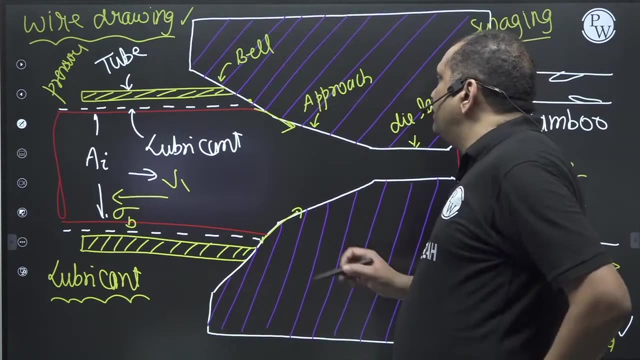 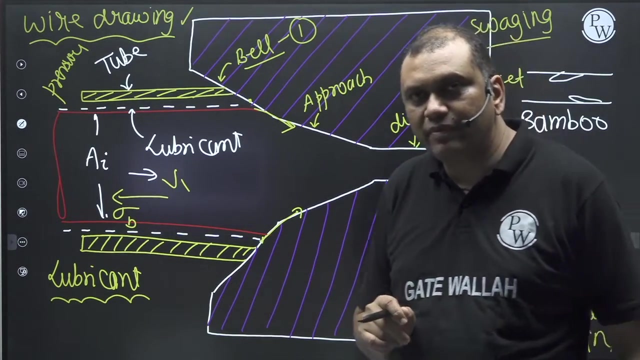 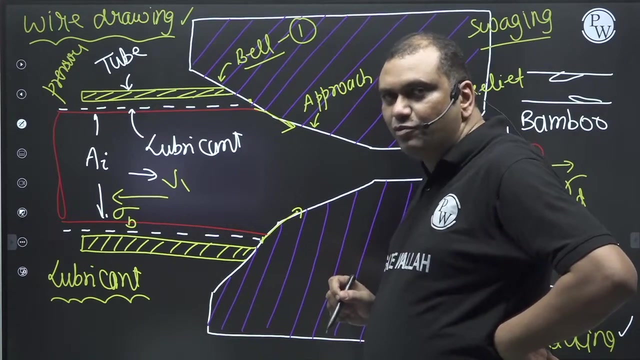 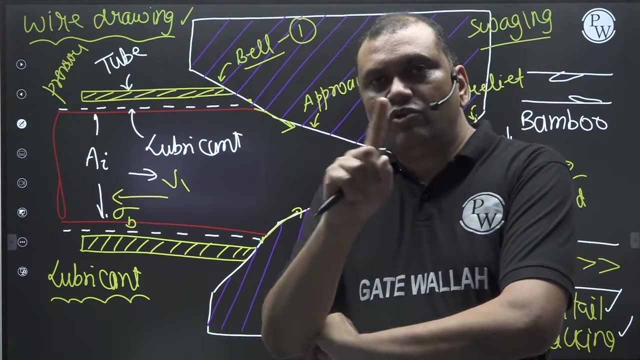 out of overnight announceいる bang Jedi dursing don't know. wait, wait, wow, 野 baby is working. I do not know any. questo 20, 20, this tube which is fitted in the bell section. there is no plastic deformation in the bell section. 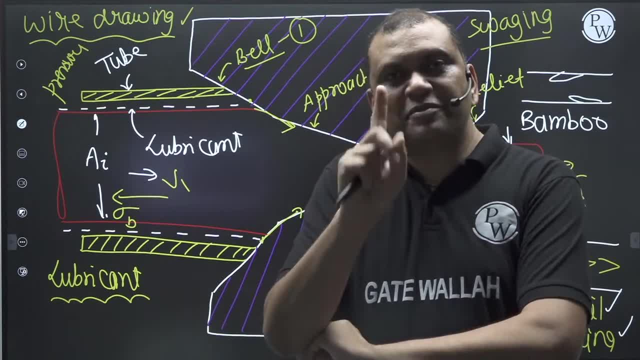 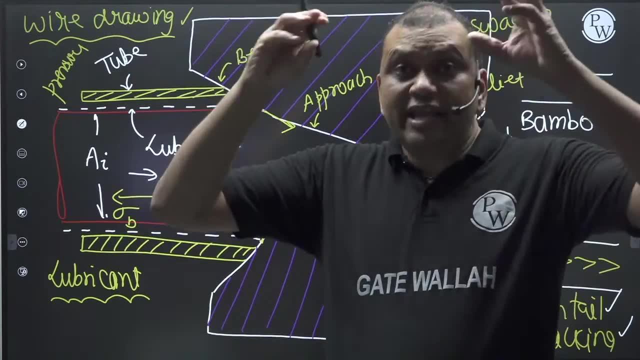 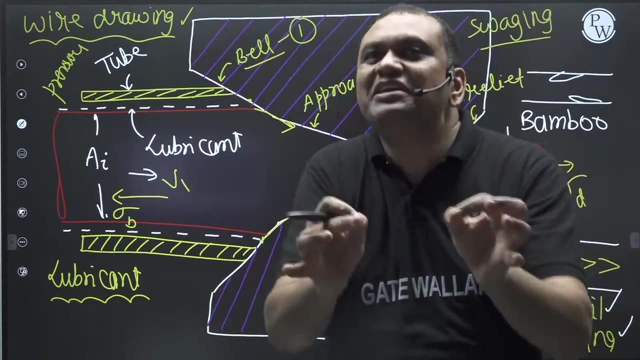 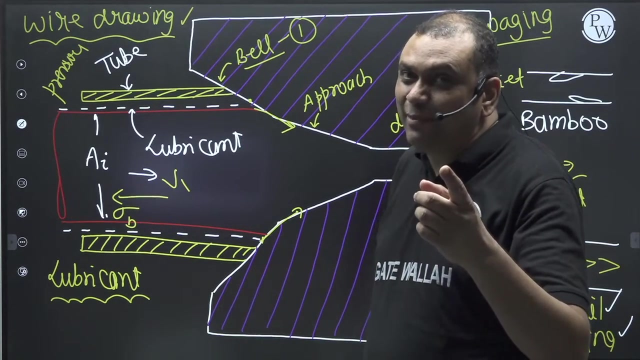 please remember, there is no plastic deformation in the bell section of the die. deformations are primarily elastic. in the bell section there is no plastic deformation. deformations are primarily elastic. today's lecture is very important. please don't doze here. it's already 10 pm, stay attentive. 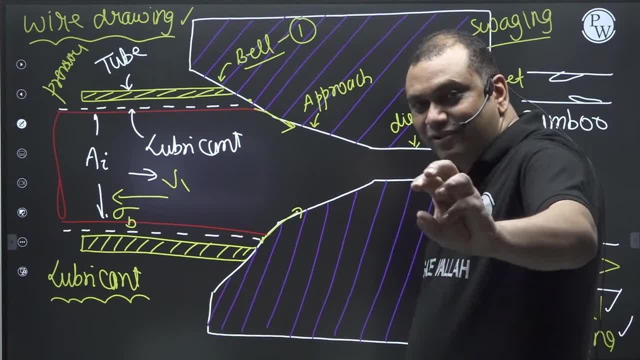 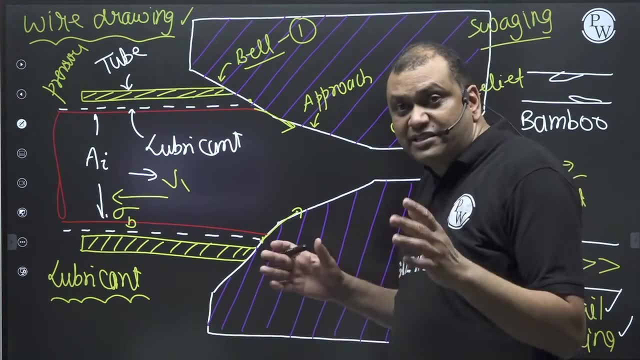 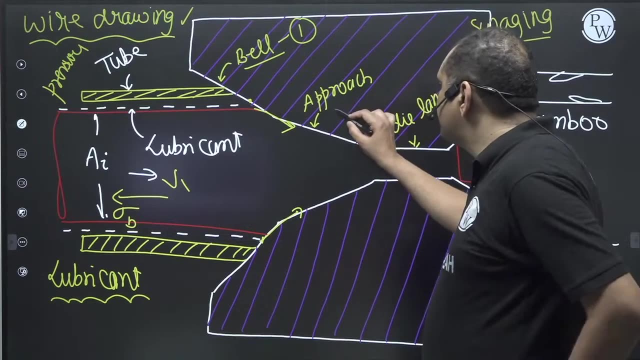 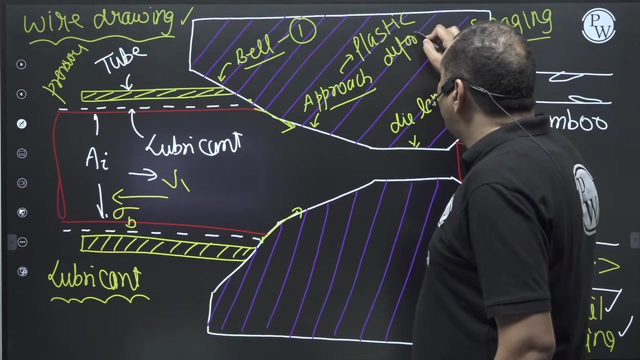 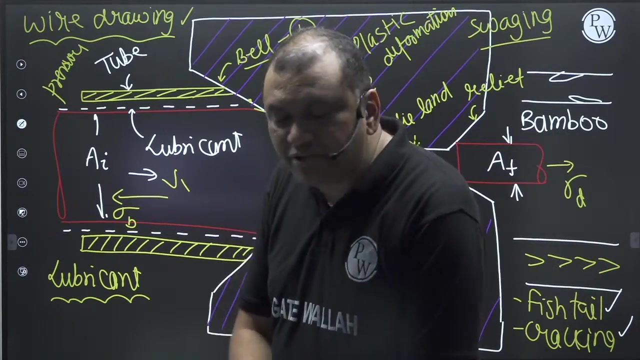 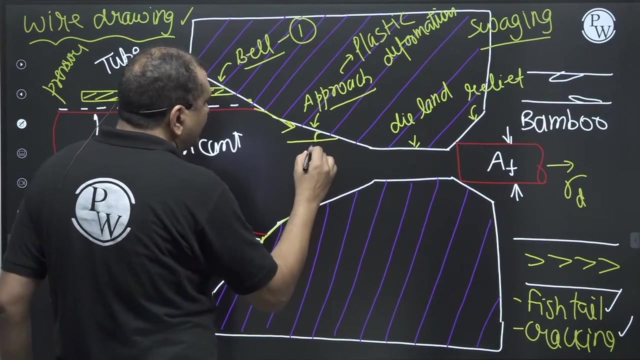 bell section. deformations are primarily elastic. plastic deformations are primarily elastic. plastic deformation doesn't take place. plastic deformation takes place in the approach section. in the approach section there will be plastic deformation. the angle of the approach section is alpha. it is called as semi-diangle. 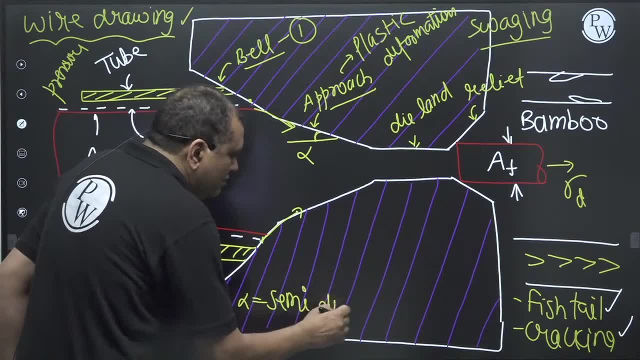 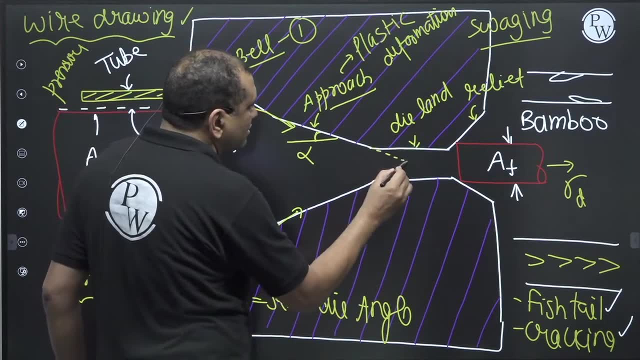 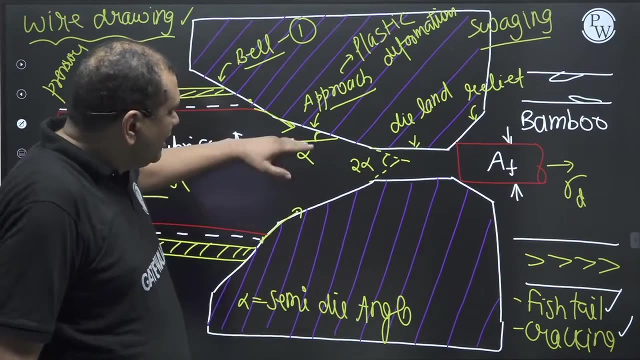 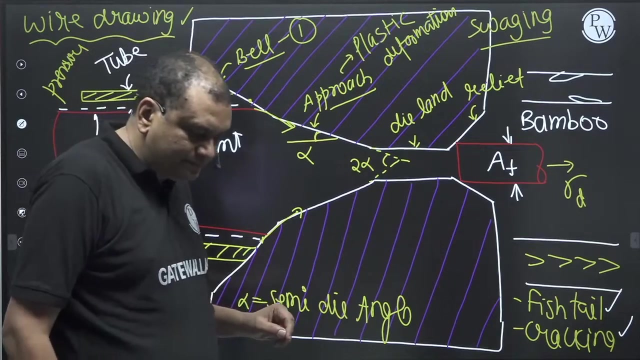 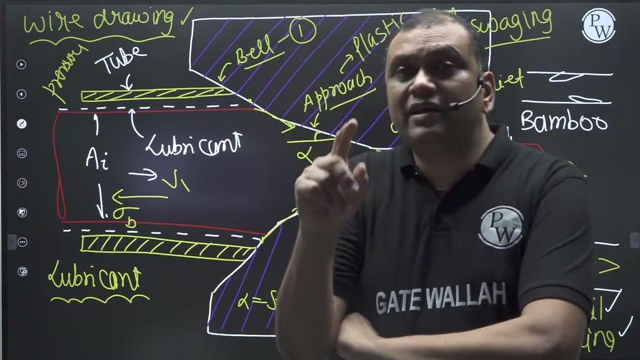 semi-diangle. what will be the full angle of the die? it will be 2 alpha. 2 alpha is the angle of the die and alpha is the semi-diangle. so the plastic deformation is taking place In the approach section. listen to me carefully. very, very important in the last 10-12 years. 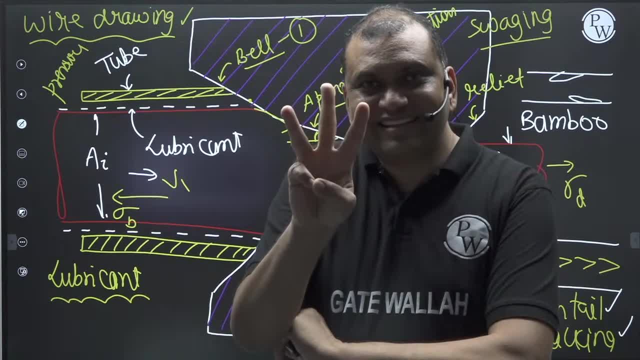 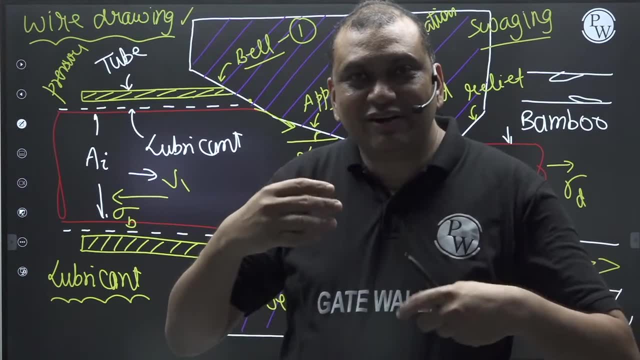 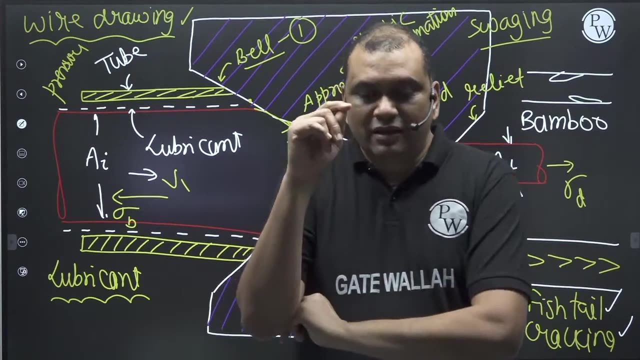 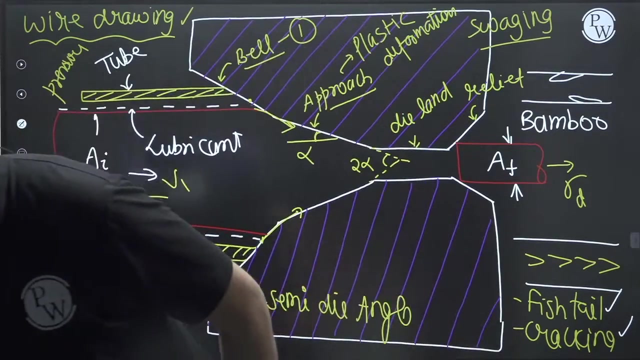 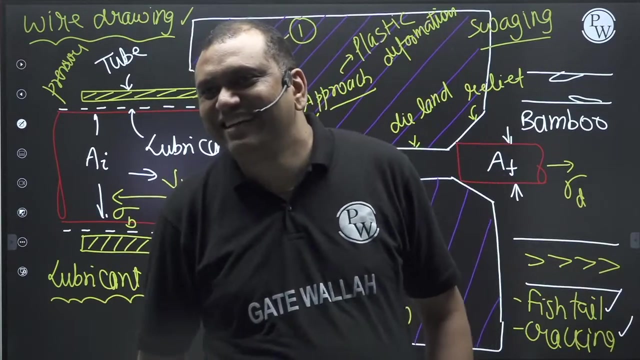 one type of question has come three times in the gate. one type of question has come three times. And what is that? Listen to me carefully. sometimes the question comes- everybody is hearing. sometimes the question comes- Brother, please mail it to me actually- notes, etc. actually I can send it to my regular class notes. 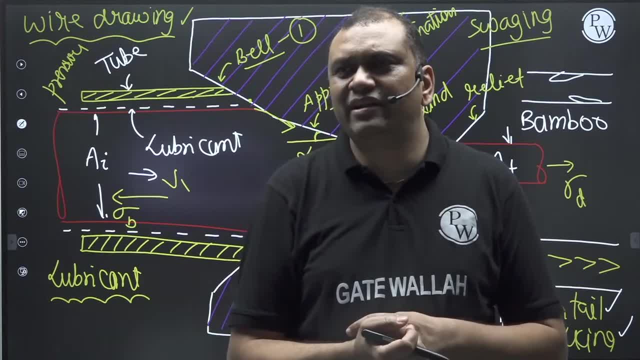 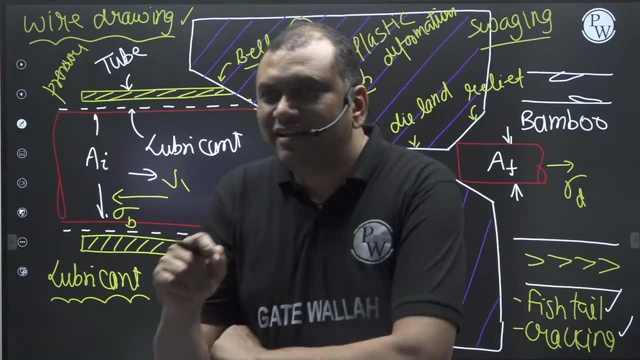 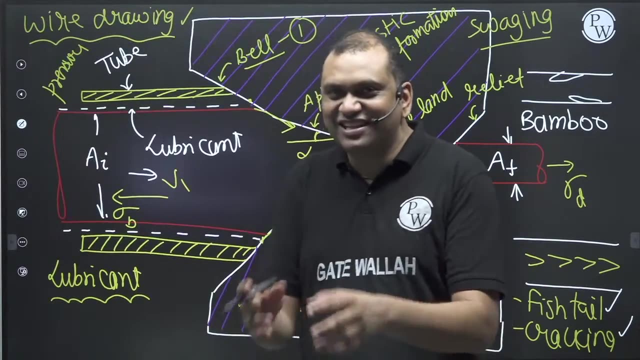 somebody can give email id to my email. somebody can put email id in the chat box, my email id. Now, how did it start? like crying gate aspirant 2023, what is happening like crying this animation? I don't understand actually, because I don't talk much in the chat box. 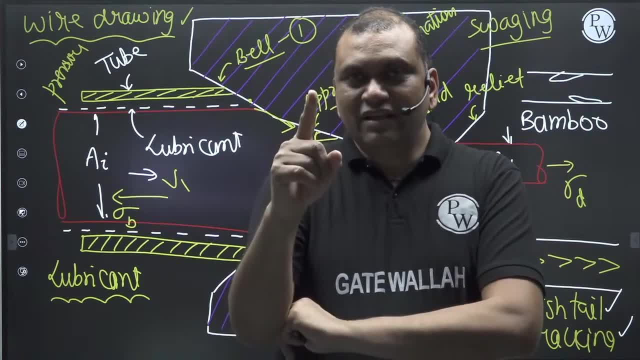 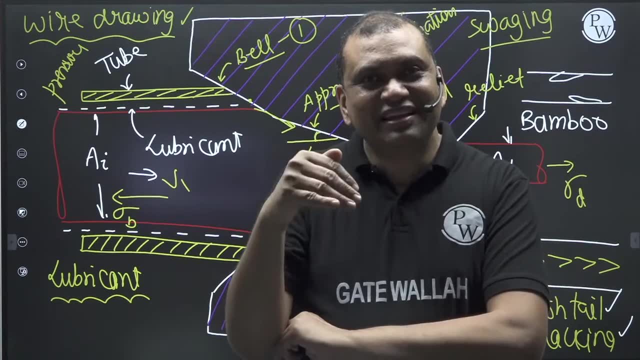 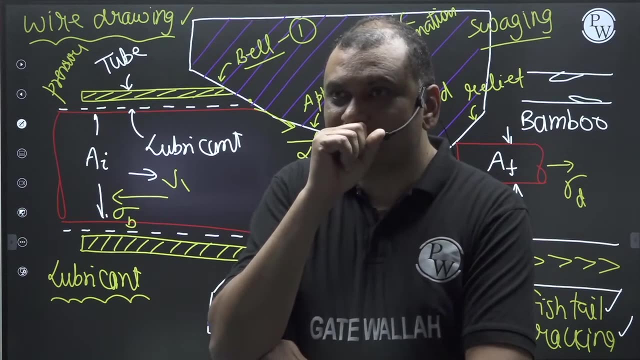 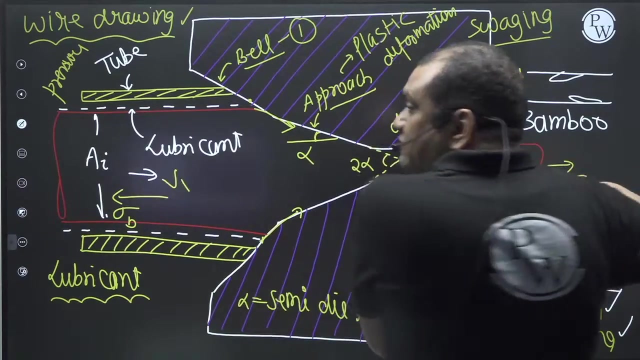 Listen to me carefully if the question comes: what are the type of stresses? in the day Drawing x to z. rolling question is: what are the type of stresses? Answer is very simple. I am drawing y. I am drawing the material from the front. 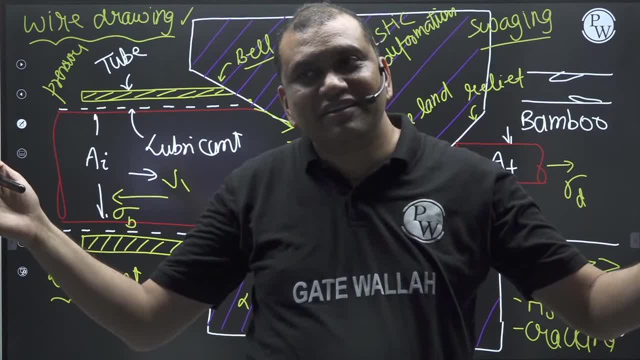 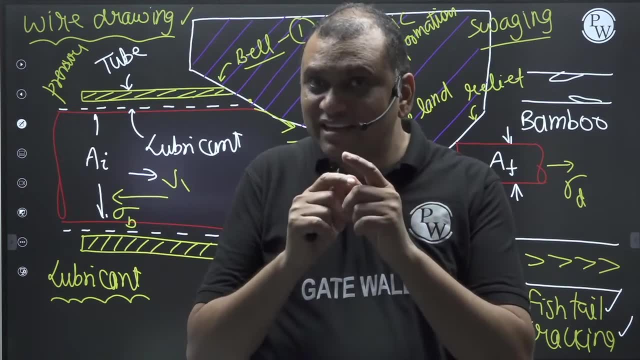 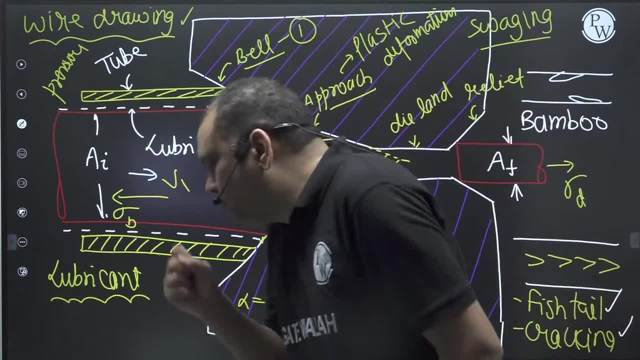 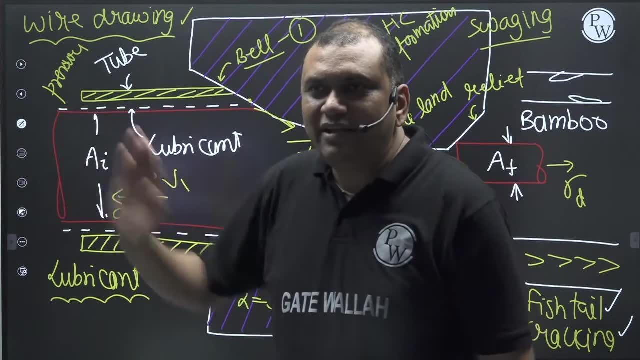 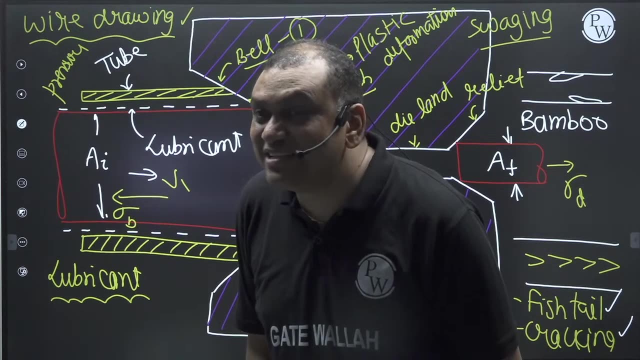 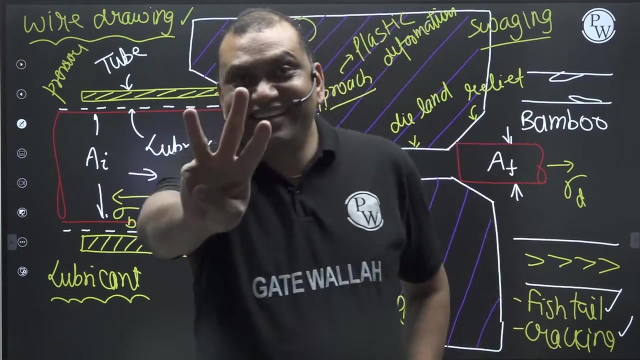 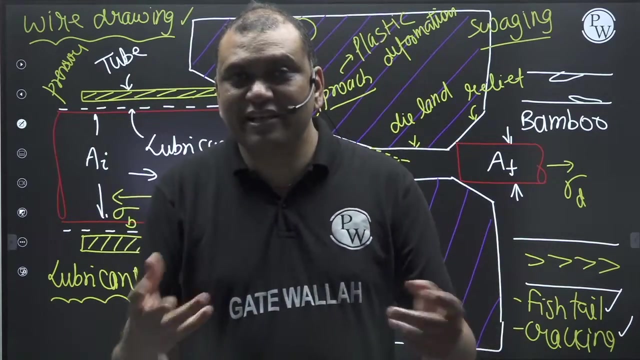 Extrusion. what I am doing is you are pushing the work piece from the back. This means it is, this means it is compressing. See again, see again, see again. Ohhh, I have put the paper like this, really, if you see, fine me now. 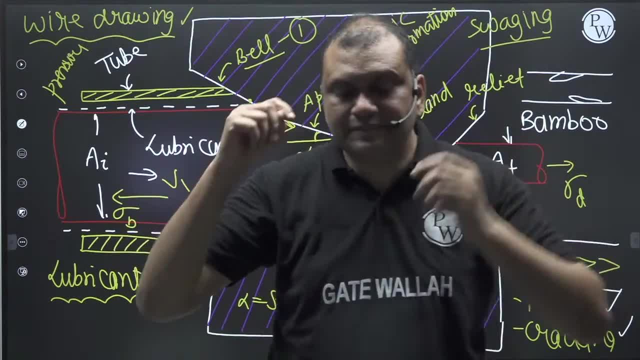 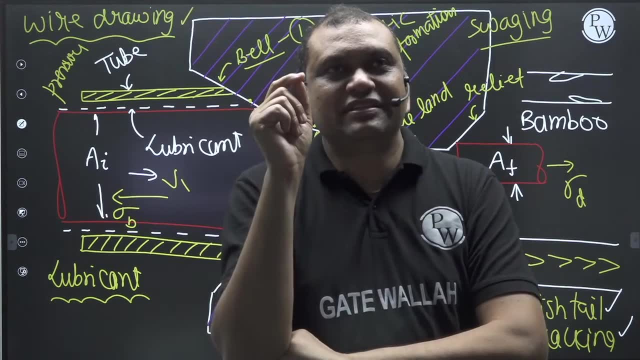 You have seen, you know well, like PYQ, Hype, Hype. That's the way I am elastic. You have seen, That's the way I am elastic. Types of stresses in the getaway hand s police rising mode is meat gas. 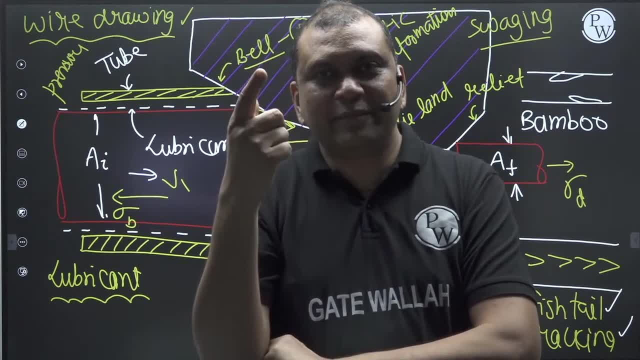 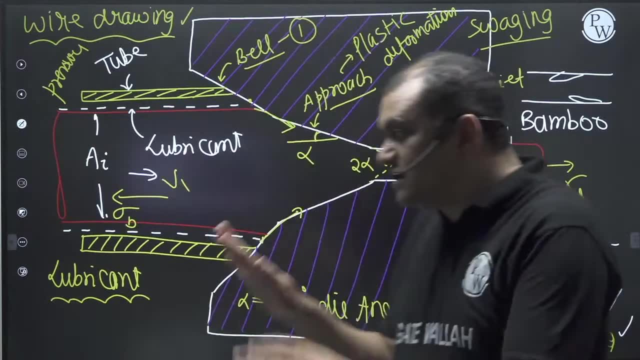 I will hit the paper, I will��� было it my weight. a lo macro wage shows that I won't delicious food". of stresses in rolling, So in wire drawing I am pulling it from the front. So tensile stresses In compression: I am pressing from the back. Compressive In rolling compressive. 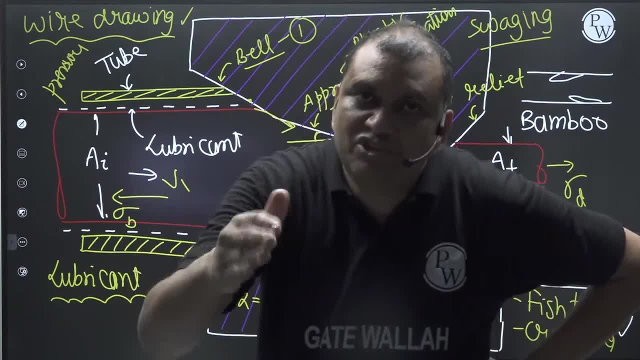 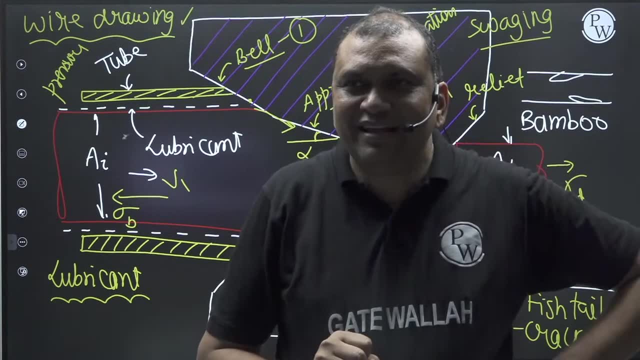 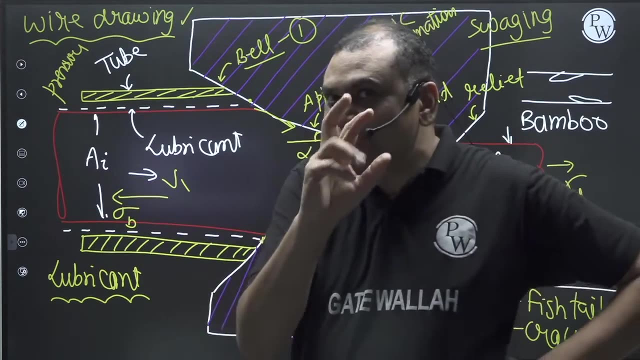 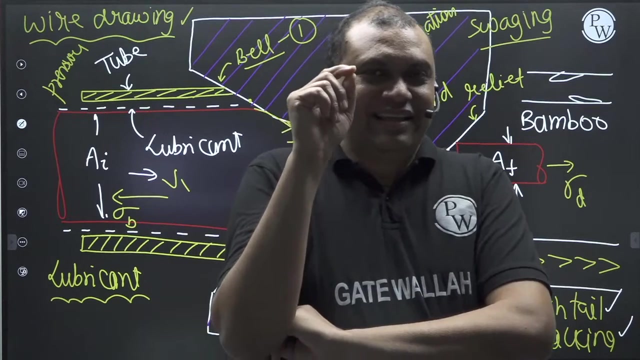 In forging compressive. So what will be the answer? The type of stress you are applying to deform The answer is correct, isn't it? There is a second variety question: Do you know what is its language? Now you will read the language properly. What is its language? 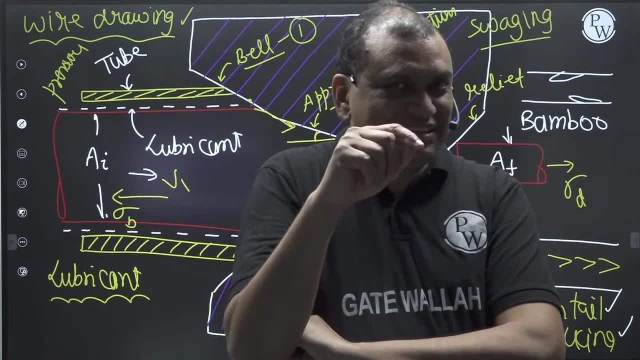 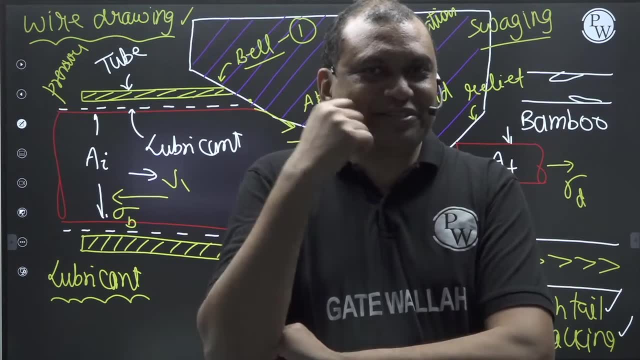 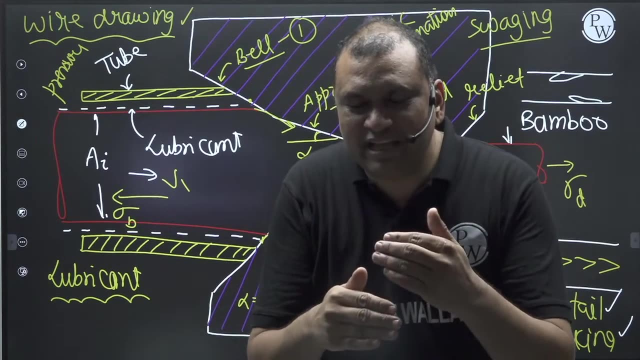 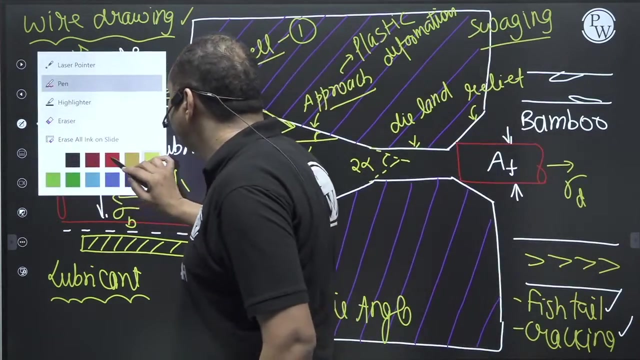 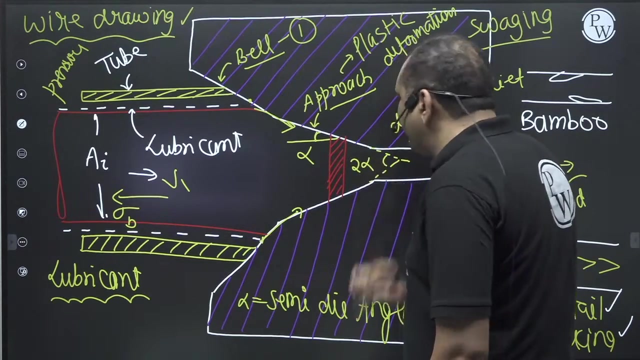 The type of stresses, the type of stresses a material will experience in the deformation zone, The type of stresses a work piece will experience in the deformation zone. Means, if you take a strip here, if you take a strip here, this is the deformation zone. 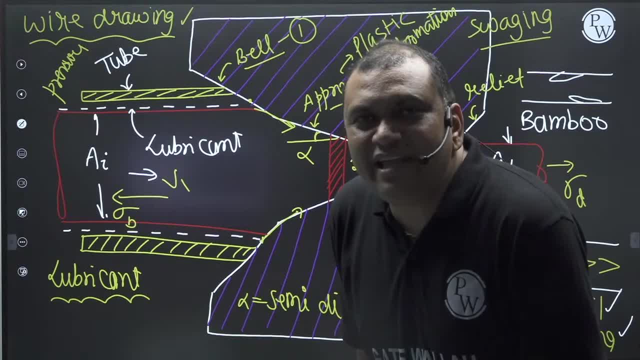 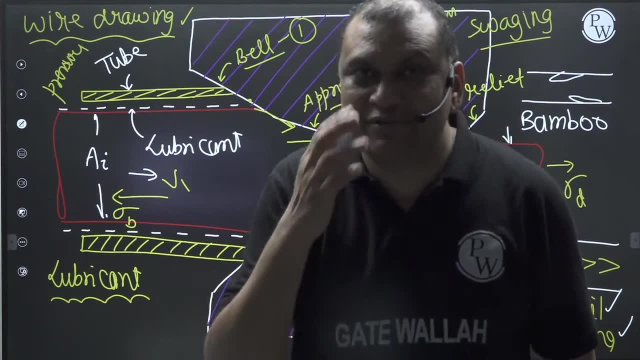 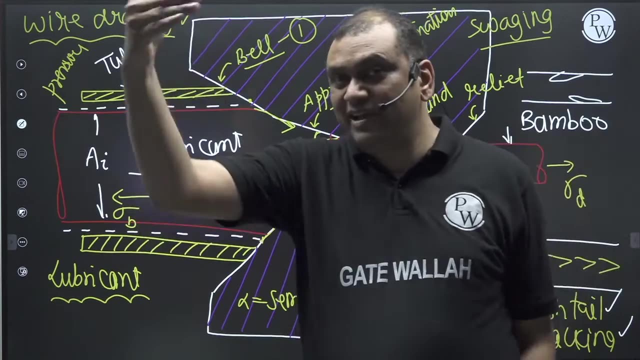 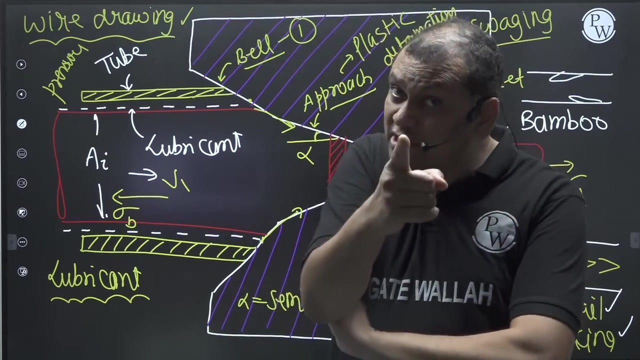 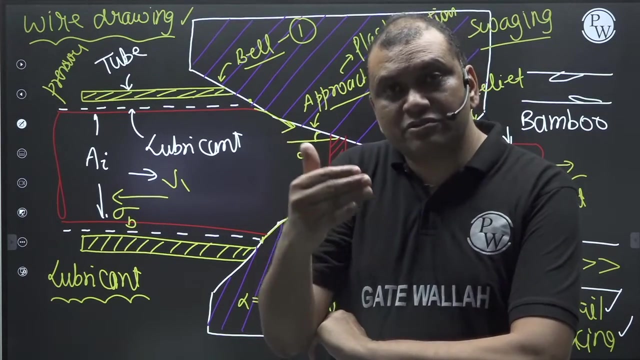 So the type of stresses any element in the deformation zone will experience. But you will not feel feelings of tension if you add shear in it, Because without shear deformation is not possible. So you have to read the question properly in the gate. The question is In the wire drawing. in the deformation. what are the stresses Tensile and shear? If our question says in the deformation zone you add shear In this gate, you will have to write the question correctly In the deformation zone. you have to write the question correctly In the deformation zone. 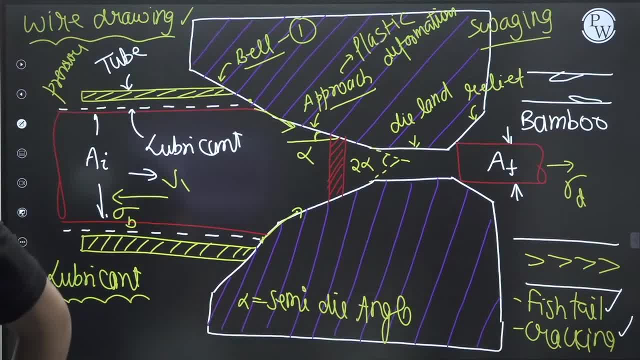 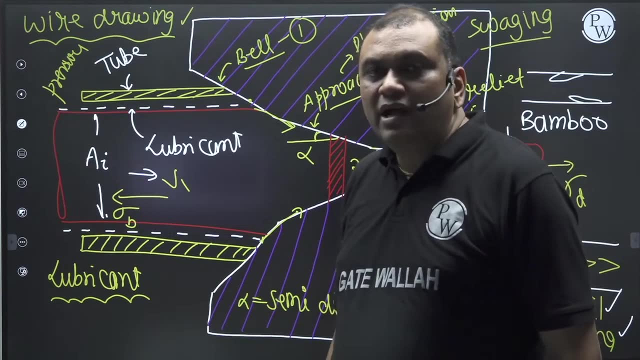 share it car. do take Anna. yeah, correct, what's my share? it come to bill goes a bullet. harsh Raj, he gonna up question pro just a, for example, rolling hair- I'm rolling me. can't hang out for a concert compression and share a good question. do Barra say below me? do Barra say below? 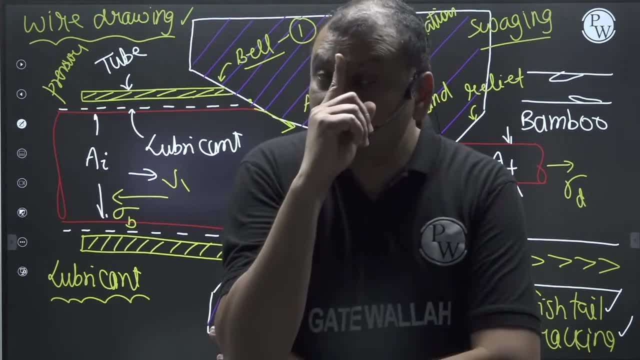 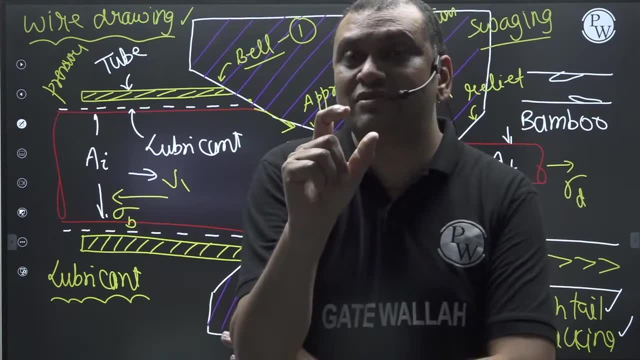 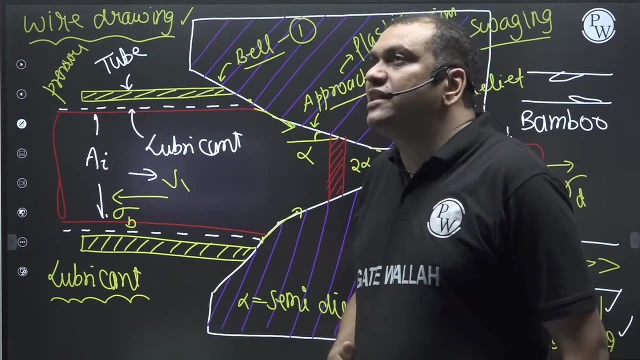 on coimbe larga: miss me career. guys say I got question man, yeah, what they're gonna have in the deformation zone. who's my share? drool at Karo. who's my share? drool at Karo. you don't get. the whole is my slab. 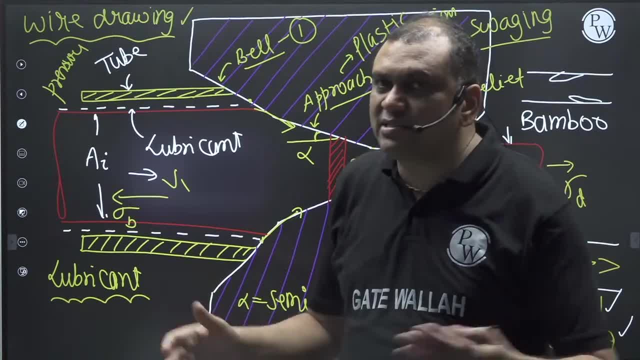 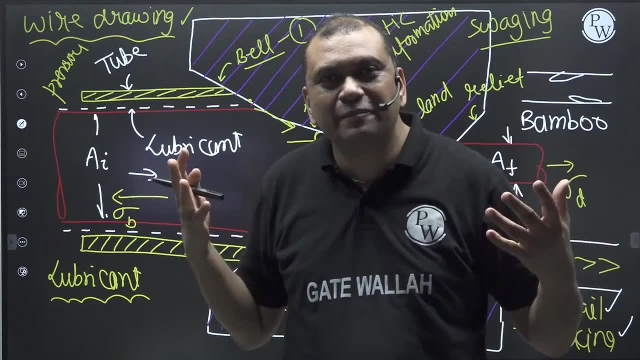 analysis. the detail proof me: Karana. balakrash course ma'am a slab analysis. the detail proof me: Karanga. I got proof karata home a to subcoach OBS. hota a kebhai binashir k kuch deformation hota nahi a myth Barra say: well Onga agar. 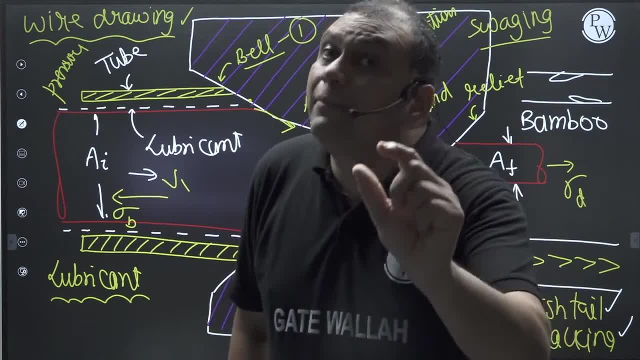 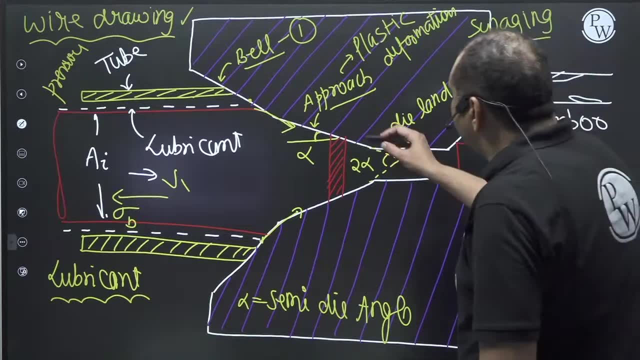 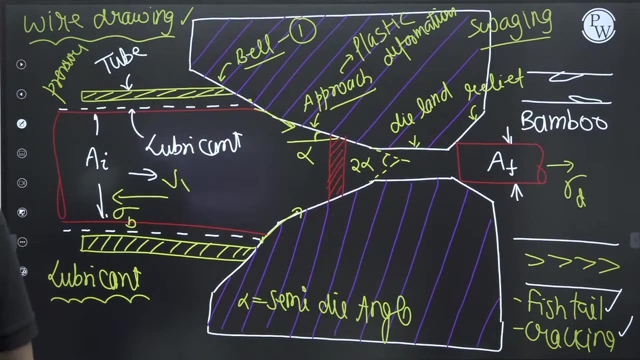 question: man deformation zone de raka. ha, I'm co share, add Karna, hey, please don't forget that. so, Amara deformation, or a pro section man, now dial and a purpose, kia, hey, share your friction, give us a yoga friction, job share, give us a yoga. 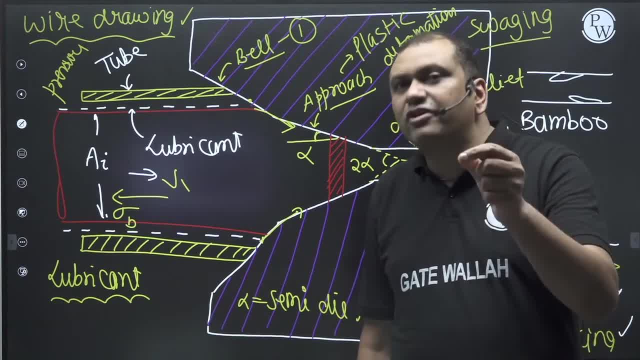 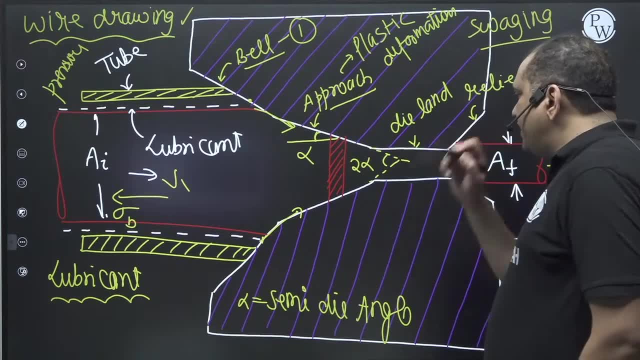 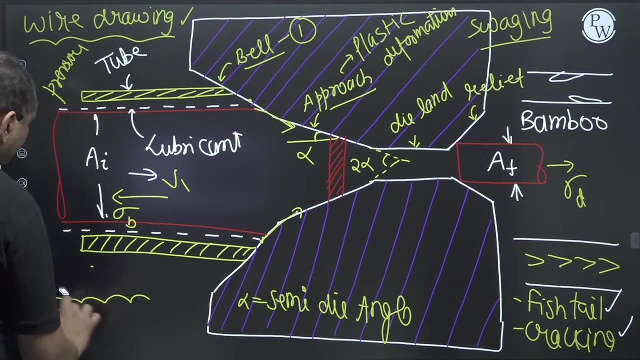 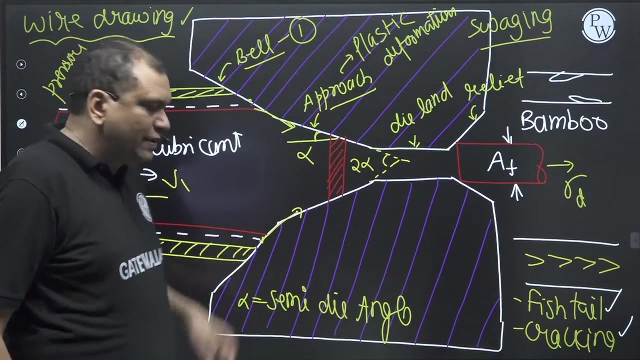 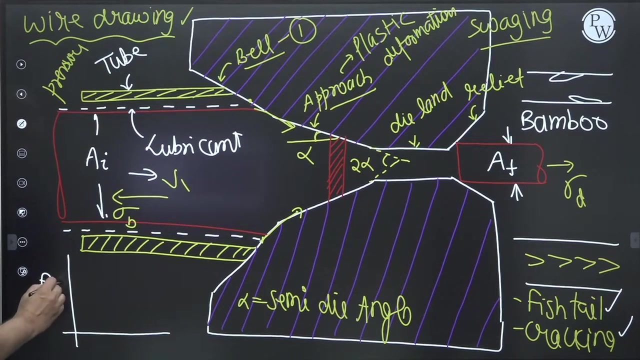 or binashir k. deformation is not possible without share, deformation is not possible. he got dial and Johan you dial and hair is dialing. a purpose kya hey? dial and car purpose, kya hey agar? a big graph thinking a between the drawing force and the diagonal drawing force iselle. 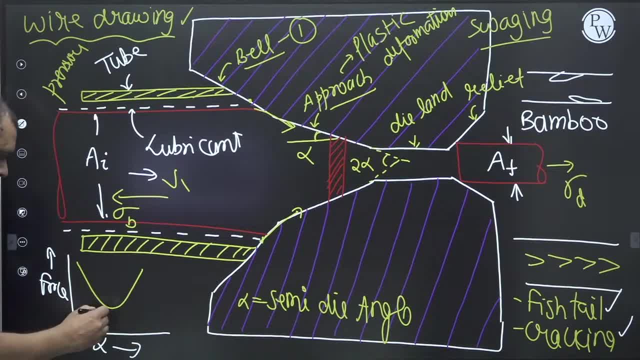 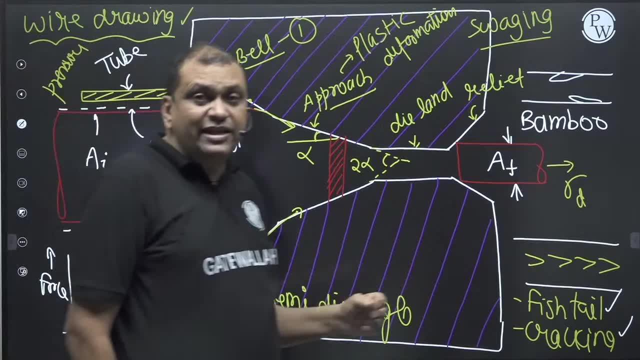 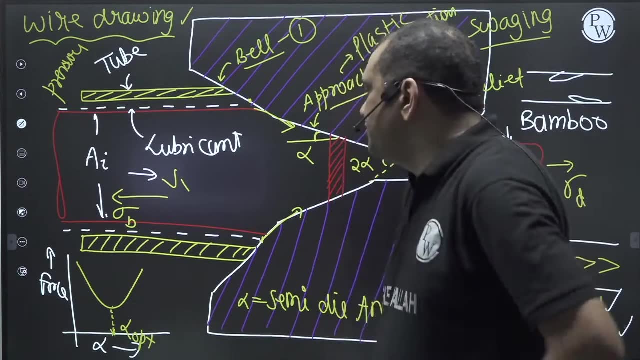 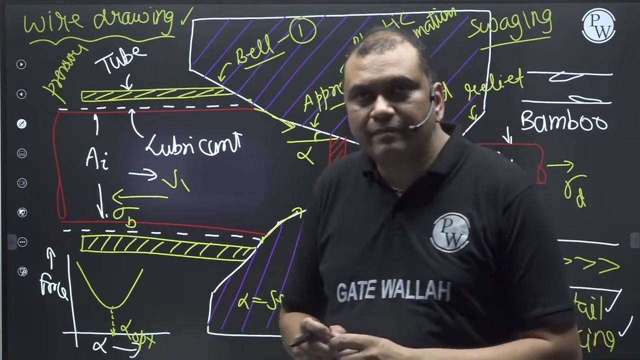 yourself kalo you, you drawing force. and the CMI triangle- tea and hair graph goes like this: there will be an optimal CME die angle thick, drawing forces minimum. there will be an optimum diagonal for which the sheer force- and I'm far with the drawing forces- minimum. 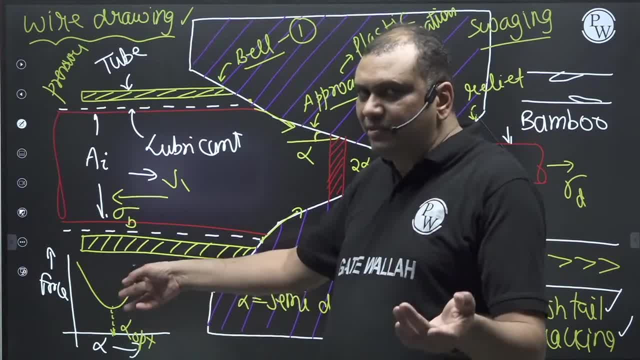 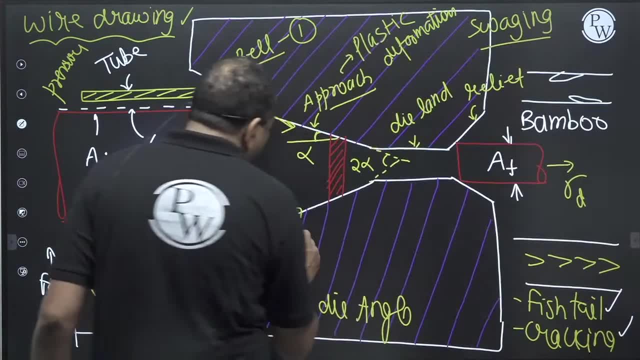 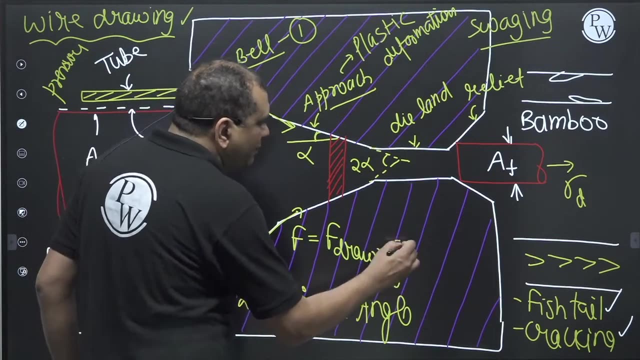 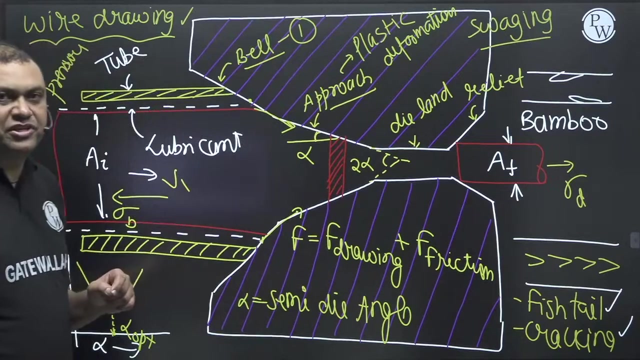 There are two reasons for this. I will briefly touch on this. I will not get into the detail. The total drawing force depends upon the energy required in drawing, plus energy required in overcoming the friction. If we increase the semi-die angle, then the friction component decreases. 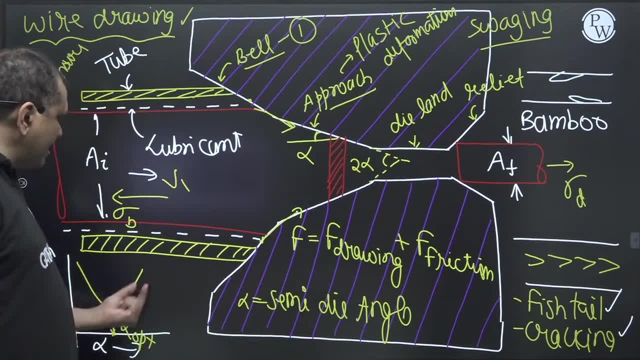 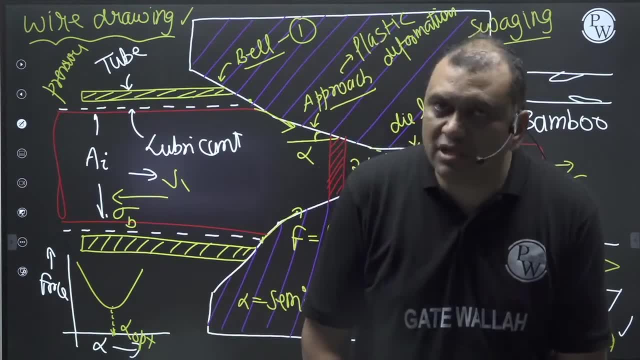 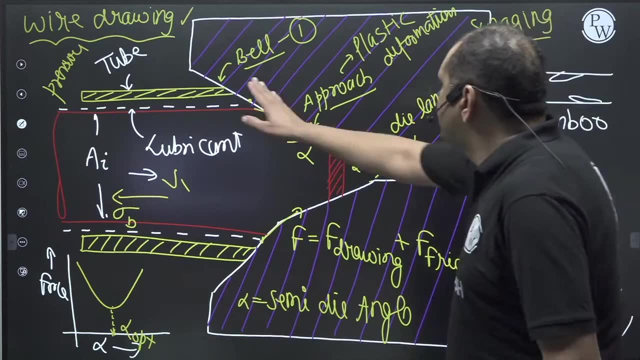 If we go beyond the optimum, then there will be the formation of dead metal zone. Due to this, the force increases. I will not go into the detail as I am teaching you a crash course. In the bell section, there will be an elastic deformation. In the approach section, there will be a plastic deformation. 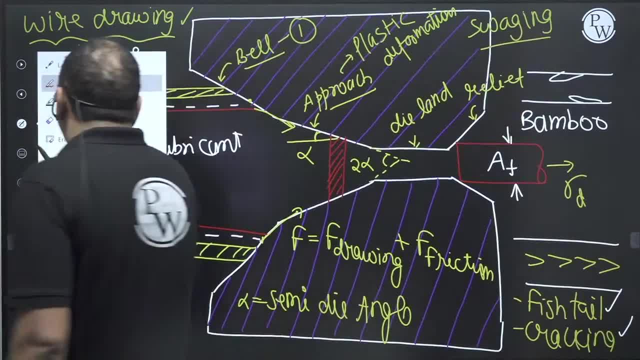 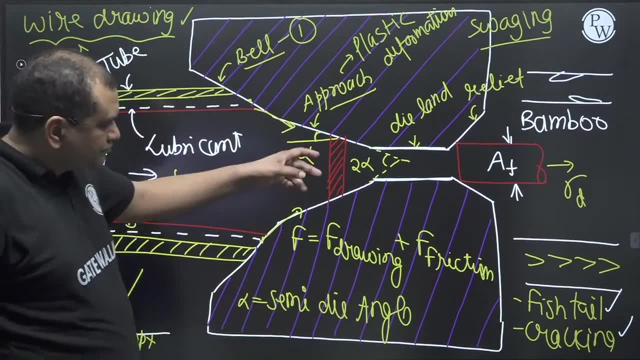 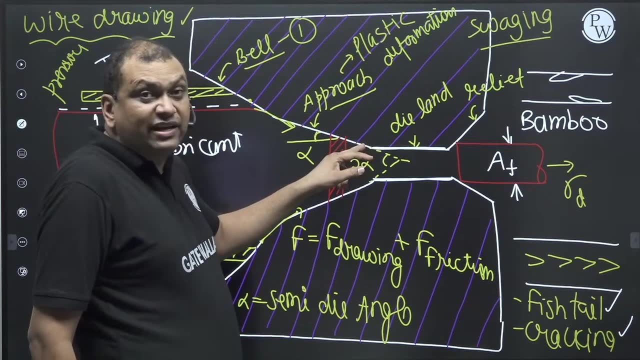 Now, in the dive section, there will be an elastic deformation. In the approach section, there will be a plastic deformation. Why do we provide a die Now? why do we provide a die? The reason for this is that if you suddenly increase the die area, then it will break. 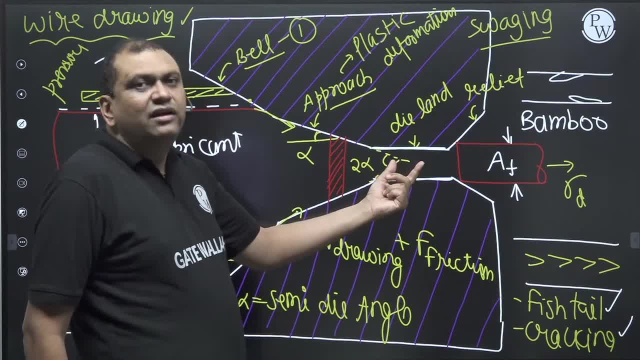 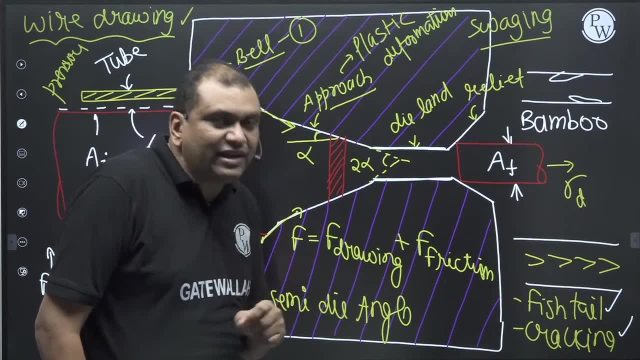 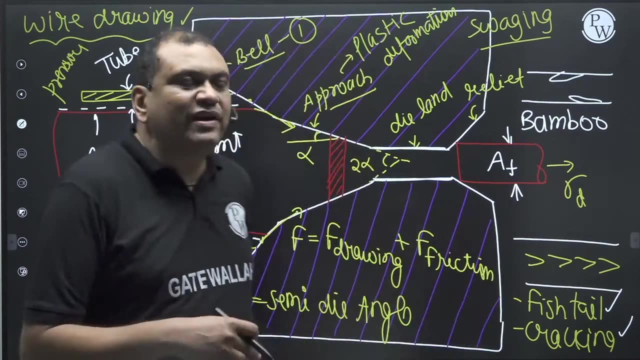 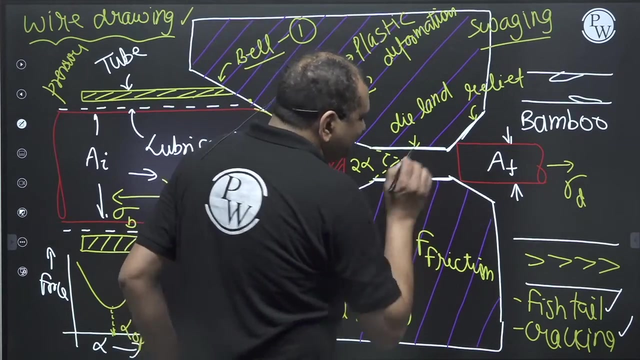 Thus we provide a land so that the die remains stable and does not break too soon. But of course, by providing the die land, By providing the die-land, more energy will be required for deformation, And this is called relief. What is relief? 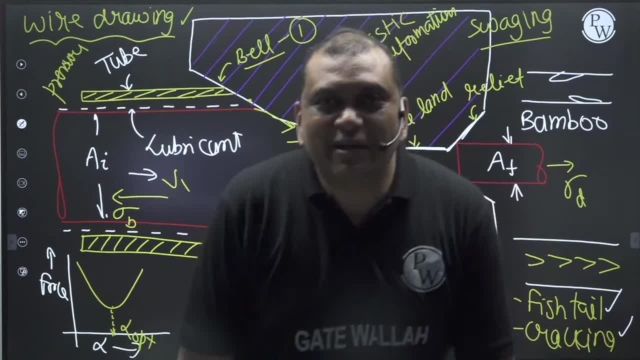 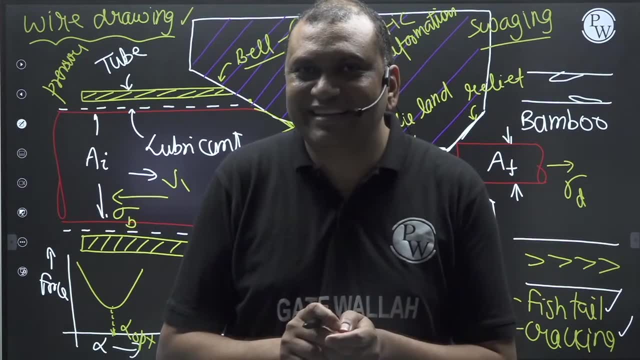 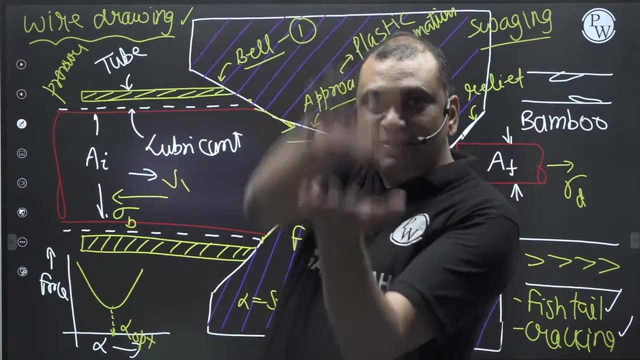 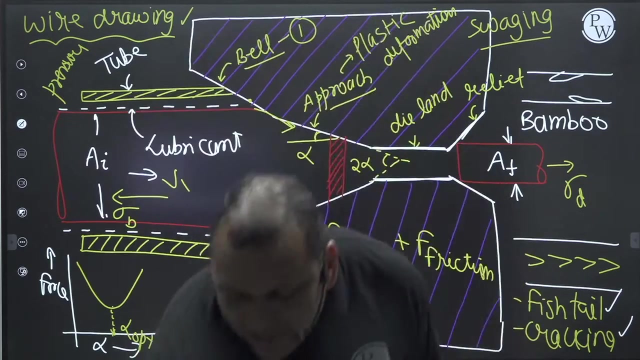 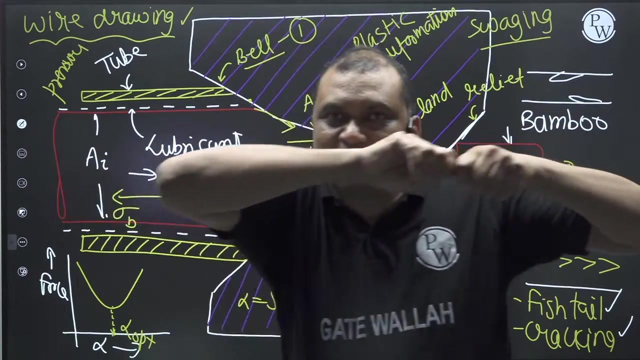 When you remove the load from the material, elastic strains will recover. For example, when you are forging. when you remove the load, the size will increase. When you are wire drawing, the length is increasing. in the wire drawing, the diameter is decreasing. 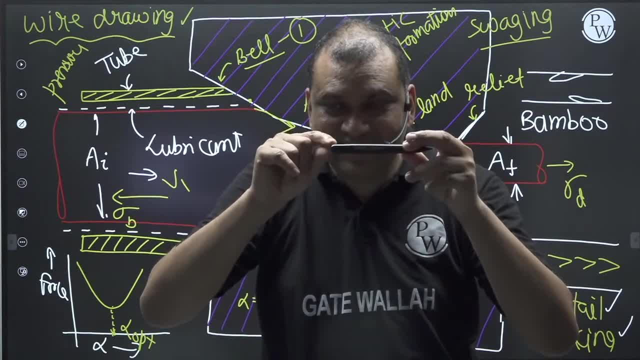 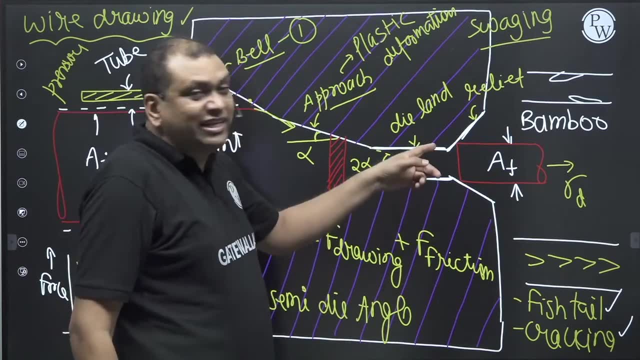 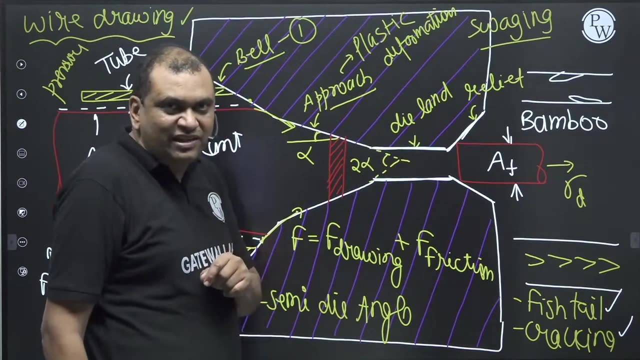 When you remove the load, the length will decrease, the diameter will increase. This phenomenon is called elastic recovery, Elastic recovery or spring back. To accommodate this elastic recovery or spring back, we provide relief. You must have seen that our outgoing area is slightly larger than this area. 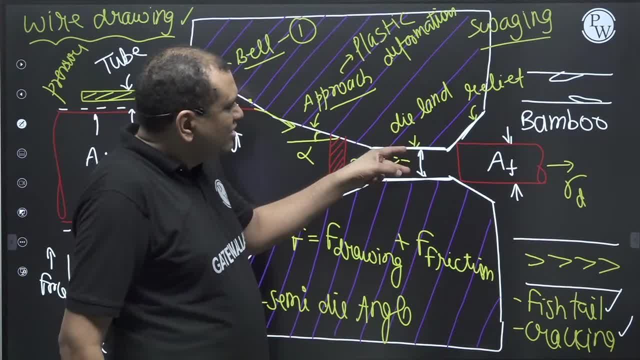 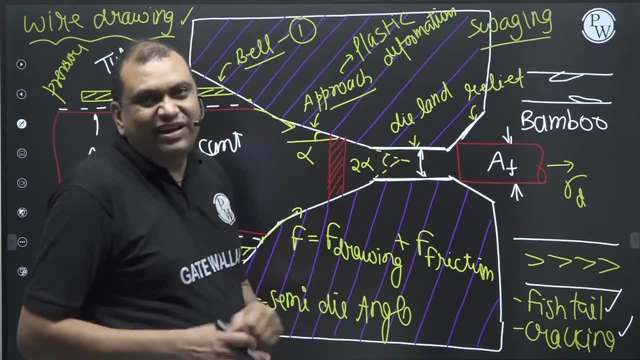 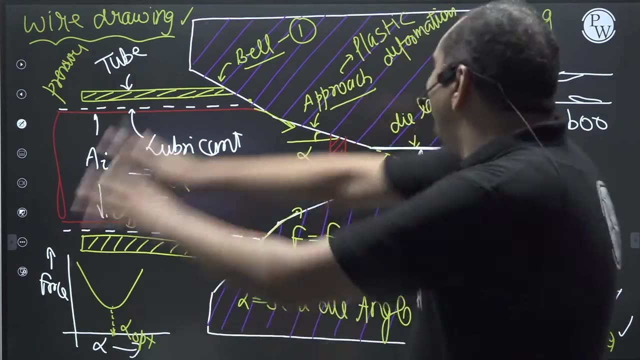 I have drawn it, The AF is slightly larger than the die area. Why is it larger? Spring back. So to accommodate spring back, we provide relief. To accommodate spring back, we provide relief. So this is the function of our die. 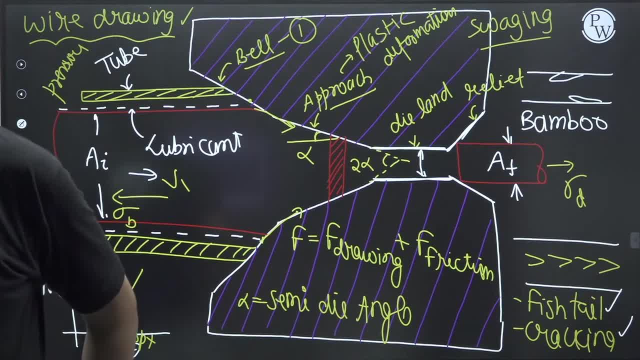 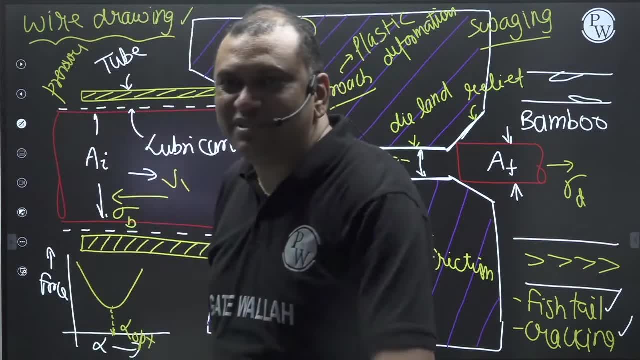 You can see what is going on in the chat box. I didn't tell you what the step-land theory is. Actually, I won't tell you Very good. Actually, a lot of positive discussions are happening in the chat box. Actually, I will limit the discussion in the crash course. 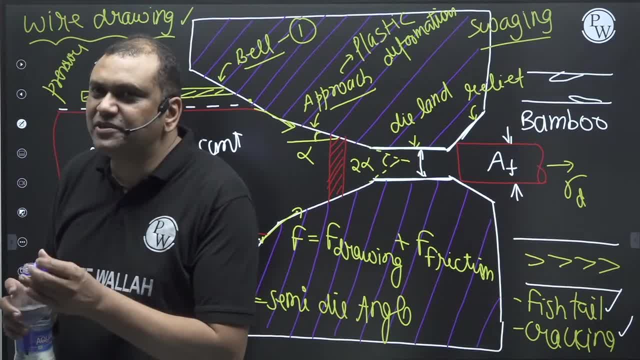 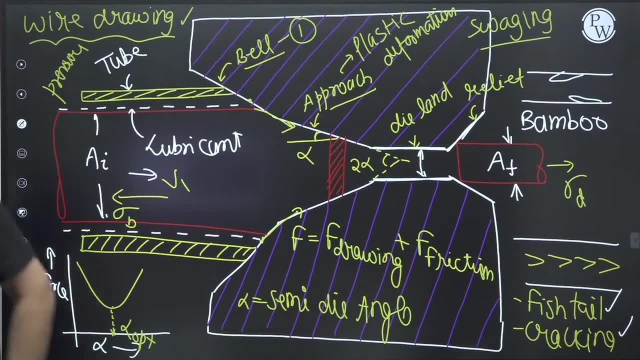 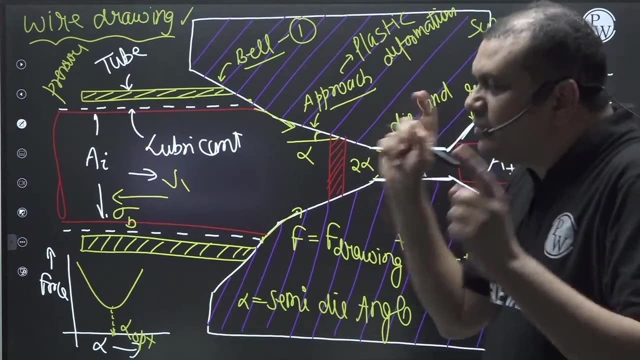 So that you can crack 80% problems in gate 2000.. Then you will also get 100% results in gate 2023.. Alright, We were going very well till now. So what did I tell you in the discussion till now? 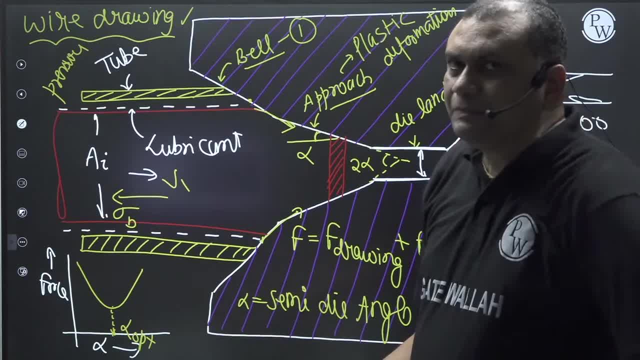 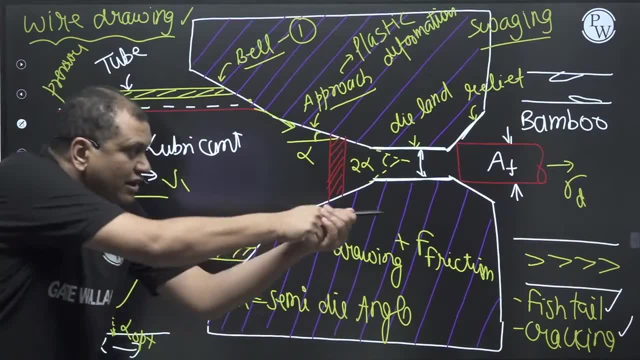 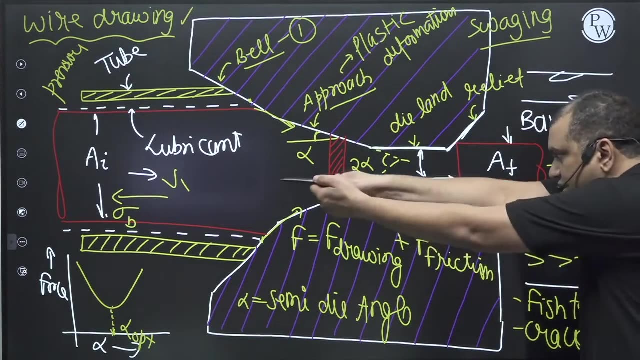 Die has 4 sections And what is the function of those four sections? You are pulling the incoming material So that they stay straight And the outgoing material is sigma d. Then you are pulling away the income. We are pulling the material from the front to draw it. 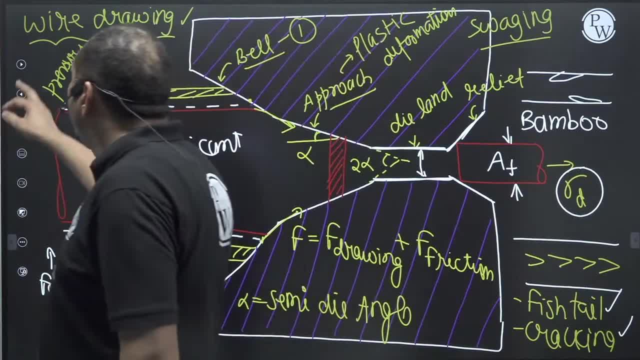 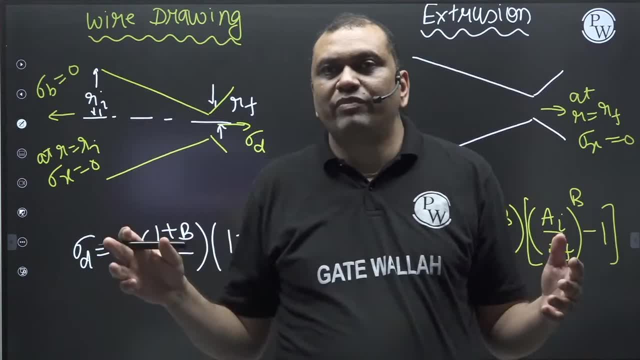 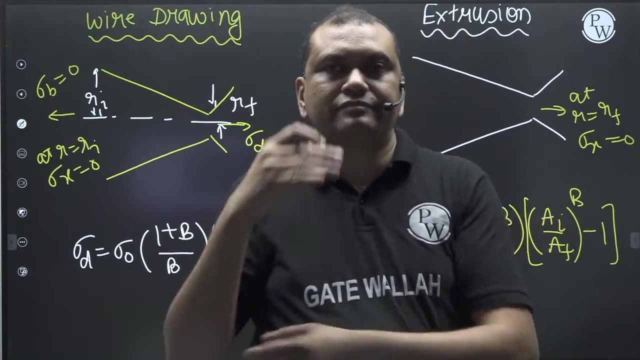 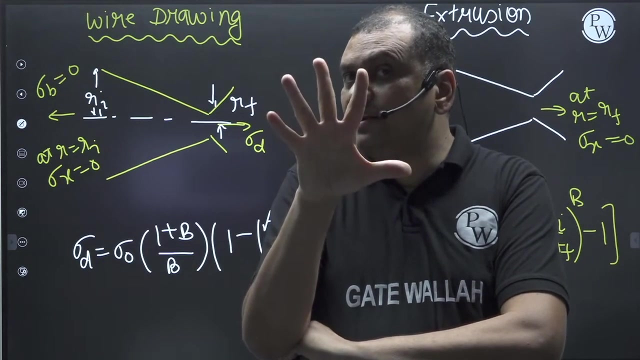 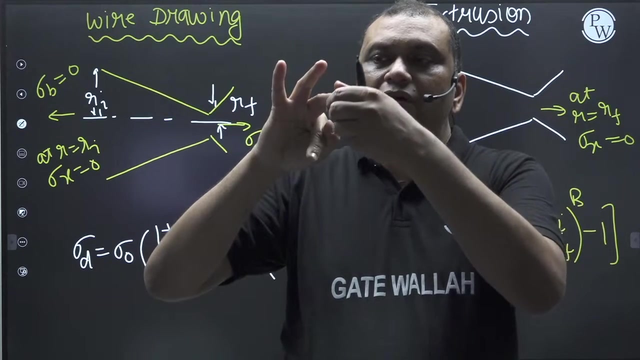 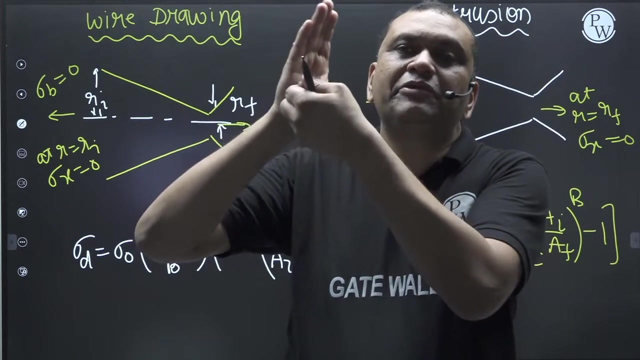 We are talking about a wide range. Listen to me for two minutes. In metal forming, there are five methods to calculate the drawing force: Upper bound theorem, lower bound theorem, slab analysis, slip line field theory and Johnson's equations. Your gate's slab is made of metal. 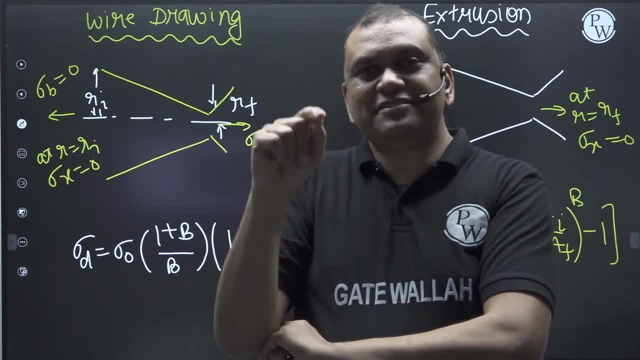 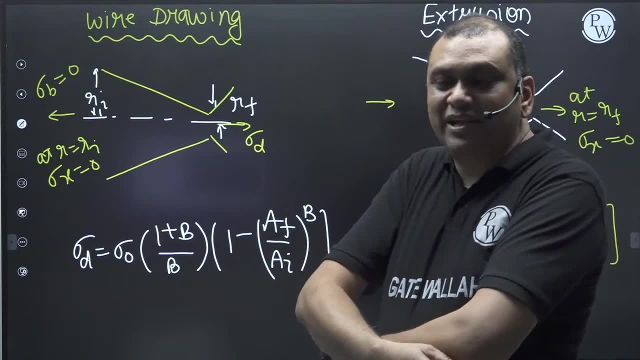 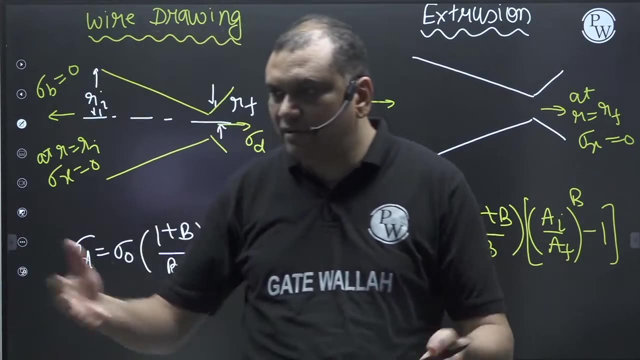 It is made of metal. It has only slab analysis and Johnson's equations. There is nothing else, Only slab analysis and Johnson's equations. There is nothing else. So don't worry later, Because you must have seen that some teachers or those who run test series, 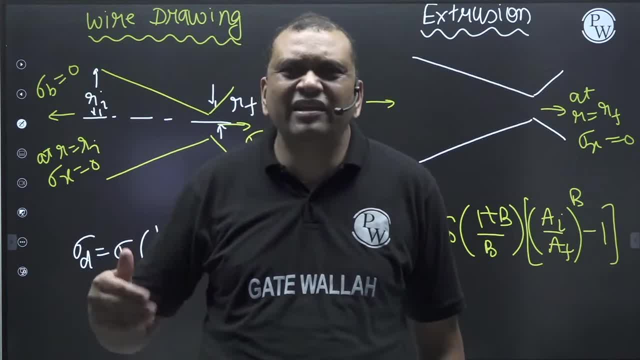 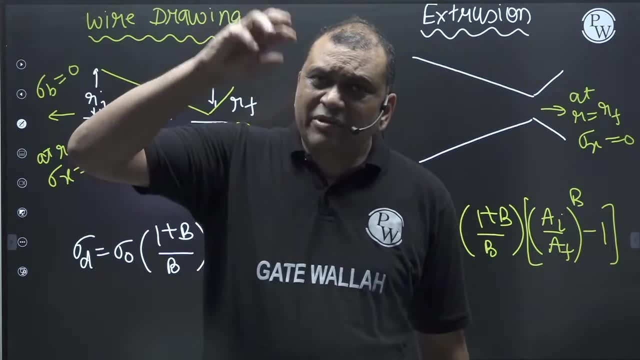 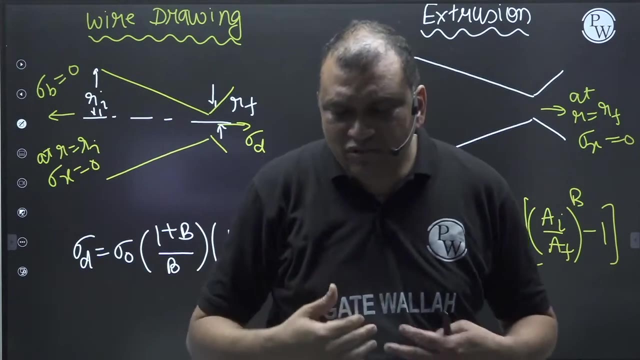 they have a habit of giving new equations. This equation is not in the course. The equation slab analysis is Johnson's equation. Look at the syllabus of P&I. It is clearly mentioned in that course. So I am telling you that in forming, follow what I suggest. 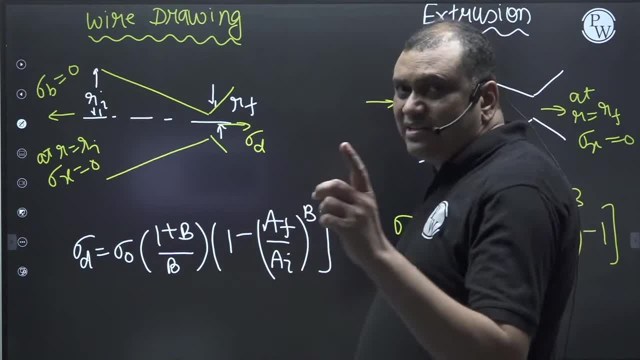 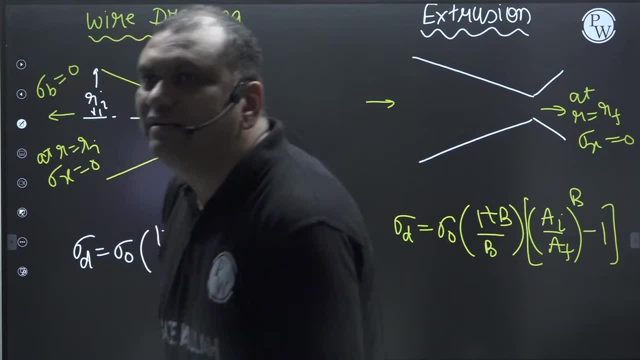 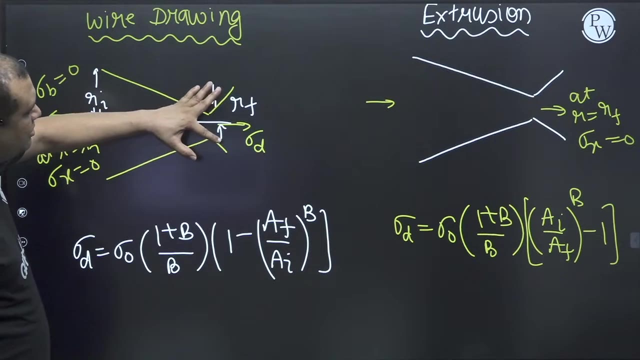 Otherwise you will have a problem. So I will not do slab analysis in crash course. What is diland? What is diland? See Here, suddenly there is an increase So this portion will break right. If it breaks, the die will get spoilt quickly. 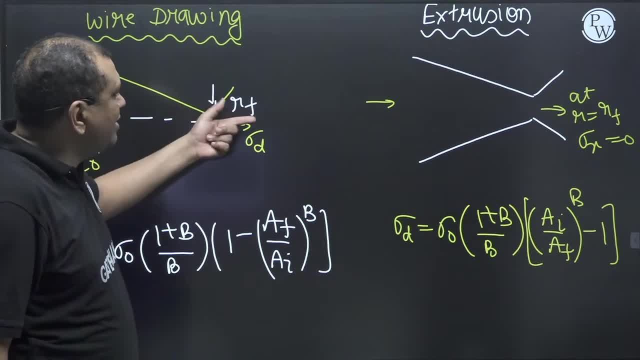 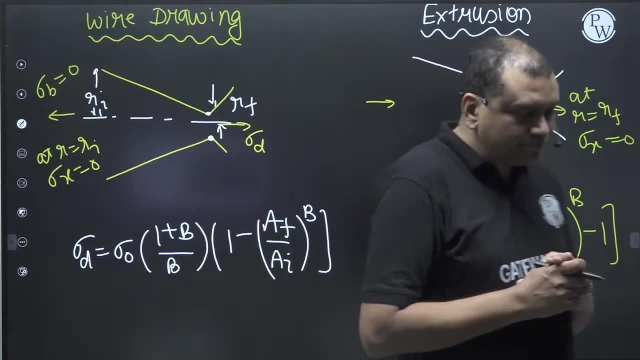 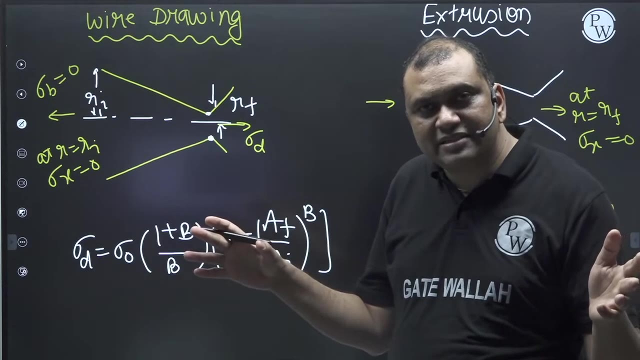 Die will get spoilt quickly. That is why we provide some diland, So that this portion remains stable. Okay, The questions that come in the gate. Very simple questions come from slab analysis. The questions that come in the gate from slab analysis: 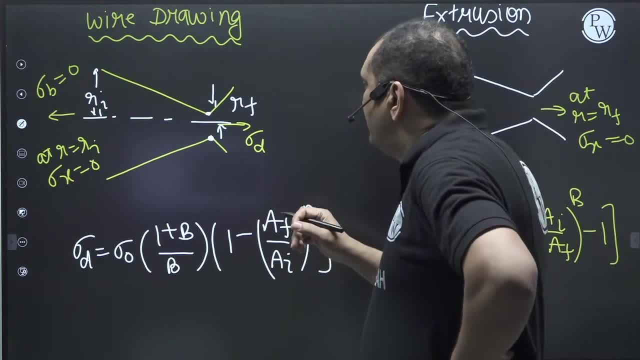 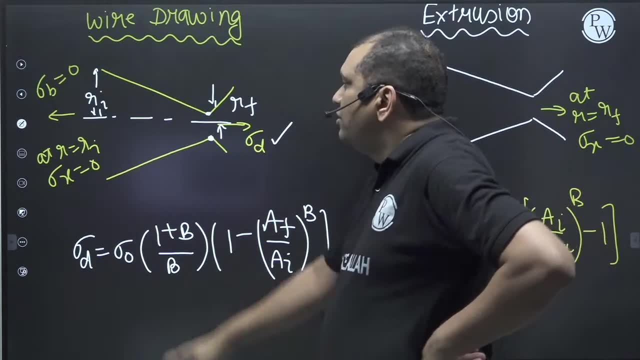 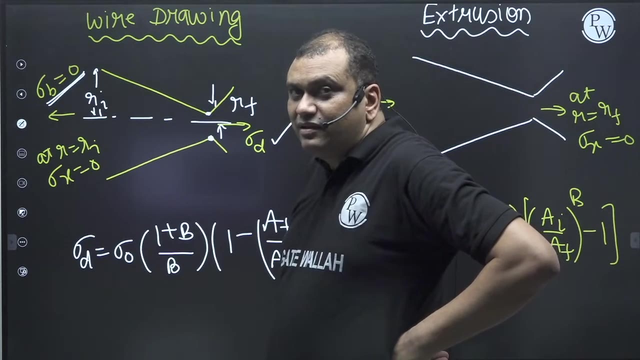 Very simple questions. come In wire drawing with the sigma D pressure you are pulling and back pull is 0.. What was the purpose of back pull? to keep the wire straight. If it is 0, then our equation A comes. Sigma D equals to sigma 0. 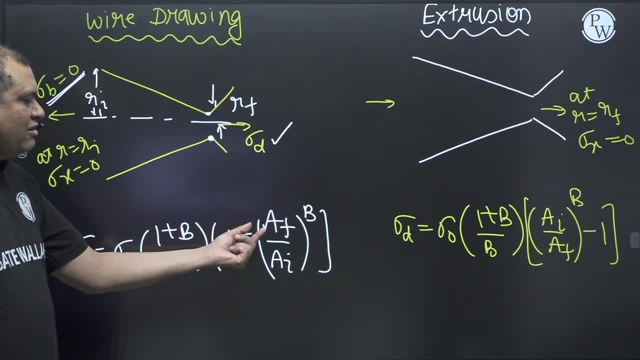 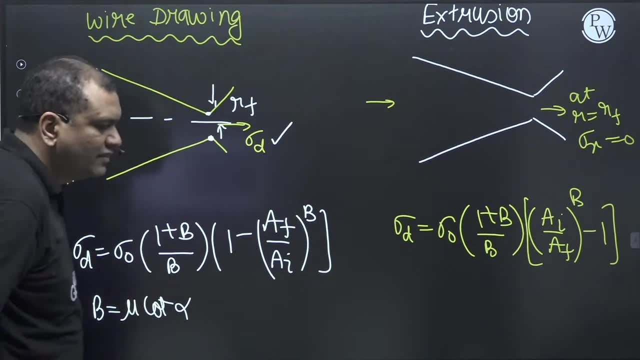 1 plus B by V. 1 minus AF means outside Outgoing area. Incoming area B. What is B? It is a mu cot alpha. We are not going to prove this because it is our crash course. We will go into detail in regular course. 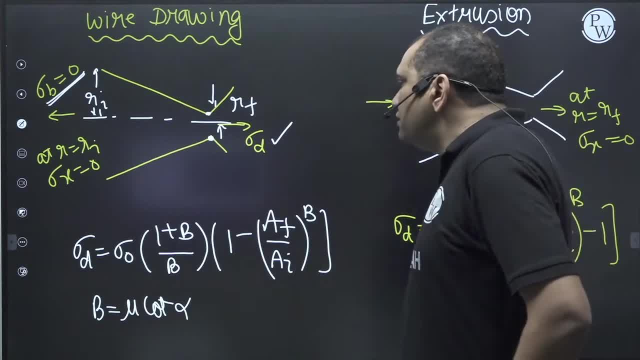 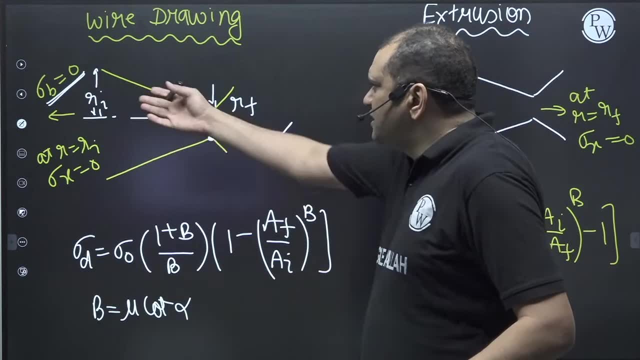 His question came last year. His question came to me last year also. Okay, So because we will put sigma B, then here will be 1 term of sigma B. Look carefully, And here is the equation: Sigma B is 0. 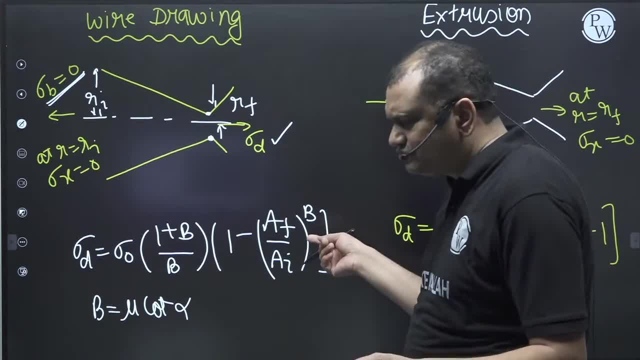 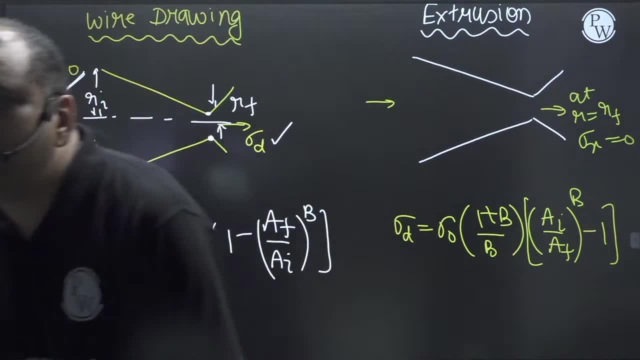 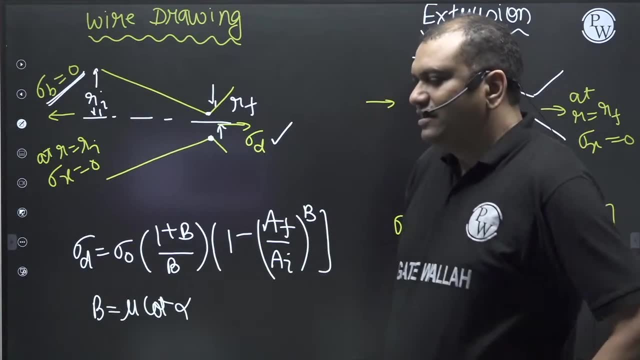 Sigma B is 1.. It is 1.. We will still have a number of assignments which will come in terms of theaults. Oh, And here sigma B going to choose sigma S, And again繼續. Beispiel B will come. 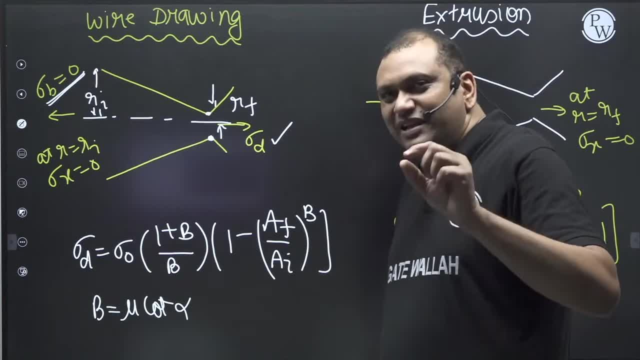 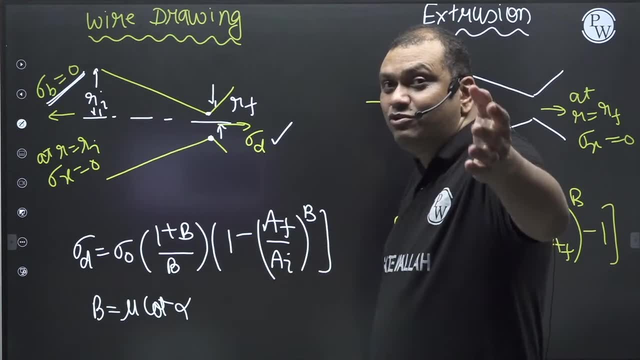 The third class here, where sigma abd will be letting us choose sigma square. As you see, sigma is volume 1.. omega 0 before me and sigma is a quantity, And the line between sigma and omega will look like this: 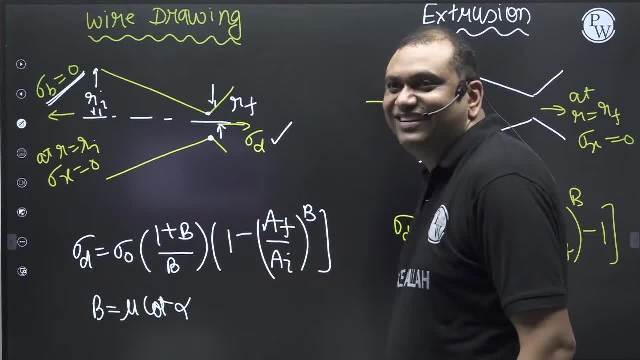 The line between sigma and omega. So this isina is linear And manga is the straight line of sigma. If through diameter gives a range, then this line would not beuming. sab log boat pe dekhenge 2 minute ke liye. mein kya gaya raha hu. 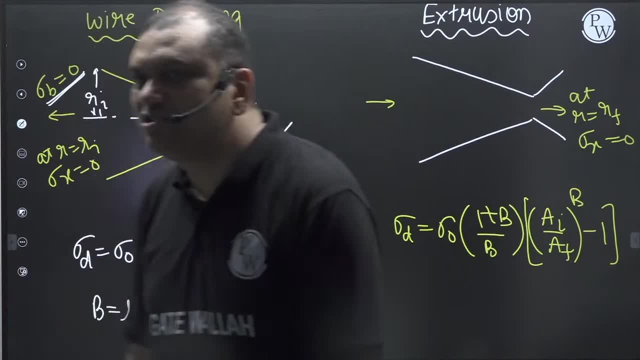 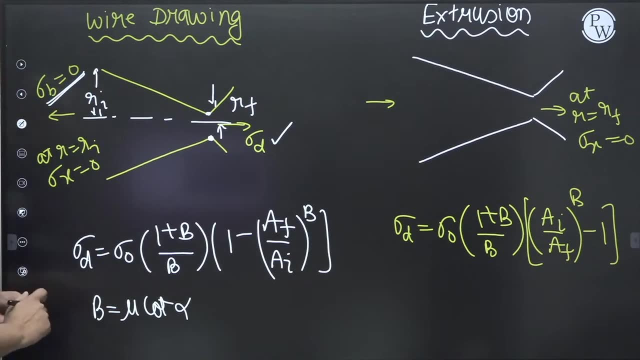 us time equation diya tha par aapko malum toh hona chahi kaise use karna hai 2 minute ke liye. sab log boat pe dekhenge. dekho, suno, ye equation kaise aayi, ye equation kaise aayi. 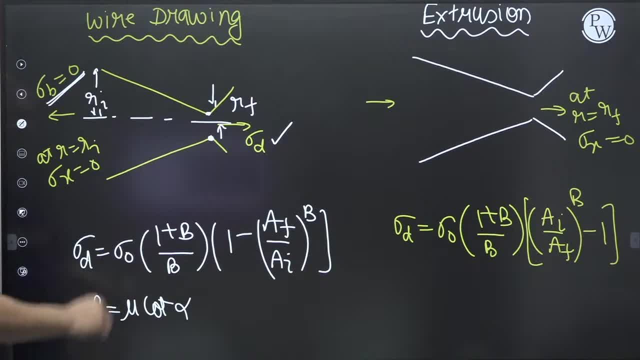 slab analysis: mein at r is equals to ri. agar sigma x equals to 0, rakhunga mein toh ye equation aajaygi. ye hai aapka y drawing yaane. aapni boundary condition: jo thi. jo boundary condition thi wo entry pe thi. 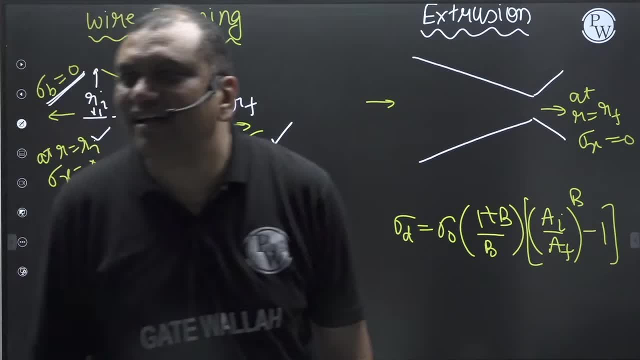 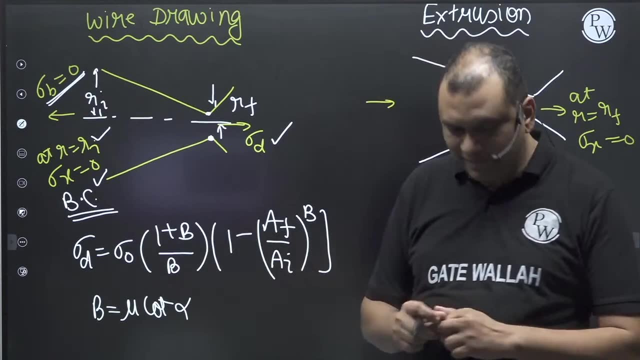 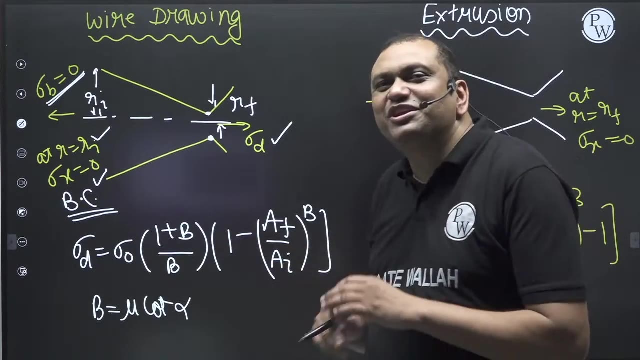 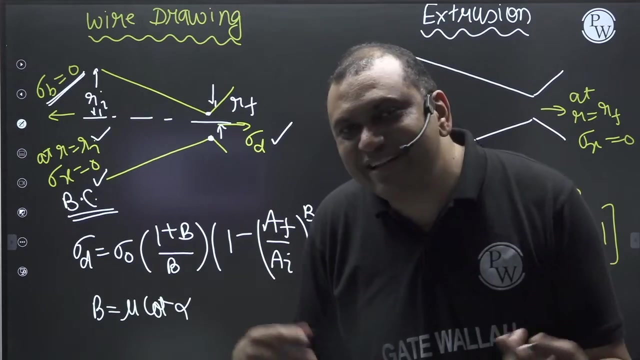 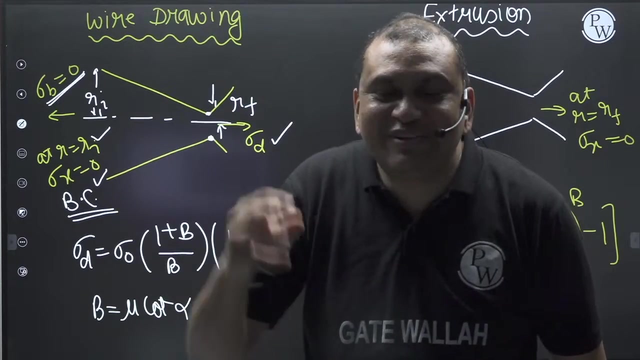 ya, ye mu hai mu mu nahi hai mu mu is a coefficient of friction. dekho kuch students par laya: the mu is a coefficient of friction. me ye equation to gate mein diya hua tha equation, ye equation de raki thi 2020 ke forging question mein kya karege aap? 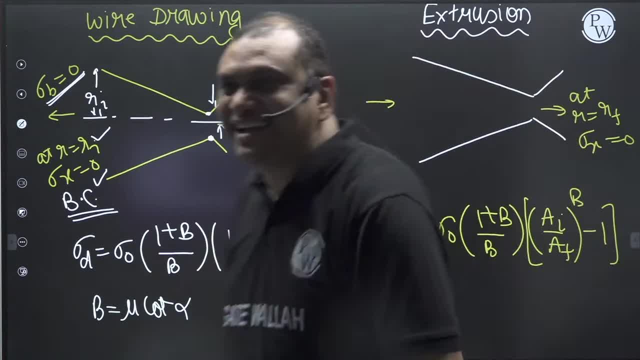 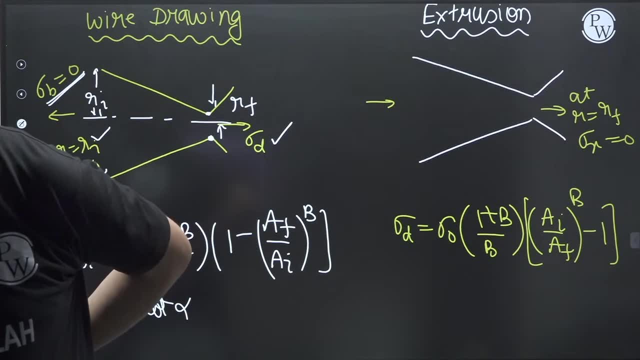 usme toh kuch bhi nahi de raka tha, aapko diagram de raka tha. ek billet hai forged kiya, batao stress kya hogi. Yeah, correct, Very good, Five questions have come, sir. 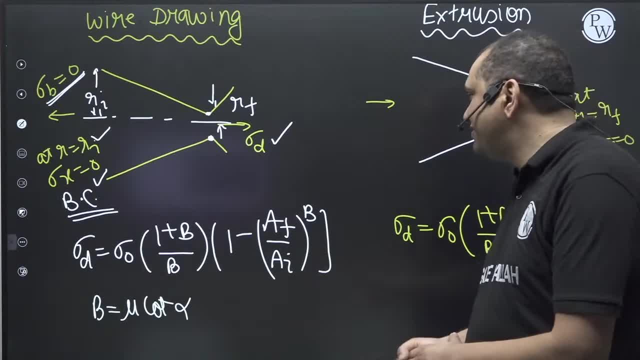 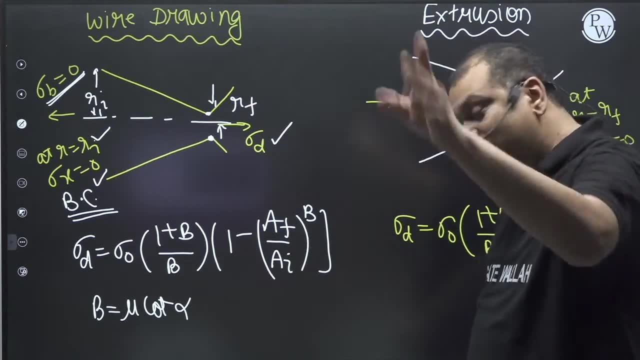 Very good, Aditya Kumar. Very good, very good. I will tell you again, because I was about to give you the answer to the question. Listen to it again. Listen to it again In wire drawing: I am pulling from the front. 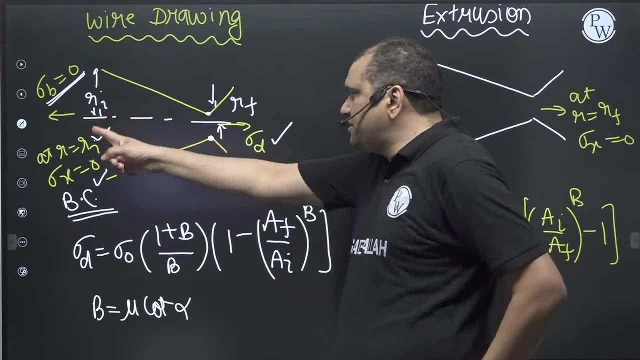 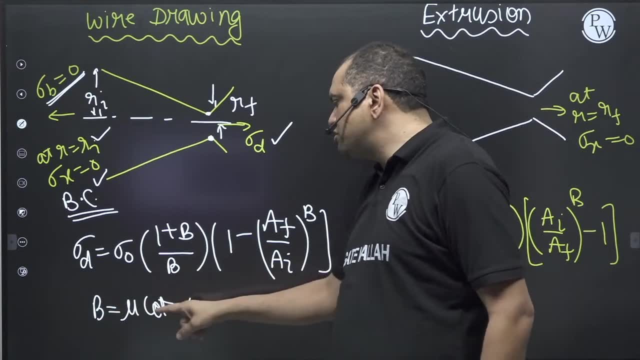 I have to take out sigma d. So the boundary condition was at the entry. What was the boundary condition At? r equals to ri. sigma x equals to 0.. So this equation has come. The b is b equals to mu squared alpha. 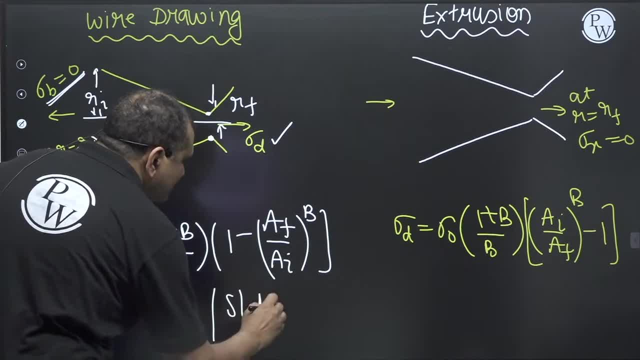 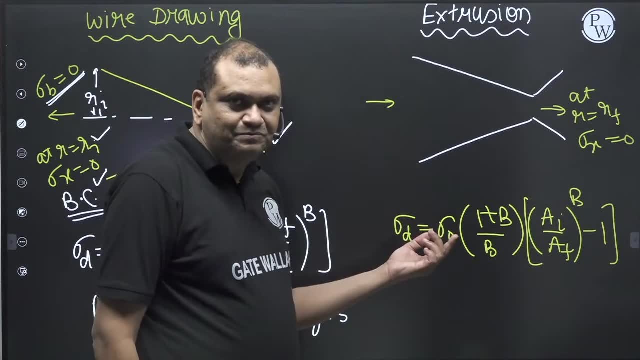 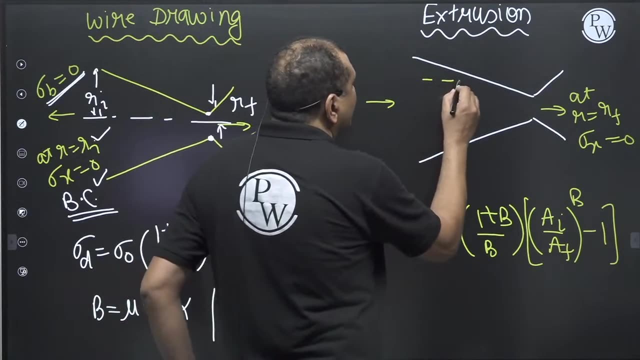 This is your slab analysis. This is slab analysis, But the extrusion is exactly the opposite. It is the same die: Everything is the same. Like this is also the same die Semi-diangles: Everything is the same, But the boundary condition is the opposite. 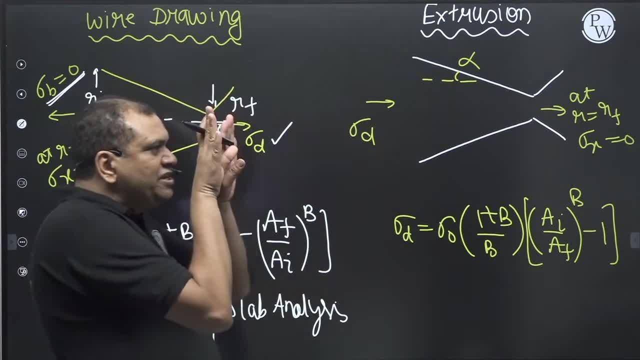 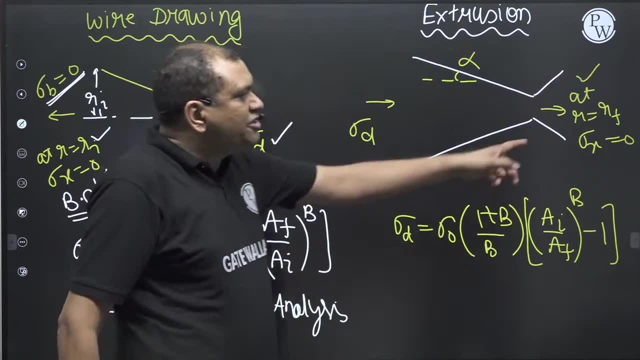 What we have to do here is to extrude. we have to press from the back. We have to press from the back. Our boundary condition is at the exit, At r equals to rf, sigma equals to sigma 0.. So what will happen? 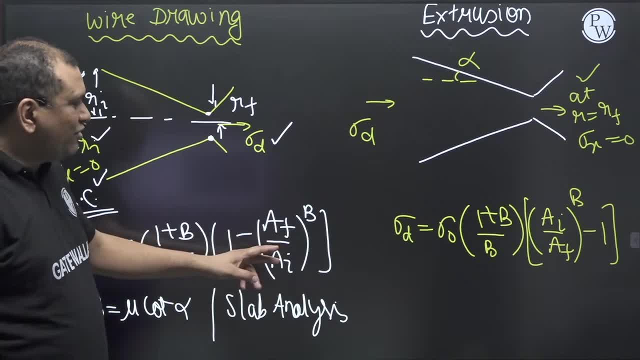 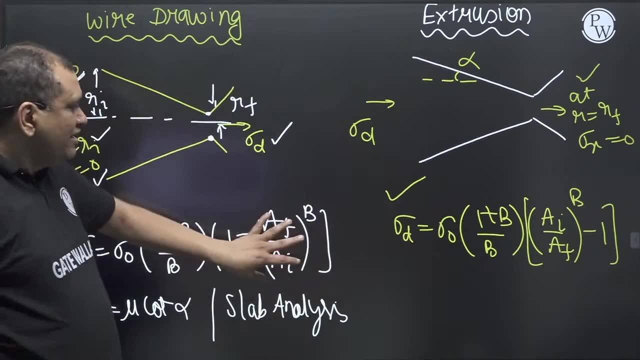 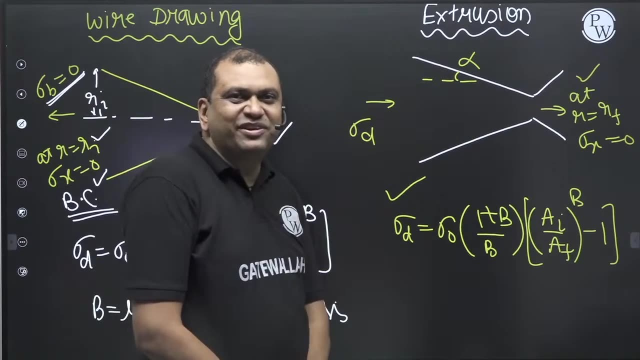 This thing will be the opposite And to make this factor positive, keep it in front: Same, Exactly same. This factor is the opposite. Why is it the opposite? Because our boundary condition was here at the entry and shifted there at the exit. 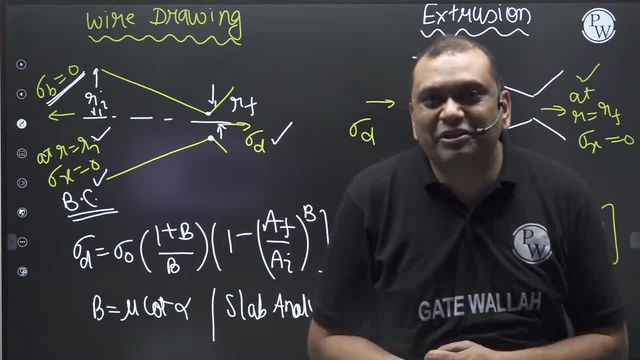 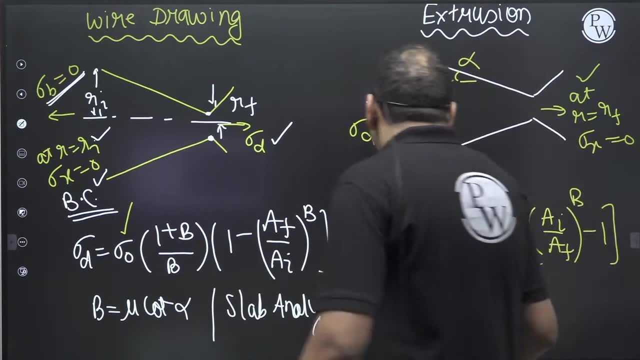 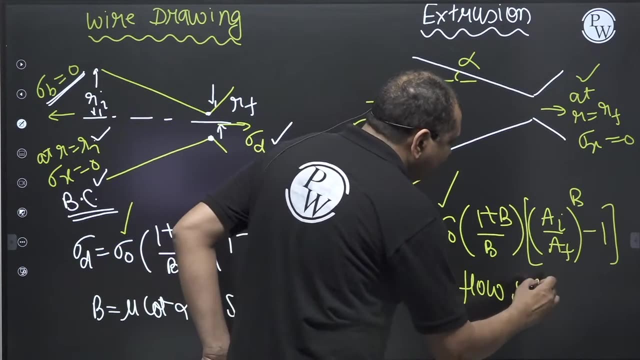 So the same equation will be valid for extrusion. The same equation will be valid for extrusion, And you are seeing sigma 0, right, Sigma 0.. Sigma 0 is called average flow stress and mean flow stress. Sigma 0 is called average flow stress and mean flow stress. 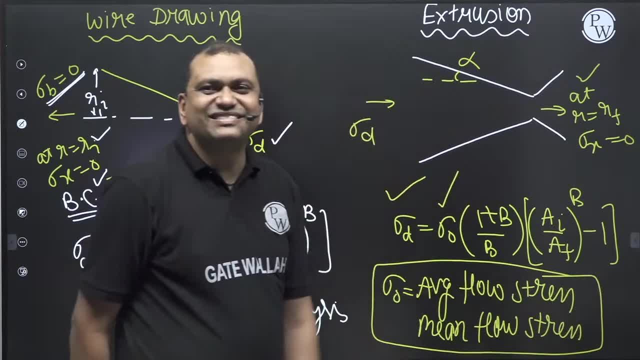 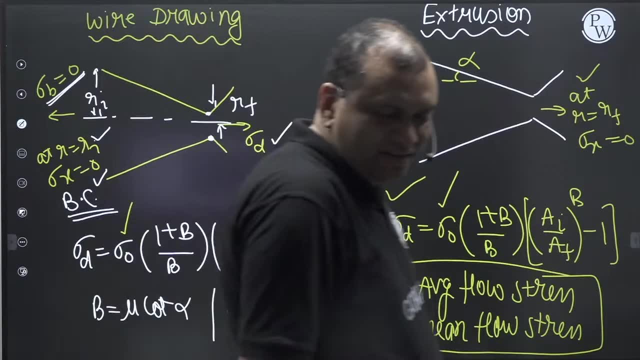 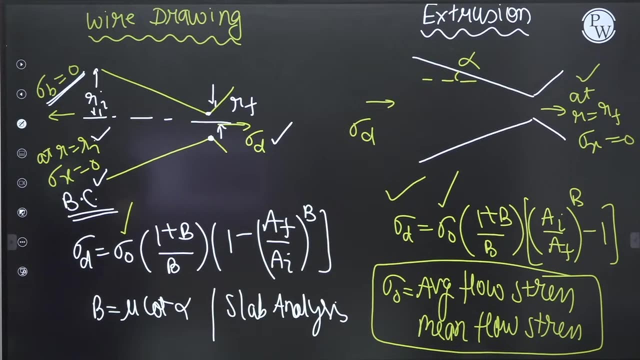 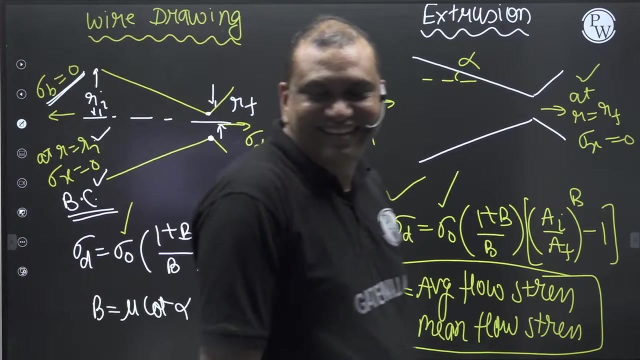 Average flow stress and mean flow stress. Okay, Average flow stress and mean flow stress. Kne œ Go watchalt. HR class material science lecture again. Fine, Very good, Utkarsh, Very good, Be happy, I taught you. I think I'm talking to a sizing. I think I taught you single. 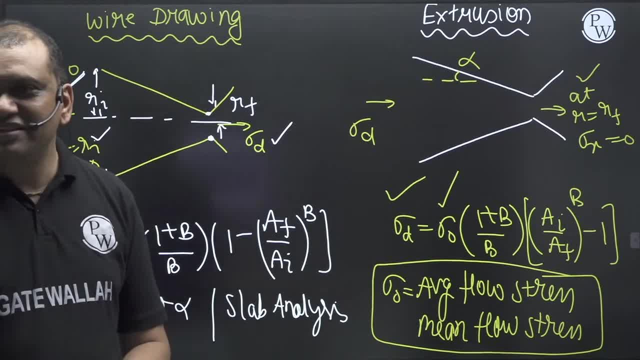 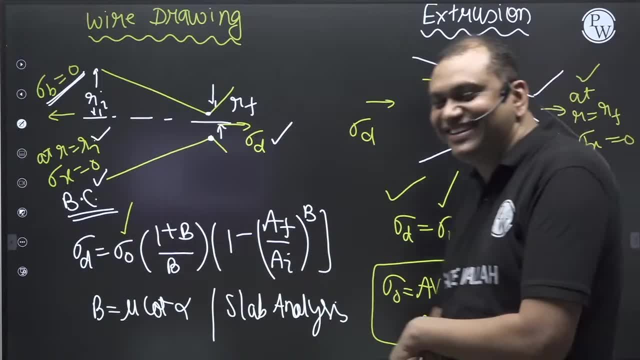 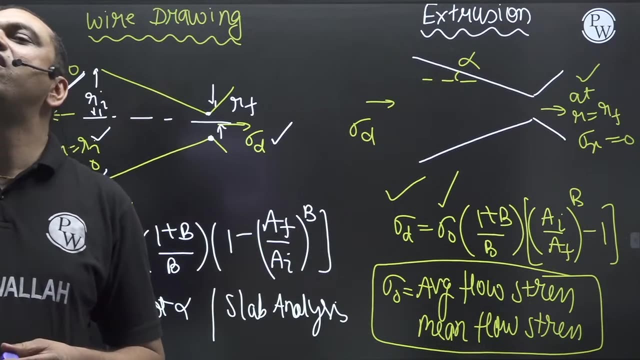 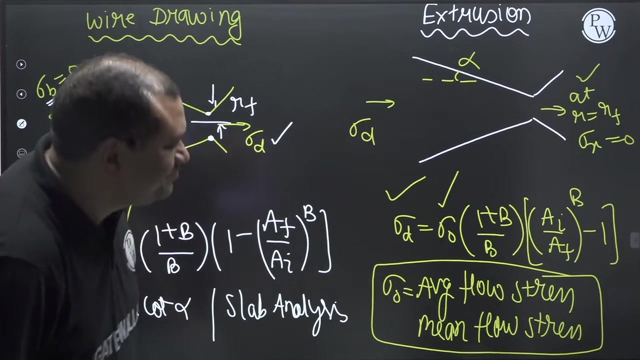 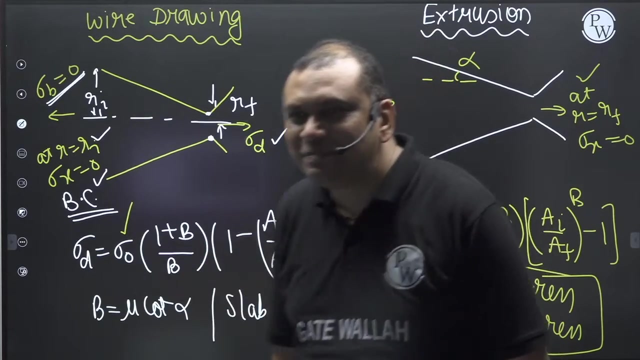 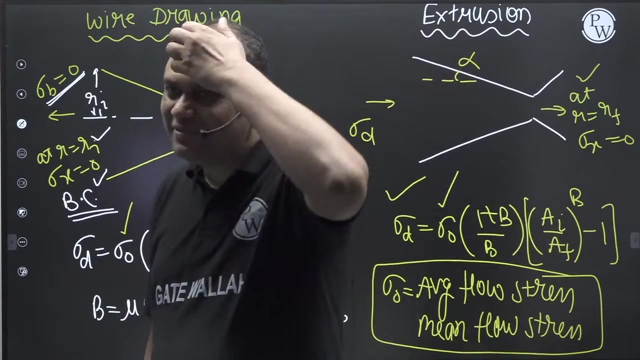 point, cutting tool, that one, I think I I was there. okay. so metal forum, Dora, but I have a crash course, a high full. yeah, I, I think if I see your face, I will recognize, because I never forget my students. if I see you a baby face-to-face, I will definitely recognize you, okay, yeah. 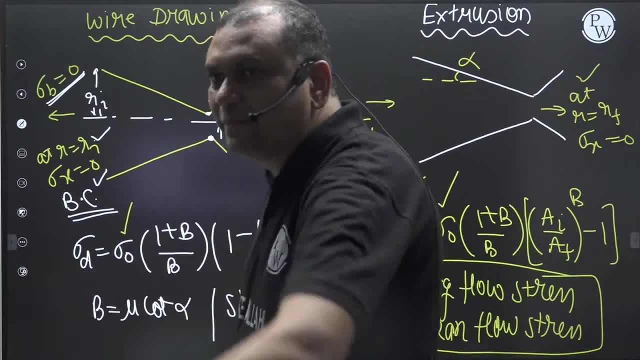 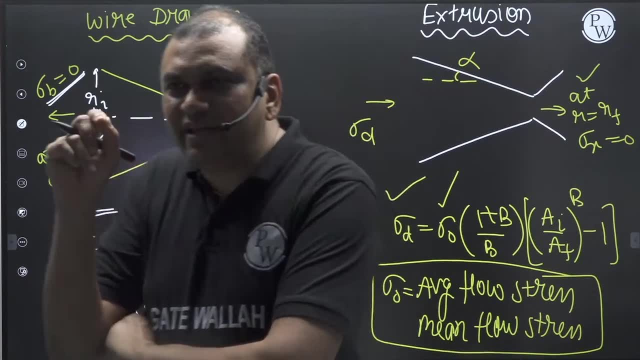 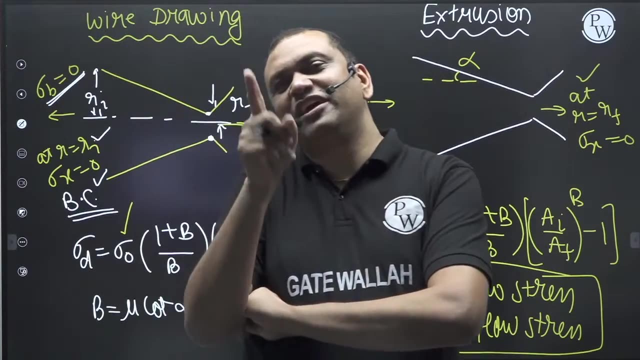 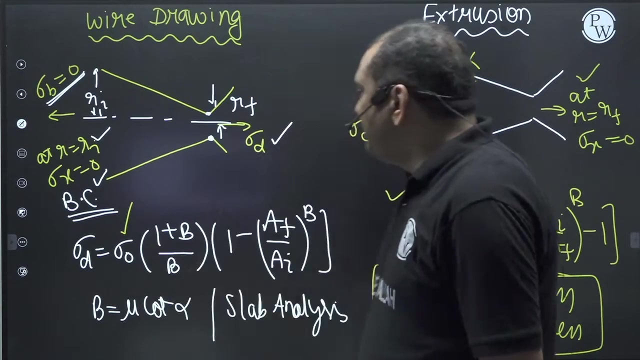 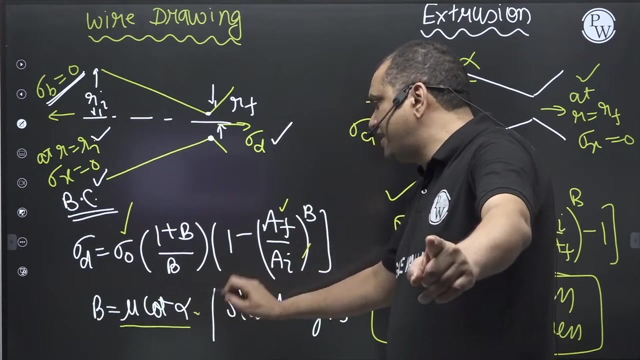 ha. is he a bar about kind of Allah who Vinay may see a bar about kind of Allah. who exam man? exam man up. come in for a stress or average flow stress, Nikala parega. take Anna Bucky Joe data there. Akai finally area, her initial area, her coefficient of friction or semi-diagonal, semi-diagonal. 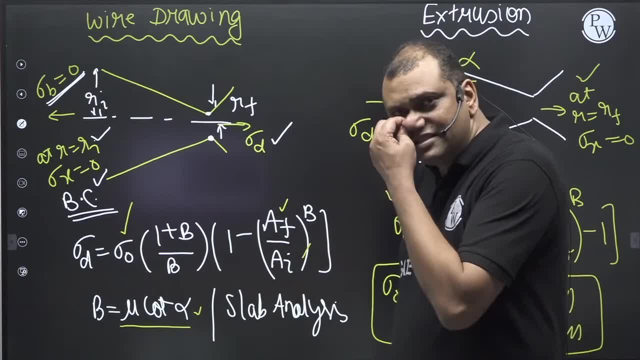 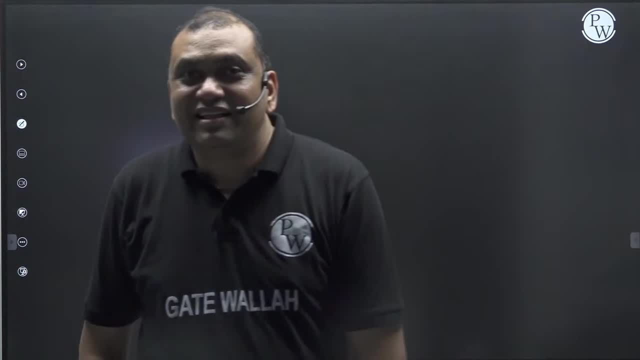 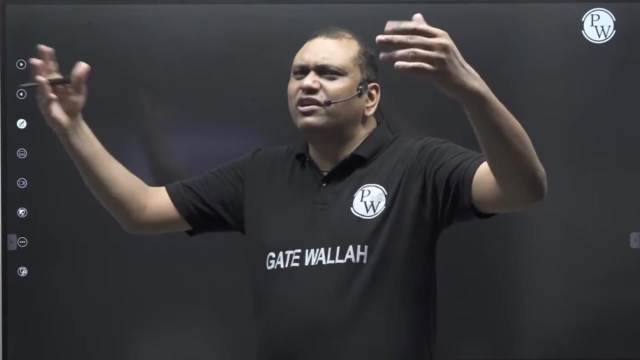 say be Nikolai got a Bacha bar Sigma, not car, Sigma not case in a Caliga. I'm very bad, that's minute Kelly, I'm the answer. so huh BK, well, you say my bottom. a new quarter alpha, alpha, semi-diagonal a or new coefficient of friction between die. 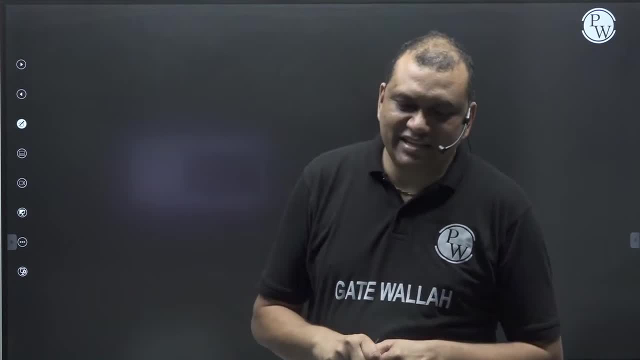 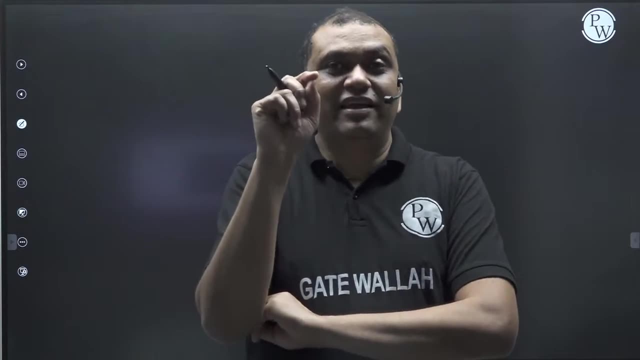 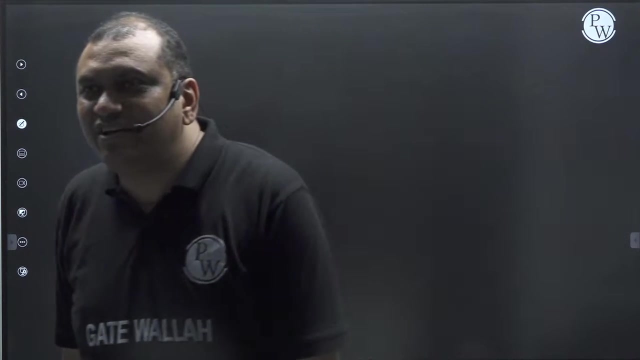 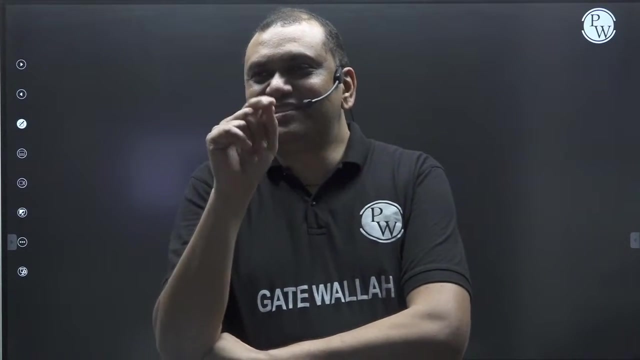 in the material. you know, I saw her. I said her: I'm you, PPR messable, the ISM, her cousin, her, yes, Sigma. not give a look at the Nikala in gay, based on, based on huh, based on the data given how to calculate Sigma, not. 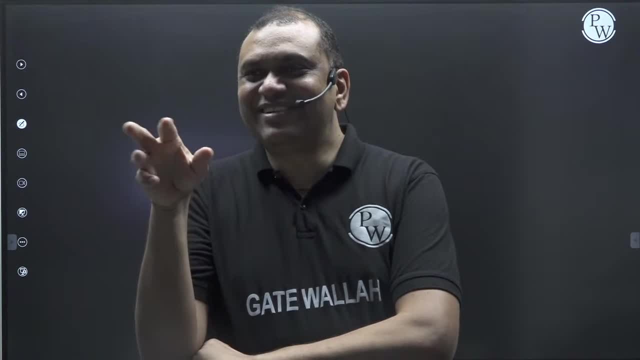 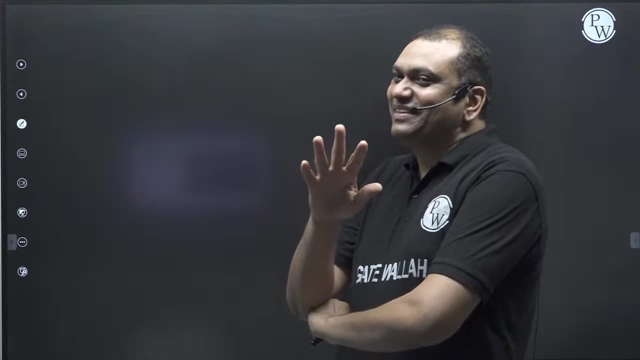 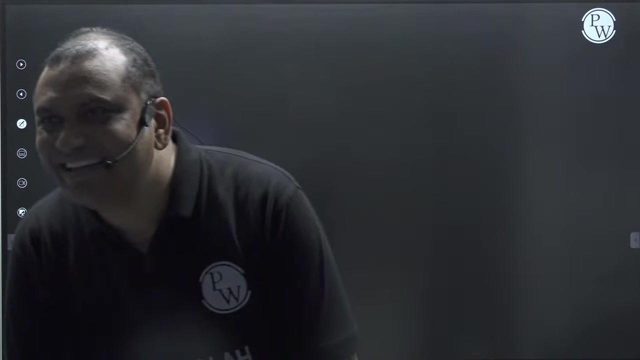 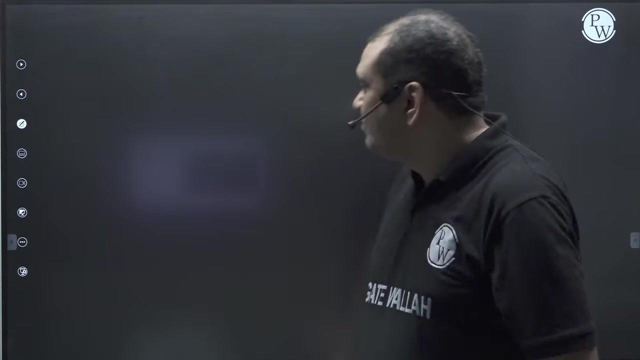 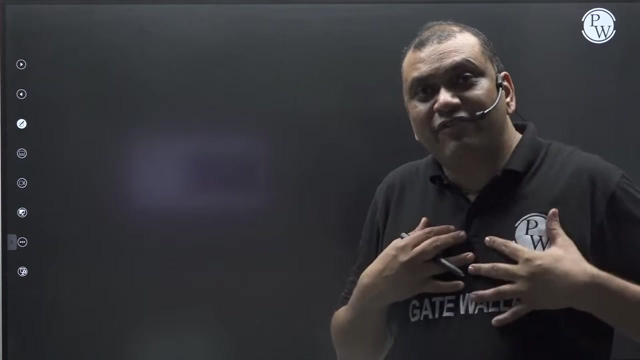 you know how to calculate Sigma, not based on the data given how to calculate Sigma, not given a one week on the given data, based on the given data. based on the given data, based on the given data, I have to find out what is sigma naught. 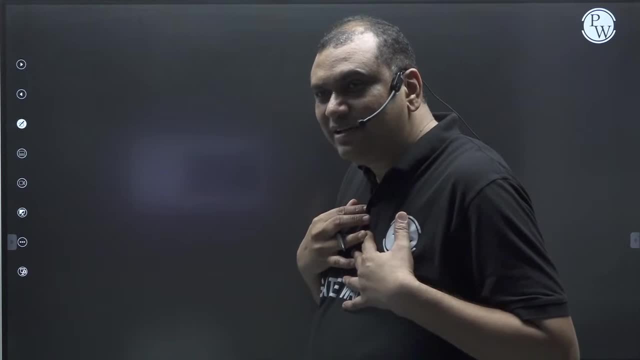 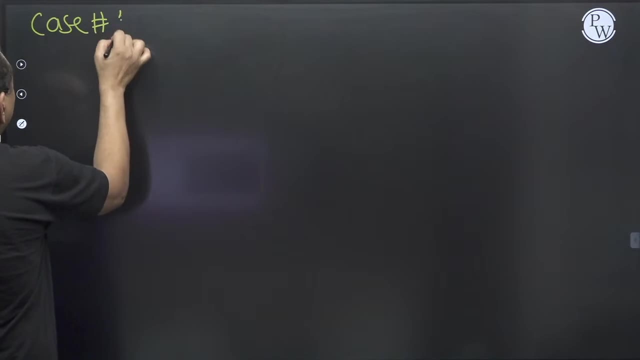 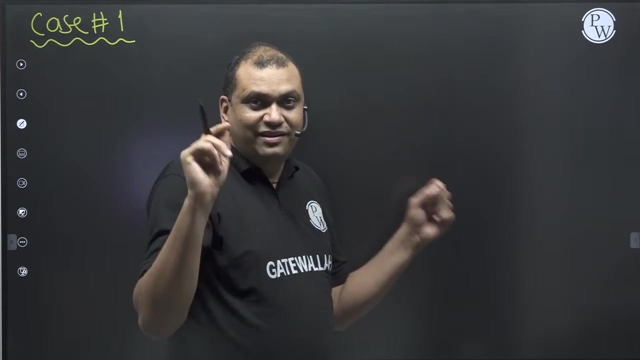 Okay, everyone is here, right? Everyone Question after 5 minutes: Case 1.. This is a very important section Because the calculation of all metal forming has been done on this 10 minute discussion. This 10 minute discussion has been done on this. 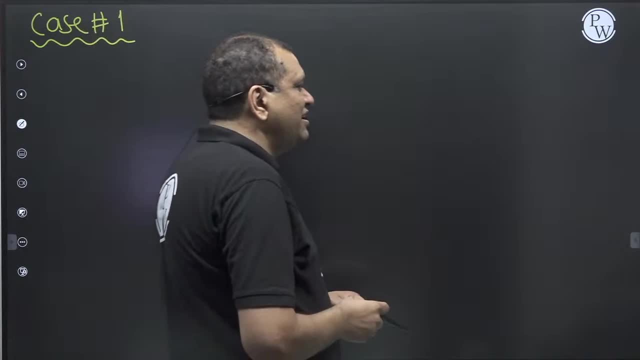 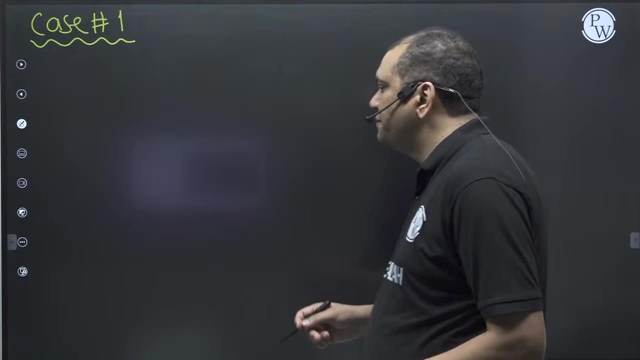 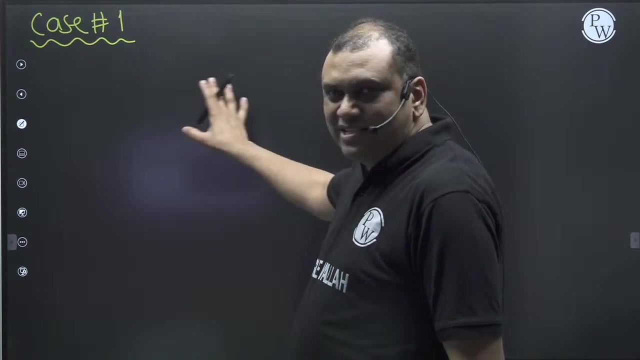 See for the notes. I have cleared everything in the mail. Send it again. If it doesn't come, send it again Tomorrow morning. I will do that. So the calculation of metal forming has been done. on this 10 minute discussion. 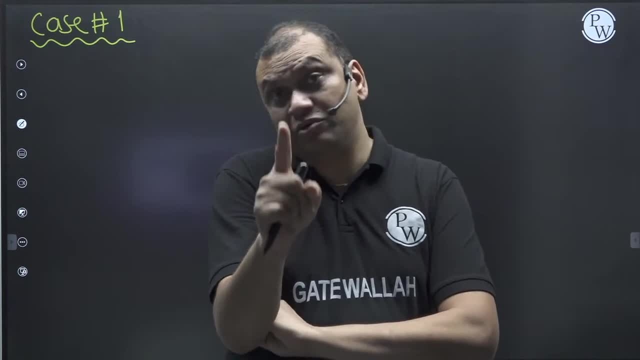 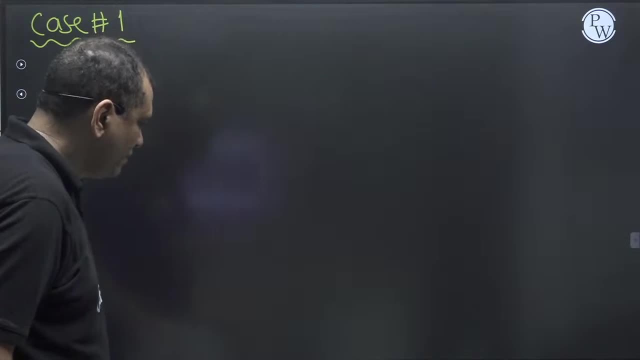 If in the question: listen carefully, please. There should not be any mistake here. I am going very slow. There should not be any mistake here. Listen carefully. This is the most important section in metal forming. If in the question you are only given a yield stand, 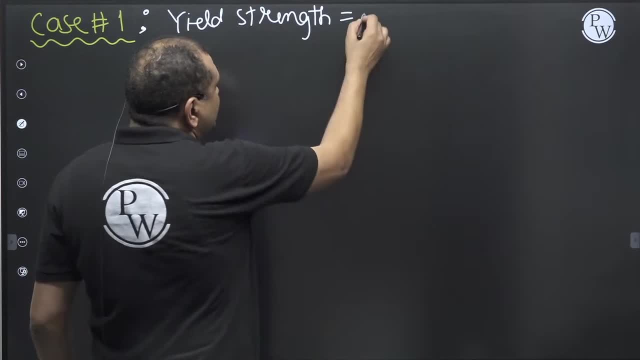 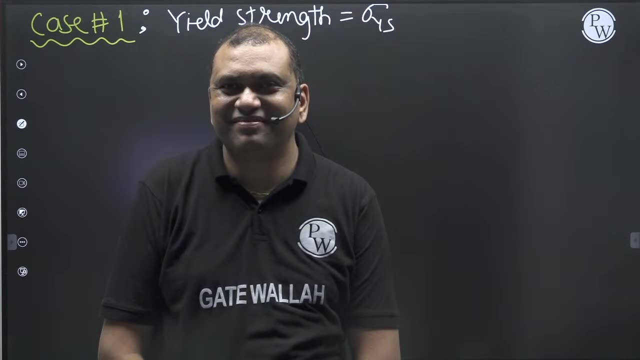 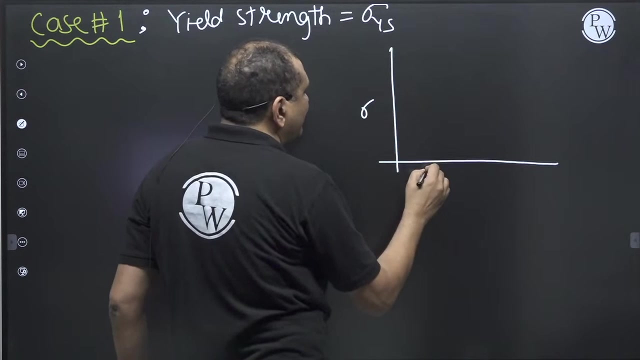 In the question you are only given a yield stand. In the question, you are only given a yield stand. This means this happened indirectly. Tell me what the question is saying to you Exactly. What the question is indirectly saying is that 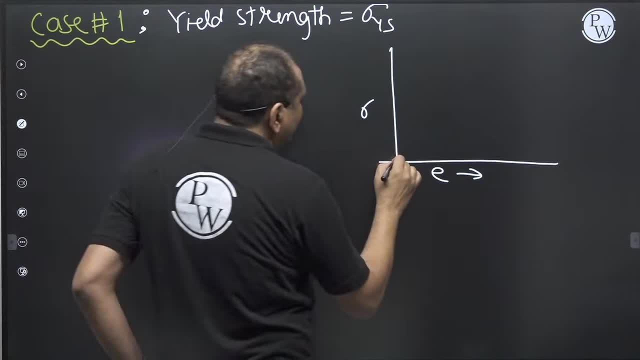 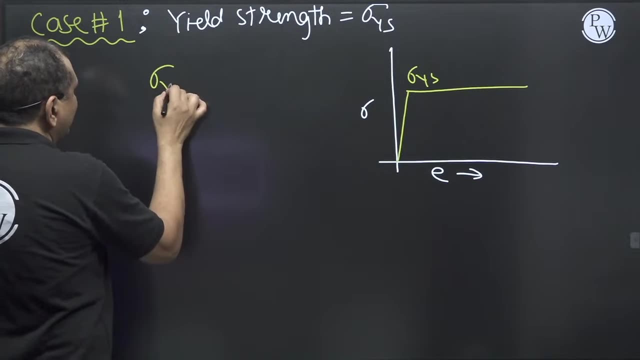 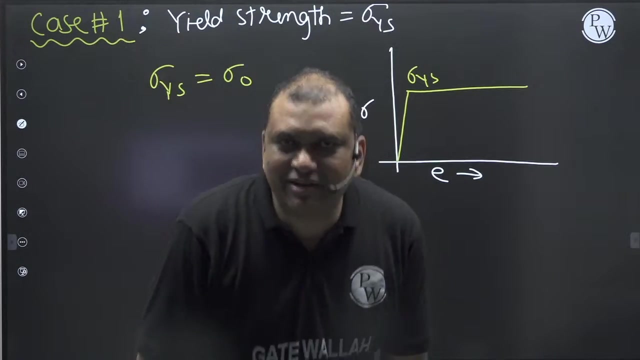 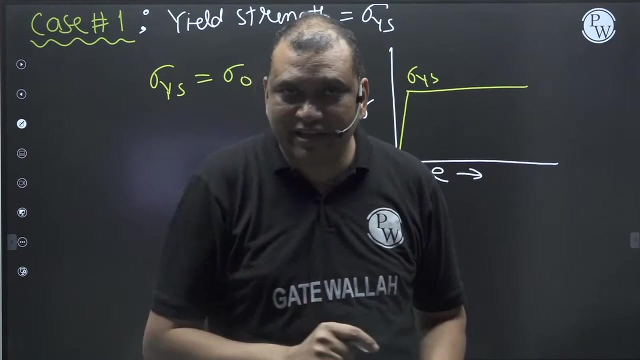 material is following: elastic, perfectly plastic. So take the yield strength as sigma naught and do the calculation. Take yield strength as sigma naught and do the calculation. You are very careful what I am saying right now. You are very careful what I am saying. 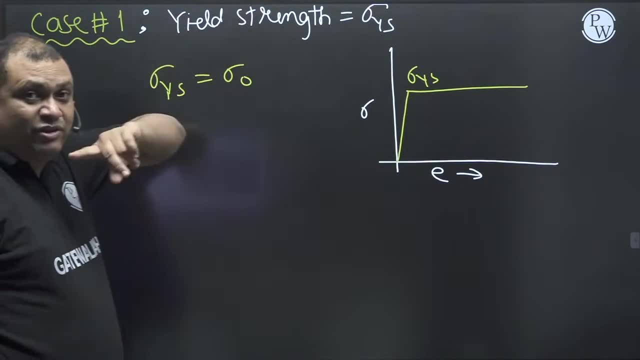 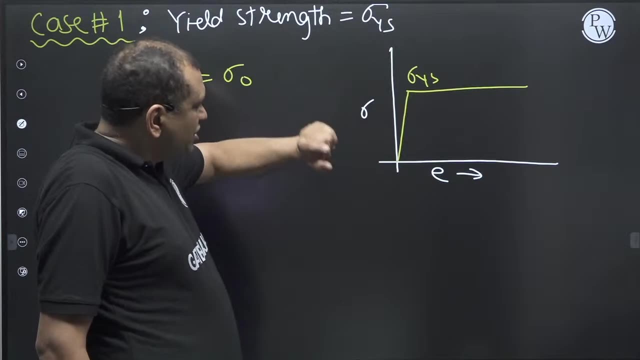 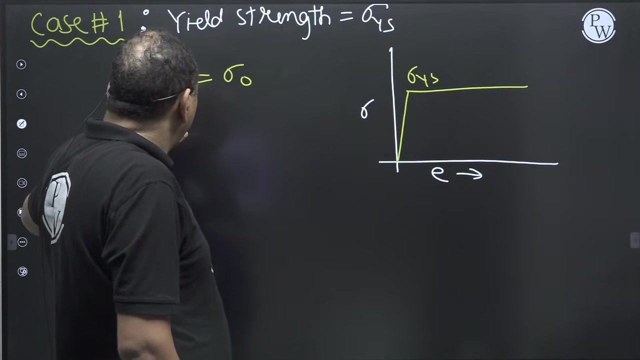 You are very careful what I am saying. If yield strength is given and no one has given any data of the material, So it means that the question is saying: material is elastic, perfectly plastic. So do one thing: take the yield strength as sigma naught, or 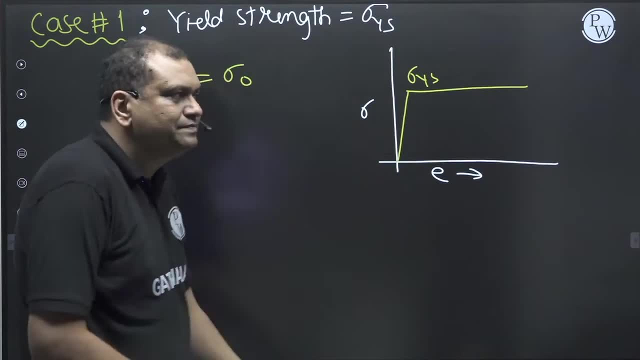 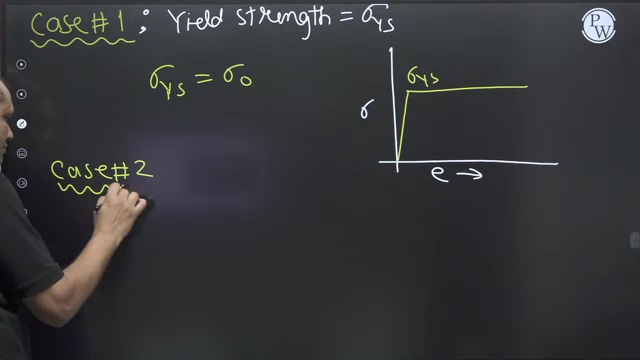 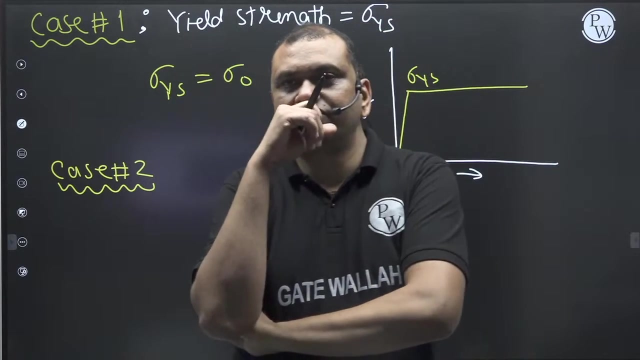 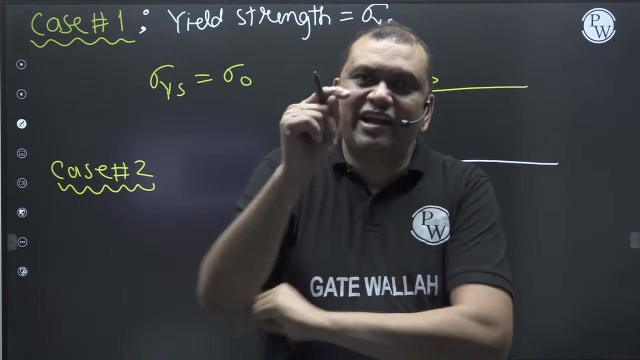 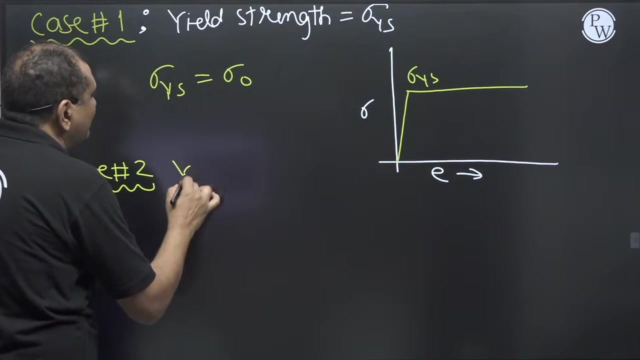 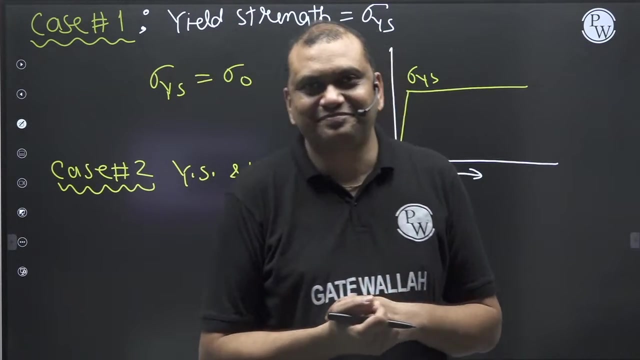 put the sigma naught in our equation and go ahead with the answer, Case 2.. Case 2. Agar question mein yield strength and ultimate tensile strength de rahi hai aapko? Agar question mein Yield strength and ultimate tensile strength de rahi hai aapko? Agar question mein: 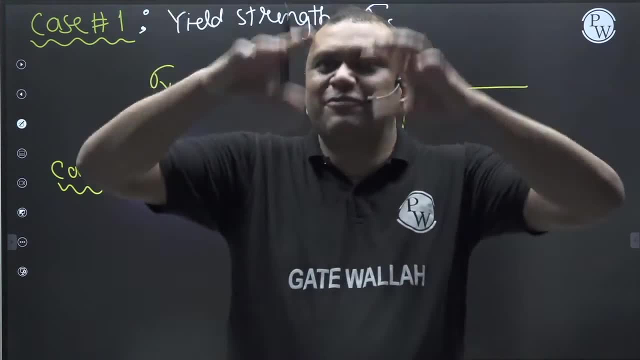 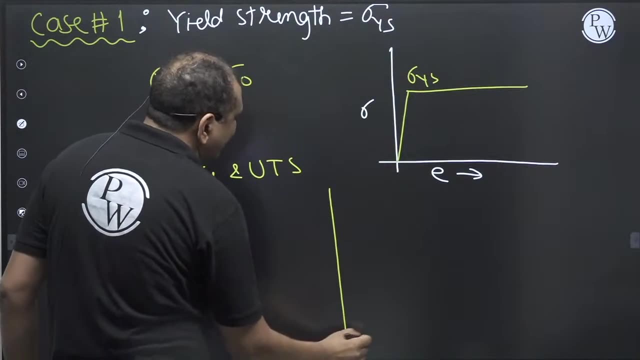 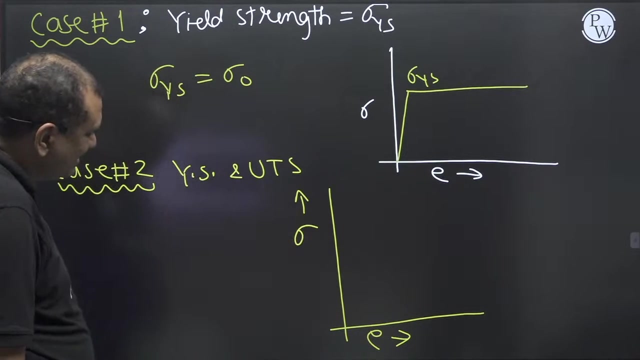 Aur koi data nahi de rahi hai. Aapko sirf yield strength aur ultimate tensile strength de rahi hai, aur koi data nahi de rahi hai. Iska matlab pata, kya hai Iska matlab? ye hai. 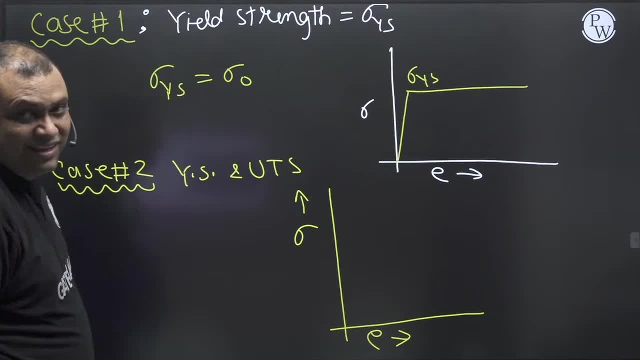 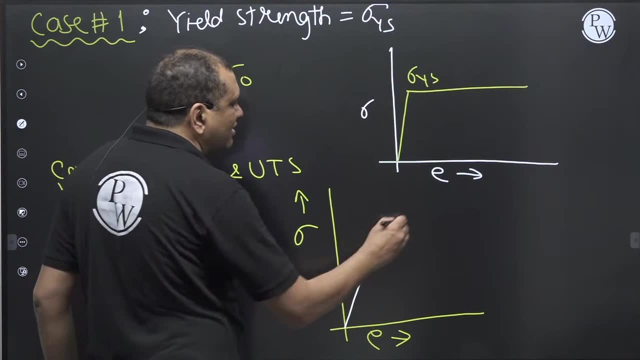 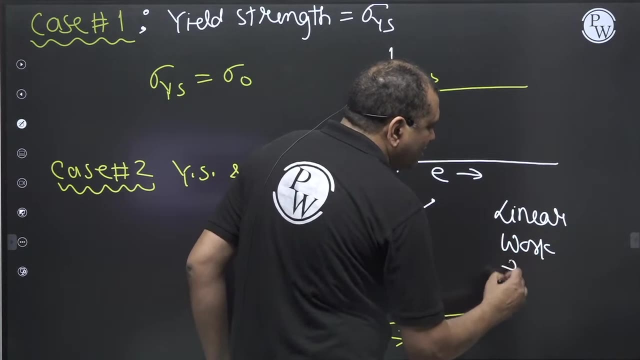 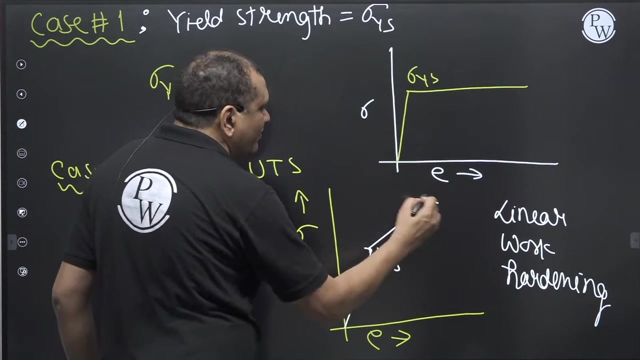 Iska matlab ye hai Isetti nahi meela icz ke question. indirect li aapse bor la hai. Material is elastic and linear work hardening, Linear Work hardening, Toh yeh aapka aaiga yield strength, Yeh aapka ultimate tensile strength And hamaara ji sigma naught ho ga hai. 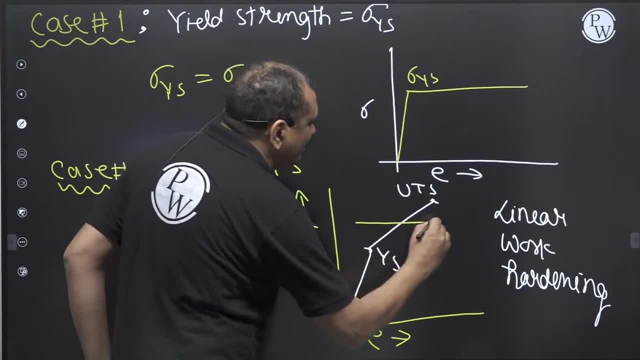 Nee石 is greens. Ini puppy, He has the heat. He has the heat Here. I am Satyaji hai, Satyaji hai, Subscribe, Subscribe, confirma hai, Satyaji hai. Your following content you can play on: 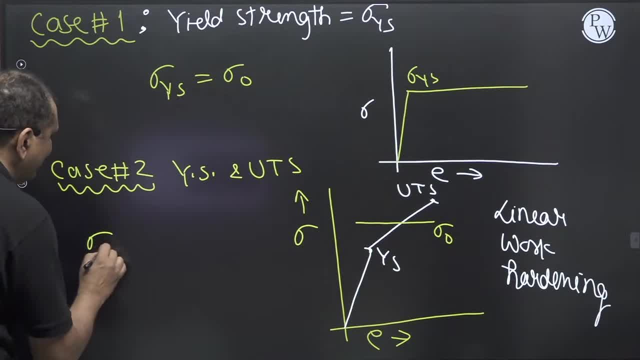 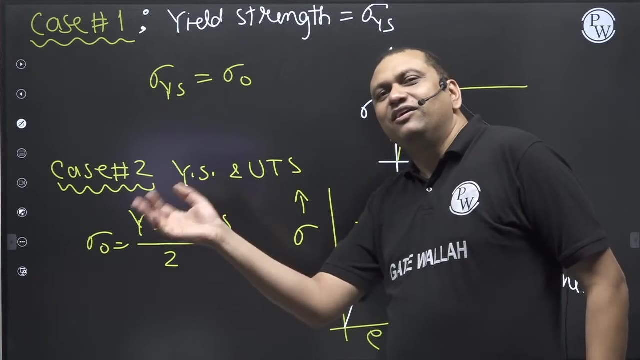 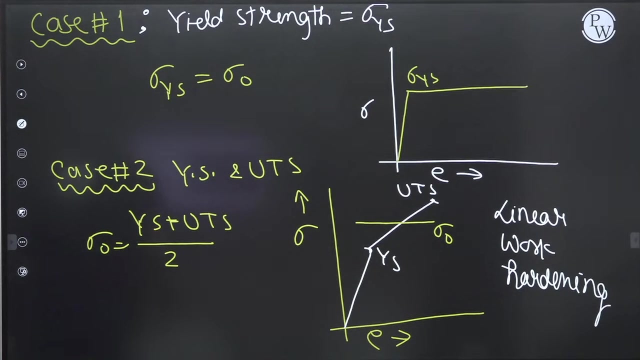 Please do watch and learn from here. Ya will come here. so Sigma naught will be nothing but YS plus UTS divided by 2. so if YS and UTS are given, then I will take this and will move my solution forward. arey brothers, are you all fine? 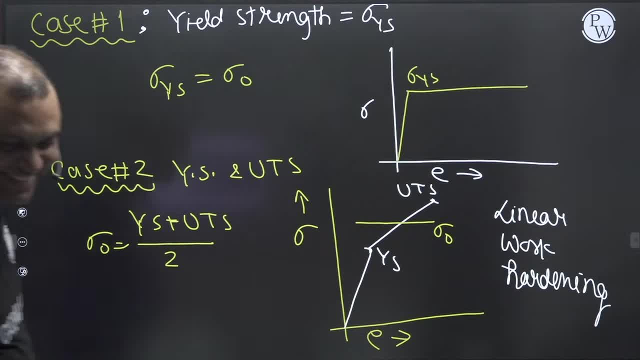 good. Arunach KD. ya, very good. ok, I think I must have taught you somewhere before, so do you understand what you have to do? and response to one question, brother, those people who are teaching are my friends or students, do you understand? 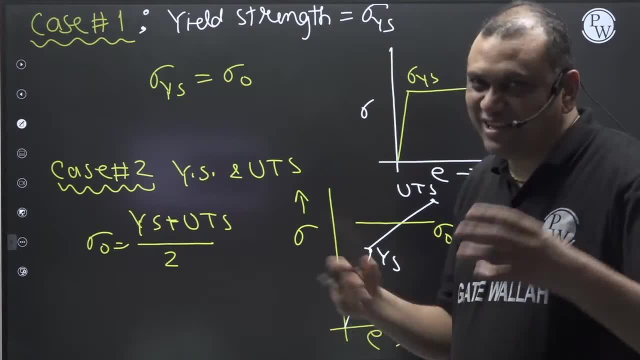 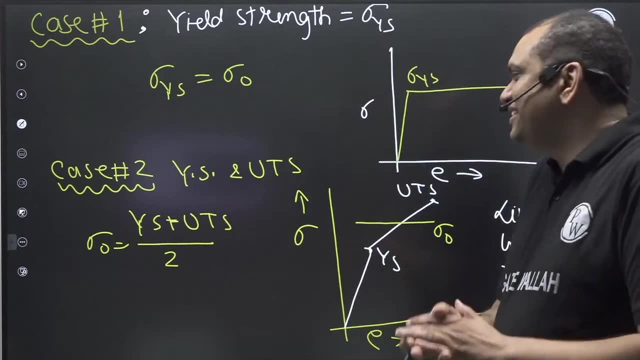 from where you have to study. my friends are very dear friends. I don't have any enmity with anyone. I consider everyone as my friend and some as very good friends. these are my students, so are you all teaching well? teacher is never bad. teacher is always correct. 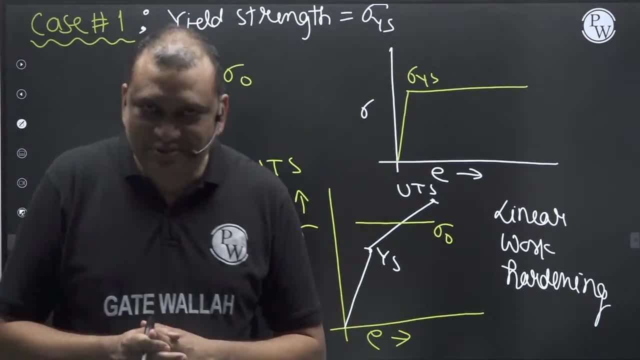 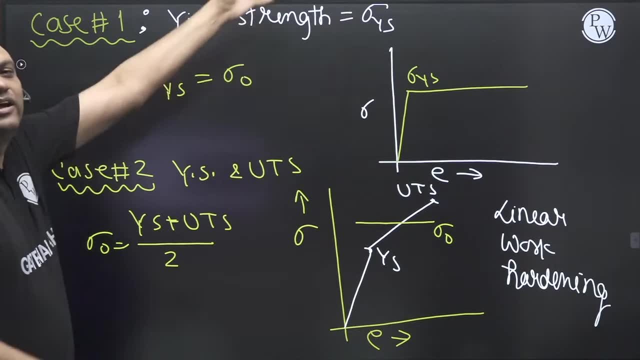 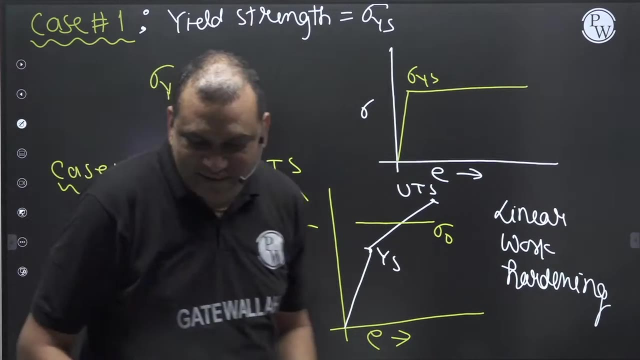 teacher is always a good person. student should think this ok. so if the yield is 10, if the yield is 10, then take this and move forward. if YS and UTS are given, then take Sigma naught and move forward. is this all right? 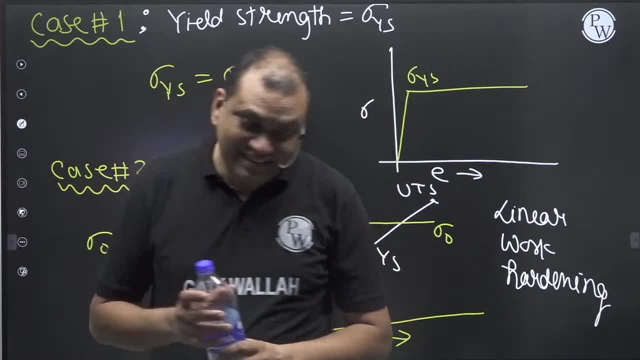 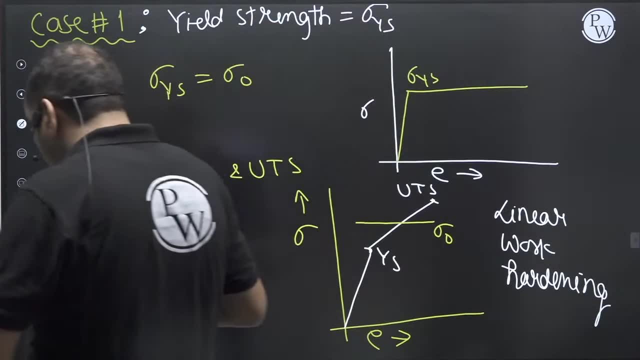 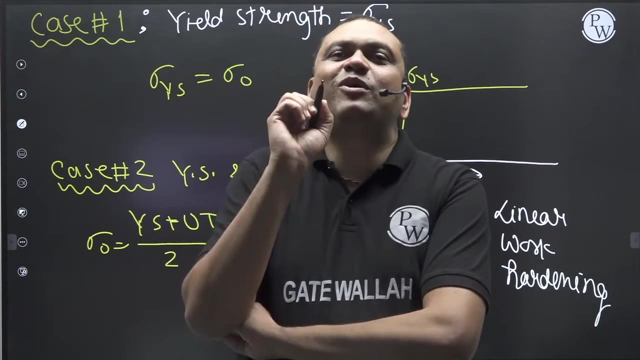 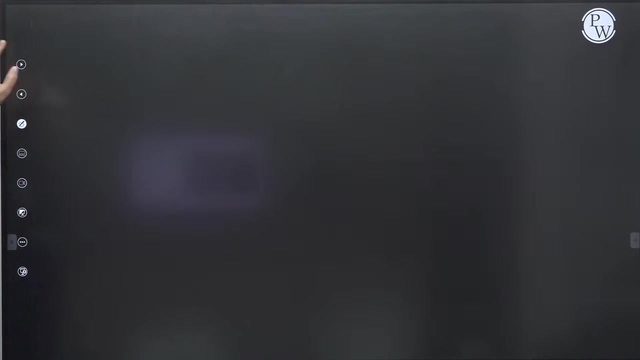 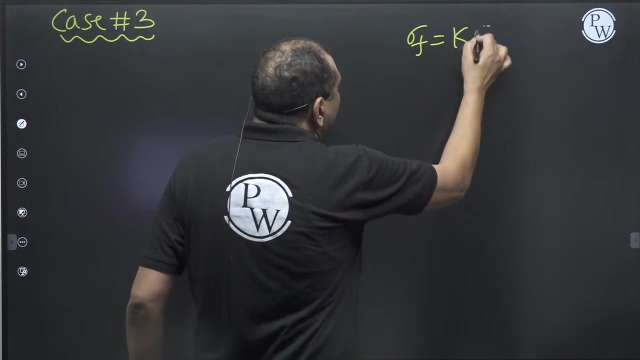 yes, but suppose. but suppose if you are given a flow curve equation. if you are given a flow curve equation, then what will you do? case 3 in the question you are given a flow curve equation means Sigma F is equal to K epsilon raised to power n. 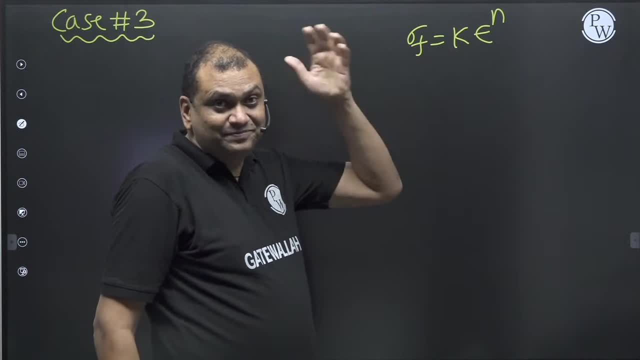 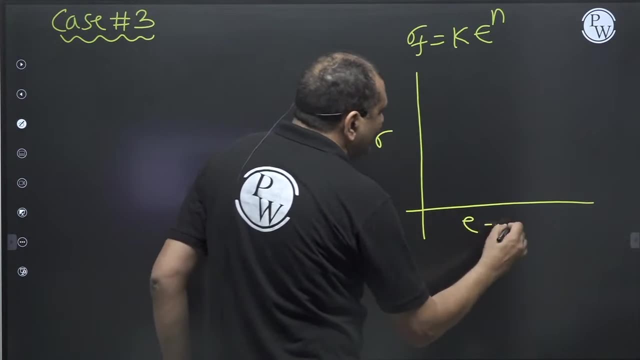 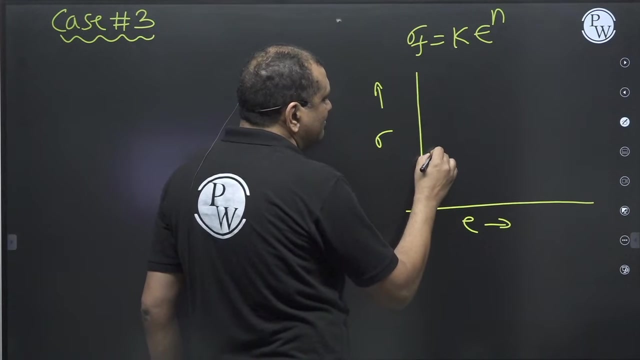 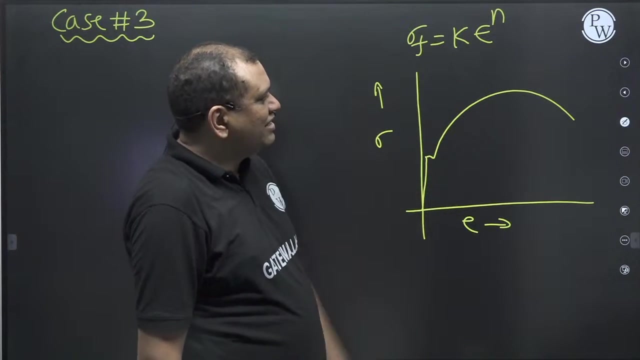 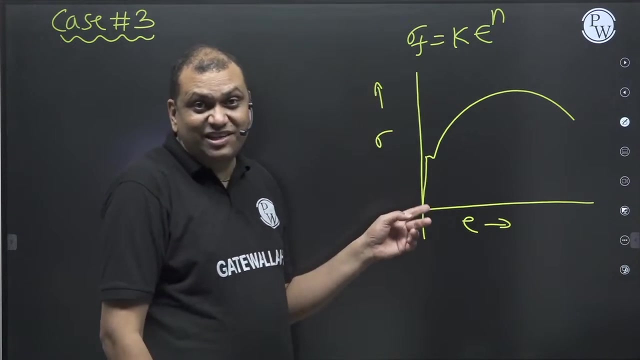 strength, coefficient and work hardening exponent is given. this means what is the question saying to you? that our material is following CG, elastic and work hardening. so when work hardening is there, do you know what it means? now look at it carefully, ok. 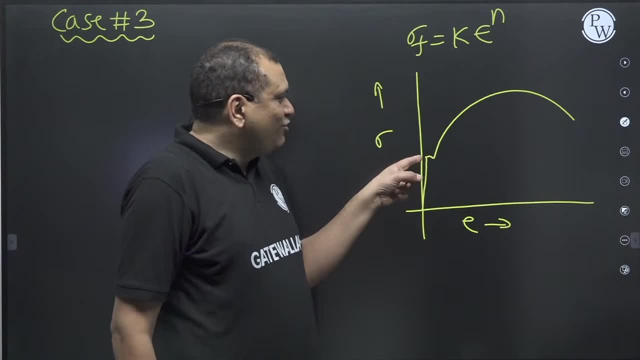 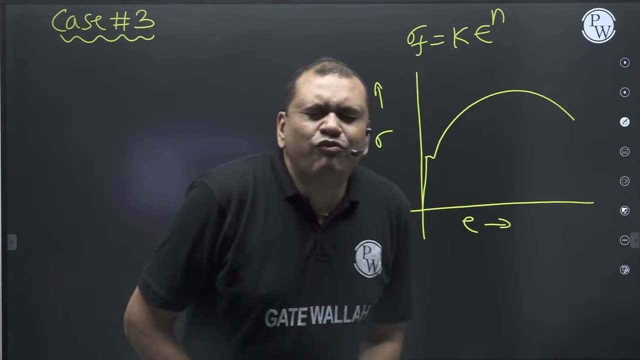 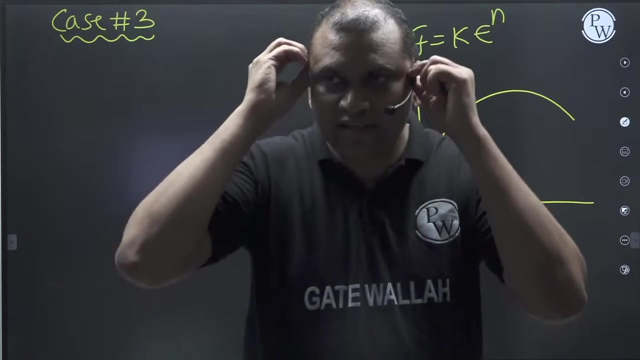 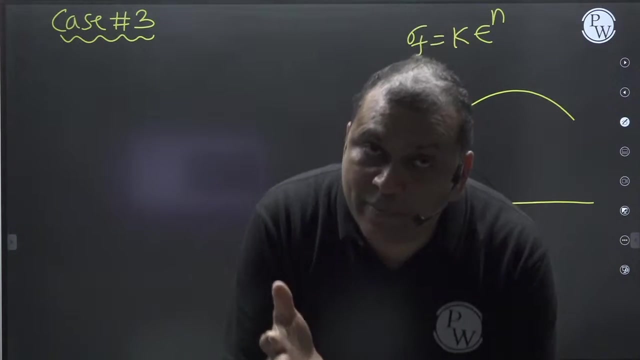 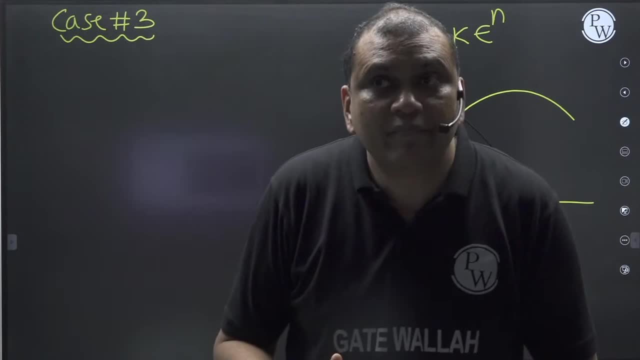 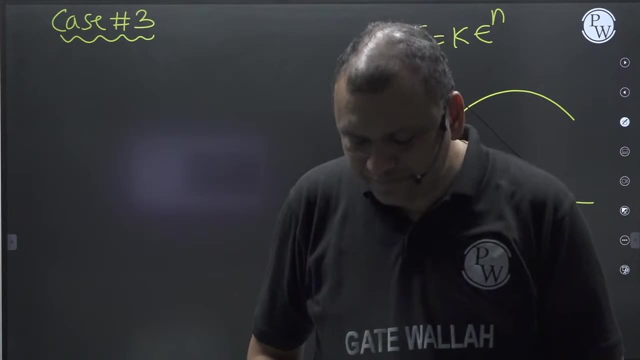 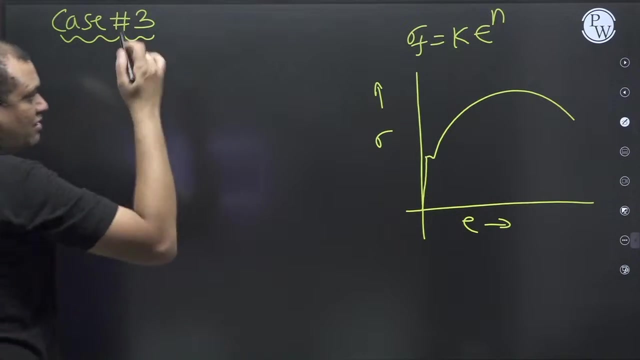 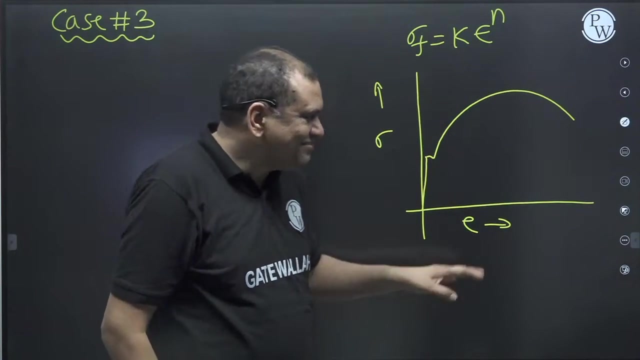 UTSB is flowing in vitamine B. metal is flowing, so I have to find out what is the average pressure at which the material is flowing. What is the average pressure at which the material is flowing? Do you understand? In this analysis, I have to find out what is the average pressure at which the material. 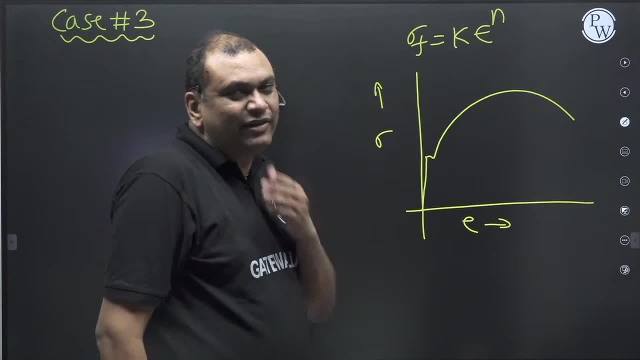 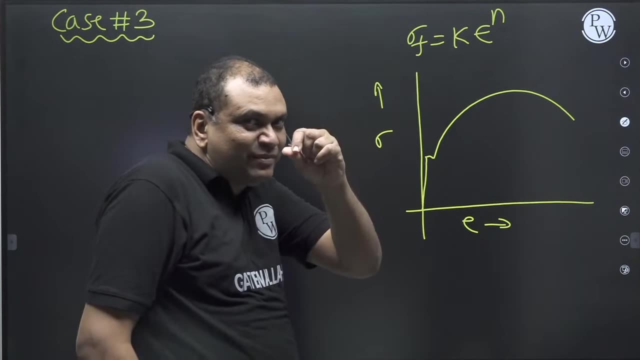 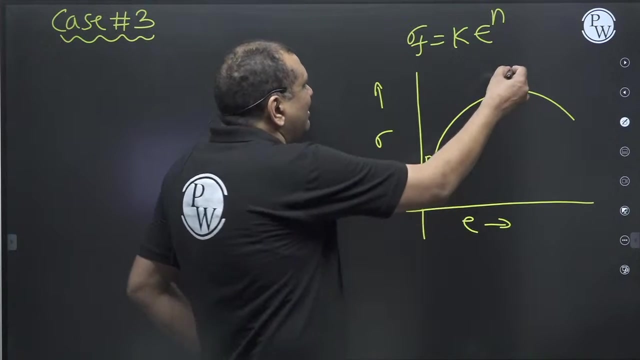 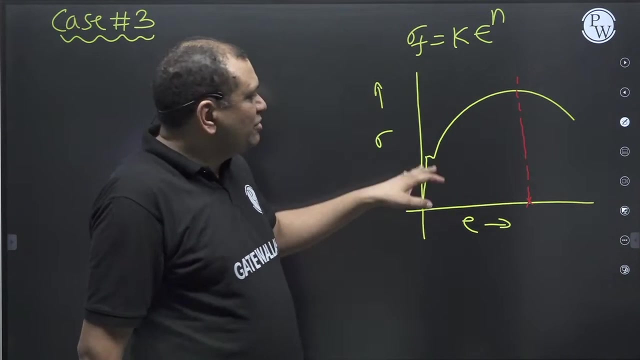 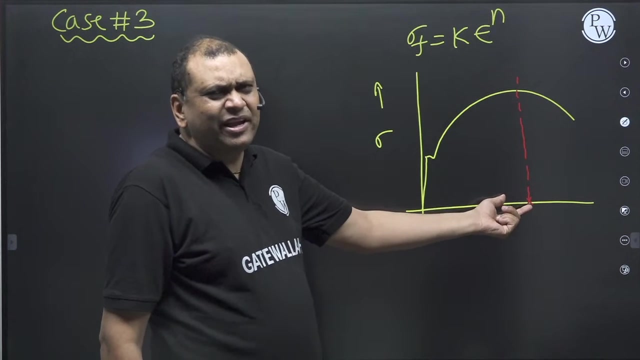 is flowing. In this analysis, I am assuming that elastic strains are negligible as compared to strains up to UTSB. Our elastic strains are 0.2% and this is around 30 to 35%. So, compared to 35%, I will neglect 0.2%. 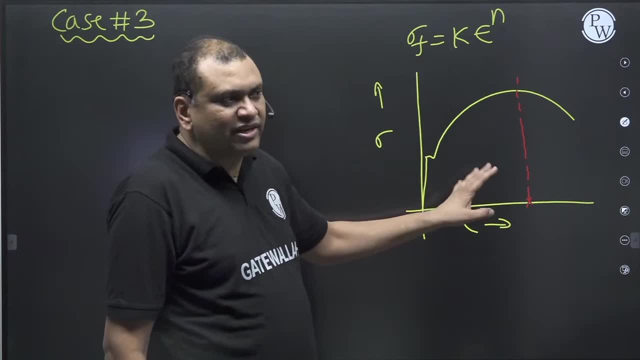 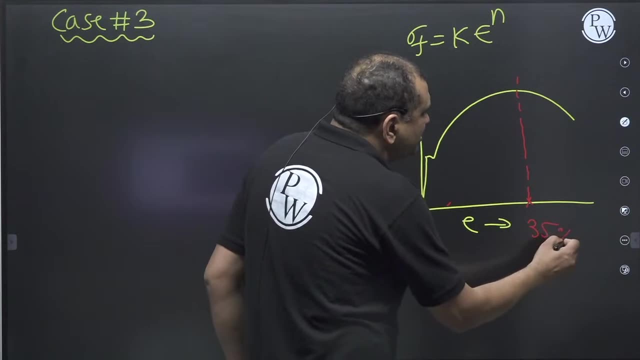 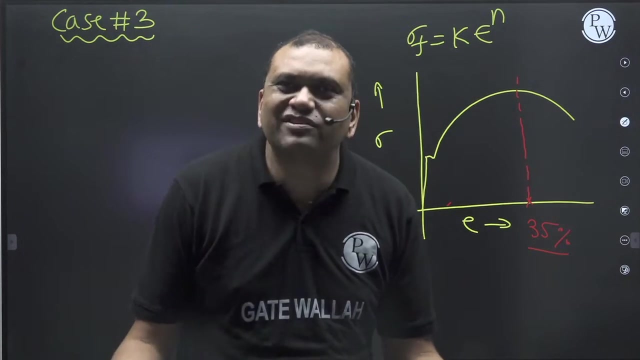 I am taking a big assumption here. Compared to 35%, the normal steel material which is up to UTSB, the percentage elongation is approximately 35% and the elastic region is approximately 0.2%. So I am neglecting it. 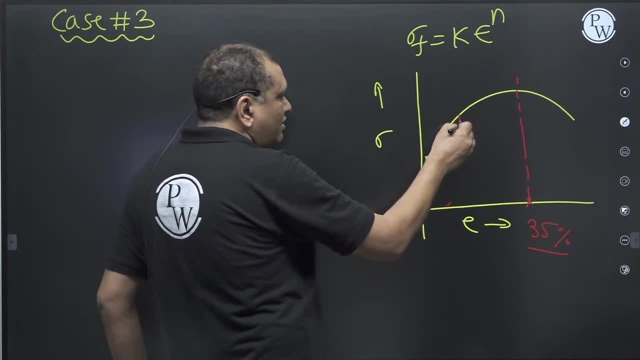 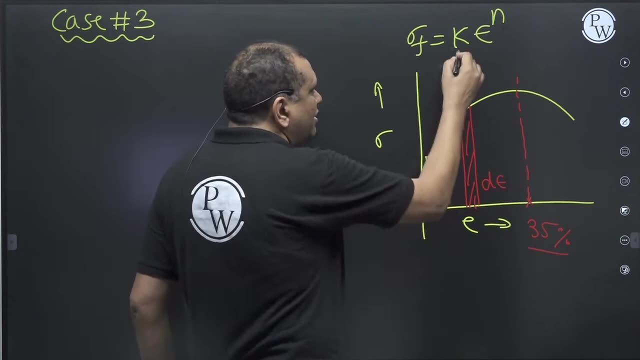 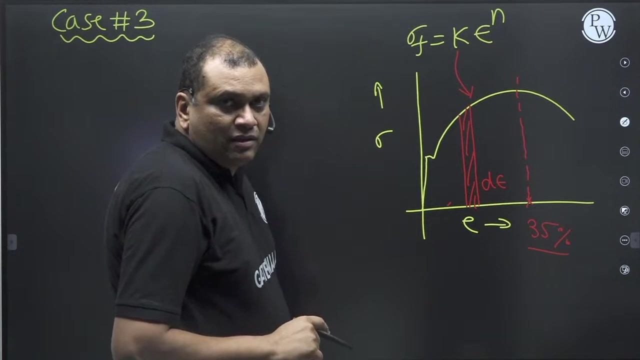 So you do this, Okay. Okay, Take an element here of thickness d epsilon, because the equation of this curve is: sigma F is equal to k, epsilon raise to power n And the total strain is up to UTSB. let us say this is epsilon 1.. 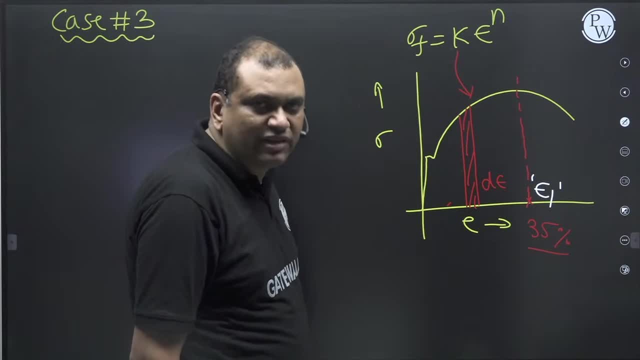 We are talking about true strain here. The total strain is up to UTSB, is epsilon 1.. So our mean flow stress is the same. So the total strain is up to UTSB. So the total strain is up to UTSB. 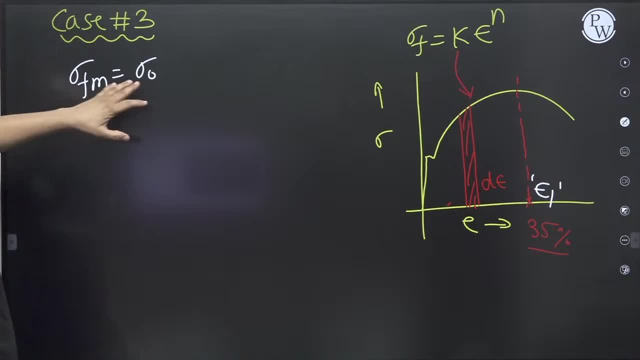 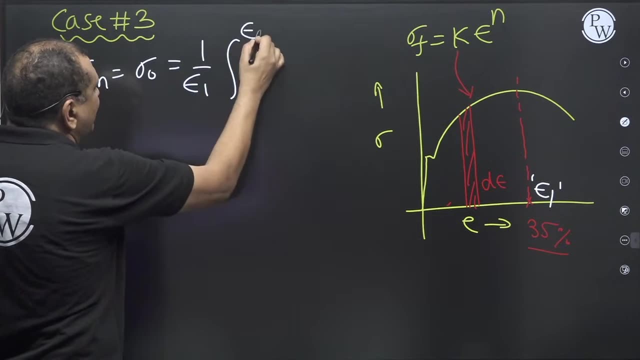 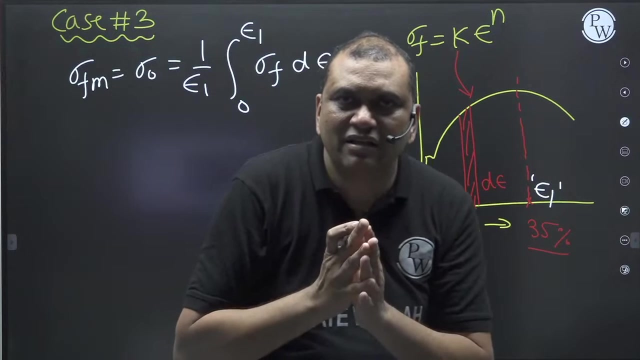 It has a mean flow stress. Mean flow stress is called nominal stress. So his average is 1. by epsilon 1 integral 0 to epsilon 1 sigma F, d epsilon. This is how the average will be. This is how the average will be. 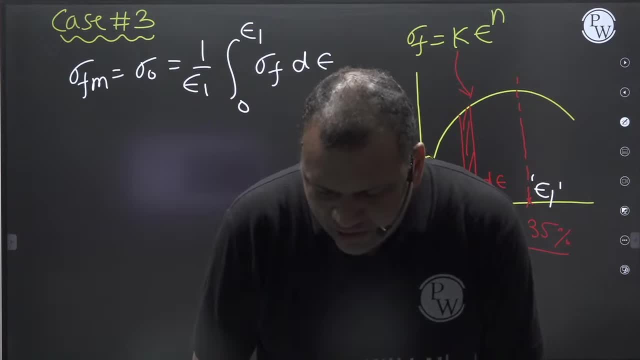 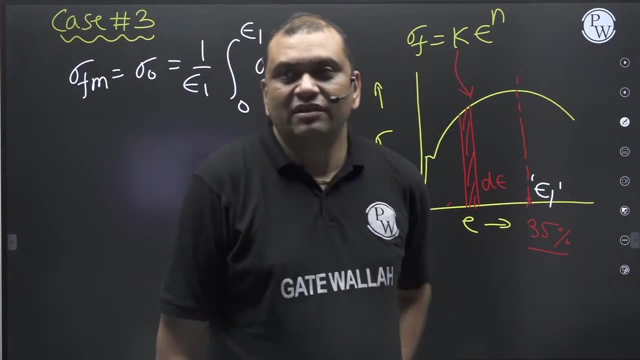 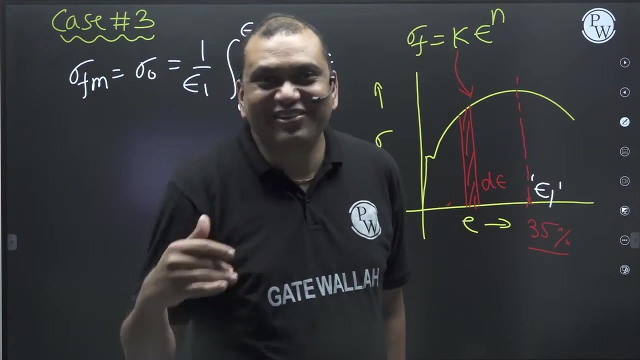 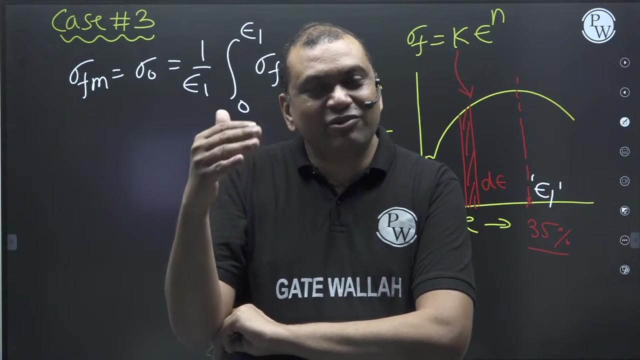 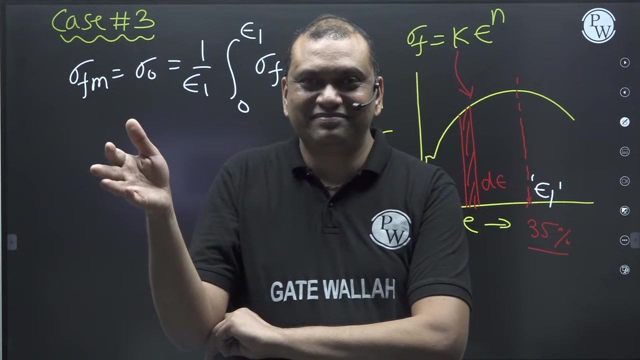 Without using red color. don't worry, I will not use red color. I wanted to take a section in the red. Okay, So you can see here I wanted to take a section. you have color contrast. I will tell you one thing: of course it is online, I am afraid to say anything. we are doing an interview guidance program, those who have reached the interview. after that there is medical, whether you take any PSU. so some people have partial color blindness. you don't have to take tension. you talk to me face to face, not on record. 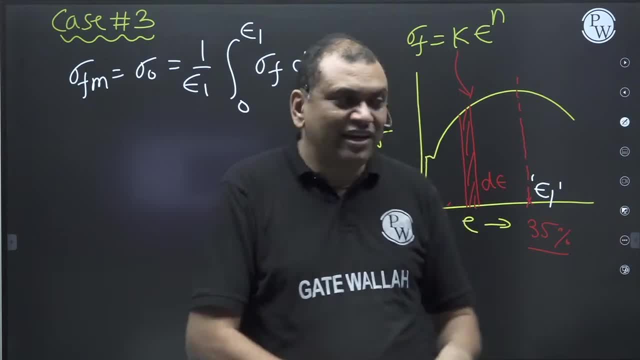 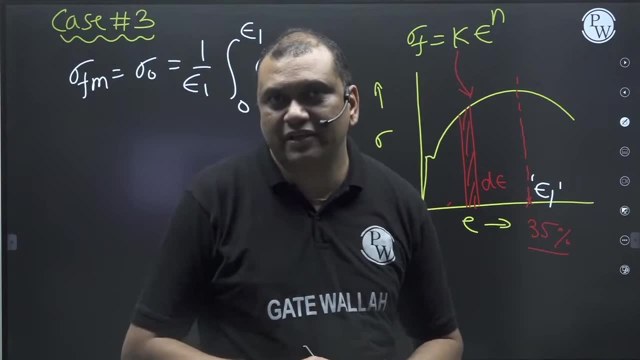 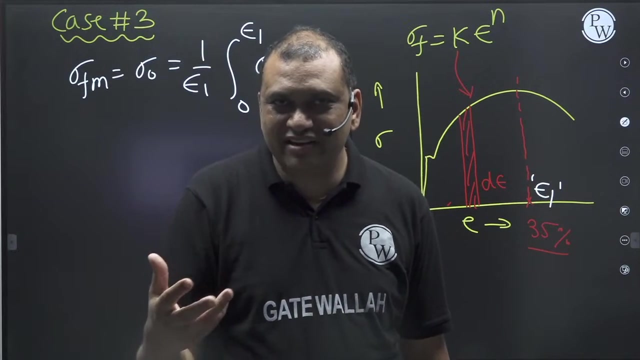 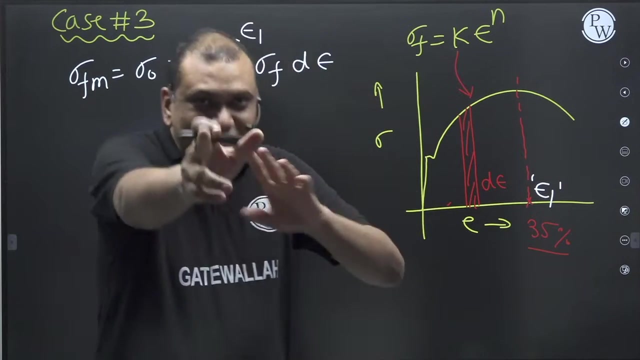 I will tell you if you have severe color blindness. some people don't see red color. sometimes they see another color. if it is partial, you can do something with it. but when we will talk to each other in the interview or you are my friend, I will tell you how to manage it. but we will discuss it offline. don't take tension, we are with you. 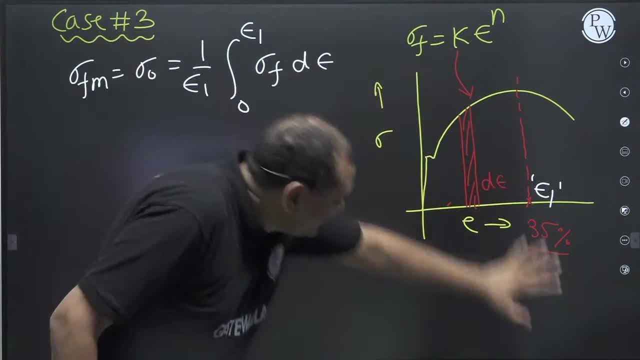 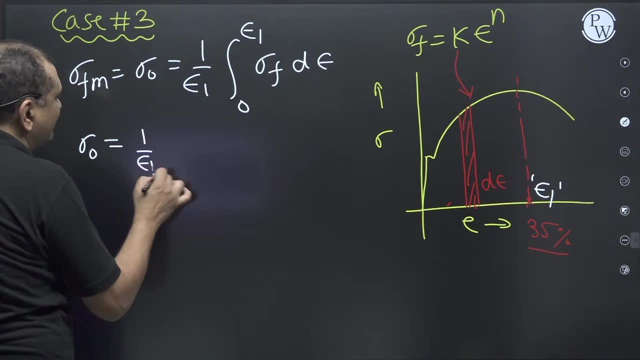 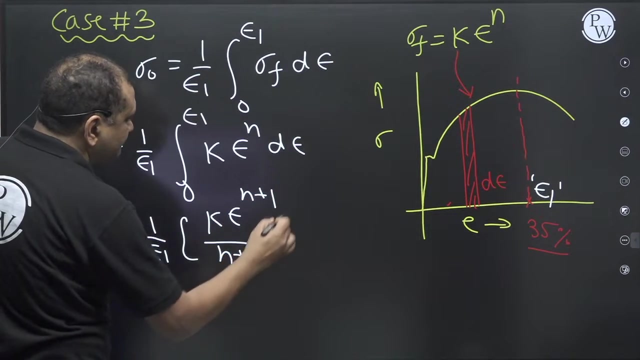 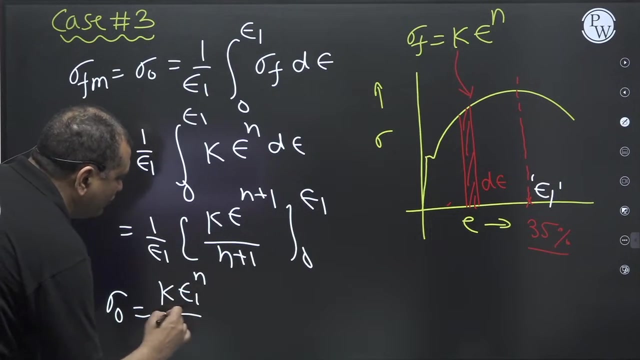 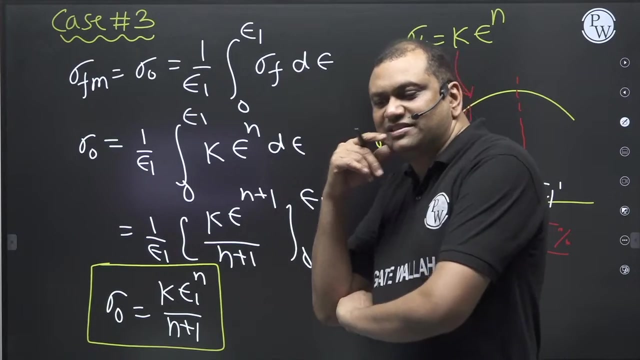 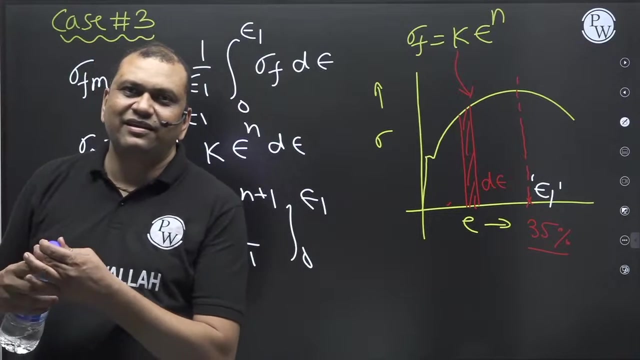 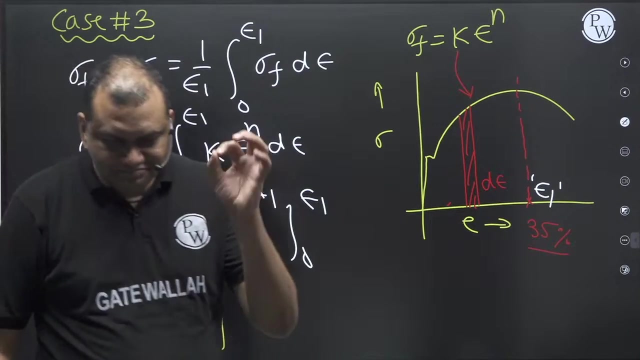 so this is coming now I have to find the average, so do it here. you all are attentive, right? everybody is attentive, right. so cool your mind again, because here 95% child makes mistake, 95% child. 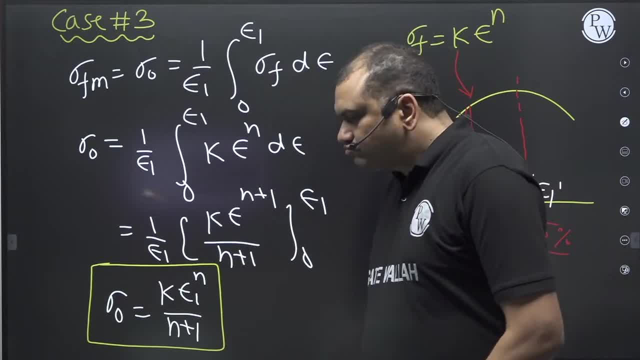 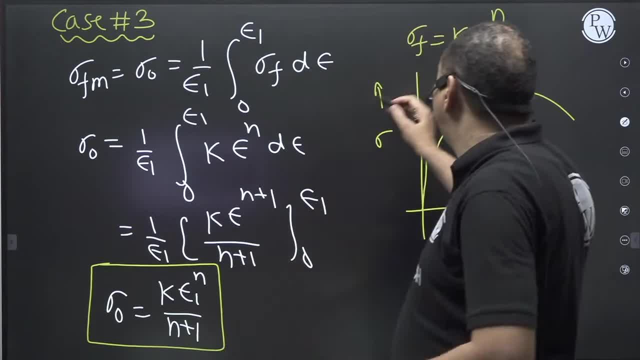 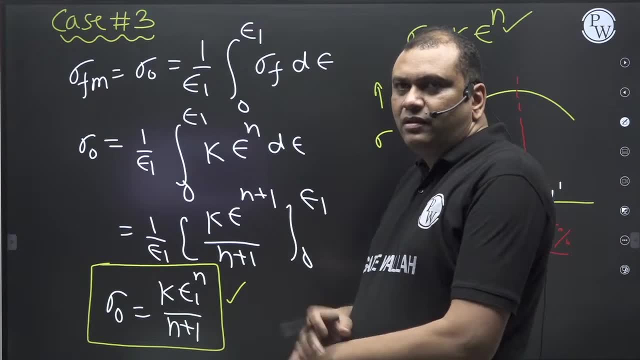 95%. I told you that we will teach yu and we will teach yu. then I have taken the skin of來了 is so OK. so this is skies and that you have been using. ha ha, that you have been using, yes. 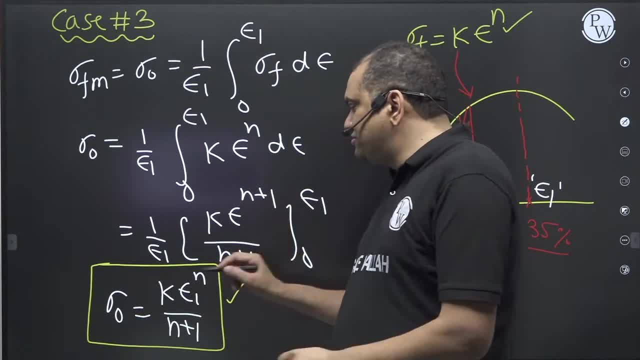 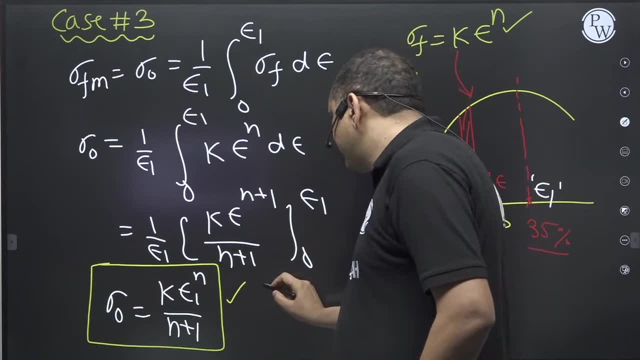 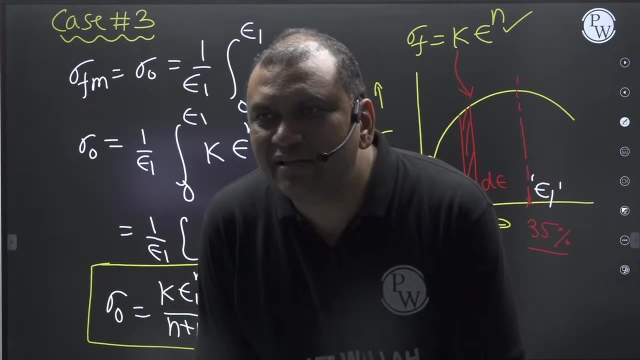 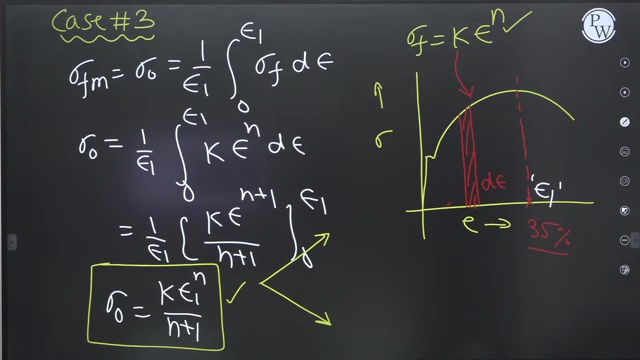 see, see, I have not done my performances by saying I am will have to, I will do my first air for my child and I will do him anyway, and that's it. You have to take care of two things in implementing this equation: Cheers. 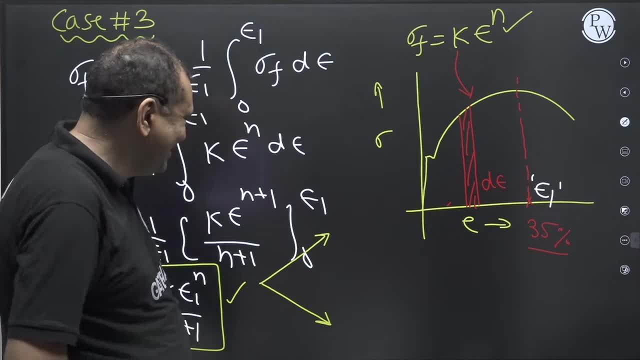 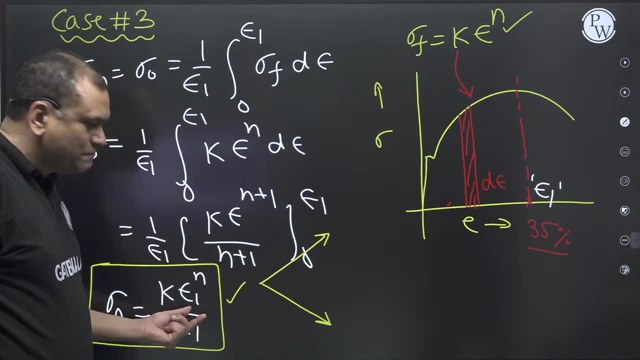 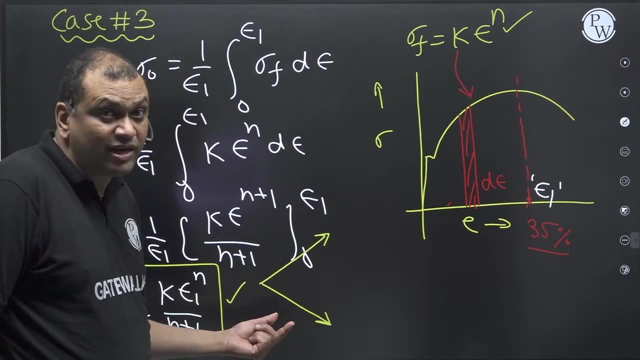 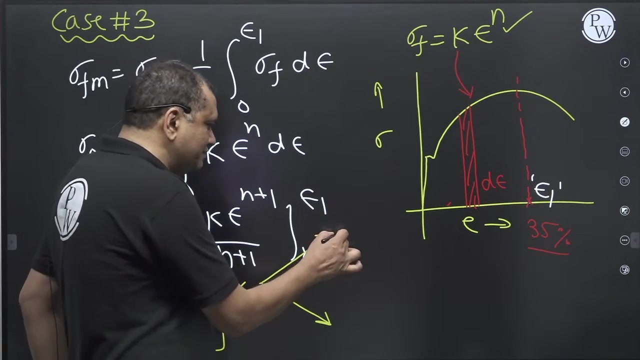 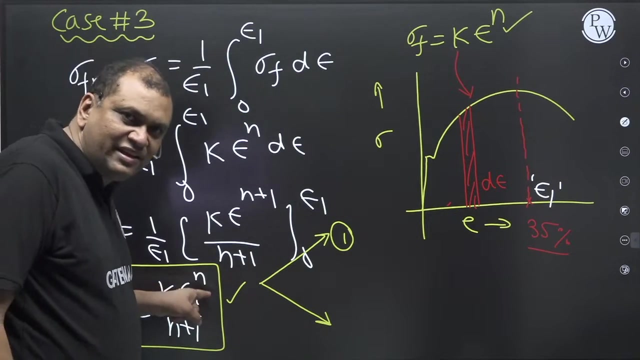 This is Lassi, nothing else. Sigma naught is equal to k. epsilon is equal to power n over n plus 1.. Don't apply blindly. Don't apply blindly. You have to take care of two things. The first thing is that our true strain. 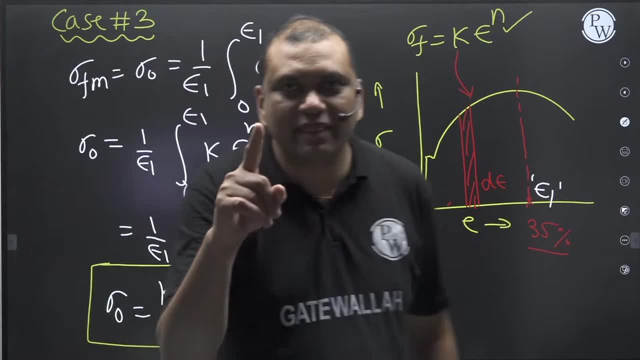 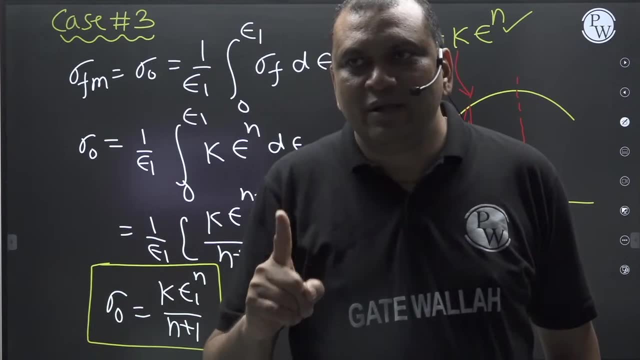 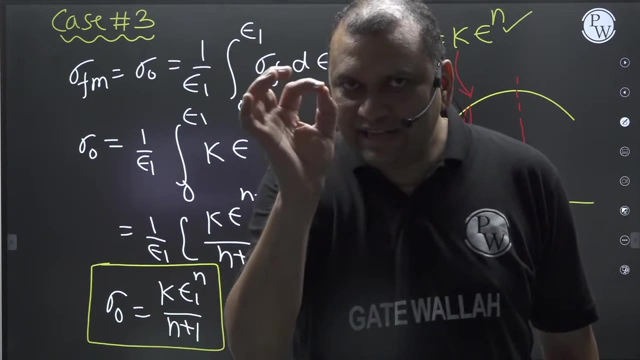 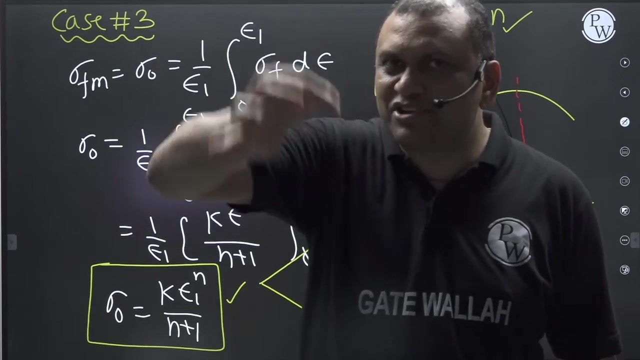 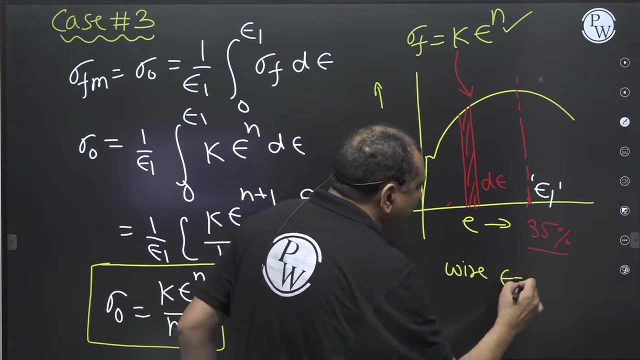 we will calculate true strain. we will calculate true strain the direction in which the load is applied. We will calculate true strain in the direction in which the load is applied. For example, if it is a wire drawing, epsilon is ln, Lf by Li. 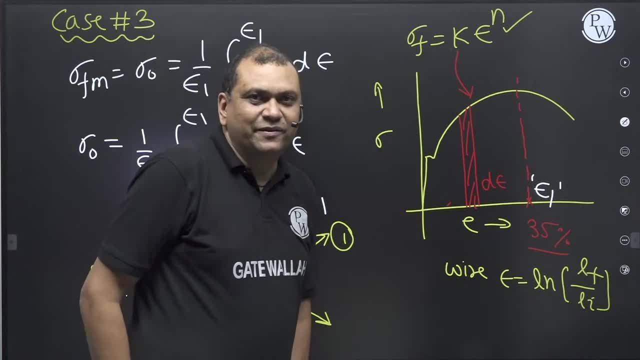 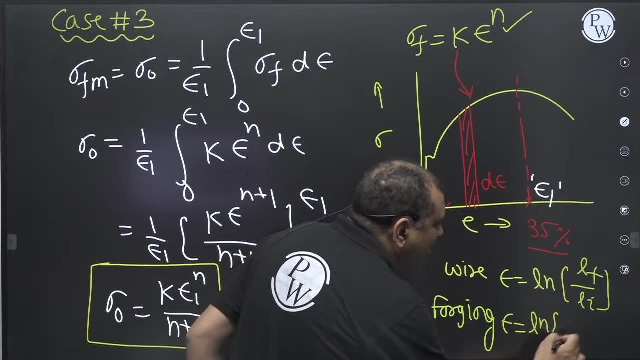 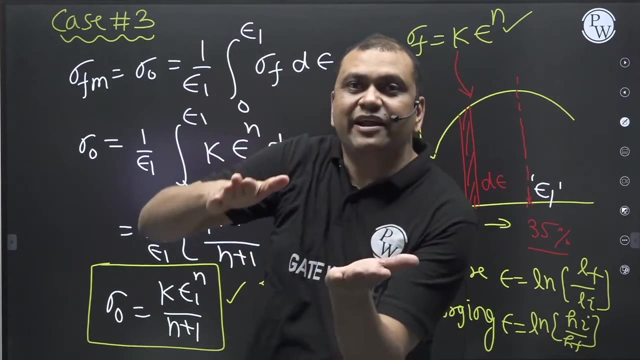 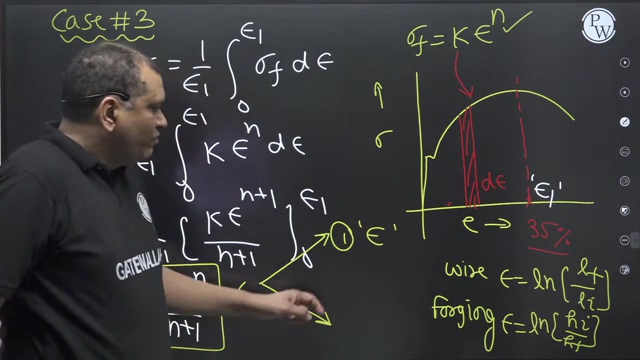 because we are applying the load in the longitudinal direction. But if it is a forging, epsilon is nothing but ln Hi by Hf, because our force is applied in the height direction. So the first thing is that where I will take the value of epsilon. 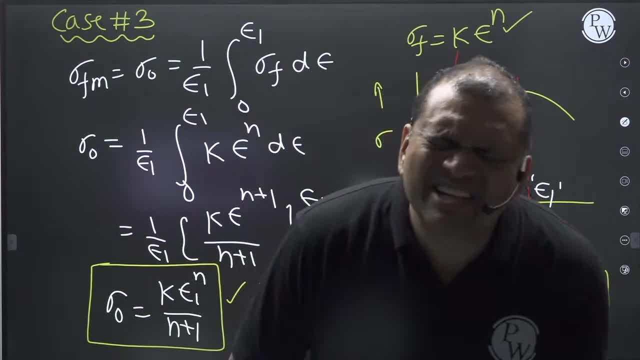 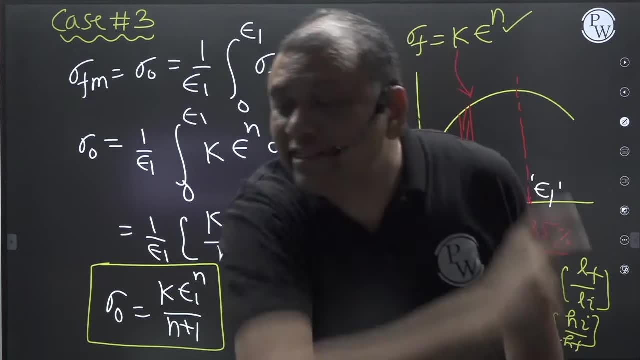 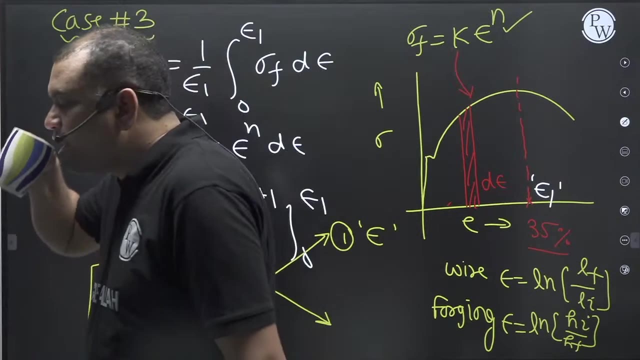 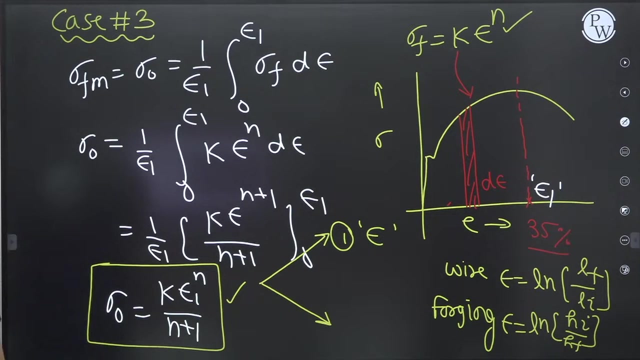 in which direction will I apply epsilon? The direction in which the load is applied in the metal forming operation. The direction in which the load is applied in the metal forming operation. The direction in which the load is applied in the metal forming operation. Okay, 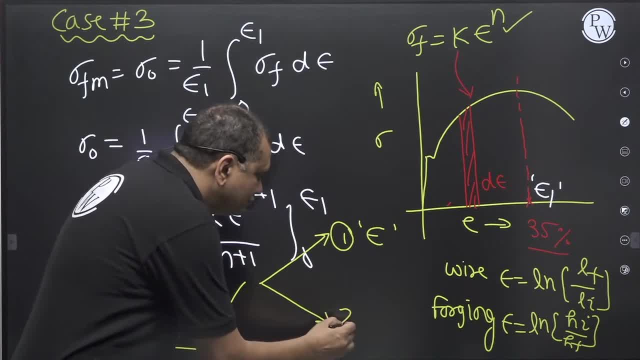 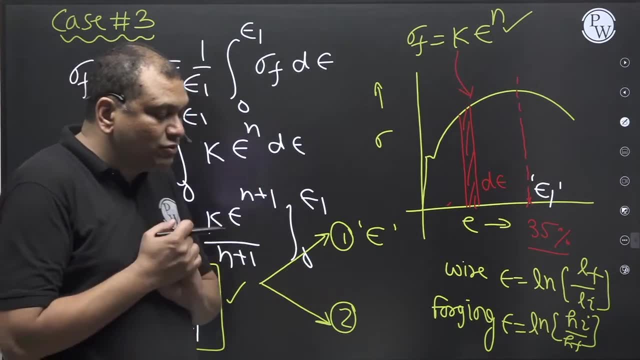 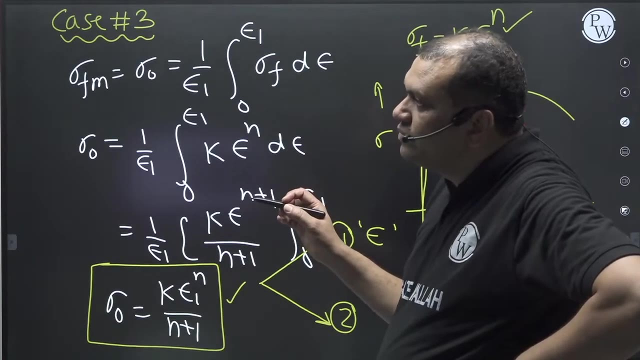 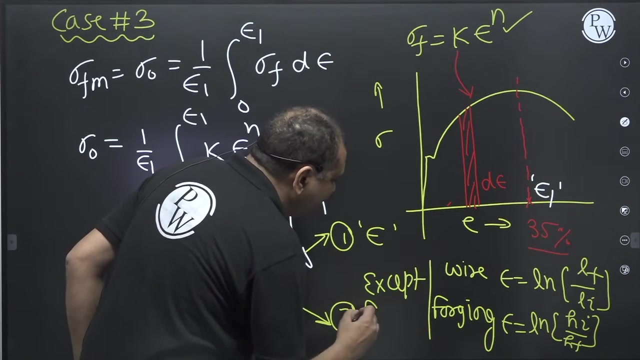 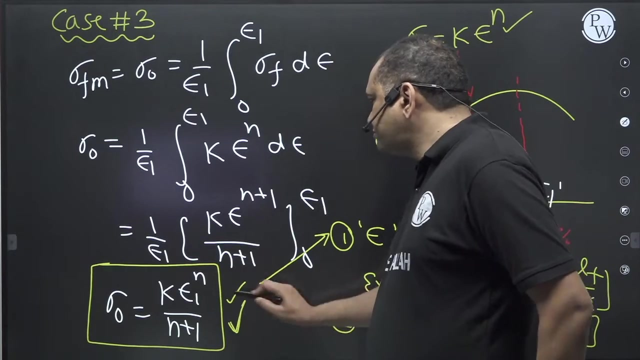 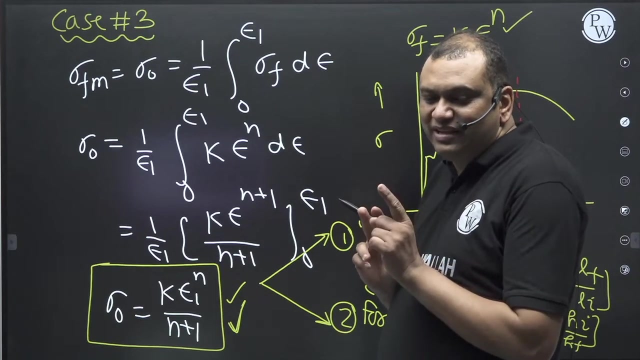 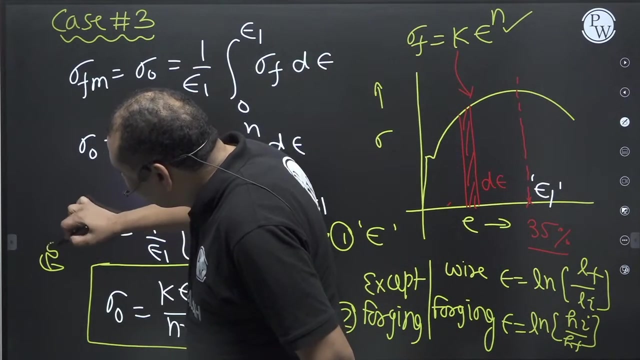 The second thing is that don't forget this section. The second thing is that, except forging, except forging, I will use this formula for forging me formula. use me Karuna forging man formula. use me Karuna way. in case of forging you, I will use direct formula. 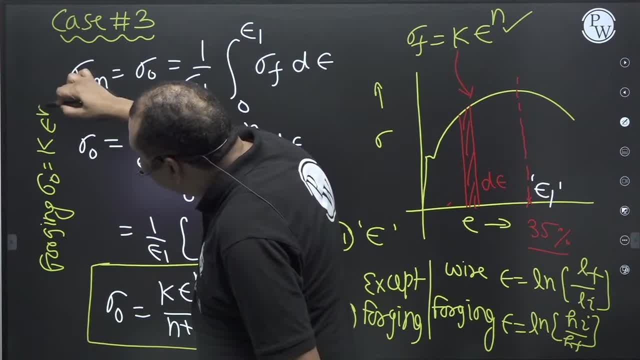 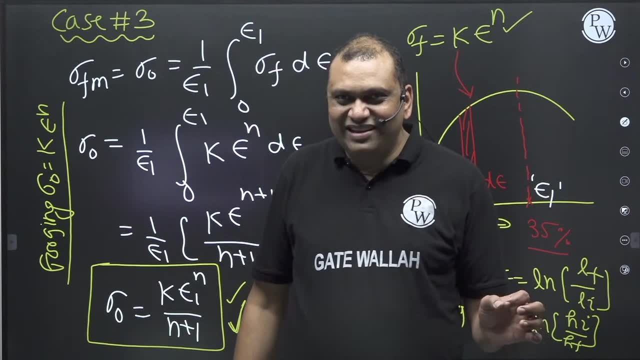 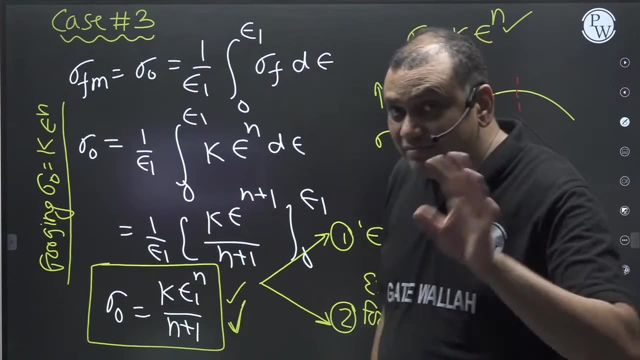 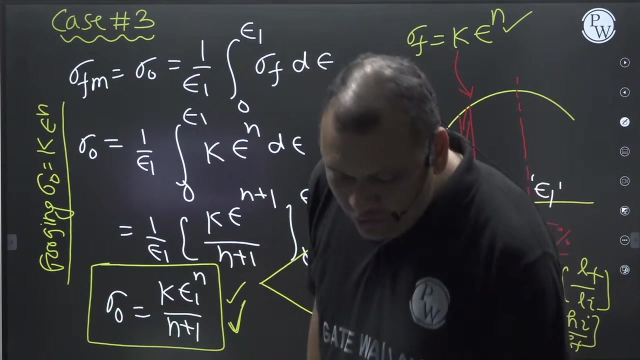 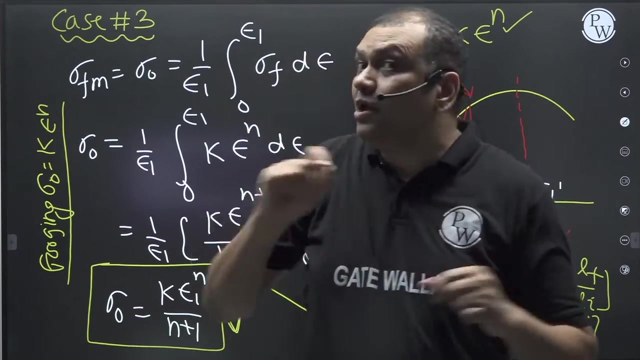 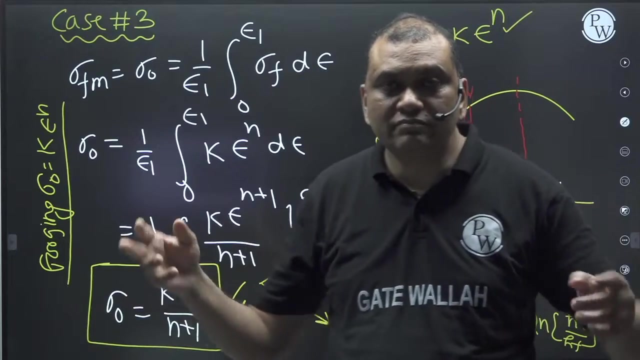 I will not calculate average. area of identity, manner you don't appoint, go for which in there. may average calculate me Karuna, me direct formula. use Karuna, it's good. or even a jo forging. with ena the load is instantaneous. buck, buck because in wire drawing or, let us say, rolling or extrusion, some time is available for. 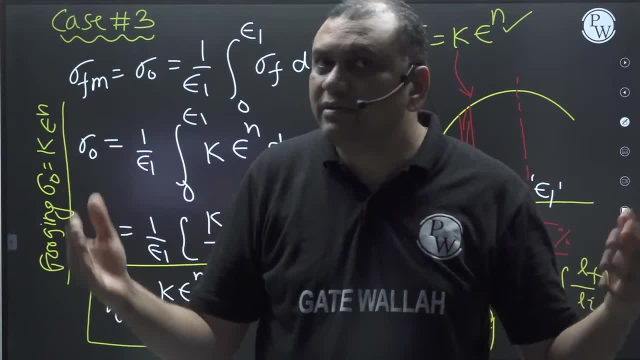 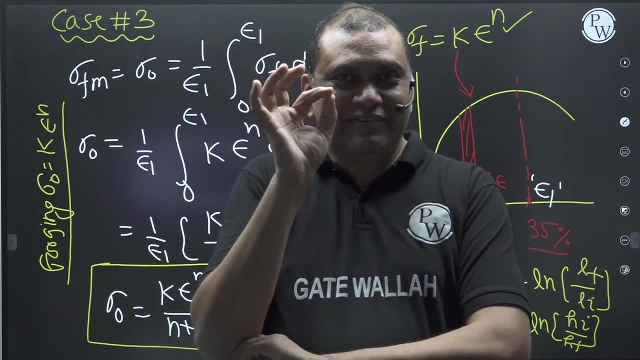 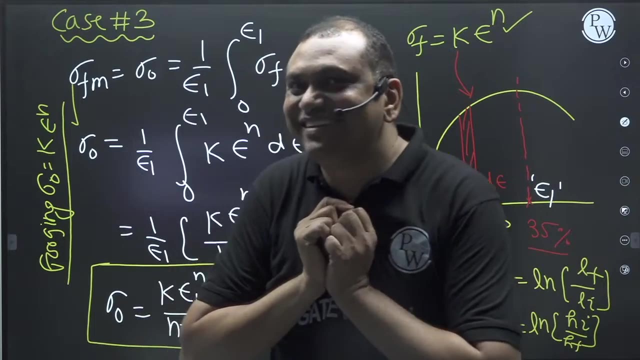 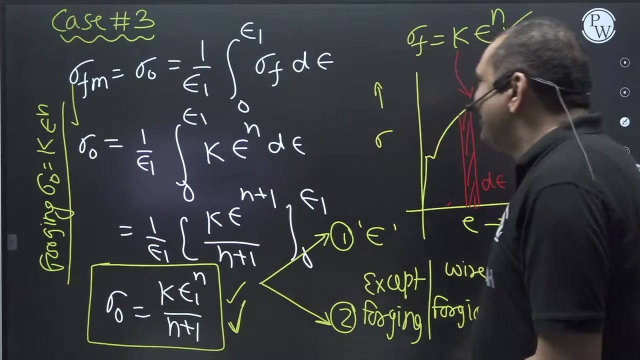 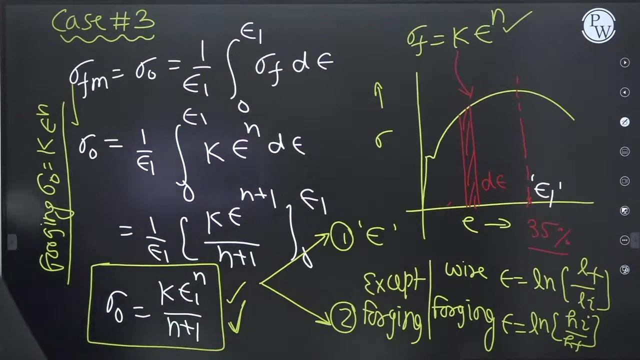 deformation, but in forging it is almost a situation. so forging man may average. calculate me Karuna man directly. use Karuna man up. so much Rihanna. so Sigma not case a calculate Karuna man a go, but idea via Sigma may calculate. Sigma not may case a calculate Karuna man a go. without the eye, again you can be. 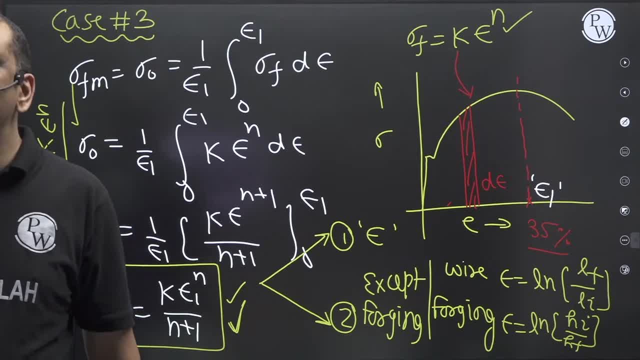 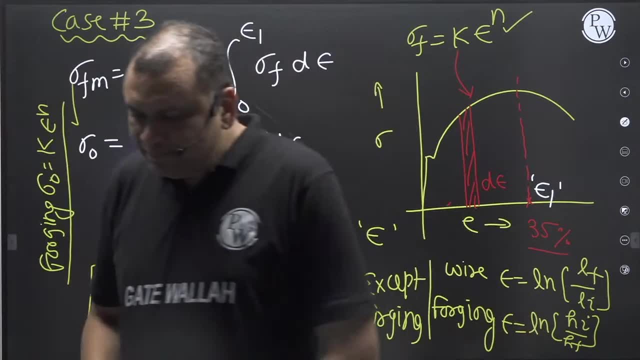 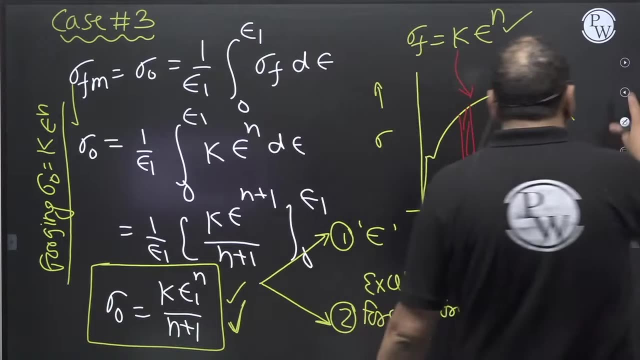 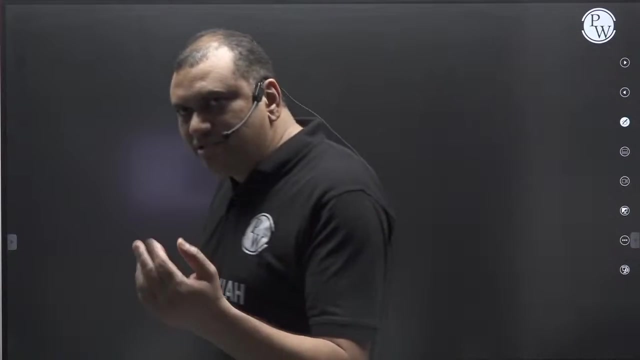 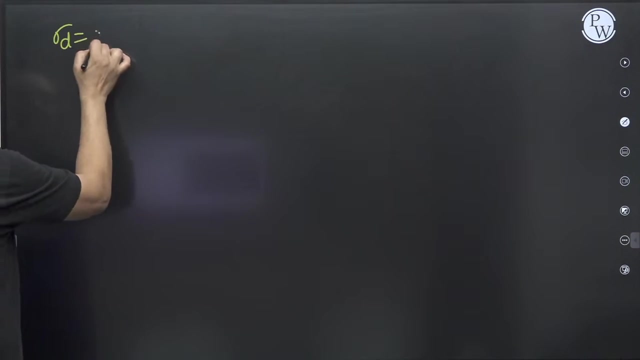 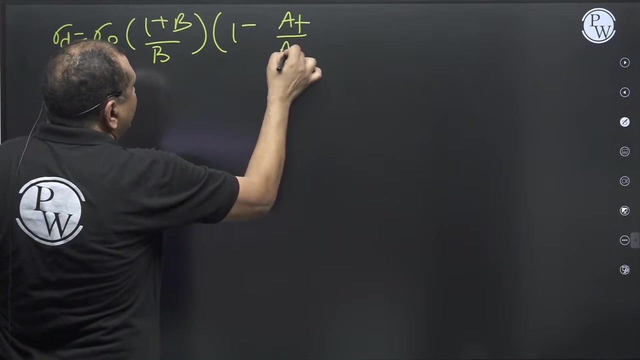 active on the chat box because I told you not to use chat box for 10 minutes. he can a. okay, all right now, get me a cheese or a Tia. apne formula, de Khanna. Sigma D is equal to Sigma Naught. one plus B by B, 1 minus a f by a, I raised to power b. 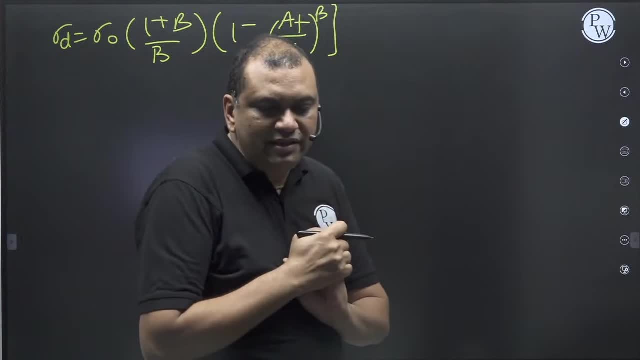 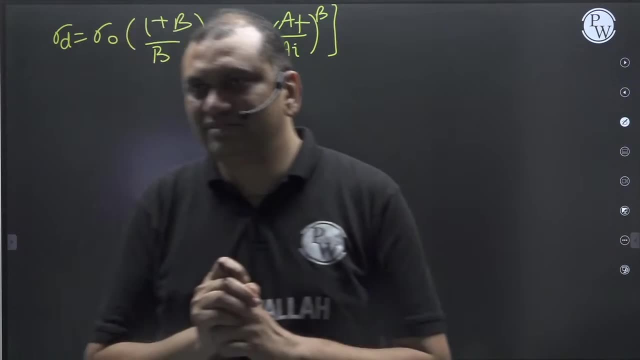 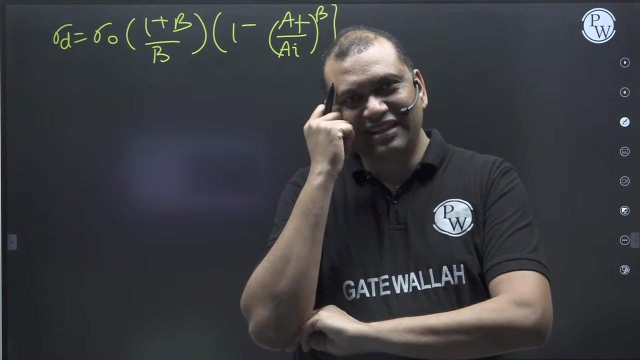 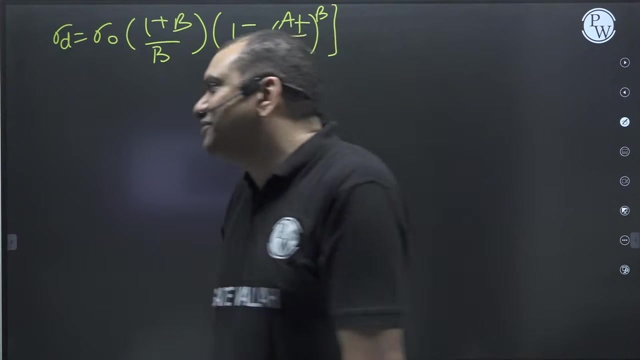 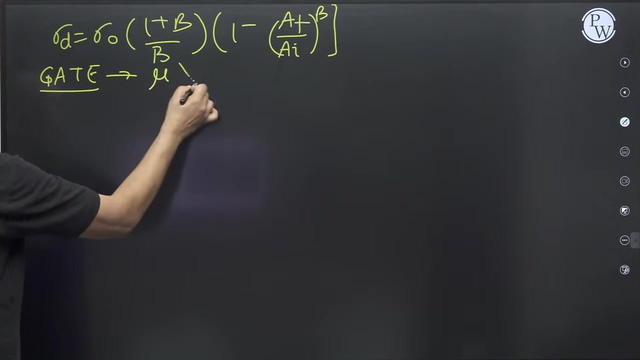 yet this lab analysis, the formula: hey, yucky. slab analysis: kaha formula: hey, Tequila, okay gate. may a questionnaire at a say okay gate. may a questioner at a say say: suppose suppose friction is not given to you in the gate question, let us say coefficient. 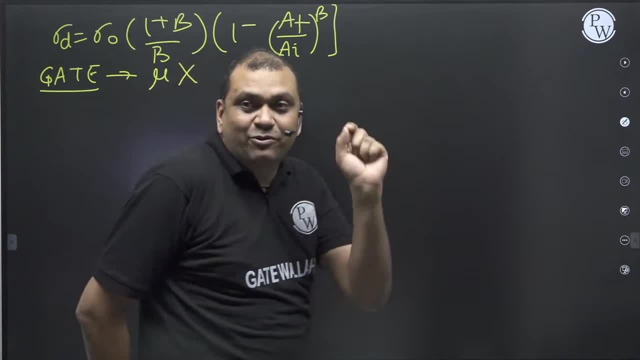 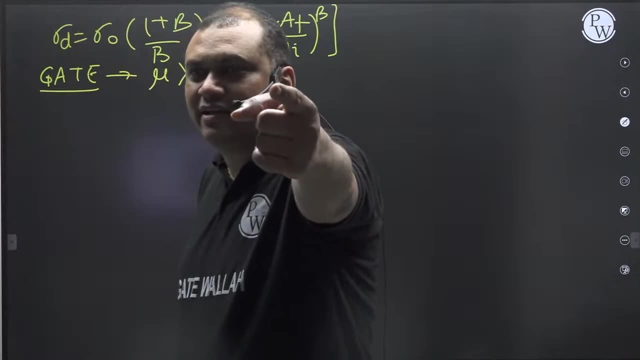 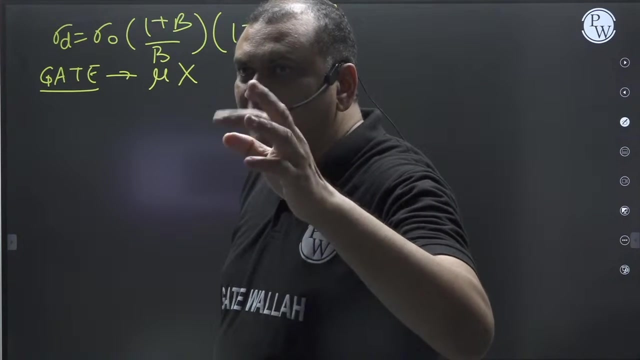 of friction is not given to you in the gate question coefficient of friction is not given to you. we will see tomorrow for forging: tomorrow I will repeat the forging point tomorrow. don't worry, because there are 3-4 students are asking about forging. we will discuss about forging tomorrow, not today. 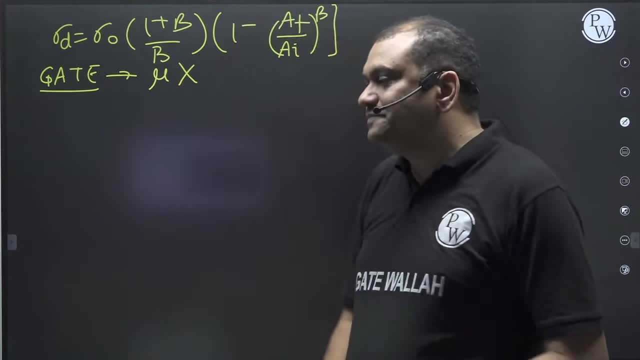 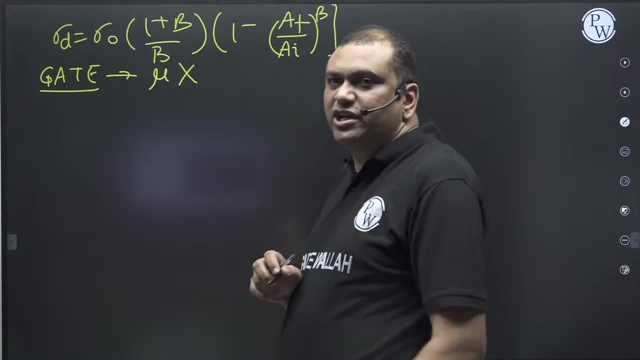 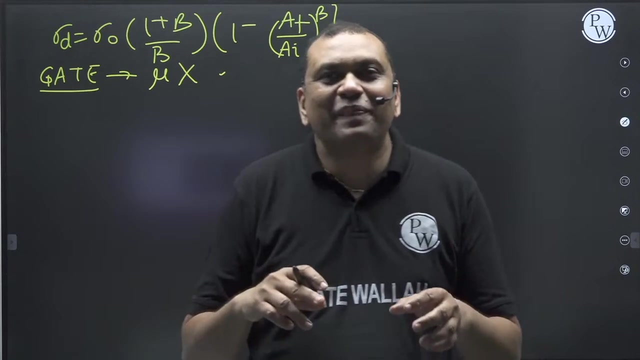 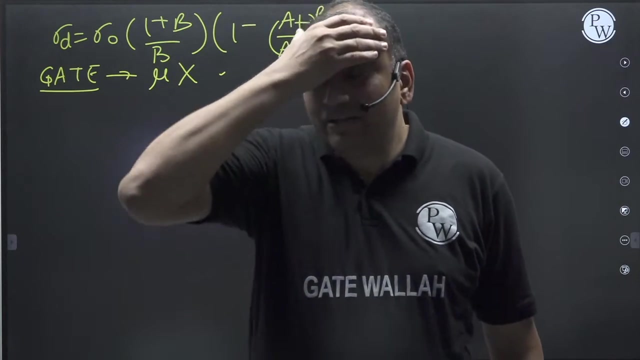 today. I have some wire drawing on it. we will repeat it again. don't worry, if in the gate question coefficient of friction is not given, it means that it is zero. please look carefully here with a cool mind, because many of our children have a warm mind, because they keep thinking wrong things. 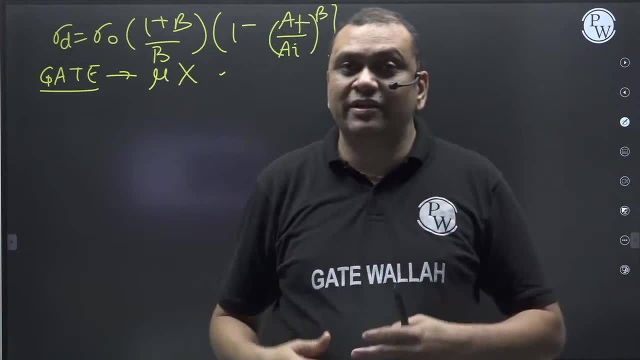 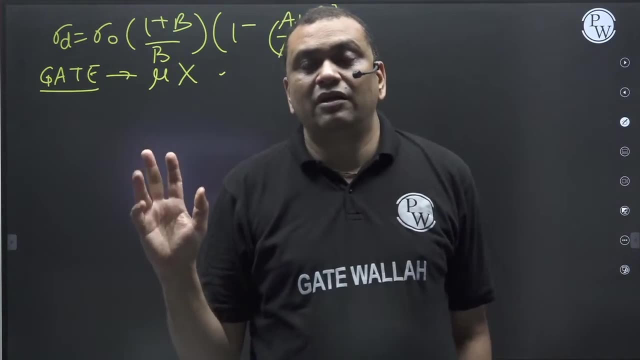 so do some bhajan for half an hour, whatever religion you follow. if you are a muslim, then do morning prayer. if you are a sikh, then go to gurudwara at least half an hour for half an hour. if you are a christian, then go to church. 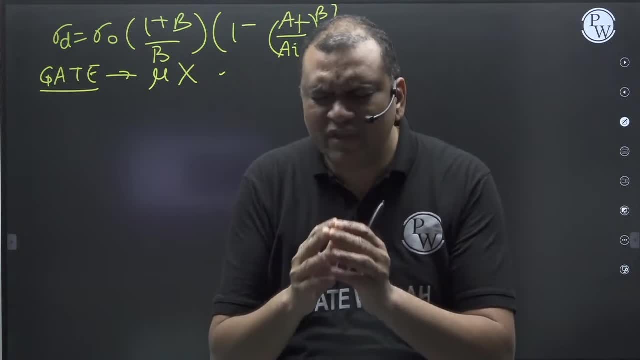 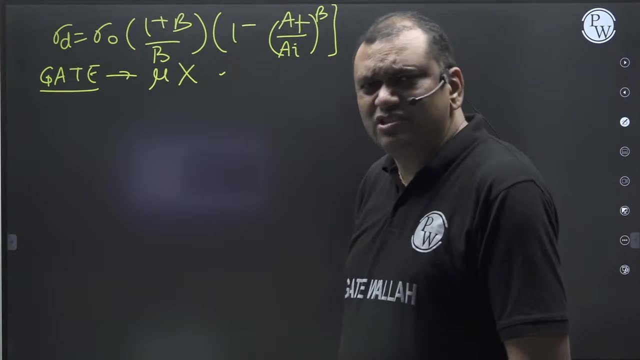 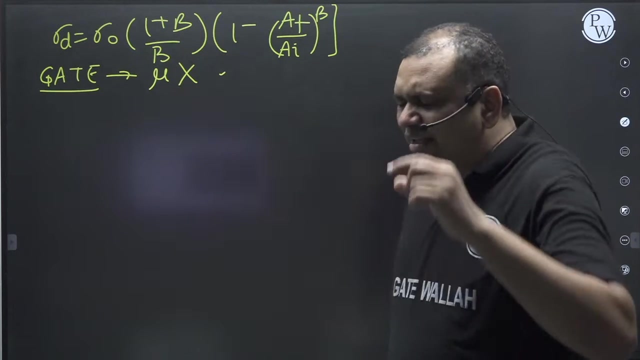 on sundays, and sundays and morning for half an hour, remember god. this will improve your character and your mind will be sharp. so, whatever religion you follow, do it for half an hour and look carefully here in the gate question. if there is any question. there is no coefficient of friction. 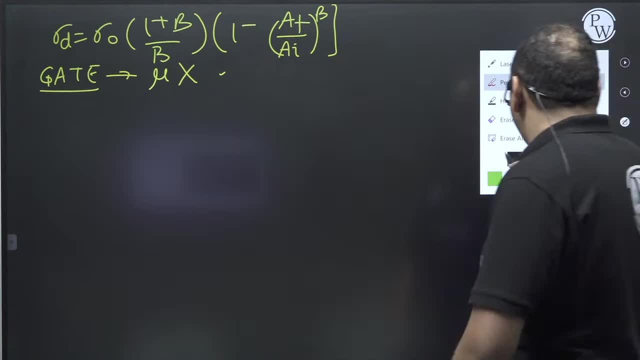 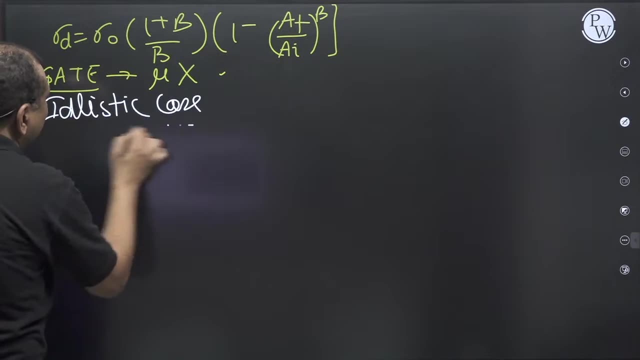 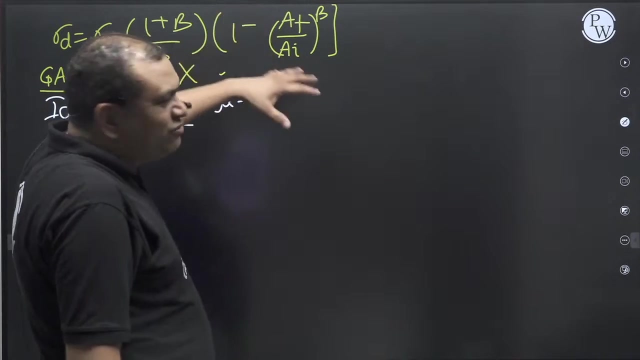 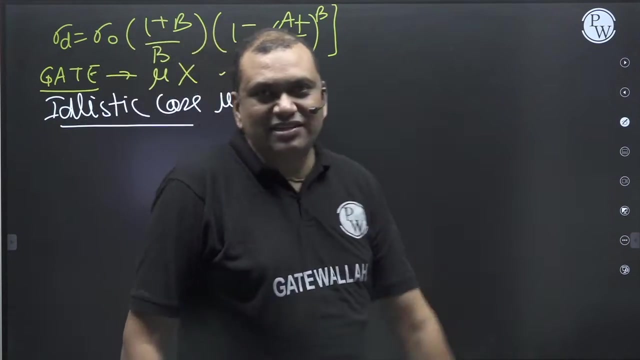 it means that it is zero. we call this idealistic case idealistic case and in that coefficient of friction is zero and if you prove this, it is the same syllabic. don't put zero in mu directly. you will not get any answer from where this was proved. 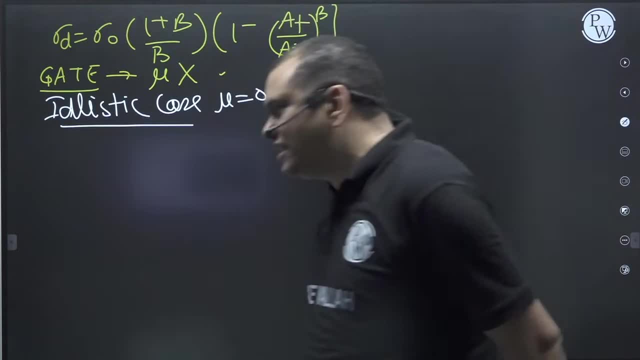 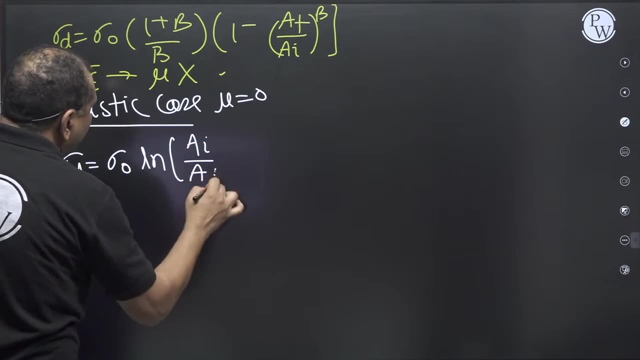 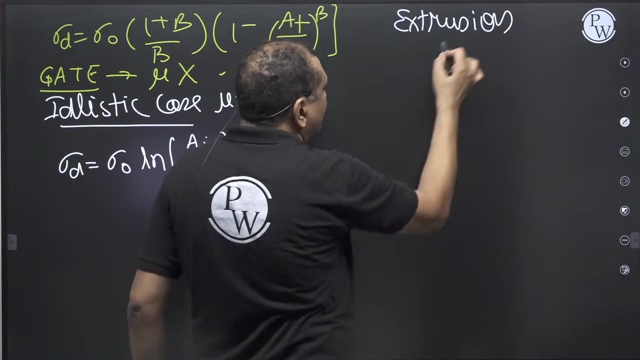 don't go to crash course if you put mu zero in it. so it will be sigma d equals to sigma naught l, n, a i by a f and in extrusion. and in extrusion a i by a f is called r. this is called extrusion ratio. 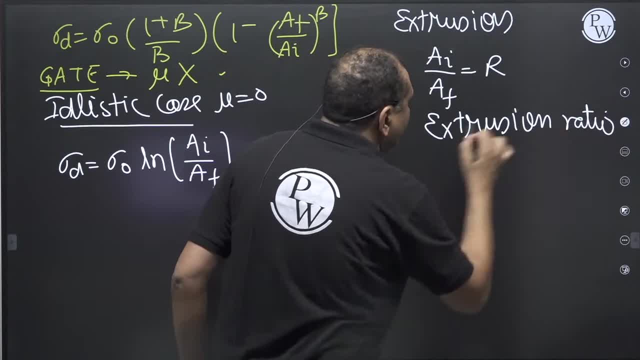 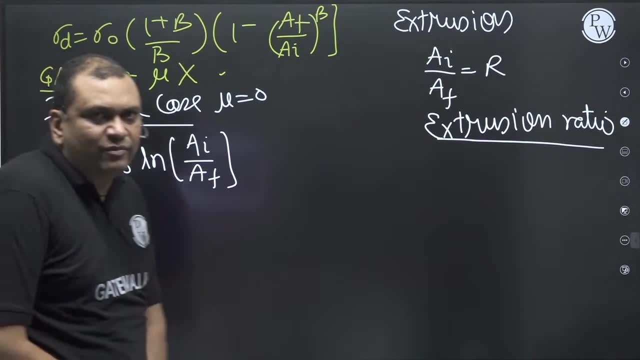 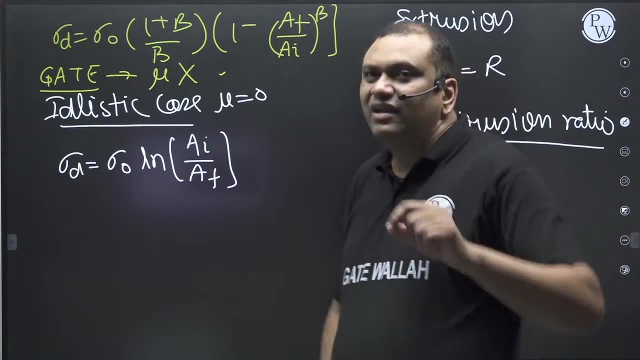 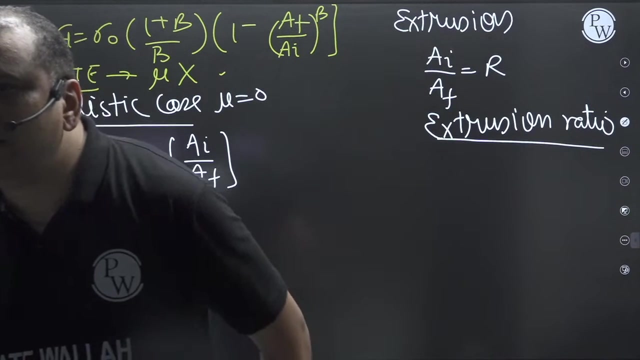 this is called extrusion ratio, so this formula comes. so in gate directly, this formula based, there are many questions. in gate directly, this formula based, there are many questions. I am explaining you the point here. I am explaining you the point point. this is: Abhir Roy, can you ask me this question again tomorrow? 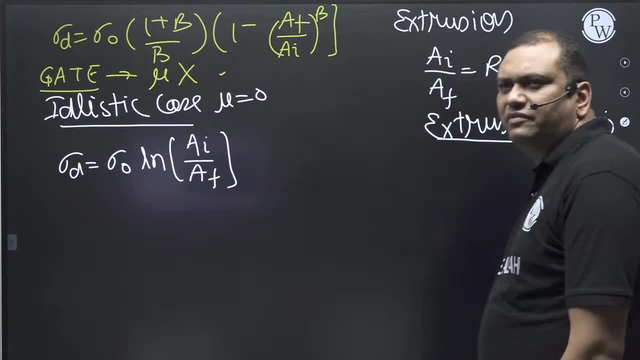 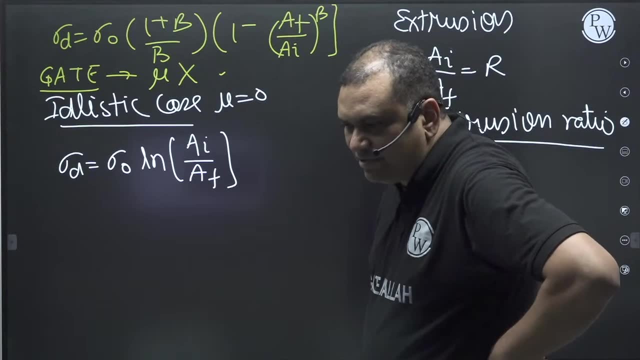 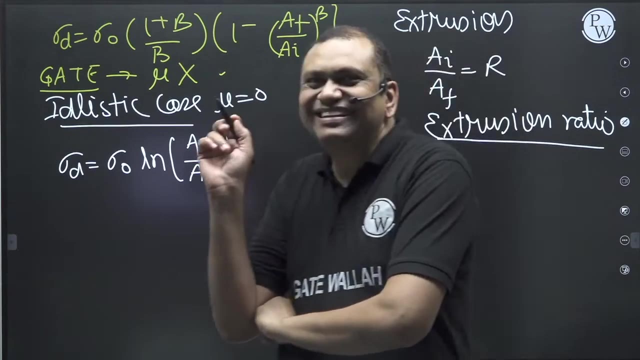 I will explain because you know it is a very good question, Abhir Roy. really very good question. I want to finish this. it was 11 o'clock today. my class is up to 11 o'clock. ok, listen carefully what I am saying. one question is repeated many times. 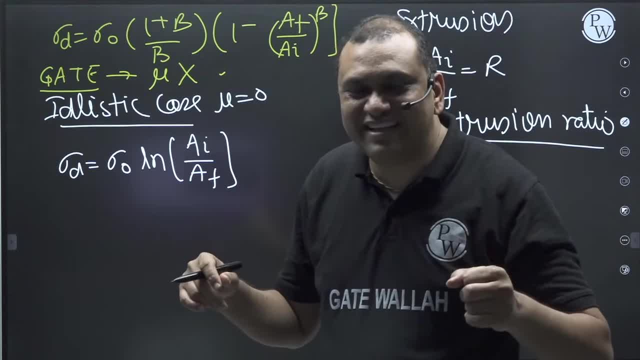 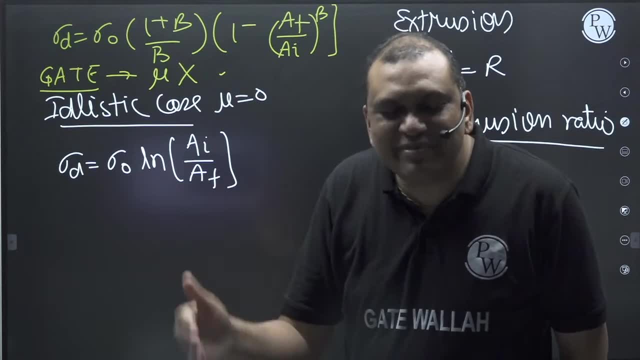 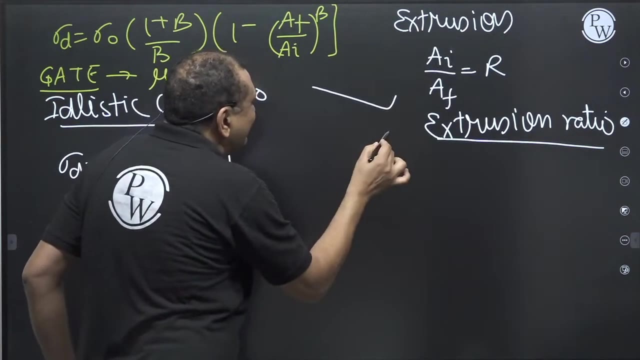 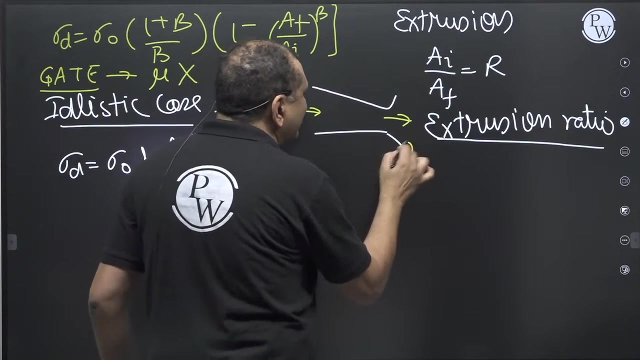 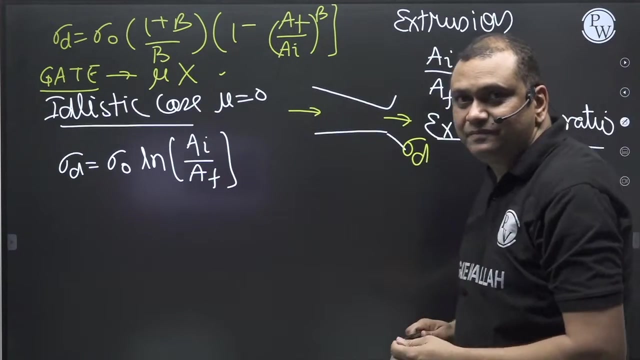 different version. what is the question? how much is the maximum reduction we can give to the material? if I draw, then what you are doing- this is the dye and incoming material, outgoing material- then you are pulling the outgoing material. you are pulling the outgoing material. this is what you are doing. 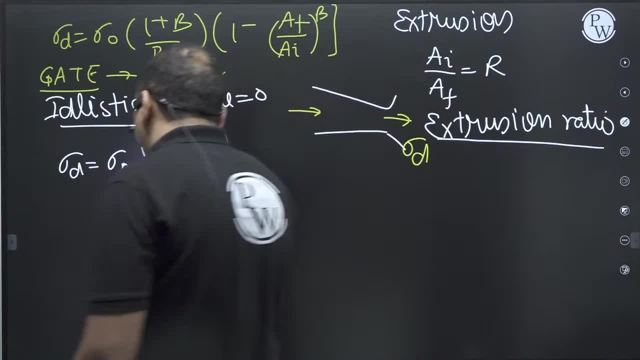 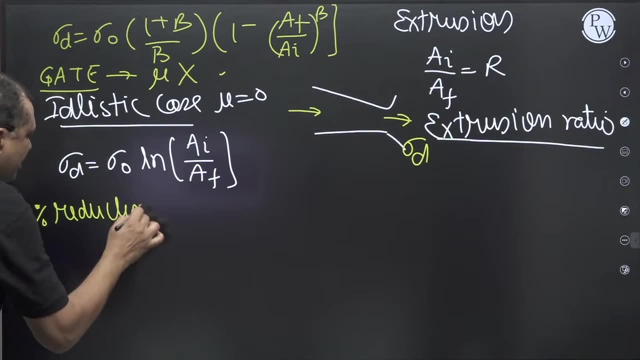 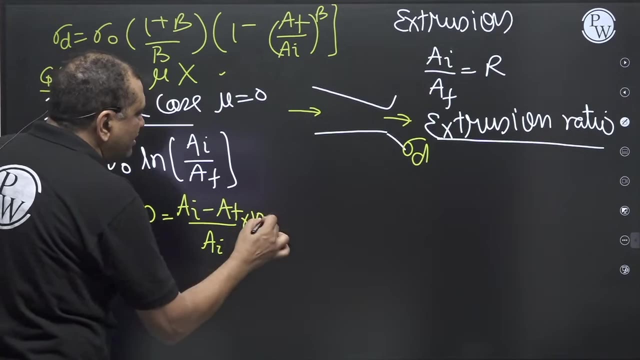 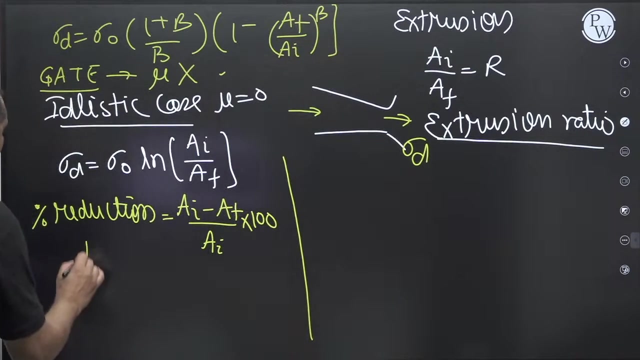 if I increase the percentage reduction of material, If I increase the percentage reduction of the material, What is percentage reduction? AI minus AF, divided by AI into 100, This is percentage reduction. If I increase this, If I increase the percentage reduction, Then drawing stress will also increase. 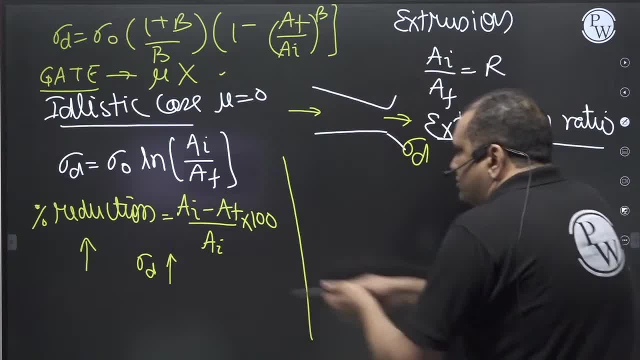 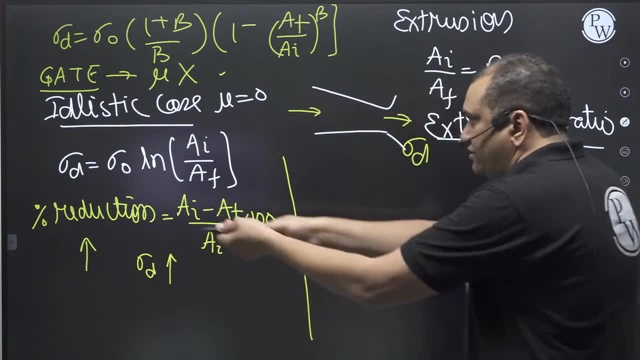 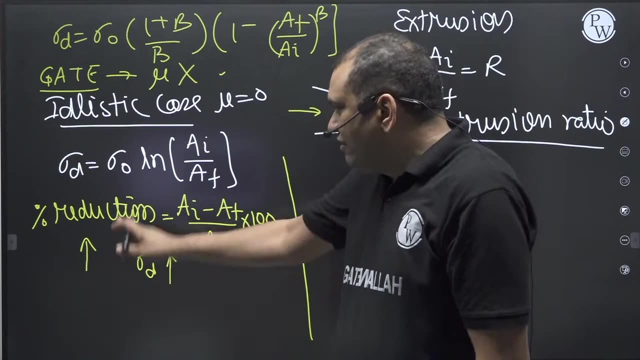 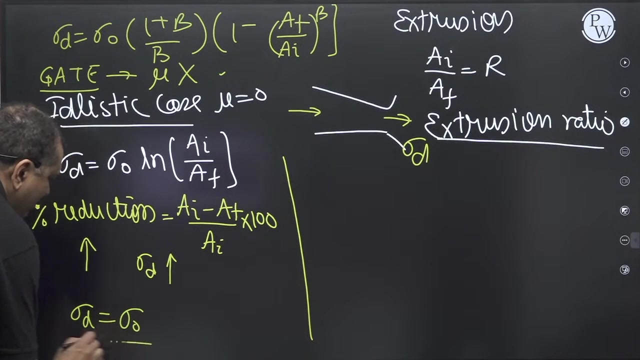 If I increase the percentage reduction, Then drawing stress will also increase. The stress from which you are pulling That will increase. If you increase the percentage reduction, Then the pressure from which you are pulling That will also increase. Correct Now, at a particular value of percentage reduction. If Sigma D is equal to Sigma 0, 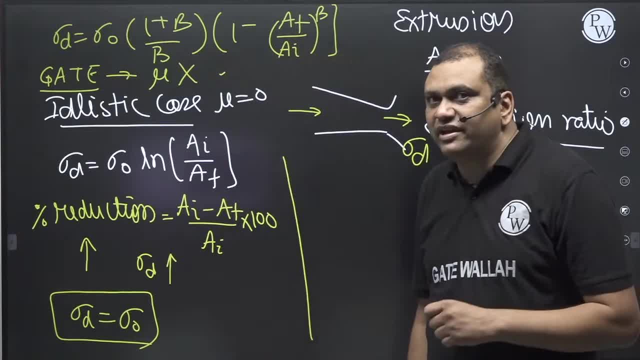 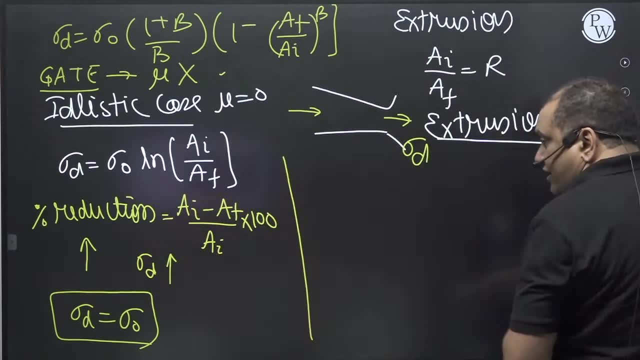 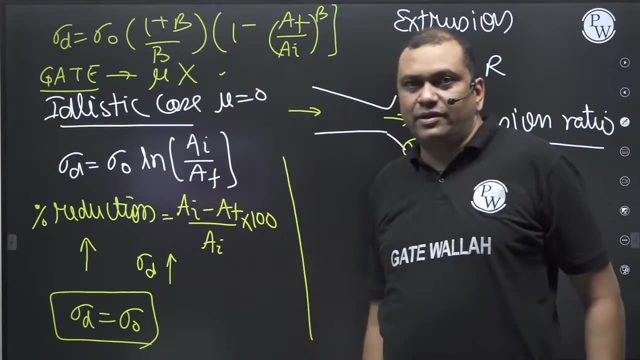 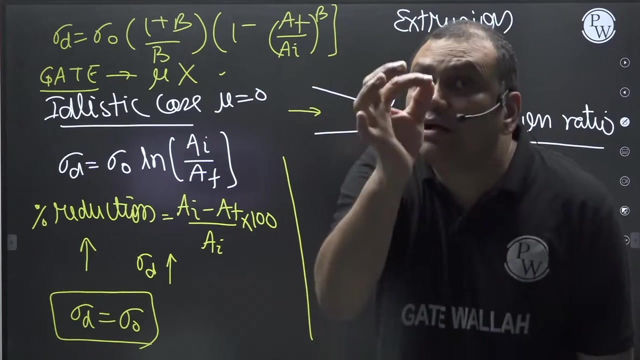 If Sigma D is equal to Sigma 0, Then the wire will not be drawn. You are pulling. As you pull, The wire will break. As you pull, The wire will break. You cannot draw. The moment Sigma D becomes equal to Sigma 0, You cannot draw, And this is called drawing limit. 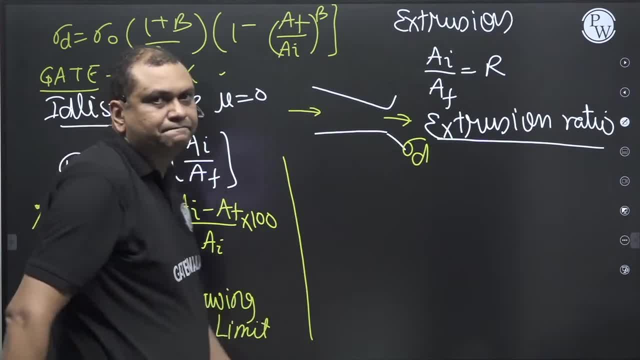 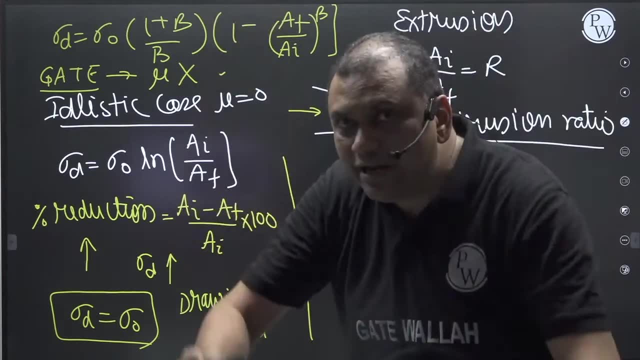 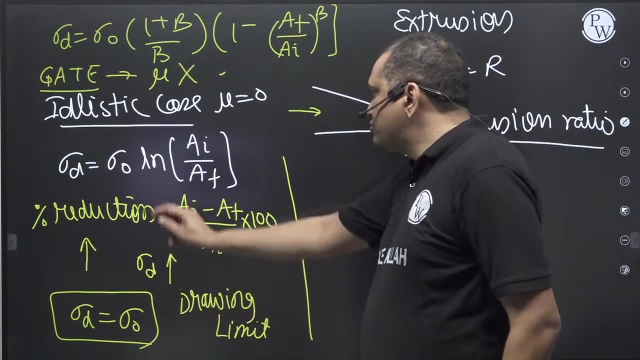 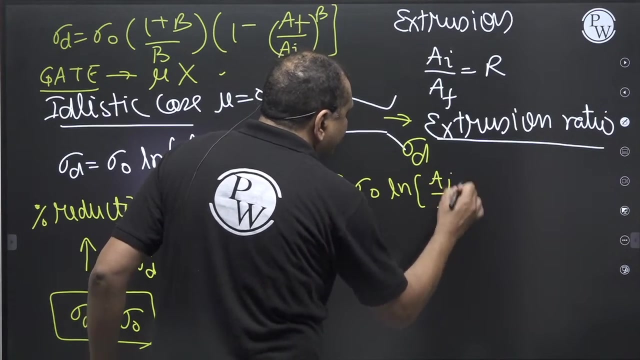 And this is called drawing limit. You cannot draw. The moment Sigma D becomes equal to Sigma D becomes equal to Sigma 0, You cannot draw. So Sigma D is equal to Sigma 0, Keep it here. It is equal to Sigma 0. ln AI by AF. Okay, 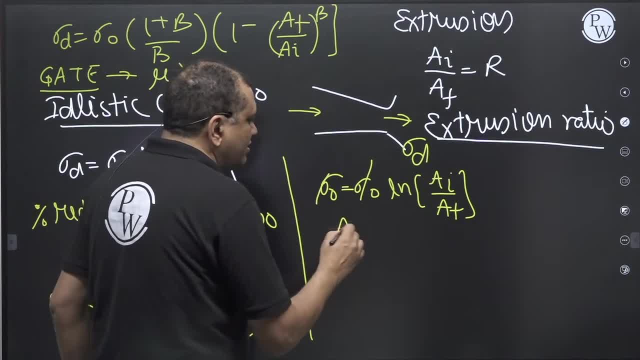 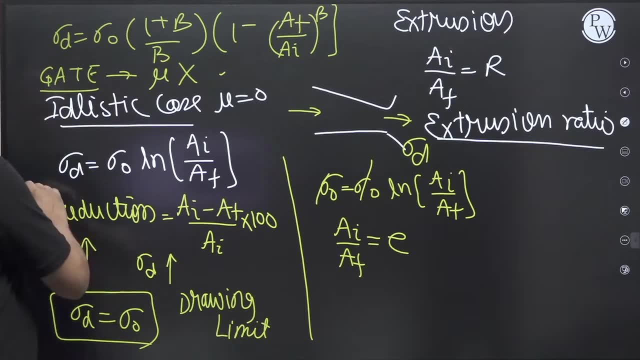 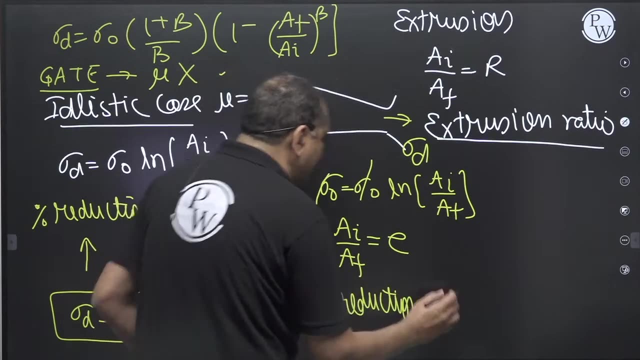 Sigma 1 and Sigma 0 have been cancelled. It will be cancelled. So can I say Sigma D is equal to E. If you take Nt log, then E will come. It is natural log. So percentage reduction: Maximum percentage reduction That can be given to the material. 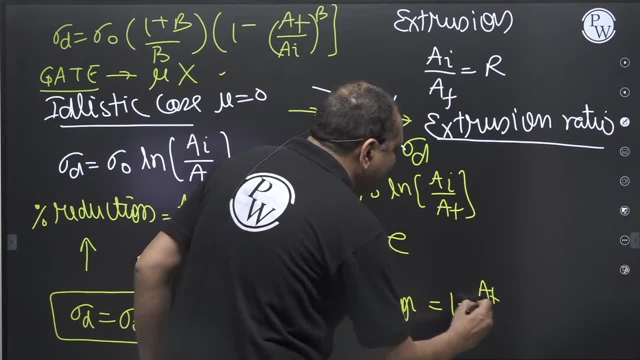 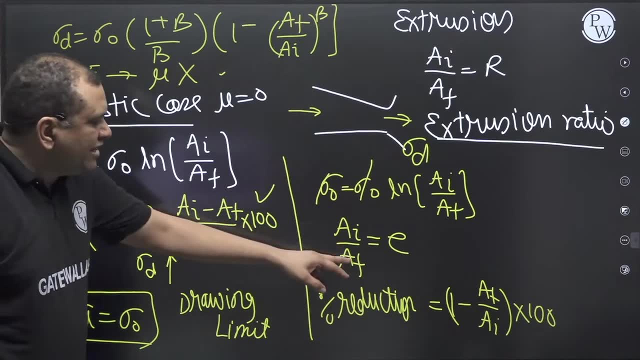 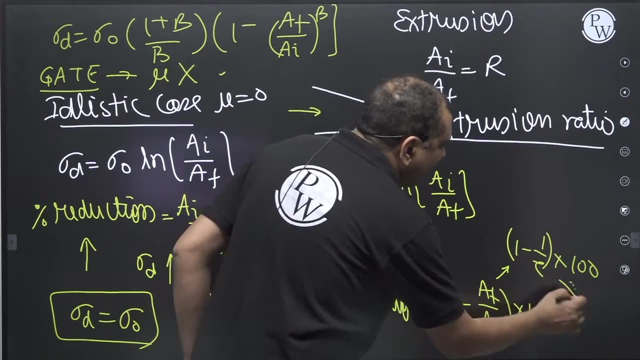 What is here? 1 minus AF by AI, 1 minus AF by AI into 100. This is it. AI by AF is E, So it is 1 minus 1 by E. So it is 1 minus 1 by E into 100, It is 63 percent. 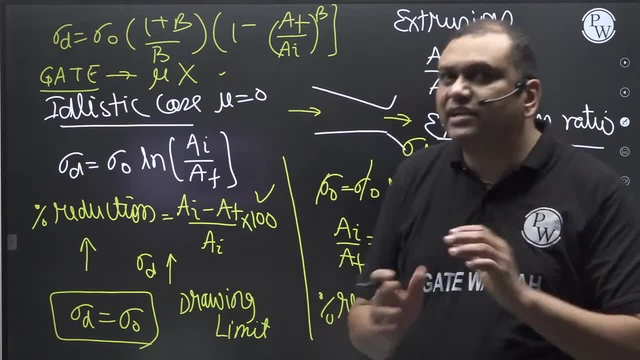 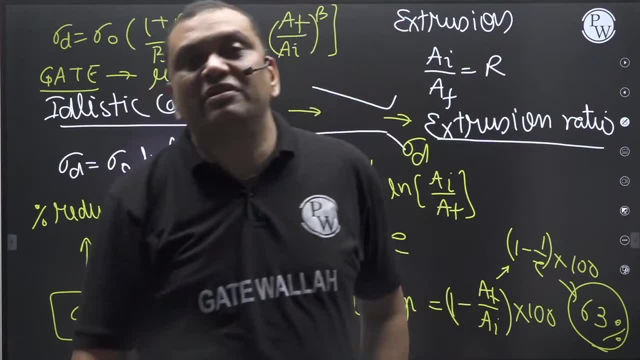 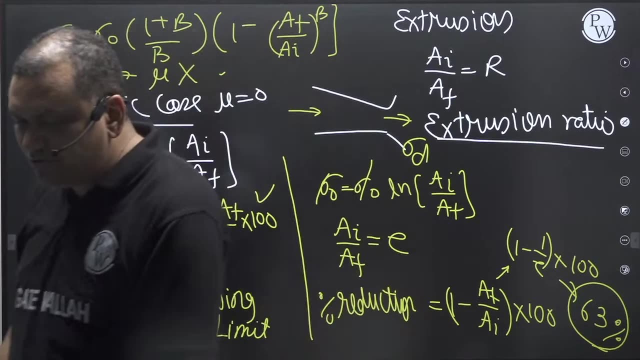 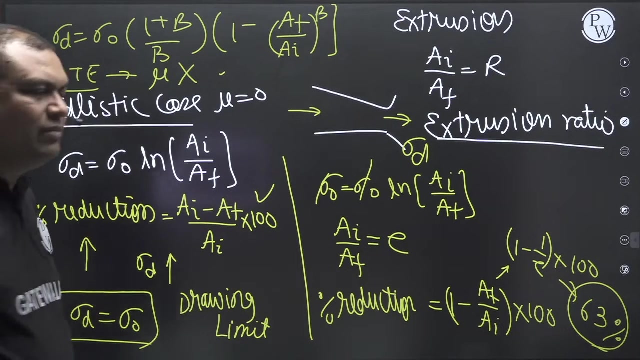 It is 60 percent. So in the most idealistic condition, So in the most idealistic condition, 63% reduction can be given To the material. Beyond that, We cannot give deformation. Beyond that, We cannot give deformation to the material. Everybody is okay. Everybody is ok. 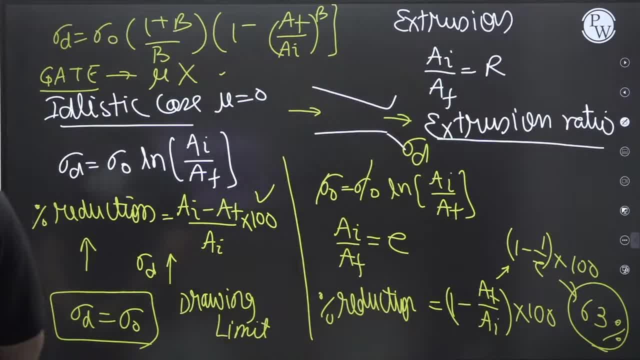 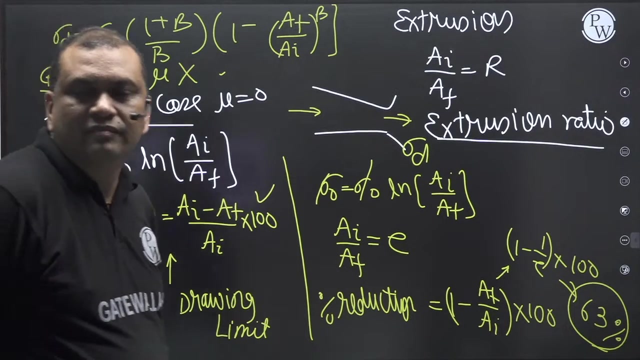 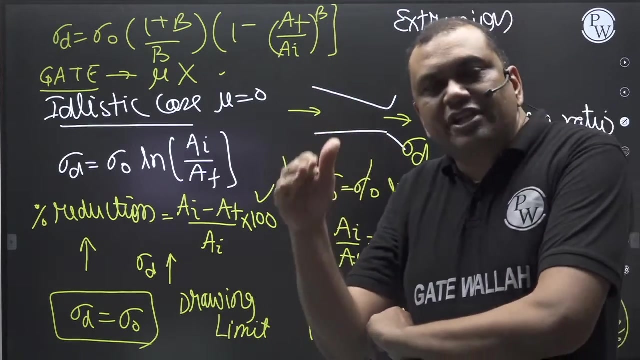 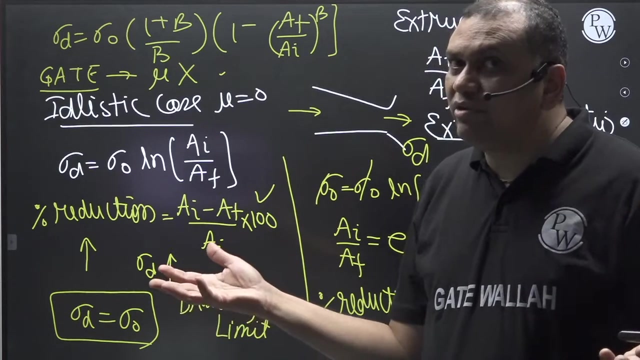 Everybody is ok. some chat box? yeah, you are correct, saumil mishra, you are correct. yeah, yeah, saiyan roy. look what is work hardening? piling of dislocation at the grain boundary that produces back stresses. that is called work hardening. so cold working man, so work hardening will be hot working. 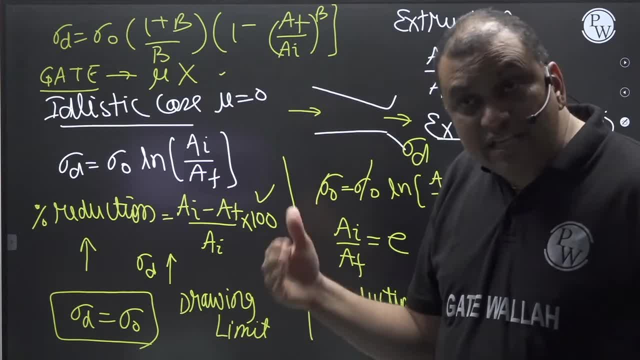 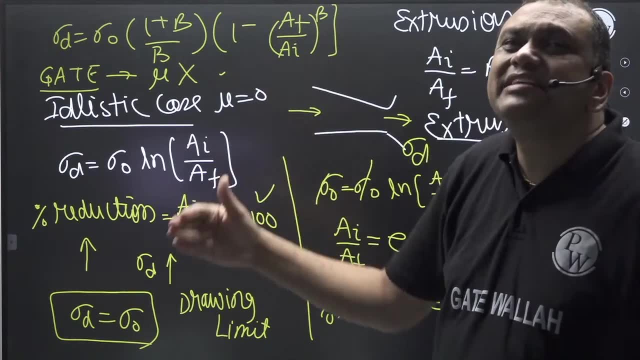 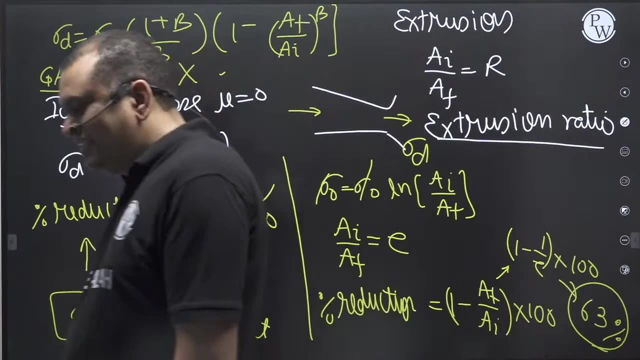 what happens? because the temperature is high so it will be hardening. so in cold working temperature is above recrystallization temperature. so our dislocation pile up the grain boundary, that dies out. so we say that there is no work hardening in the hot working. okay, i hope everybody. 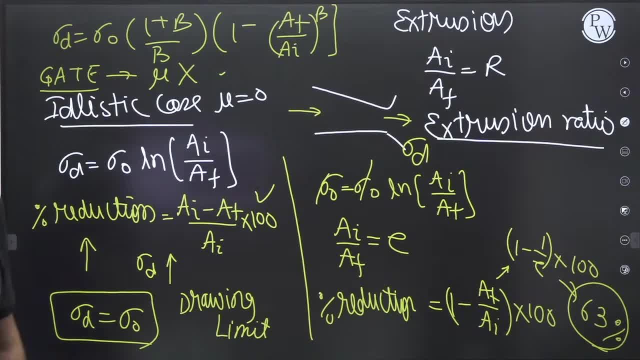 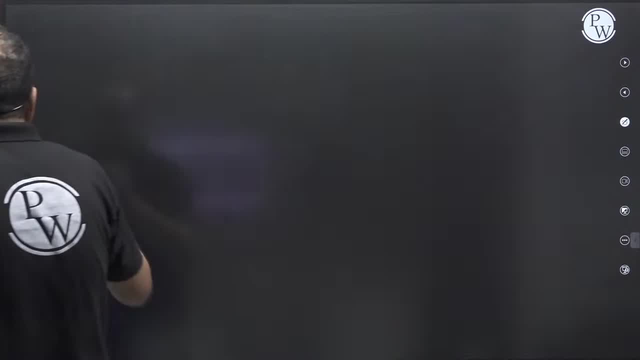 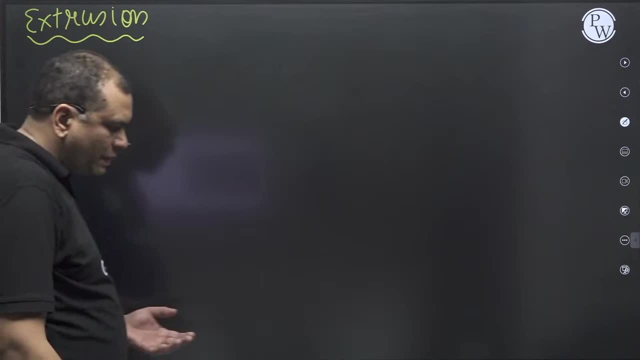 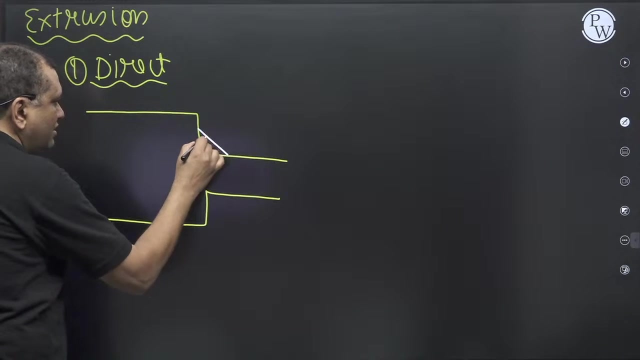 is okay now, nida basheer, i think you are also from kashmir, so now you see. little bit about extrusion. there are four types of extrusion process. one is called direct extrusion. in the direct extrusion there is a container and see, the die will be here. 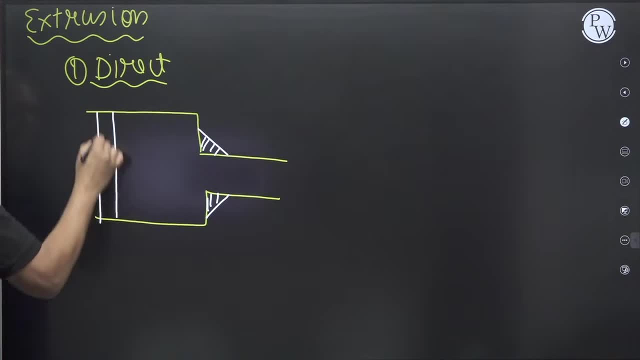 after this, when you have out from the container open, it will result into delicious product. so there are four types of extrusion. there is original extrusion and separate working system. also there is steel你是. there is solid. knowing all these principles off một of the Organization's is hard to understand because of so much answers, so i just say you. 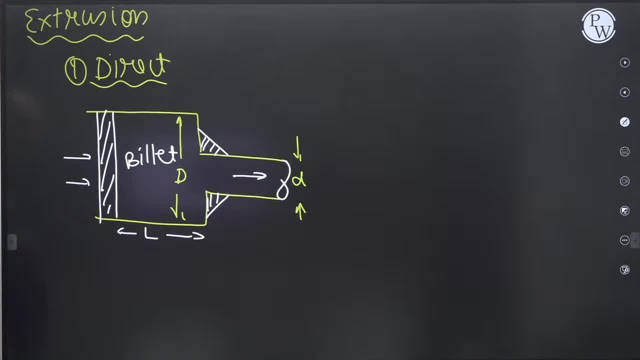 diameter of extruded part. so direct extrusion may kya hota hai extruded part comes out in the same direction as that of piston movement. jo maara extruded part hai, it comes out in the same direction as that of piston movement. ek hota hai reverse extrusion, sorry ek hota. 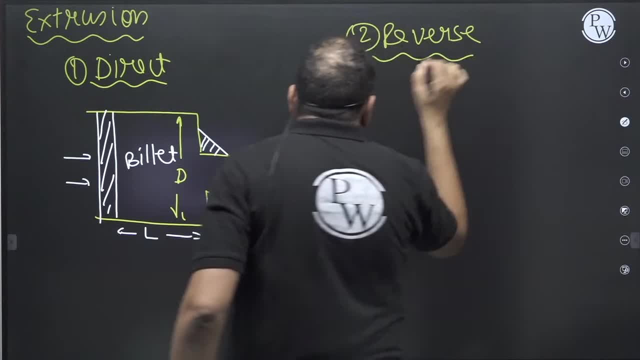 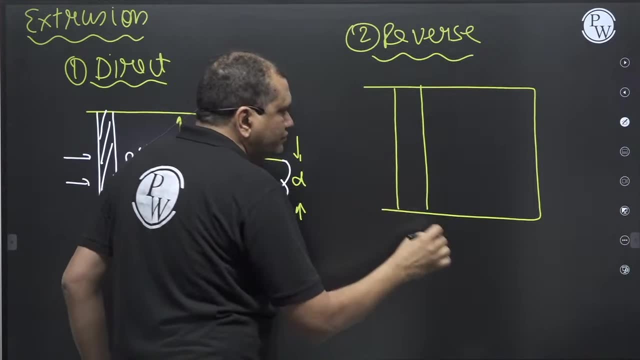 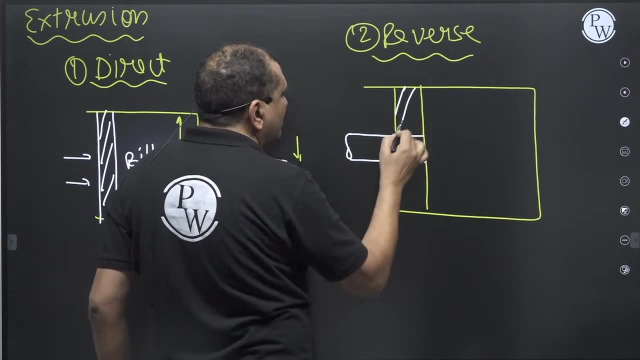 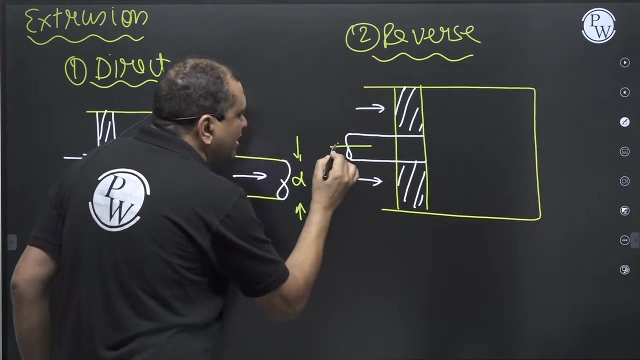 hai reverse extrusion, reverse extrusion me kya hota hai. hamari jo die hoti hai, die piston me hoti hai. hamari dekho, yeh hamara piston hai, isse aise press kar raha hai aur extruded part opposite direction me aata hai. this is the black. 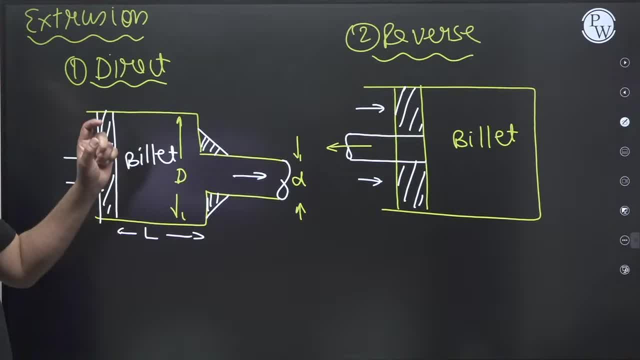 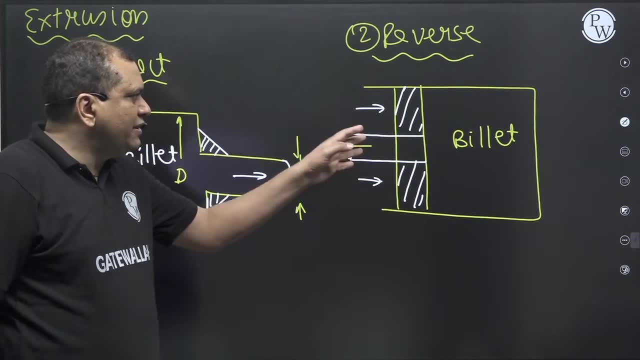 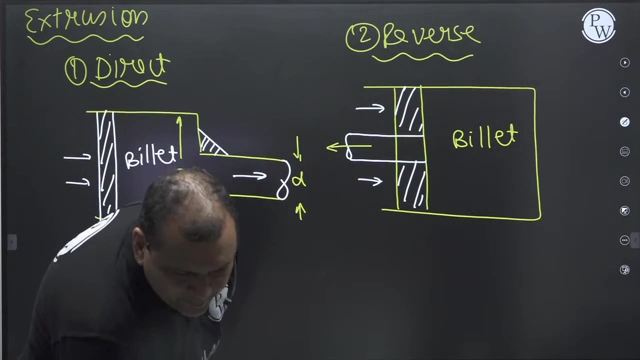 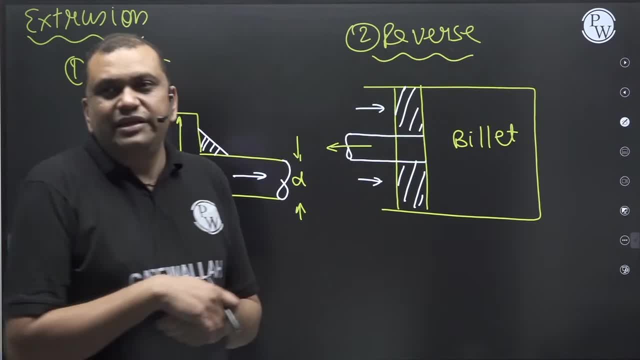 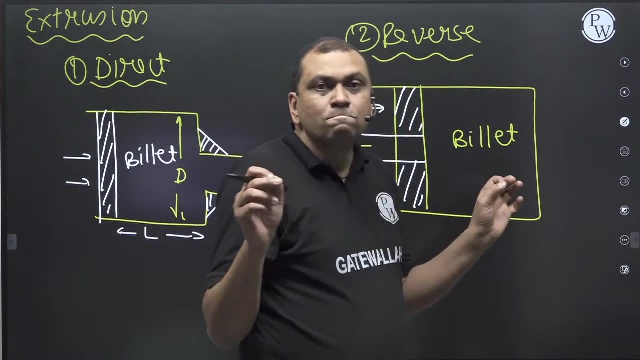 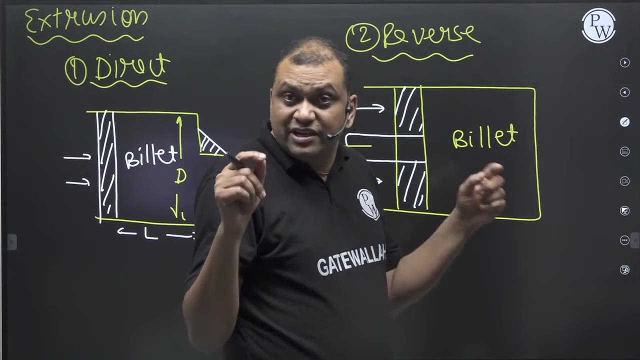 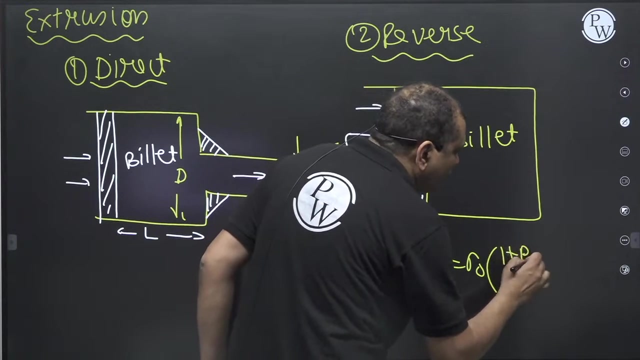 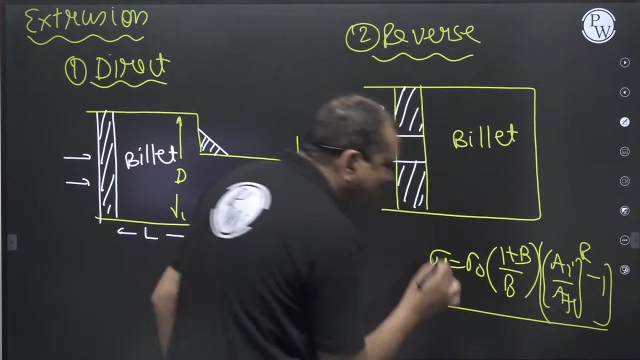 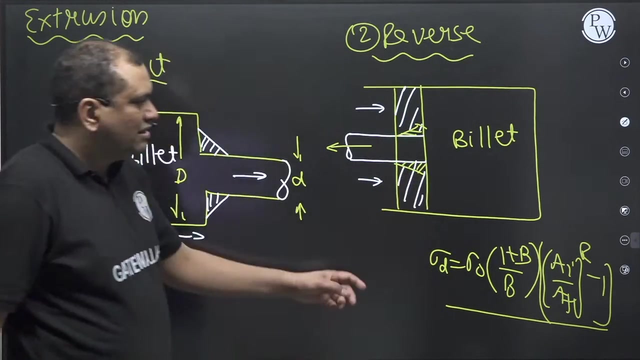 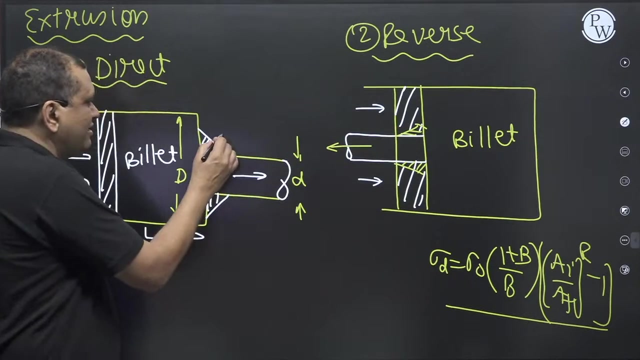 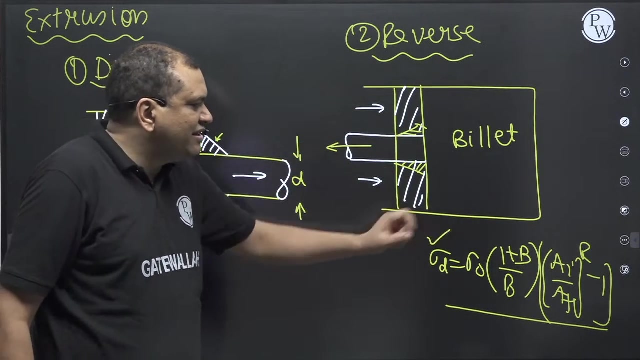 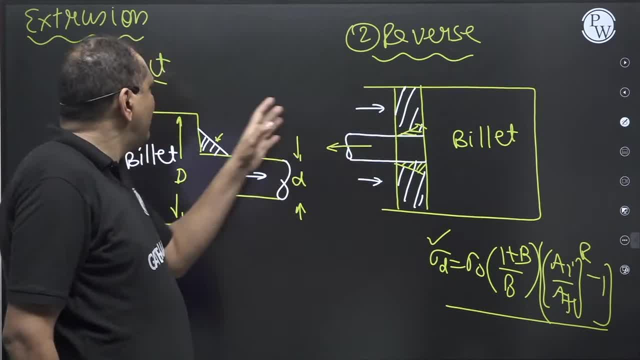 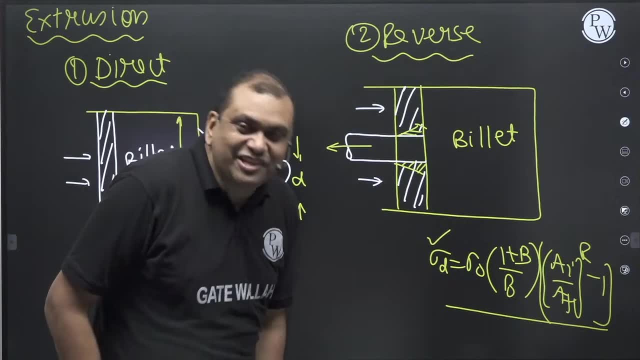 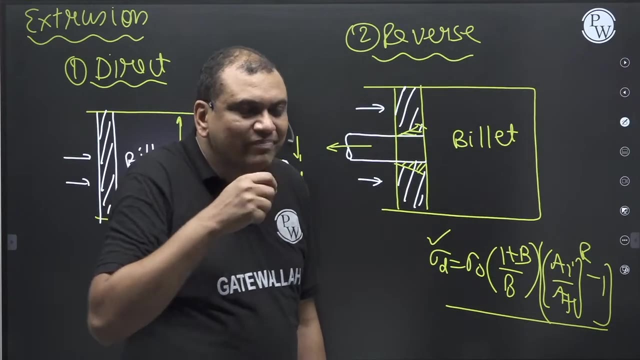 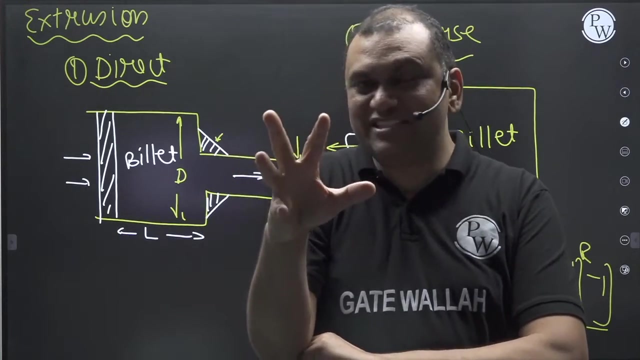 and both will be same, reverse and direct. both need this much energy for deformation in the die, but in direct extrusion a little additional energy is required. as far as deformations, once again here, please don't get confused here. these are very important things. 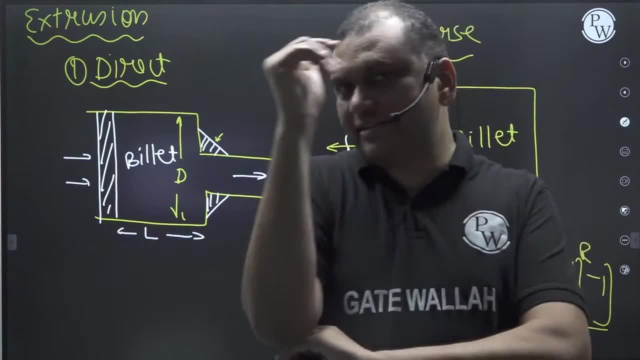 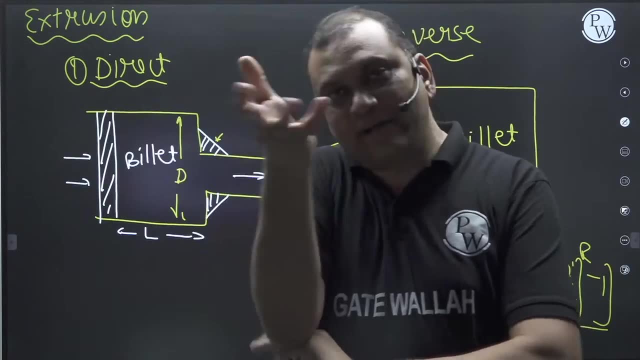 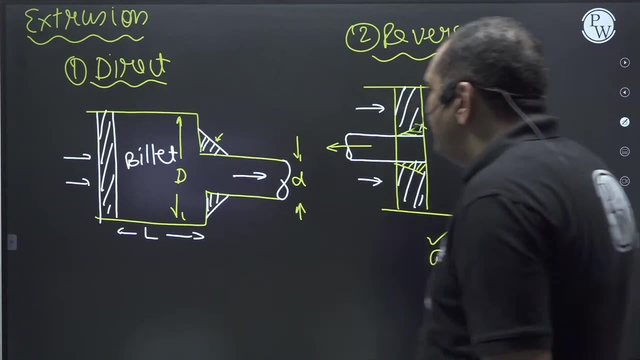 as far as deformations in the dies are concerned, forward and backward extrusion, sigma d will be same. if alpha and mu are same, then both will be same. but in forward extrusion when you are moving the piston, so entire billet is moving in the drum. 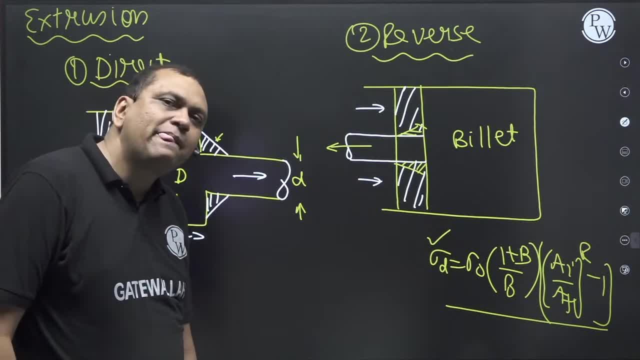 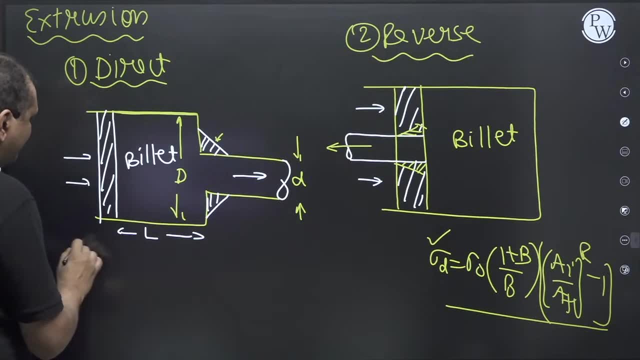 entire billet is moving in the drum, entire billet is moving in the drum. so this friction, friction between the billet and drum, friction between billet and drum. because of that on the piston you need to apply additional pressure, sigma f, because in billet and drum there will be friction. 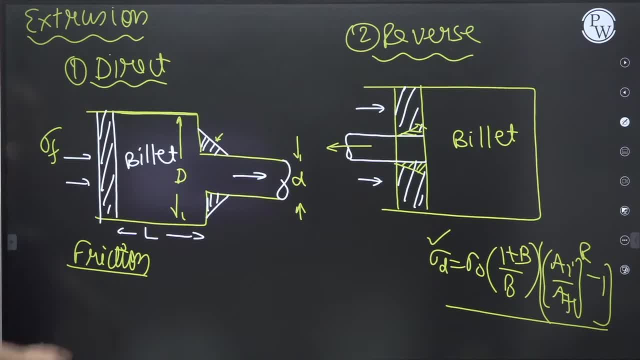 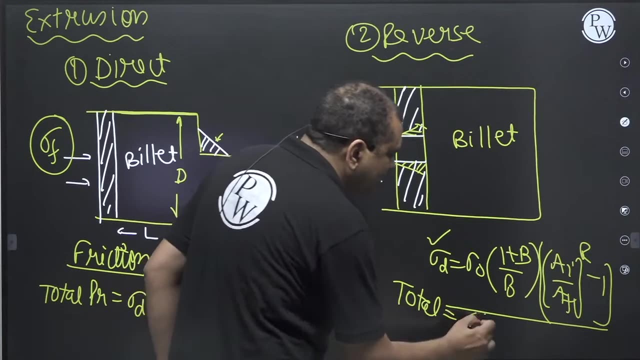 to overcome that, you need to apply, you need to apply additional pressure- sigma f, so the total pressure will be sigma d plus sigma f, and here only sigma d will remain, here only sigma d will remain. so that's why more energy is required in forward extrusion. 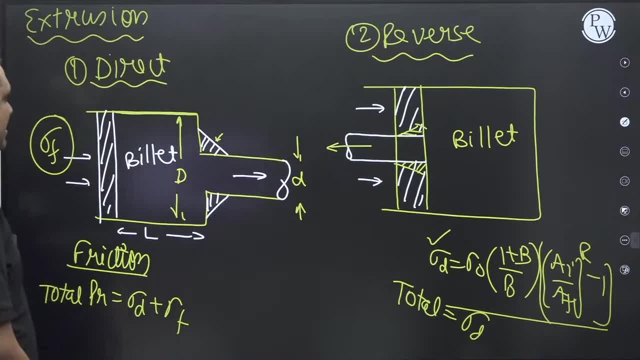 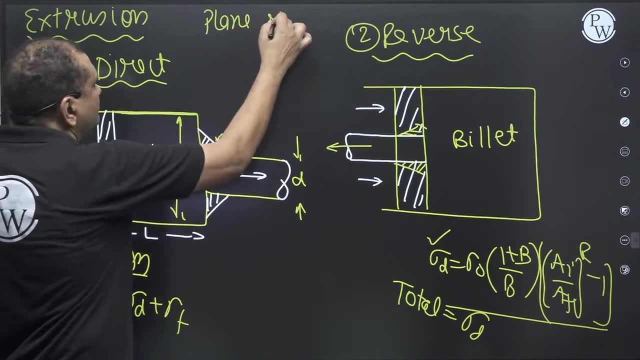 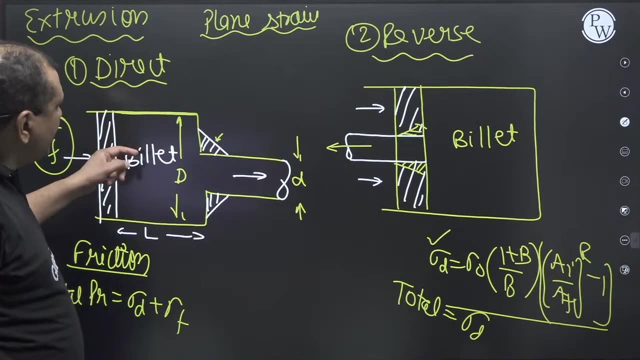 not in backward extrusion. so how will this sigma f come out? this is our plain strain case. this is our plain strain case. plain strain means. plain strain means what is plain strain? I don't want to study much in this cycle. I don't want to study much in this cycle. 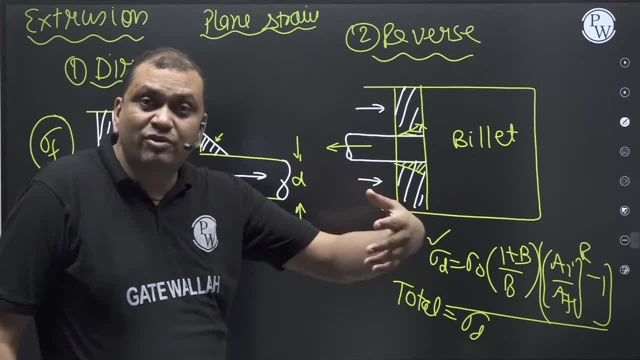 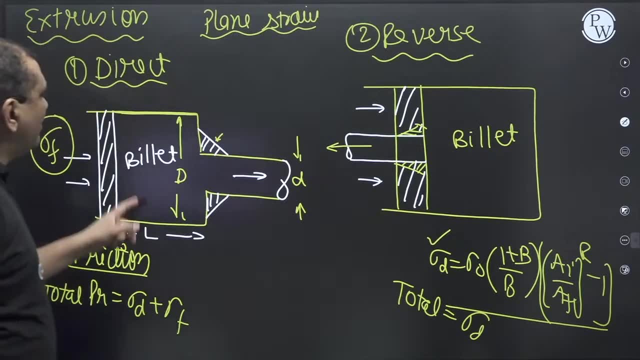 because actually, if we had full time, if we had full time, then we would have talked for half an hour, then we would have talked for half an hour. our billet will not come out. our billet will not come out. so this side movement is restricted. so this side movement is restricted. 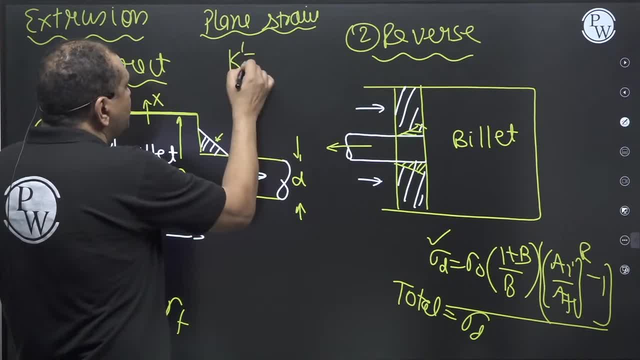 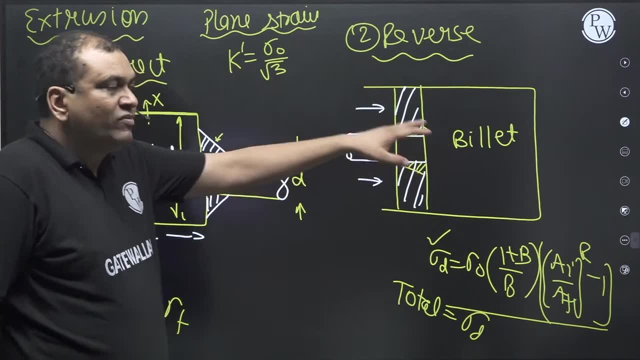 so it is a plain strain case. so yield strength in shear is nothing but. so yield strength in shear is nothing but sigma 0 by root 3. sigma 0: we will get out from the same procedure, so k dash will be sigma 0 by root 3. 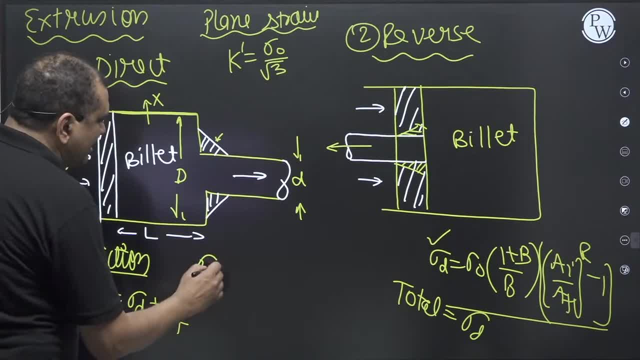 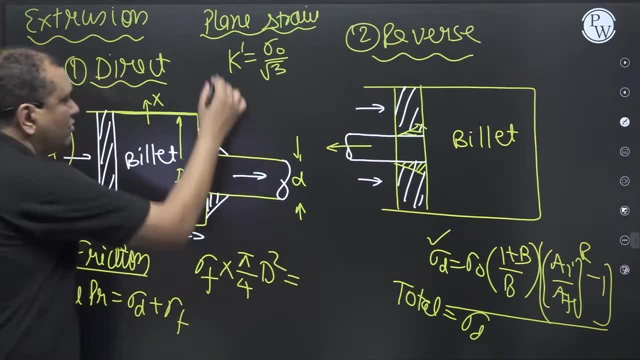 so k dash will be sigma 0 by root 3. so how will we get sigma f out? equalize the force. sigma f is equal to pi by 4 d square. this is the force and according to plasticity k dash, how much is the friction area? 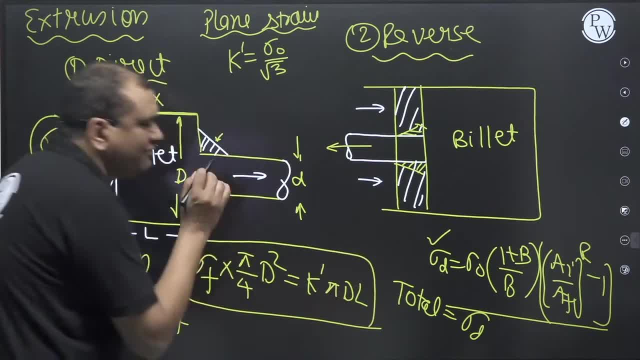 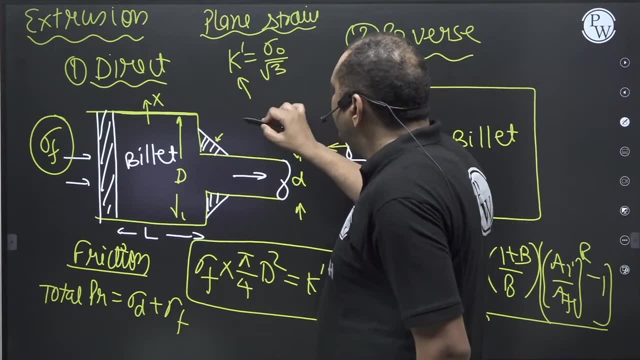 pi dL. you will get sigma f out from this. you will get sigma f out from this. so take a look at this. we have done four sequels. k dash is the yield strength in shear. we have done four sequels. k dash is the yield strength in shear. 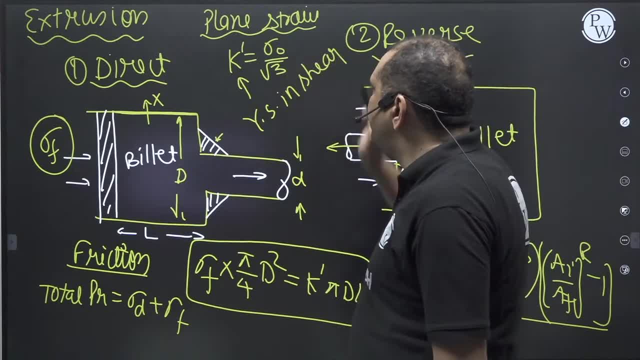 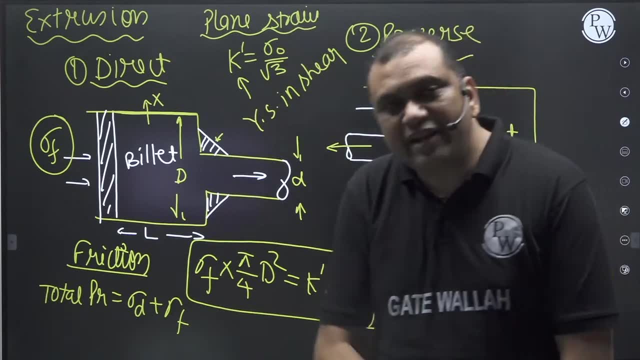 and because it is a plain strain case, k dash will be sigma 0 by root 3. if it was a plain stress, if it was a stress hypothesis, then k dash will be sigma 0 by 2, but it will be sigma 0 by root 3. 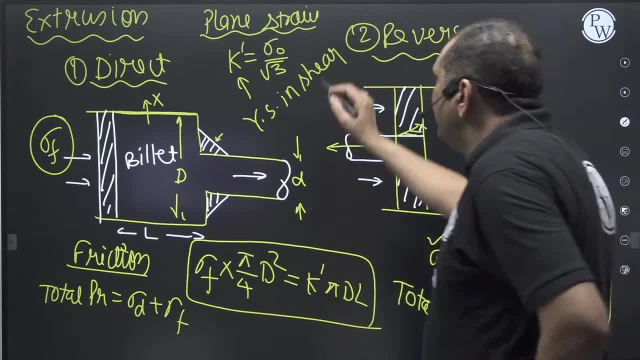 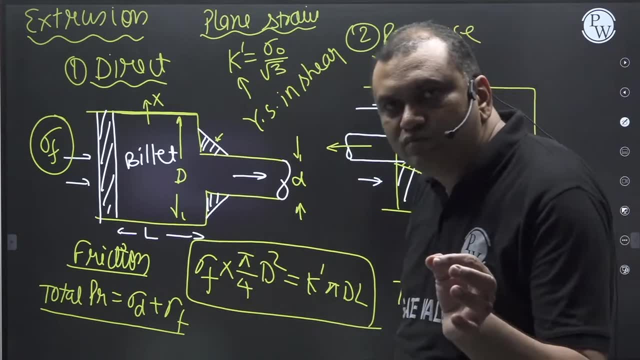 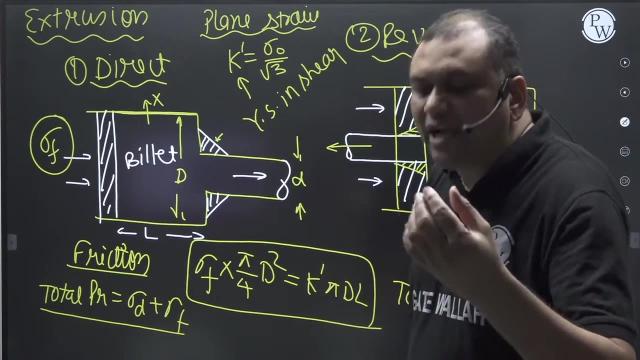 because it is a plain strain case. but it will be sigma 0 by 2 because it is a plain strain case. so the total pressure will be sigma d plus sigma f. is this good in direct extrusion? we need more energy to form in backward extrusion. 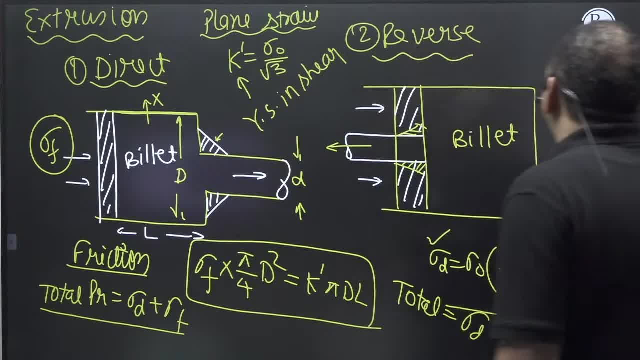 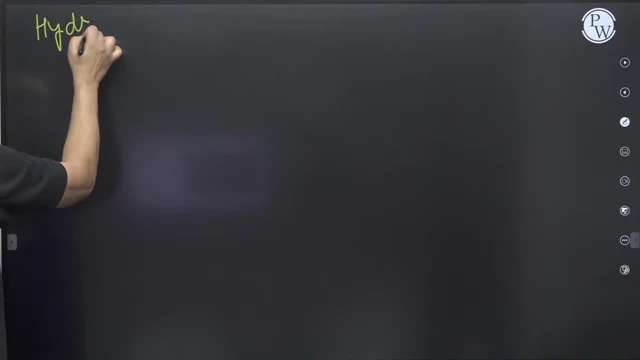 we need less energy to form in backward extrusion now. there is something called hydrostatic extrusion. there is something called hydrostatic extrusion here. look at me for 5 minutes here. look at me for 5 minutes here. look at me for 5 minutes. 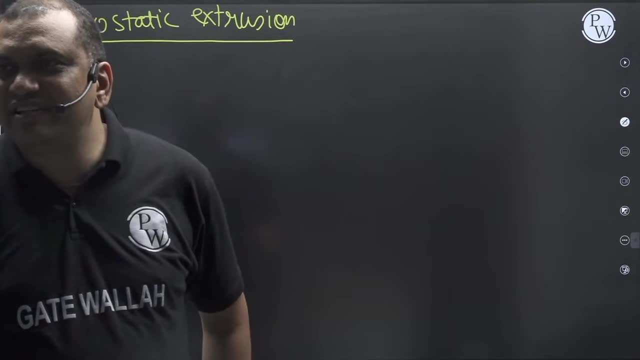 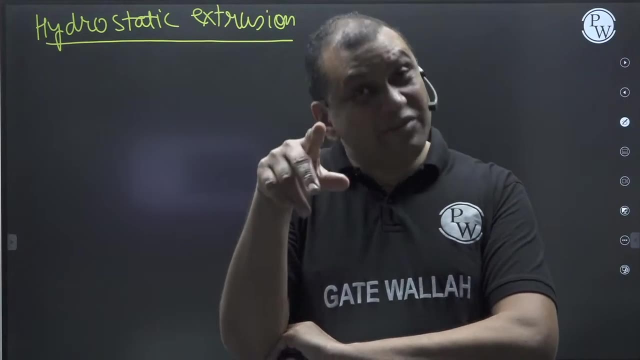 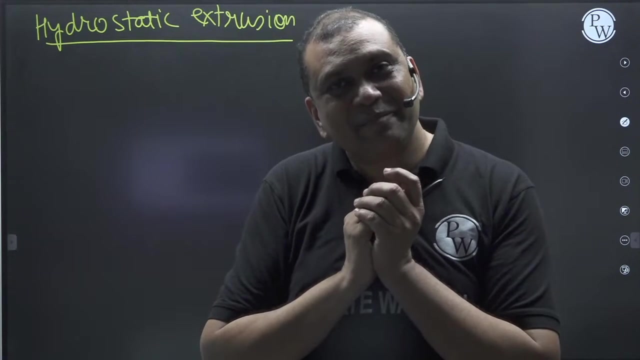 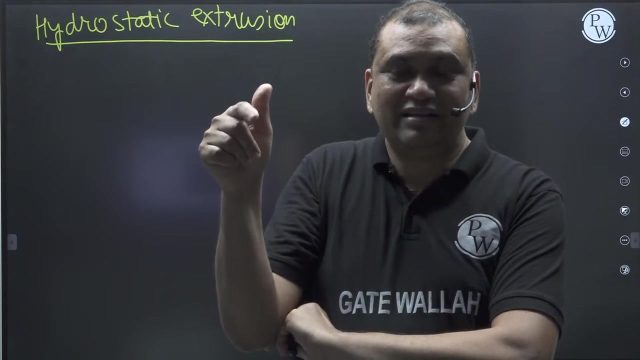 no, no, wrinkle friction also generates in reverse extrusion. listen, listen, see, there will be friction in di. there will be friction in di. we have considered it in sigma d. we have considered it in sigma d, but there is an additional friction in direct extrusion: friction between billet and drum. 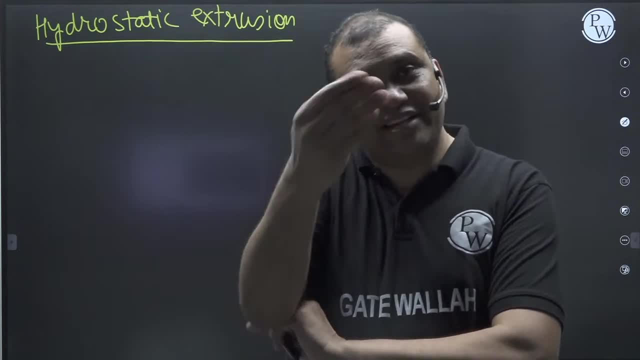 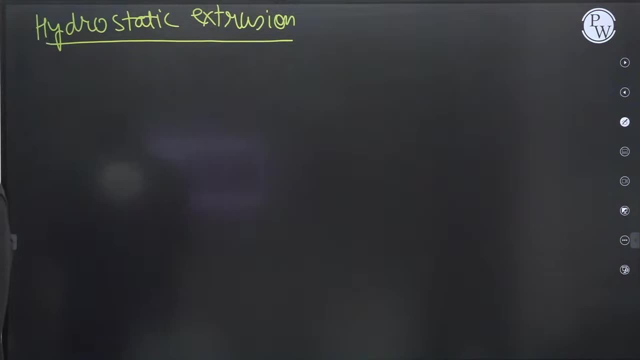 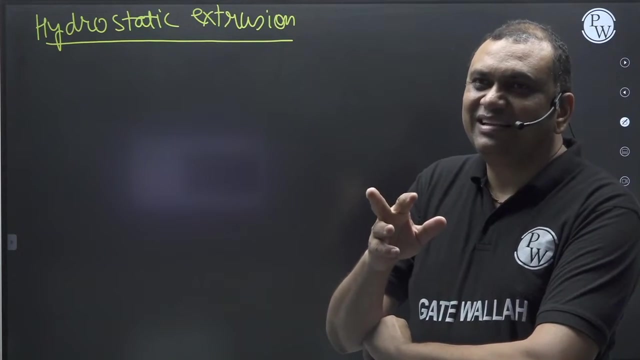 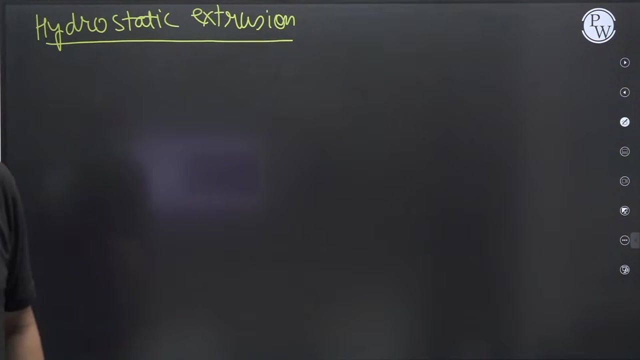 not in backward extrusion. in backward extrusion, billet is stationary or in sommel memoria. our boundary condition has changed. that's why the expression is the same. very good, i have 8-10 questions, but i want to do the theory. we will not do it randomly. 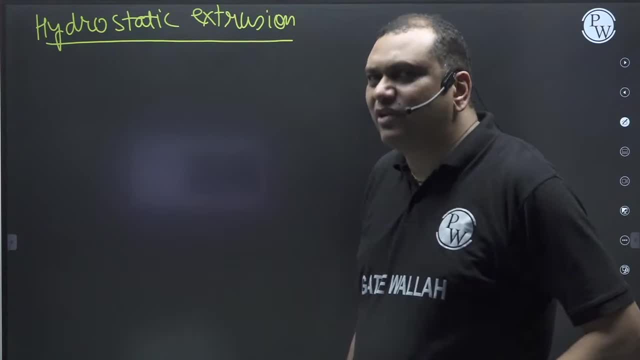 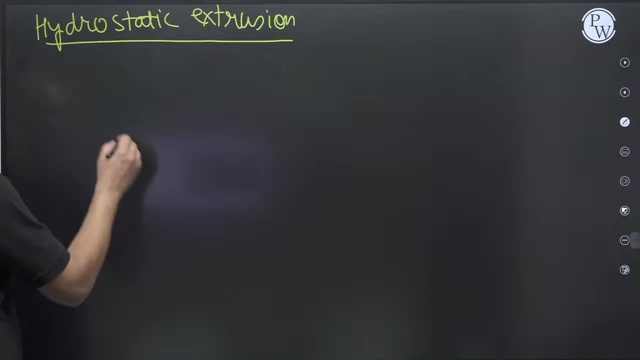 we will not do it in a system. we have 4 days. we will do the theory tomorrow. what is the problem? why are you taking tension? it is my tension. what i have to do, it is my tension. what is hydrostatic extrusion? what is the problem? 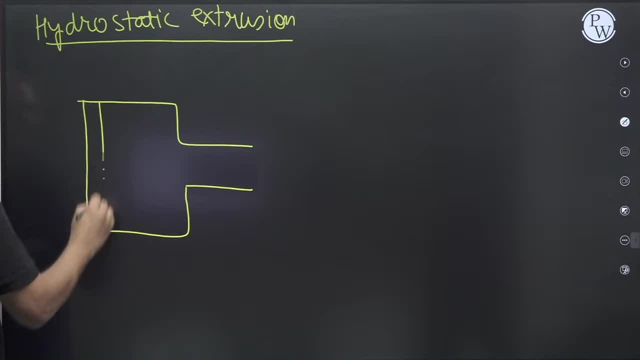 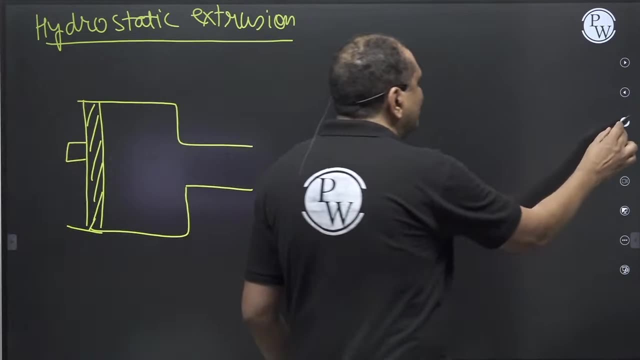 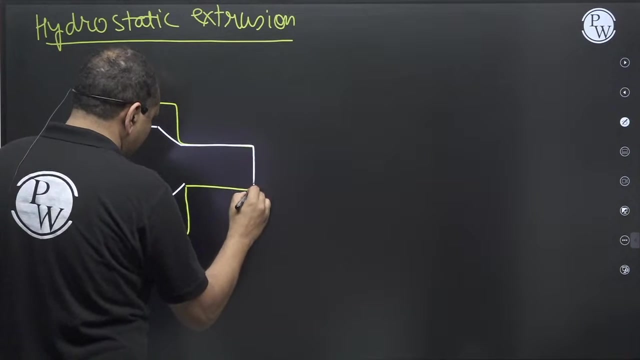 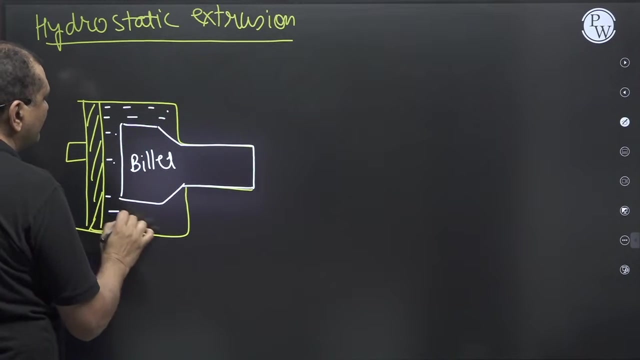 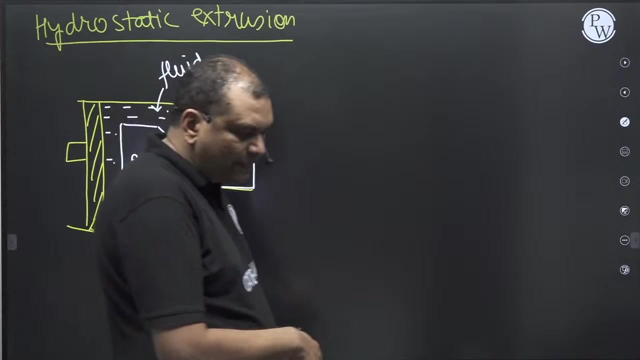 this is the most confusing question. this is your piston and this is your billet. this is your billet and this is filled with oil, hydraulic fluid. so our piston is not directly applying pressure on the billet. it is applying pressure through a hydraulic fluid, this hydrostatic extrusion. 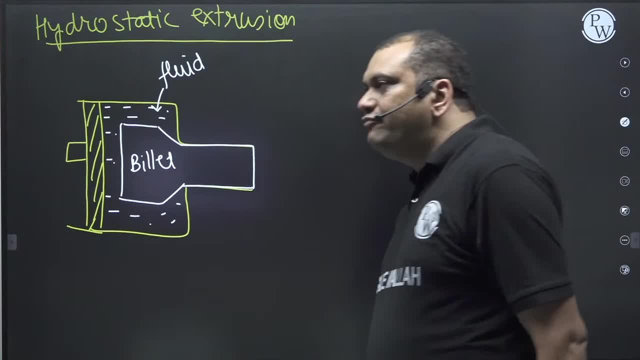 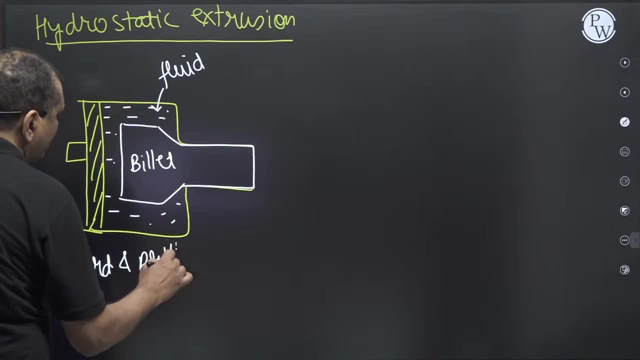 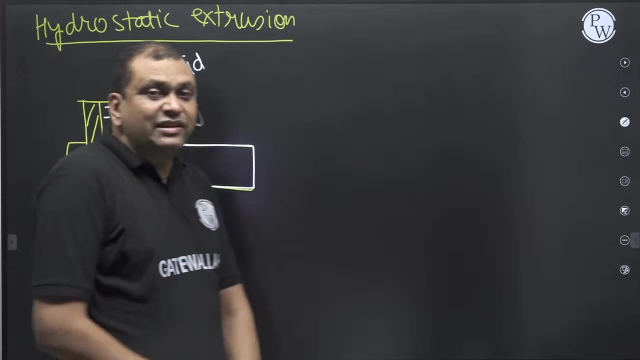 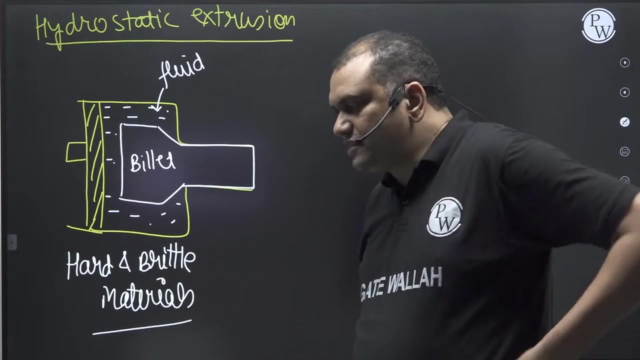 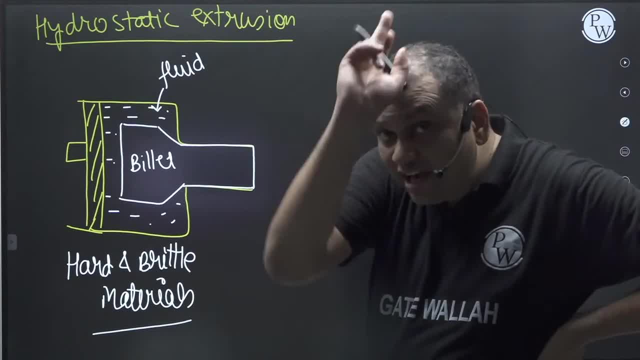 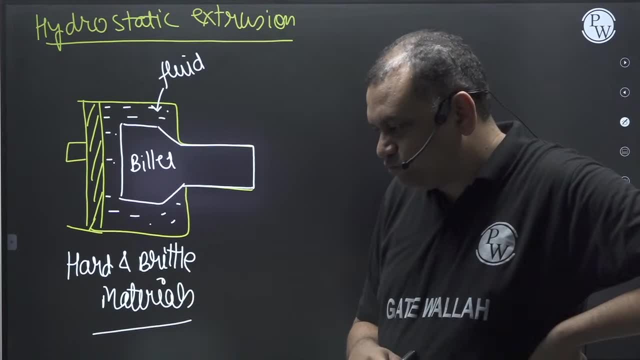 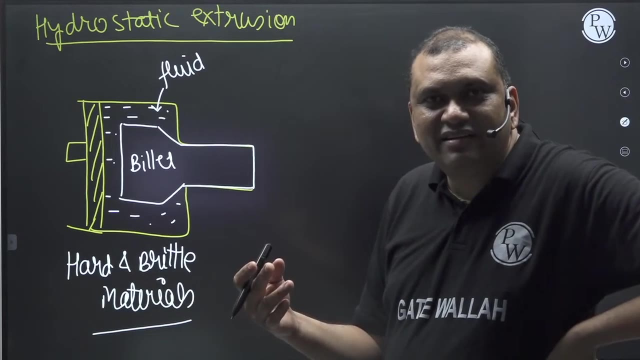 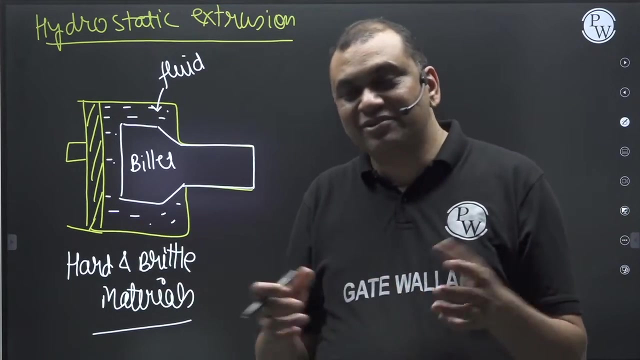 hydrostatic extrusion is meant for hard and brittle materials. now, unfortunately, do you know what some teachers teach? that in hydrostatic extrusion brittle material. why do they form? in brittle material there is a crack, so the crack closes with pressure. unfortunately, this is written in any book. 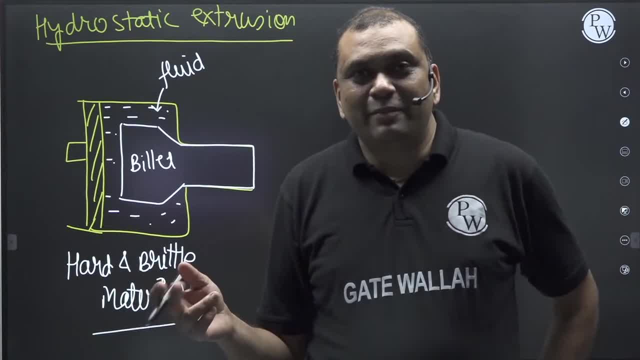 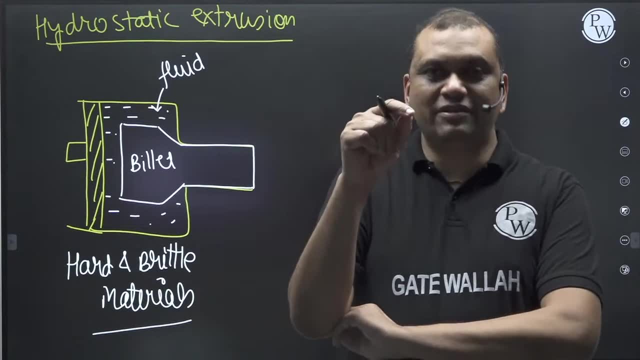 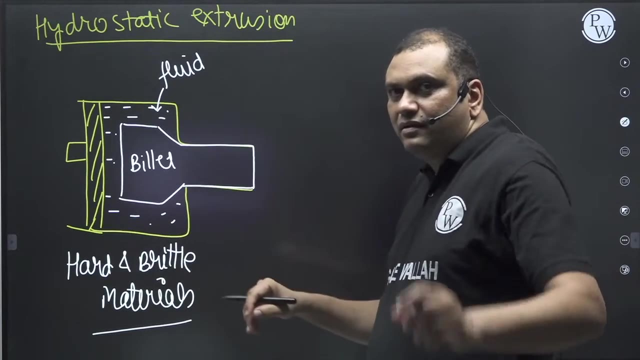 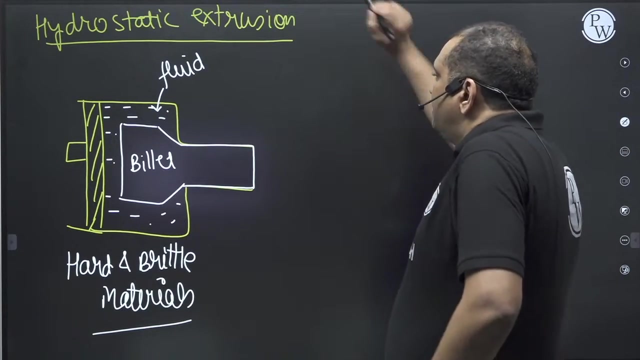 unfortunately, this is wrong. actually, I am telling you the answer and I also understand that 90% of the people will not understand the answer, so you have to take a break. I am telling you the answer in two minutes. if you don't understand, shoot me. look at our history. 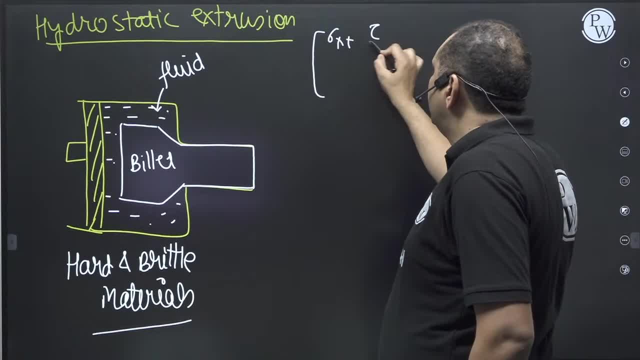 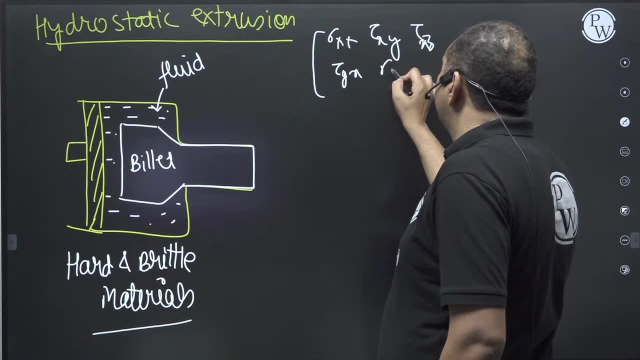 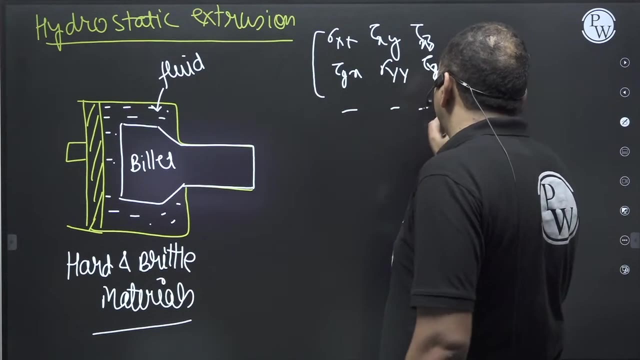 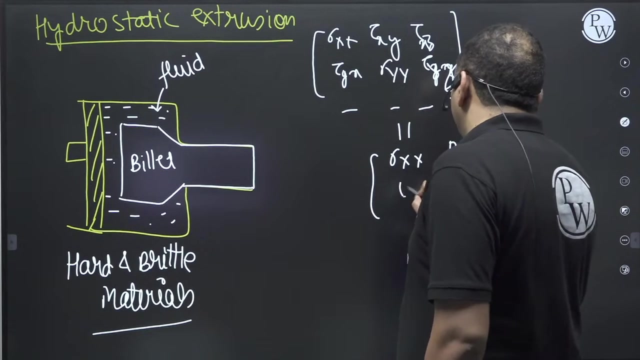 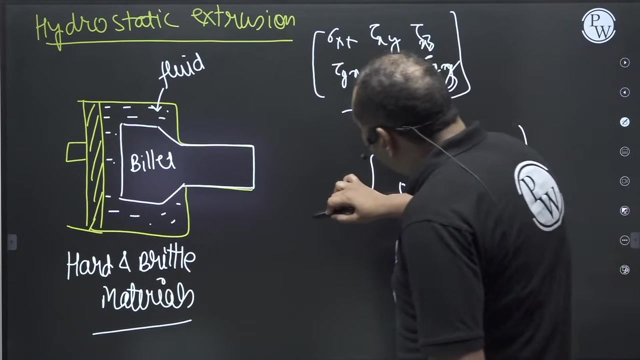 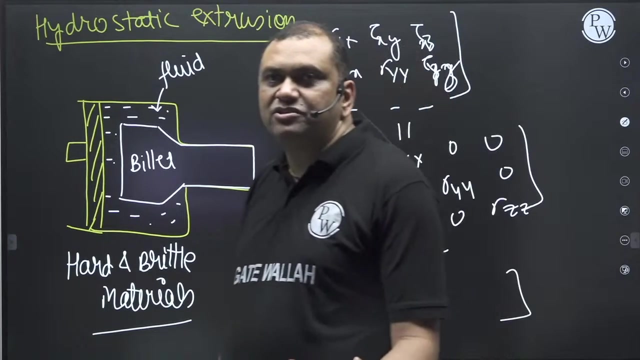 now look at this, but then I will give you a video on this. you will understand like this: for example, zero Sigma said that you're the hydrostatic and plus deviator component. yes, 10th of materials. map detail in putting in Chicago or agar up kobe. 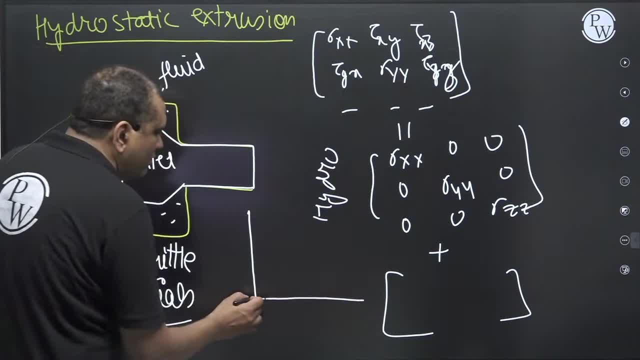 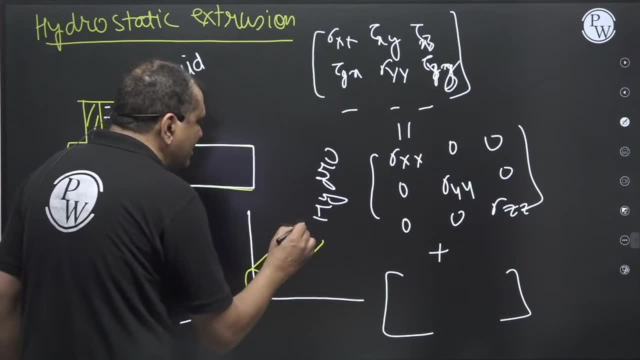 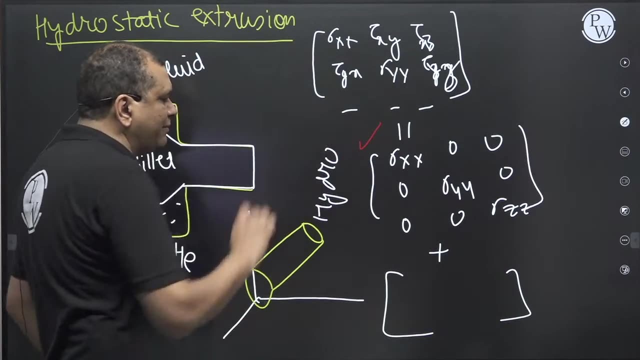 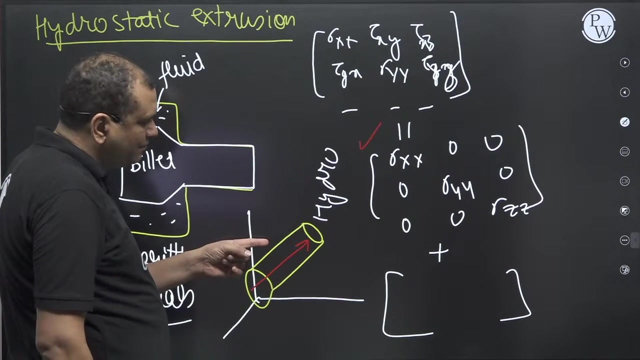 theory of plasticity. they can. I have the three dimension manner theory of plasticity. yes, I want my sister, so I want my sister under hair. take a. so, Joe Hamara, hydrostatic component hair that is acting along the longitudinal direction of the one my sister under, or the. 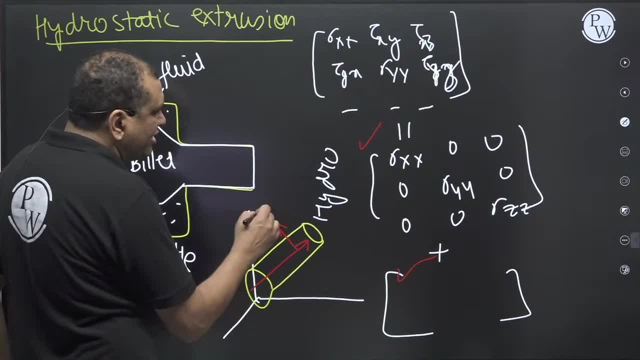 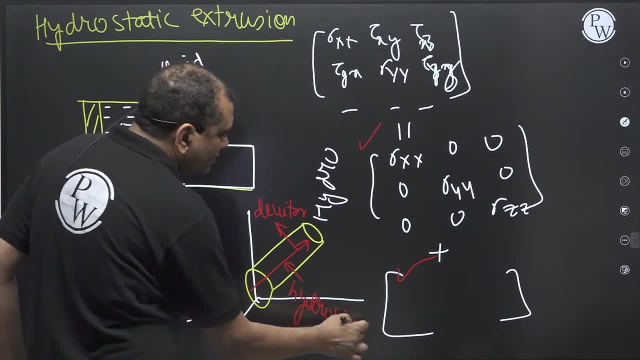 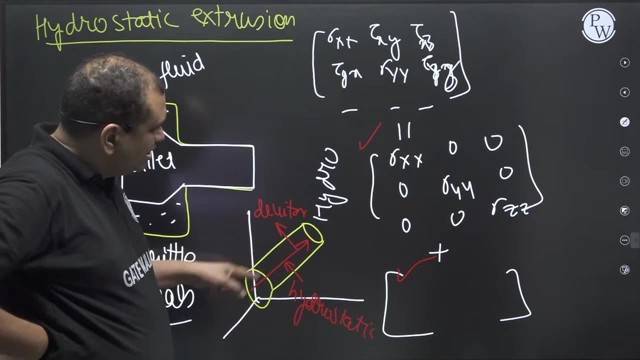 deviator component hair. it is in the radial direction, your deviator component, a very hydrostatic component hair. so they give us make a hotel hair. Hamara, plastic deformation, Hoga job. Hamara, resultant cylinder surface by Jagga, so bottom key, a bat agar, a hydrostatic component. Jada Hale LL and. 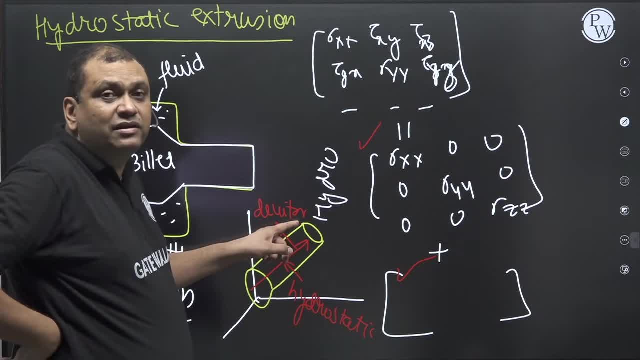 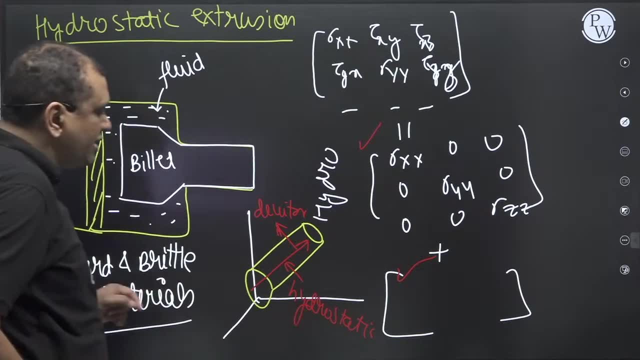 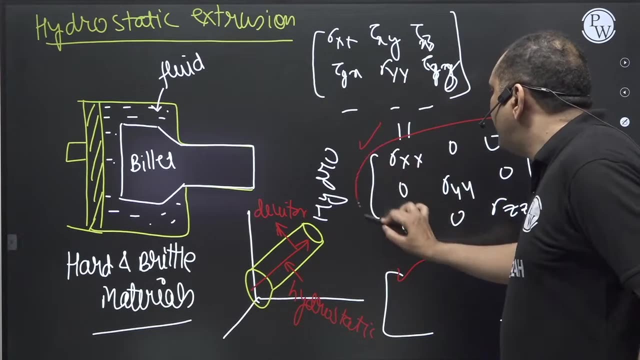 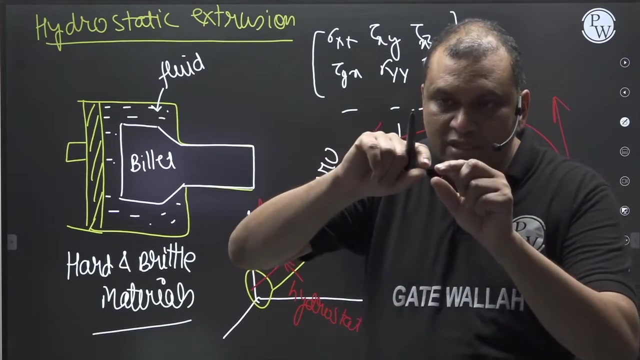 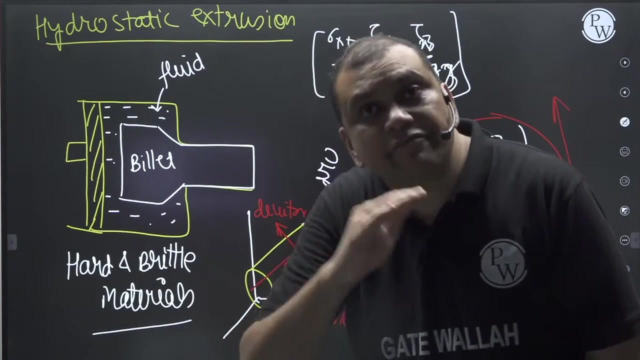 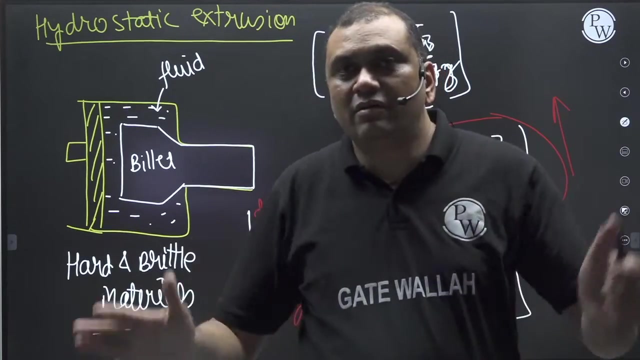 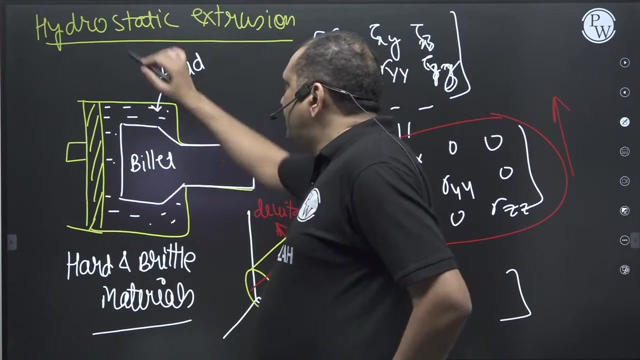 Jada, hair material undergo large deformation before it fractures. so it's my ham, hydrostatic pressure Laganese, kakakata ham. if we apply hydrostatic pressure Laganese, I saw me go get a mask. cracks go right away. so you got a big lot interpretation, but actually after exam, Kelly up in a rut, low that. 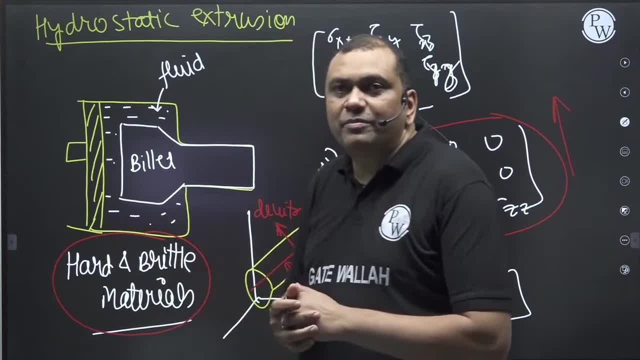 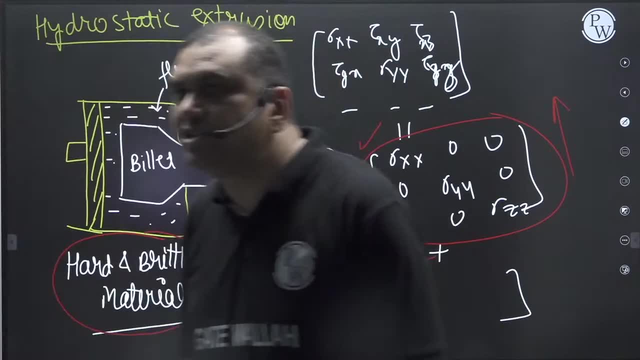 hydrostatic pressure. Laganese kakakata ham. if we apply hydrostatic pressure, Laganese kakakata ham. if we apply hydrostatic extrusion is meant for forming hard and brittle material. okay, now, yeah, deviator along the radial. now they're bashing, you are correct. so hydrostatic. 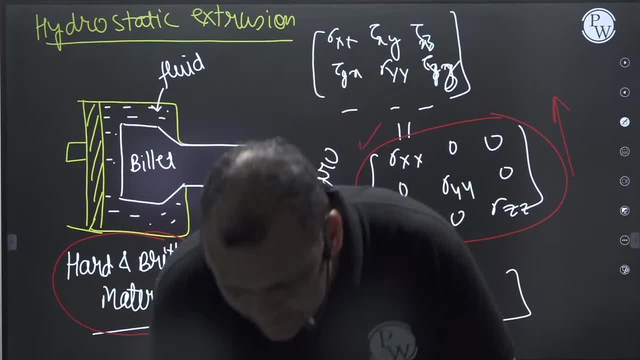 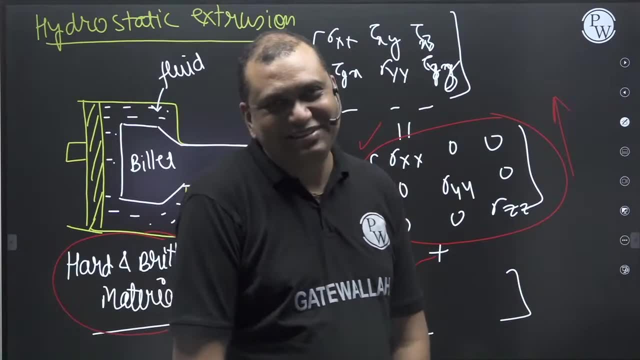 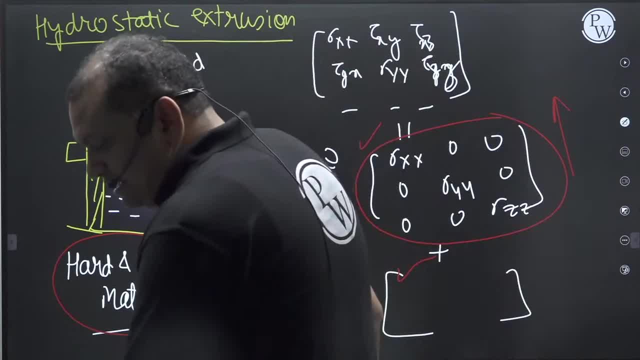 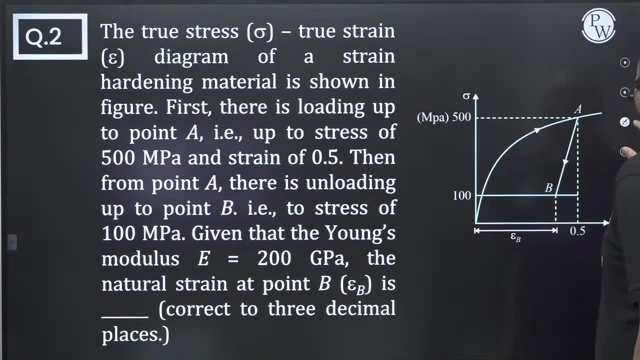 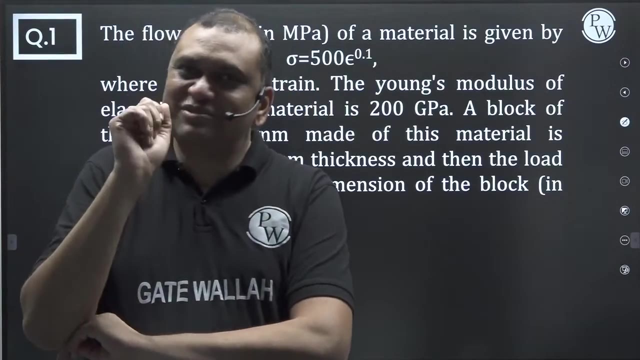 theory be crash course to otherwise Javi theory for a year. normally it takes around five or six years to get it done. it's not possible. Now let's make some questions. let's make some questions a little earlier. There are already 2-3 problems like this in GATE. I think there is a problem of 2015 which 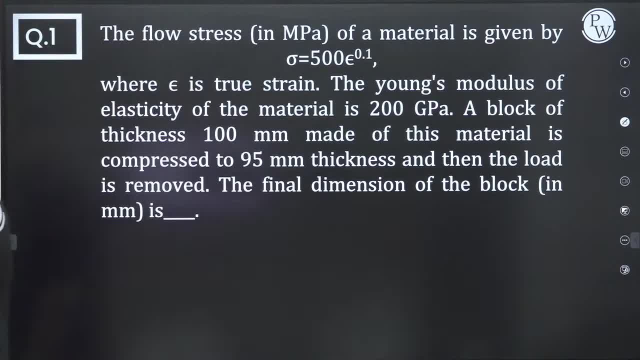 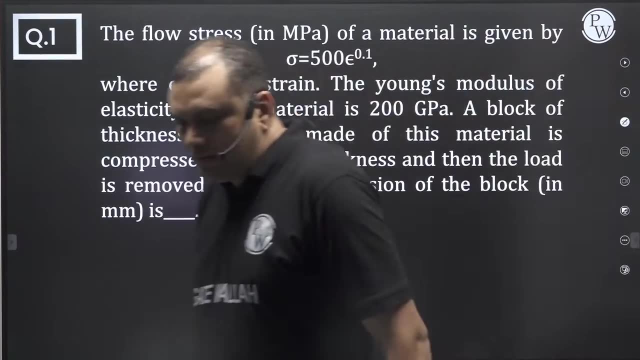 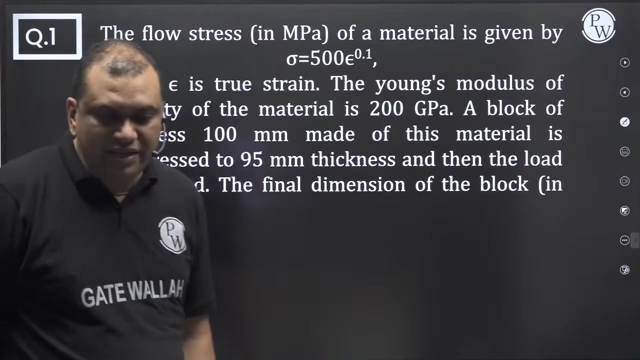 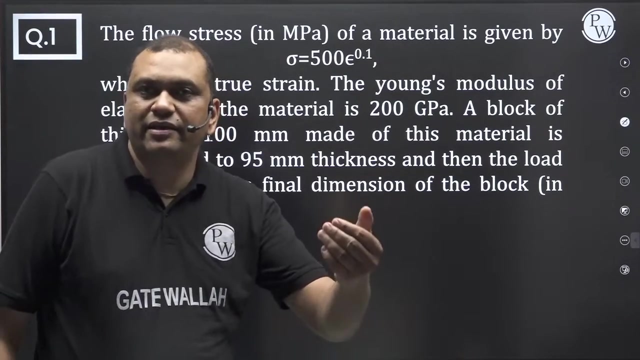 is seen on your board. Go and read the problem. GATE 2015 has a problem, So we will make some questions now. ok, See what I had planned. we will not be able to do that much problem. We will do the rest of the problem tomorrow- our section, And tomorrow we will do forging. 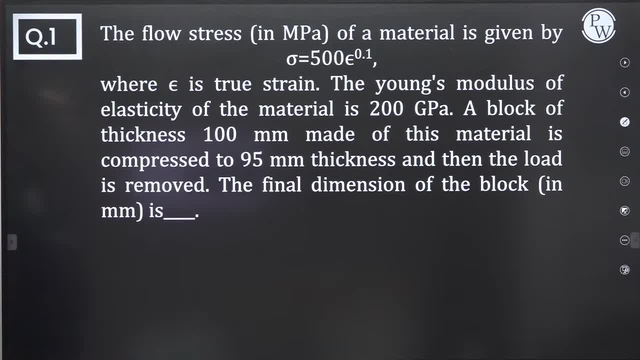 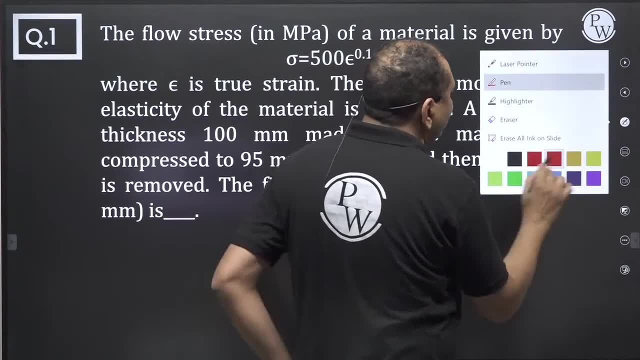 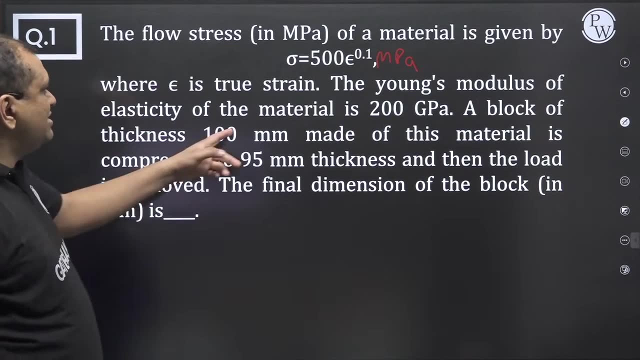 also ok. The flow stress in MPa of the material given by 500 epsilon raised to power 0.1 MPa. MPa color change, otherwise some students will say Sir red is not visible Where epsilon is the true strain. the Young's modulus of the elasticity of the material is 200 Gpa. 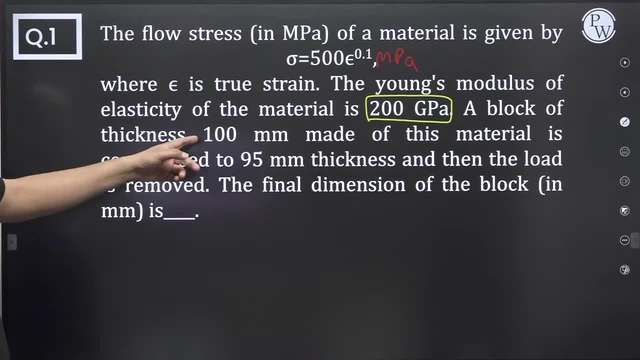 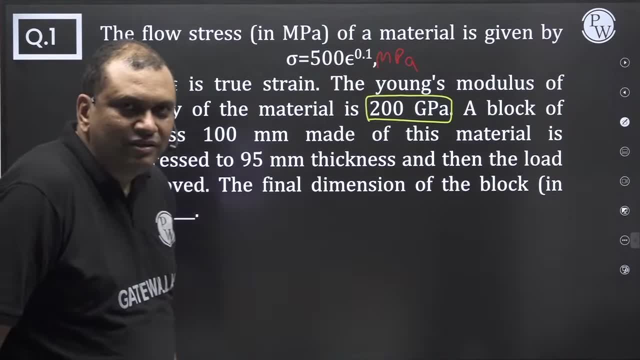 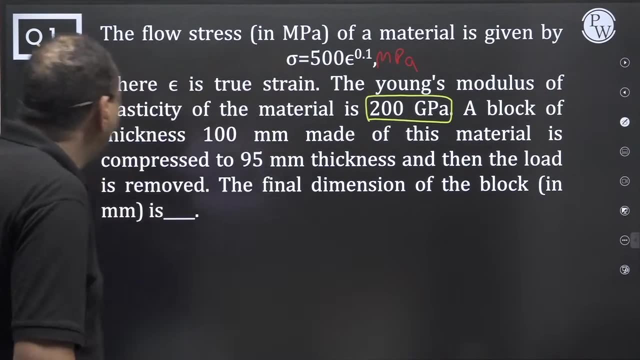 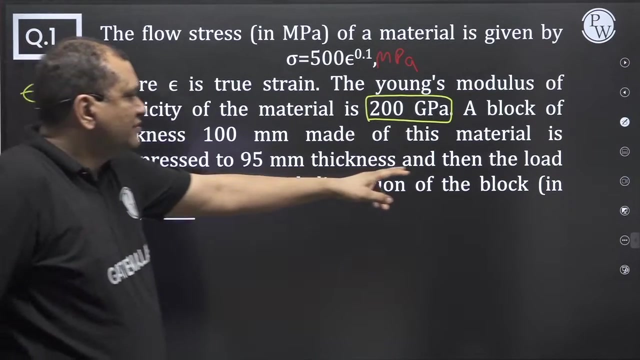 200 Gpa, A block of thickness 100 mm is made of. this material is compressed to 95 mm. So true strain will be calculated in the direction of applied load. So epsilon is nothing but ln h1 by h2, ln 100 by 95, ok. And then, when the load is removed, the final dimension of 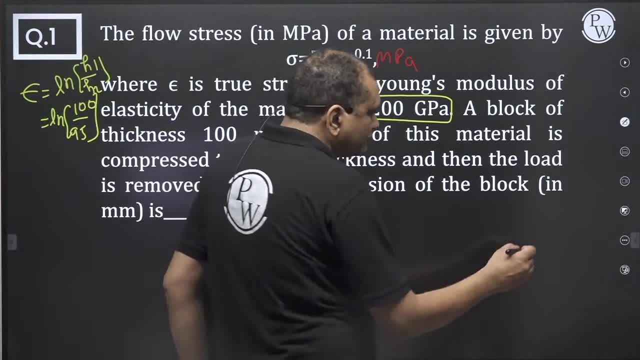 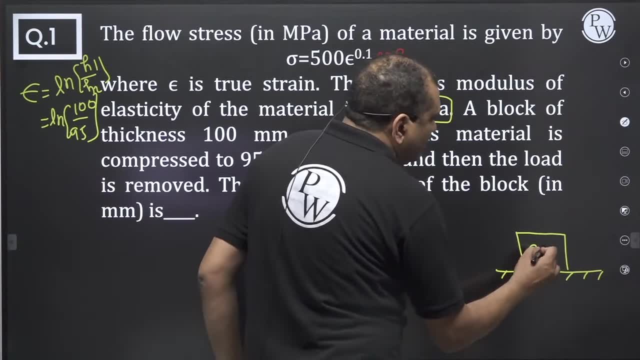 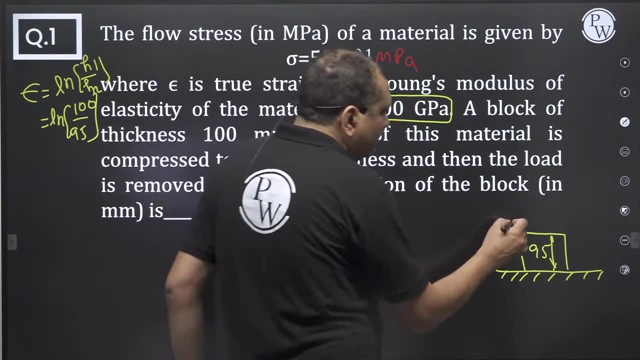 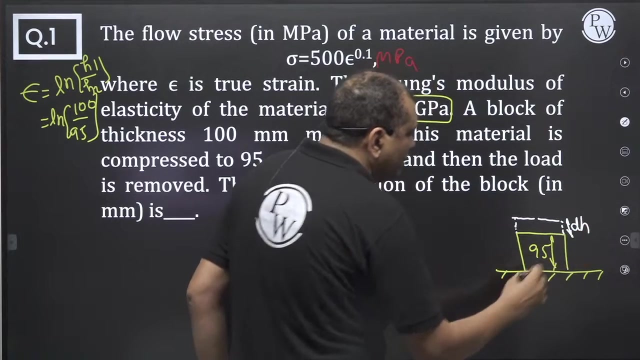 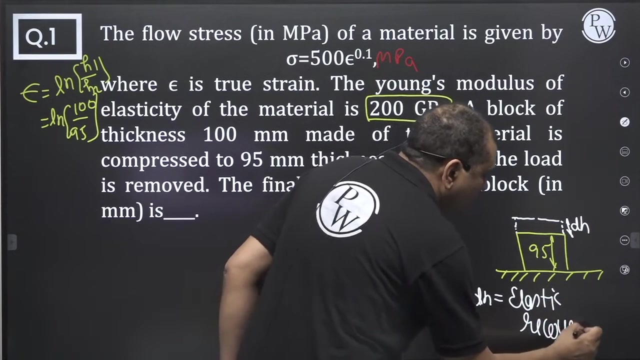 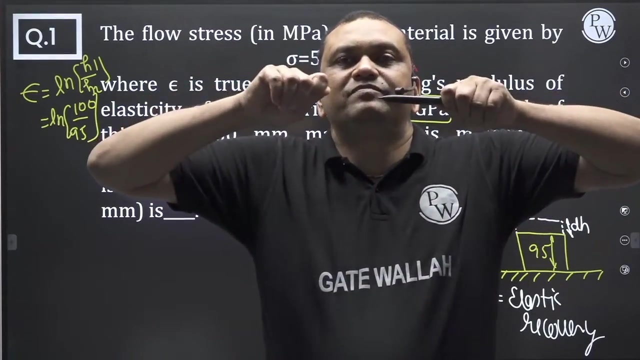 the block in millimeter is because of elastic recovery. I had told you that there is wire drawing. You put the load. 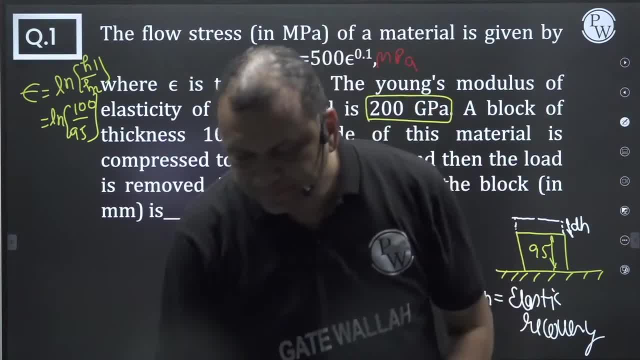 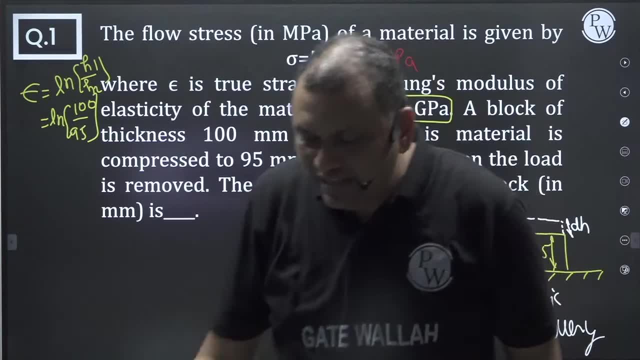 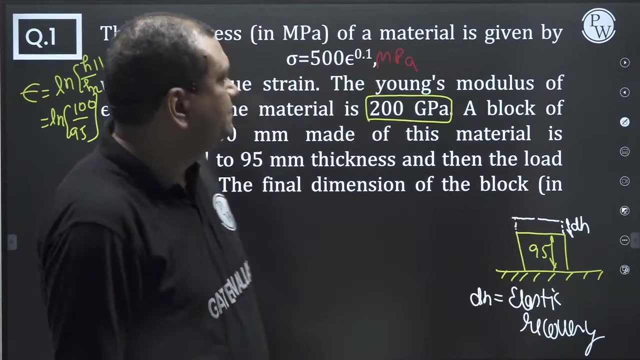 As soon as you remove it, the length is reduced. There is forging. You press it. As soon as you remove it, it will increase a little. It's called elastic recovery. Elastic strains will recover. Now don't jump so fast. It's not that easy actually. So what will we do here? 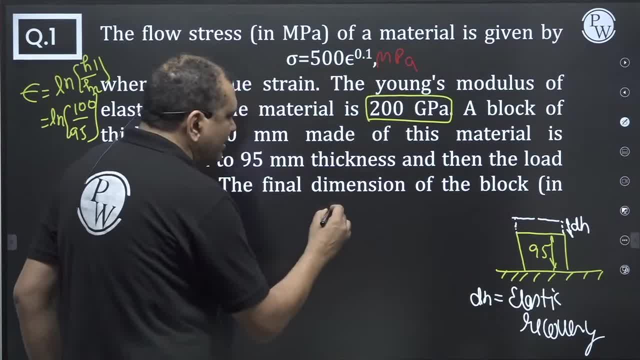 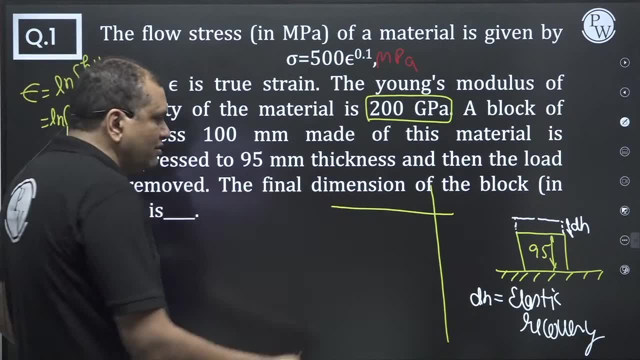 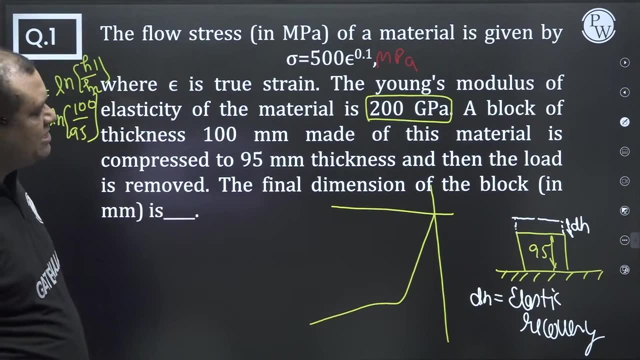 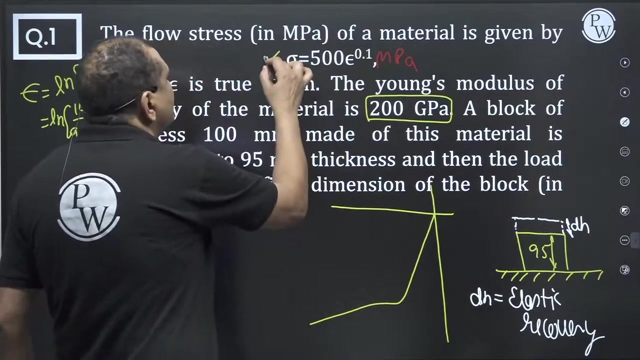 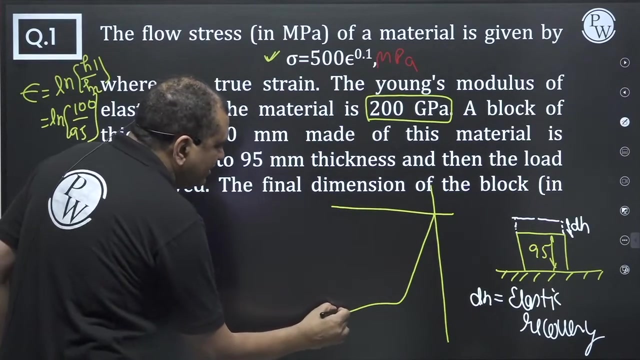 Let's make a diagram of this. first, This is compression. We are applying compressive load. So in compression your stress-strain diagram came like this: Right, And this is sigma. So let's make a diagram. So you have taken the load up to here. Now how will this come out? True strain you have. 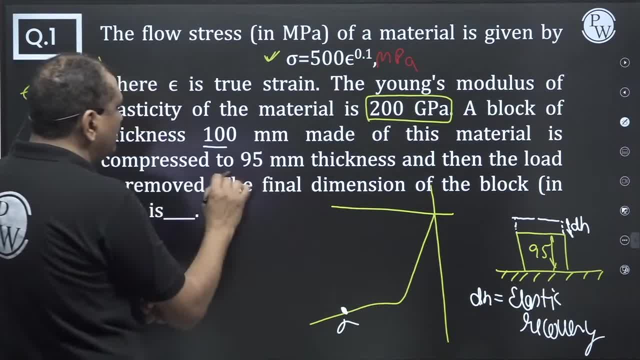 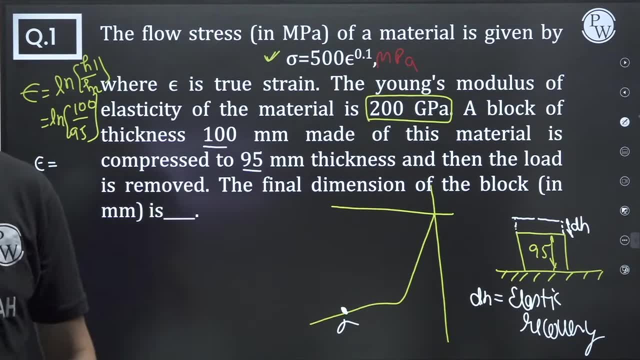 calculated right: H1, H2.. So how much is your true strain? I have solved it for you: This is 0.051.. 0.051 is the true strain. You have to find out where this true strain is. 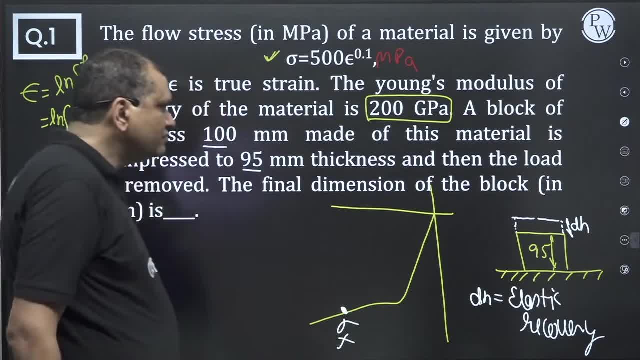 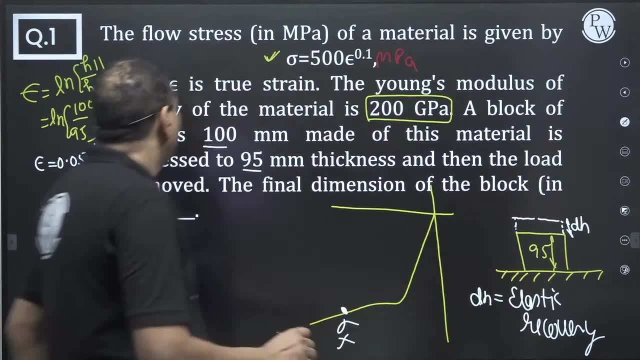 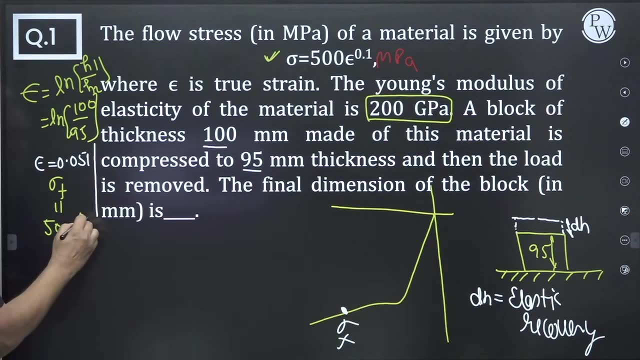 How much is the true strain here? So keep this there. Let me change the color a little so that the question and the solution have a different color. So sigma F is equal to 500 epsilon raised to power 0.1.. If we put it in this, then take it out. How much is? 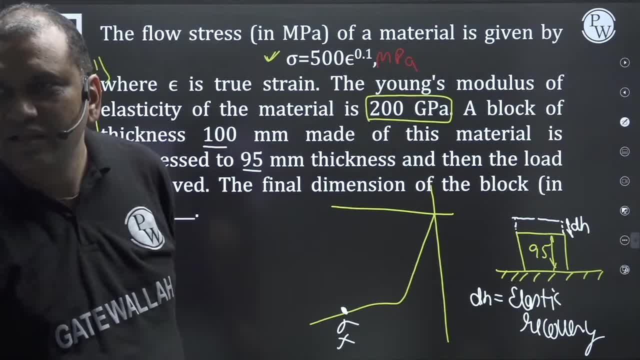 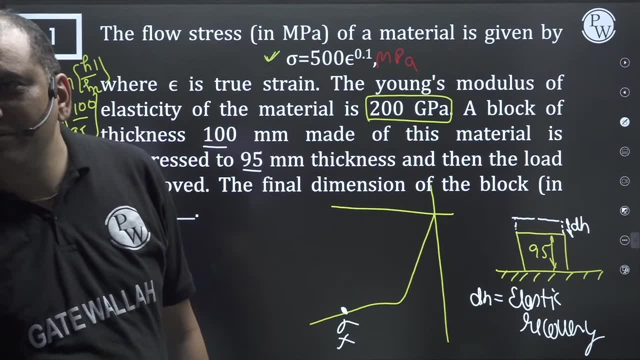 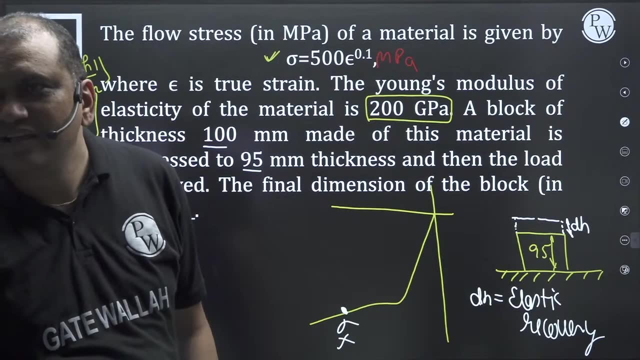 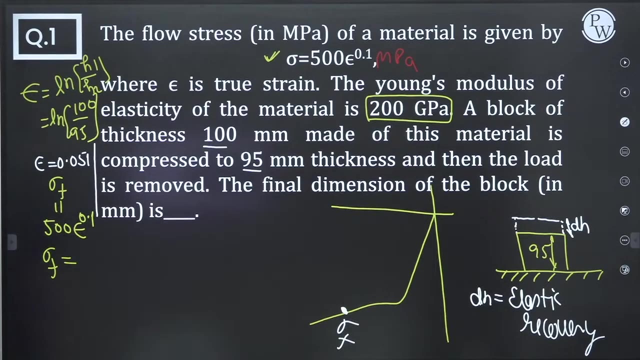 coming out. Take it out, Or have you done it before? All right, Okay, Karan Madhuriya, Let's see, Take it out. 370 upon 0.5 MPa. Take a look. 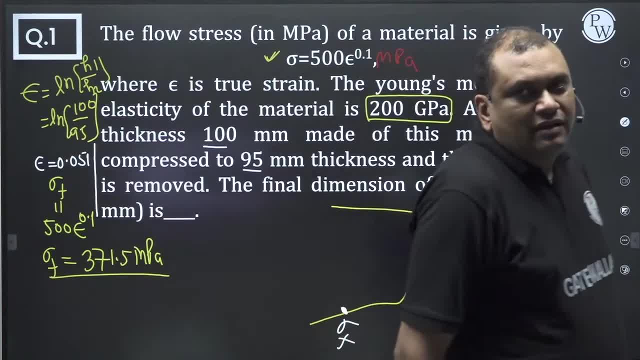 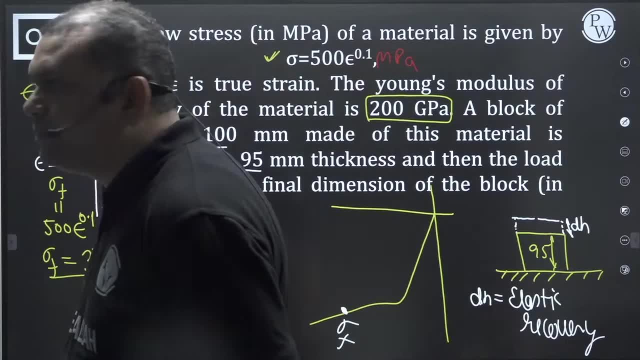 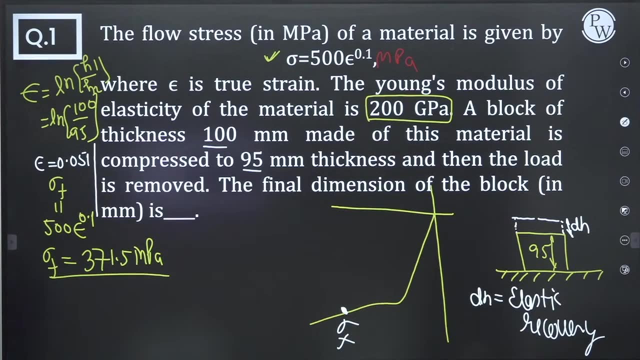 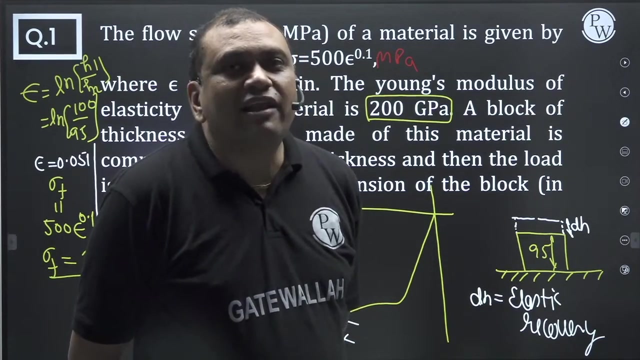 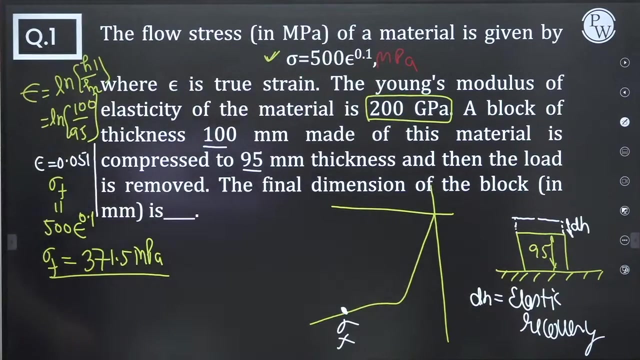 Is everyone getting this much? or should it be 370- 1.5 MPa or 370 1.5 MPa? Be careful, because on the royal road there are accidents. Understand the problem. it is a very good problem. There have been 2-3 problems based on this in the last 5-6 years. 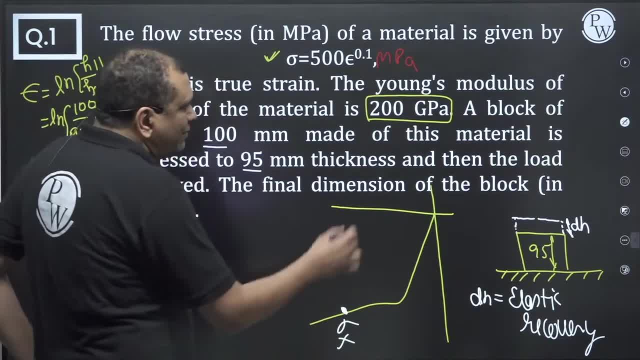 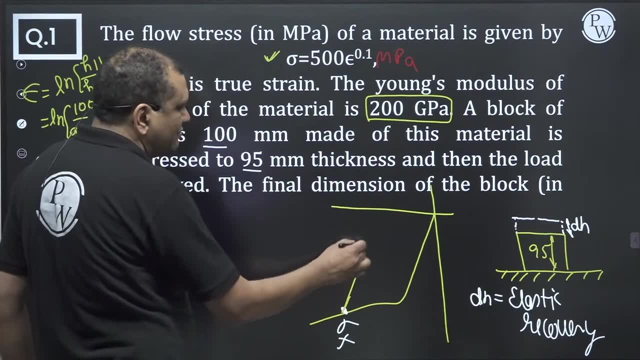 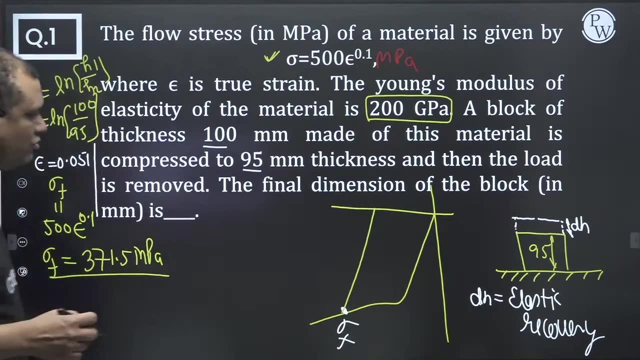 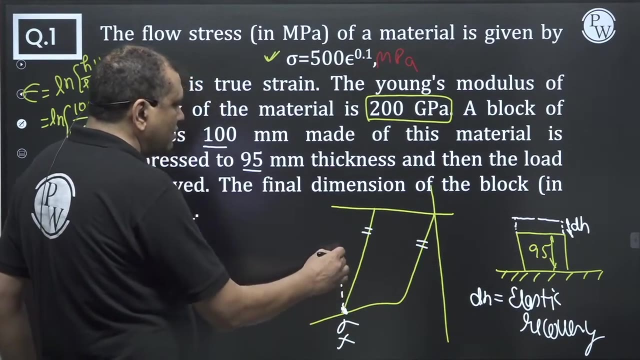 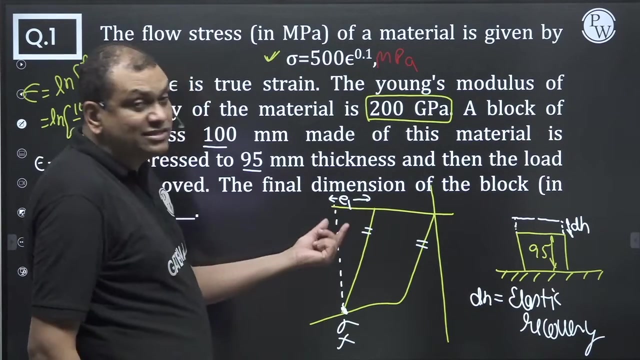 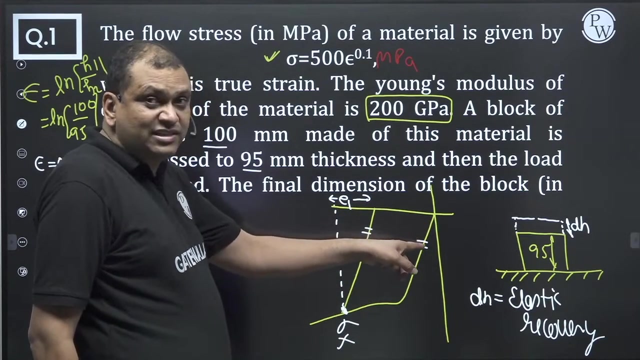 Now listen. you have loaded the material till here. If we unload it, it will follow this curve. This line will be parallel to this. This line will be parallel to this And this E1 is called elastic recovery, Because the unloading curve will be parallel to the elastic region. 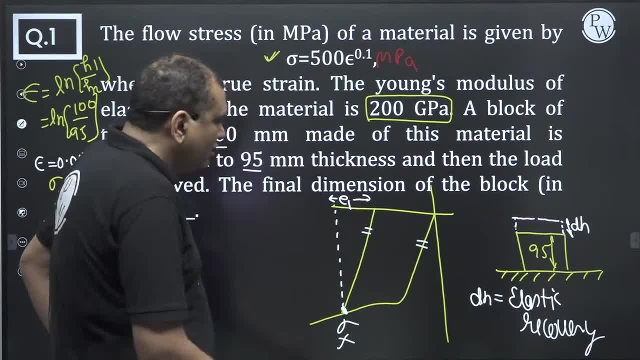 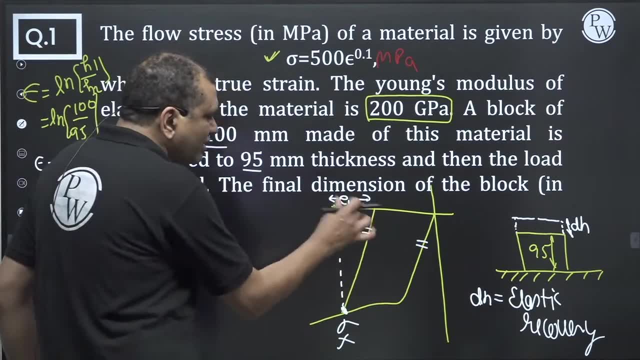 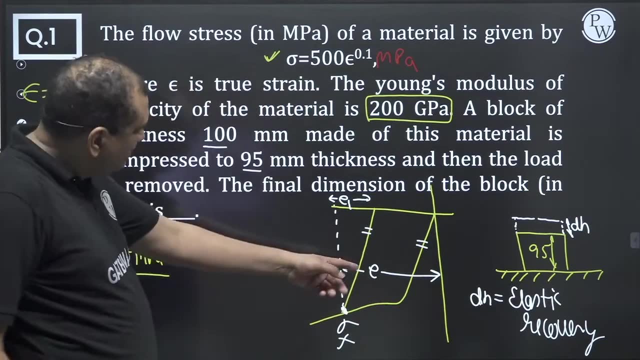 If you start with the strength of the material, then it will be explained in detail. So this is yours And the total strain here, this E1, is elastic strain. This is the total strain. let us take it from the ladder. What is E Total strain? 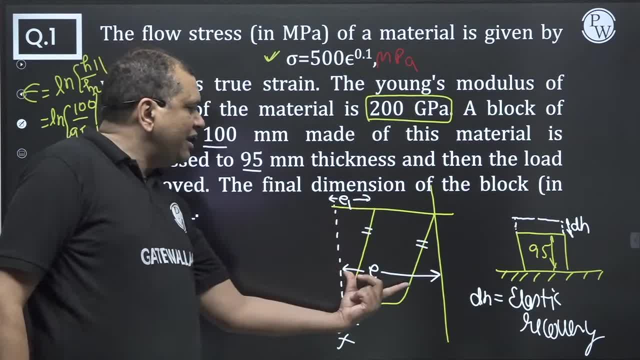 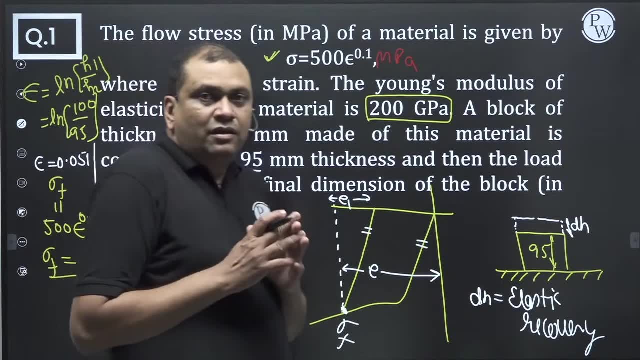 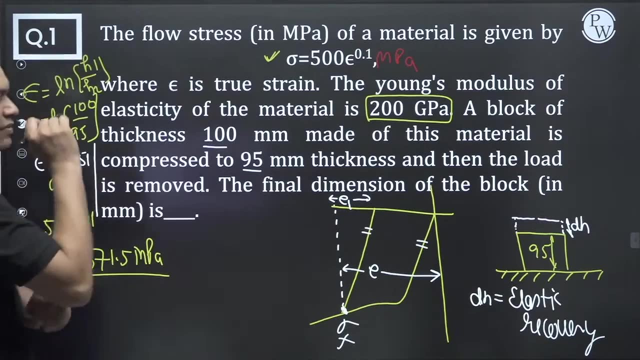 What is E1? Elastic strain, which I have kept here. What is E, Total strain up to the sigma f? And what is E1? Elastic recovery. So to get E1, you will apply the Hooke's law. To get E1, you will apply the Hooke's law. 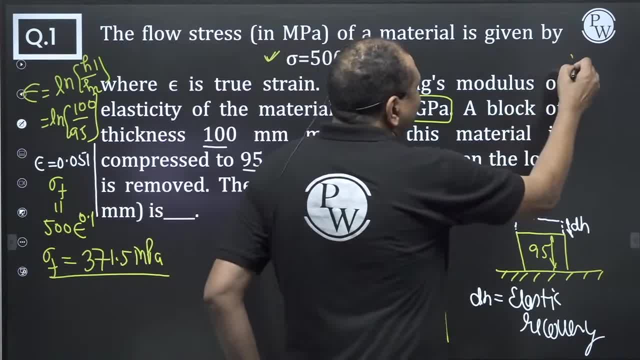 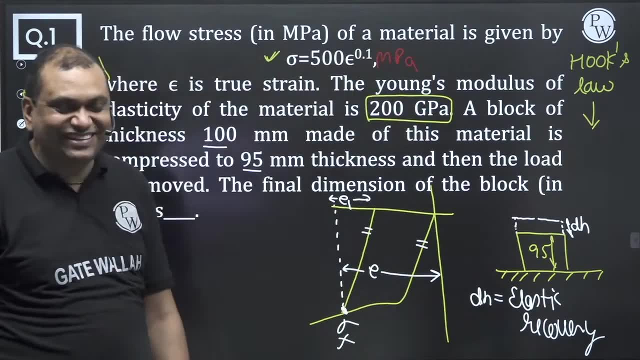 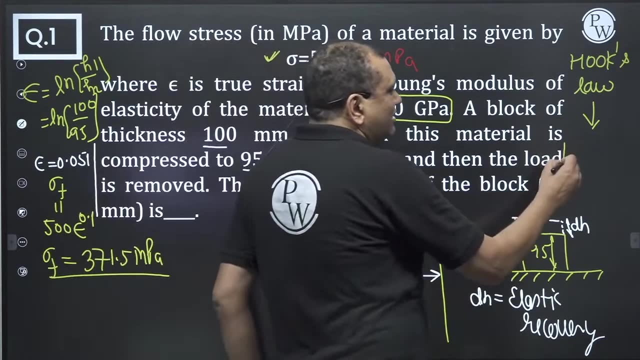 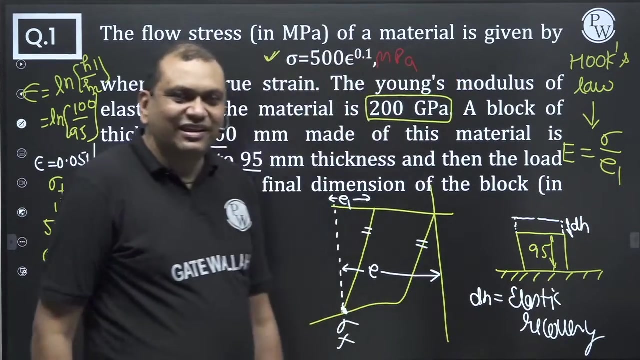 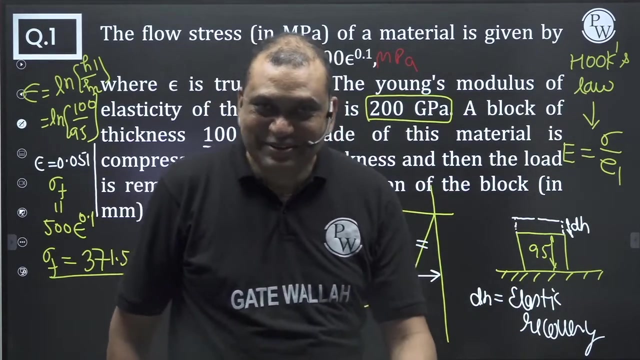 But remember one thing Here: many students make mistakes, But with a cool mind. In Hooke's law Young's modulus is nothing but sigma divided by E1. Here sigma is not an engineering stressor, not a true stressor. The sigma is an engineering stressor, not a true stressor. 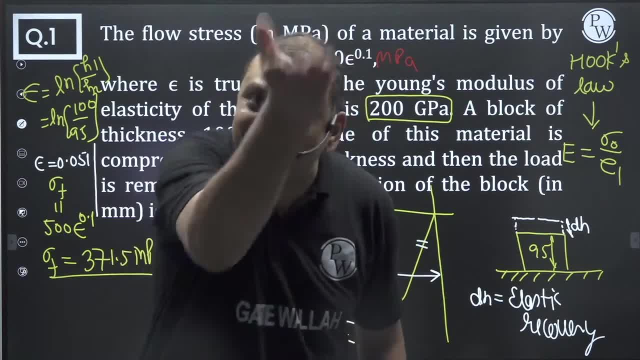 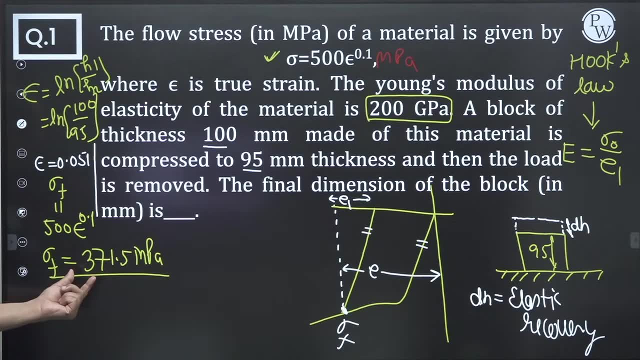 In Hooke's law, true stress is not an engineering stressor, And what you have taken out is a true stressor, isn't it? So first convert this into an engineering stressor. So sigma f is equal to sigma 0 E plus 1. 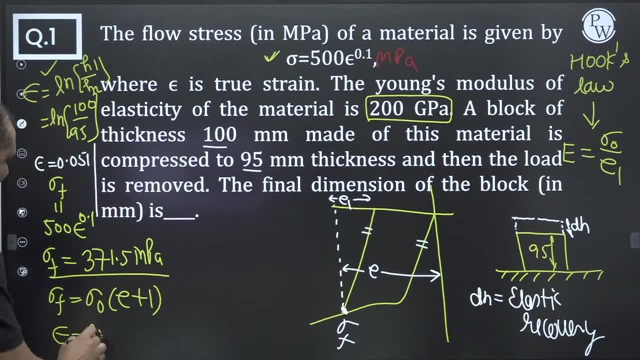 And you have already taken out epsilon. Epsilon is equal to ln. E plus 1. So do one thing: You know the value of epsilon, Take out E plus 1 and put it here. You know sigma f, you know this, So you will get sigma 0. 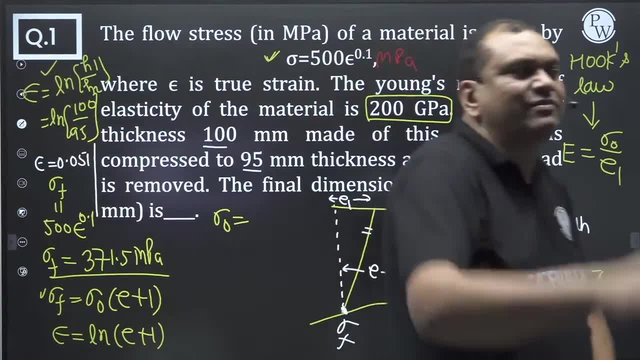 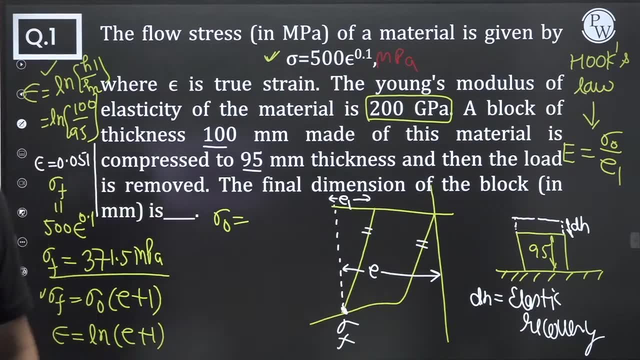 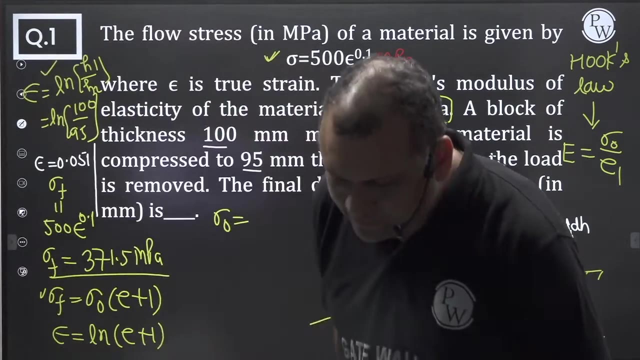 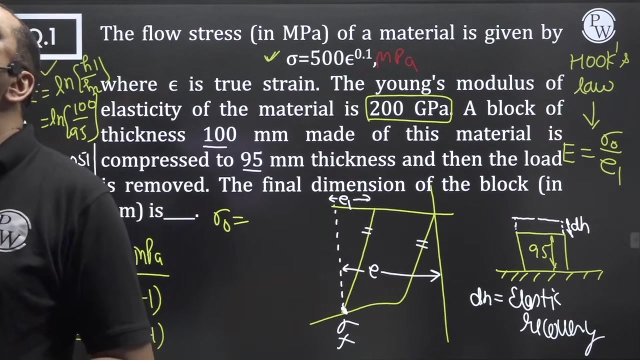 Take out sigma 0, there will be a slight difference, But calculate sigma 0. There will be a slight difference, But calculate sigma 0. Tell me what is coming. Calculate sigma 0. Take out sigma 0. quickly see what is coming. Hurry up, hurry up, hurry up. 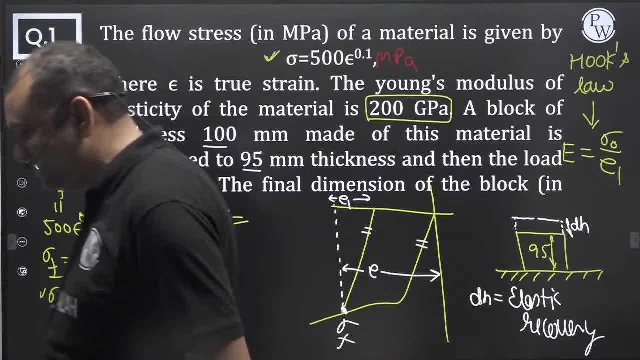 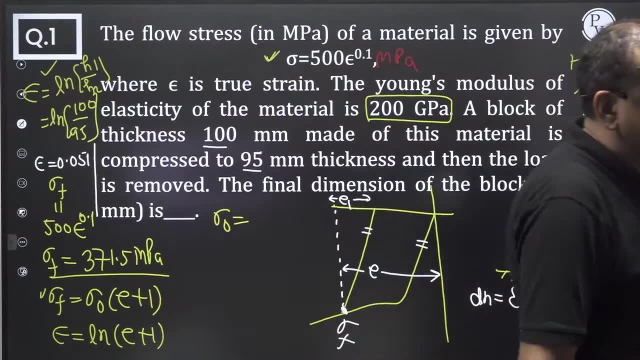 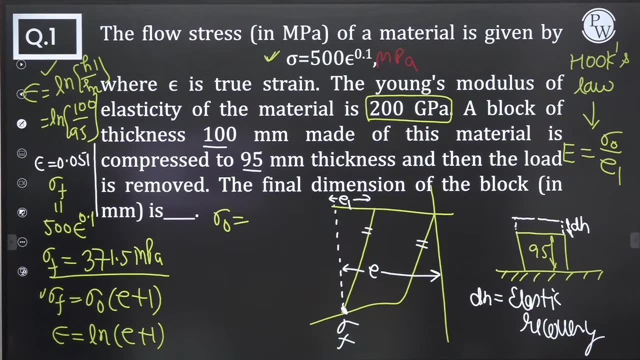 Because it is going to be 11 o'clock. Hurry up, hurry up, Because it is going to be 11 o'clock. Because it is going to be 11 o'clock, Okay, Now do one thing: give me the final answer. No. Gaurav Mohrana. 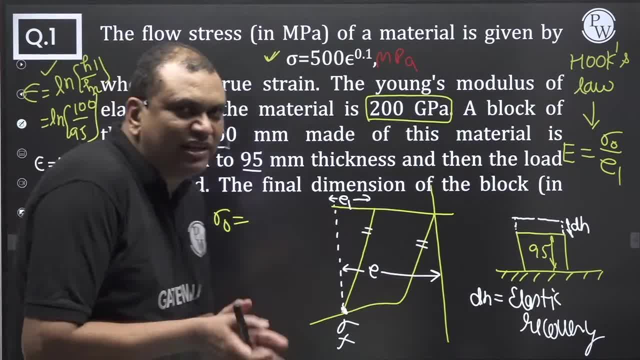 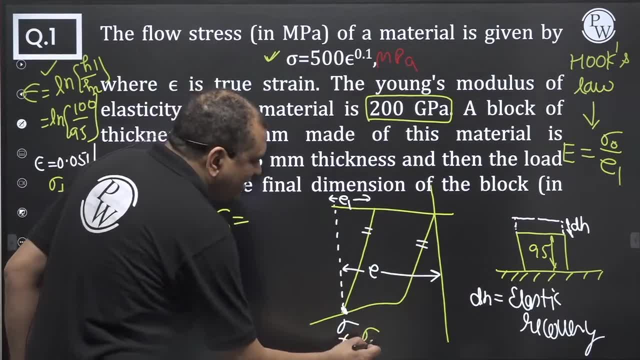 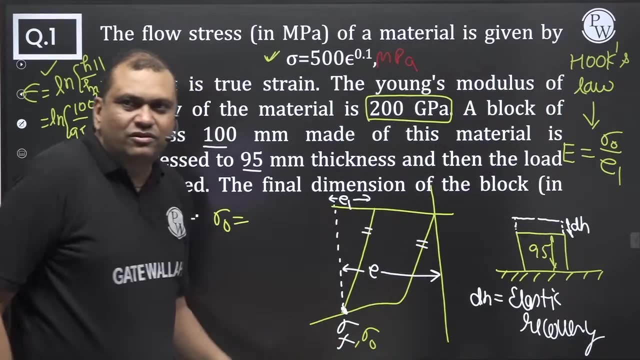 Actually there is a slight offer for your answer. Listen, everyone look at the board. Everyone look at the board for two minutes. Your sigma 0 has come. What is sigma f? True stress? What is sigma 0? Engineering stress. So everyone look at the board. 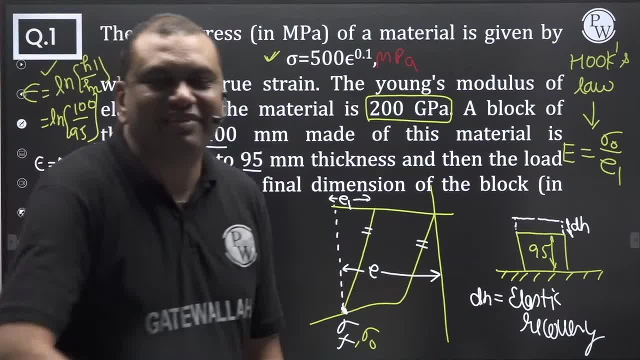 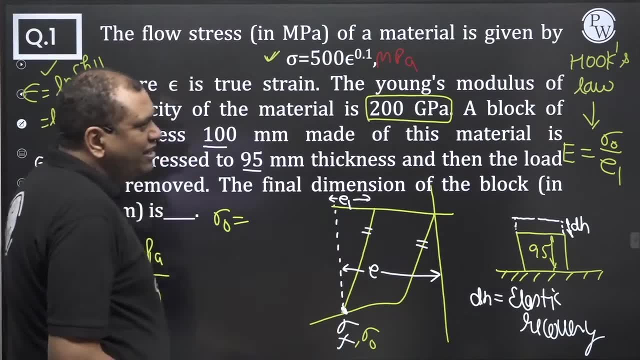 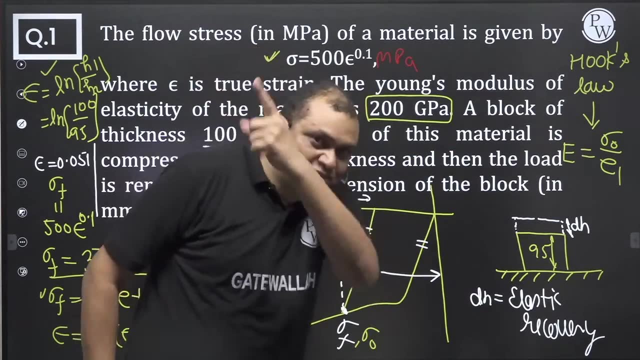 Very good, very good, Very good. Everyone, look at the board for two minutes. I have come to a very critical thing, Because in Hooke's law Only engineering stress comes. Only engineering stress comes. in Hooke's law, True stress does not come. Keep this in mind. 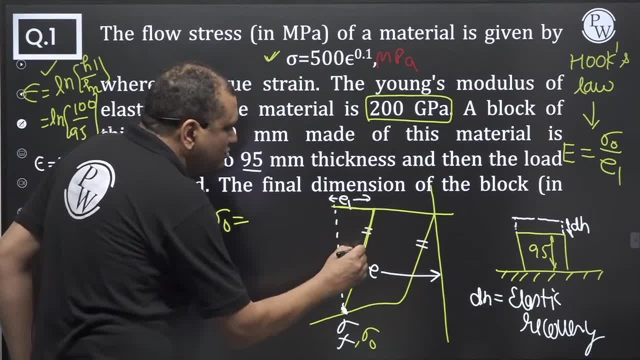 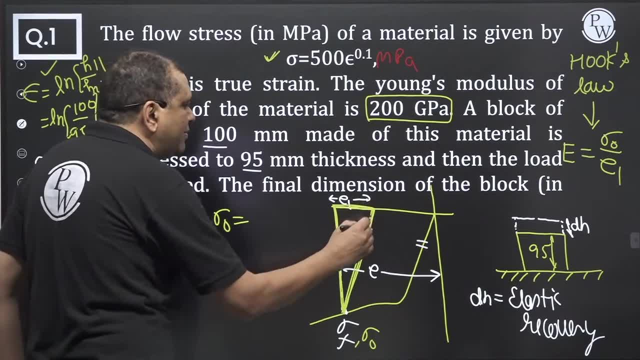 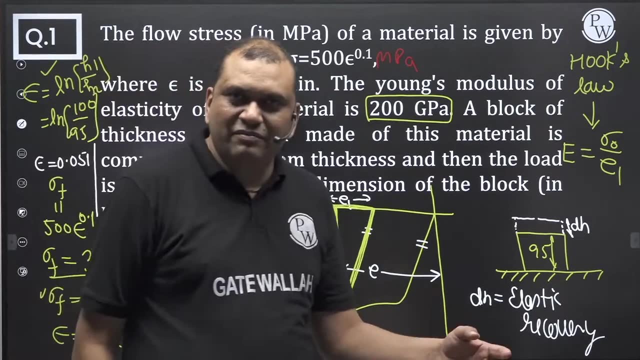 Now what I am doing. See, in this region, I am applying Hooke's law. In this region, I am applying the Hooke's law. Anyway, the questions we have set. One of our team members, Rohit Jeevan, has worked very hard In designing these questions. 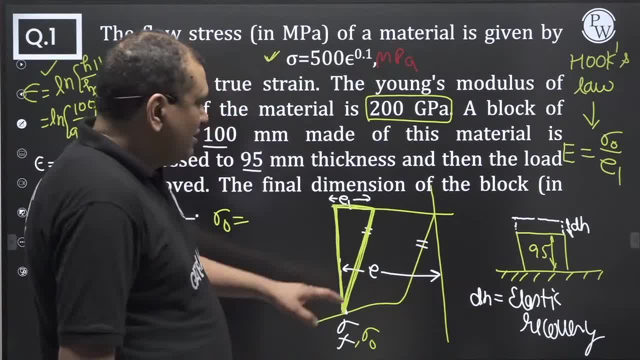 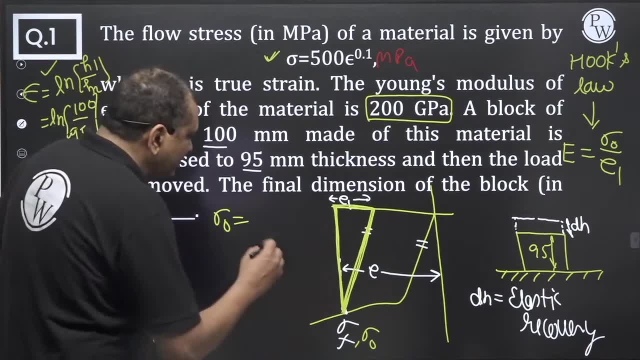 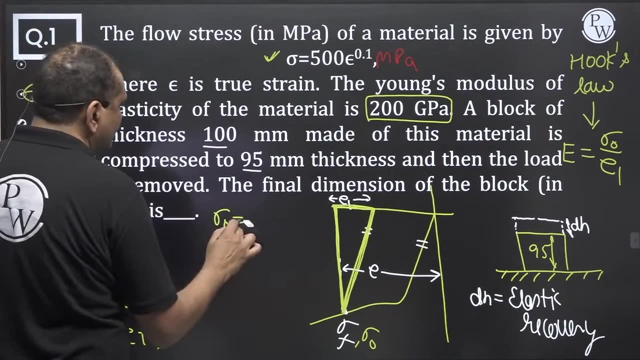 So tomorrow we will definitely do these questions. Okay, So he is a very good person. So look, now I am applying Hooke's law in this region. So look, sigma 0 divided by E1, Sigma 0 divided by E1, Is equal to Young's modulus. 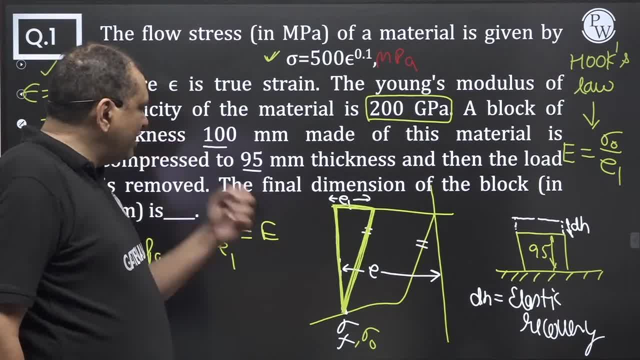 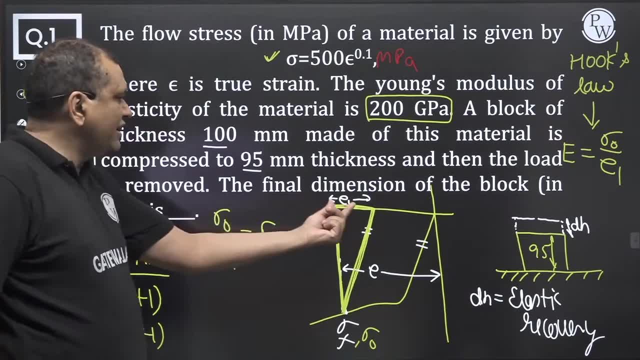 Because our Hooke's law, Hooke's law- can be applied only with the engineering stress, Only in the elastic region. So from here to here there is a straight line. What is E1? Elastic recovery? So keep the sigma 0 here. You know the value of E. 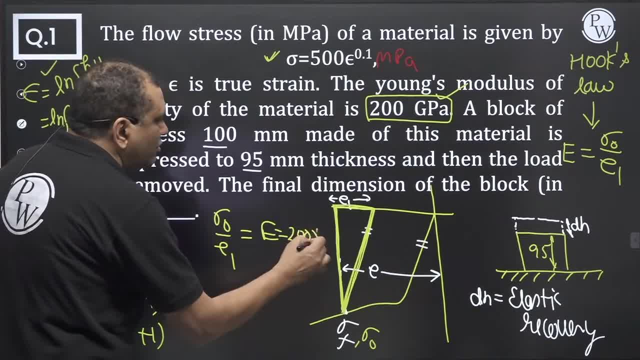 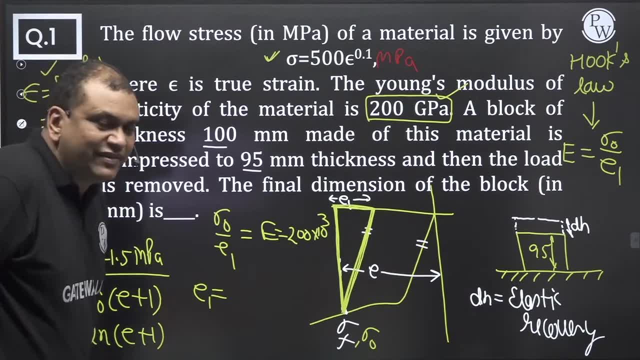 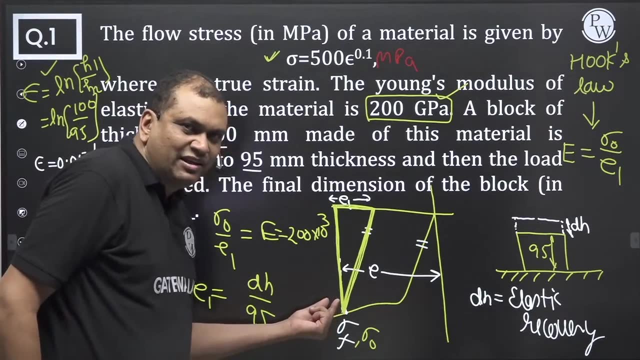 200 GPA 10 raised to the power 3. Why Is it GPA or MPA? So you will take out E1. E1 is nothing but dH by 95. See, we have reached here 95 height. After that there is elastic recovery. 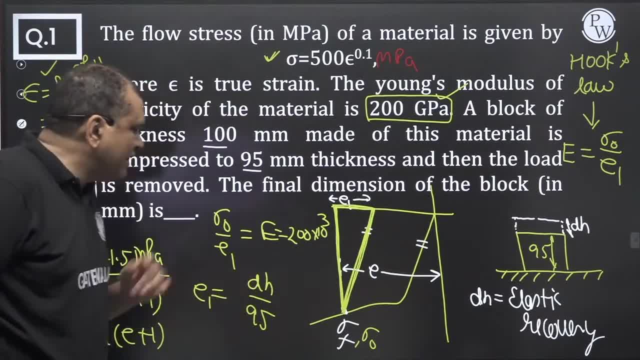 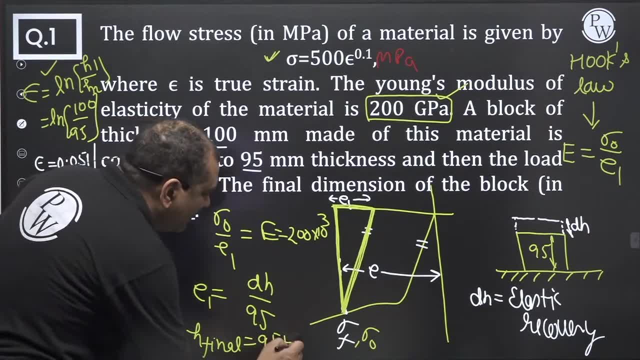 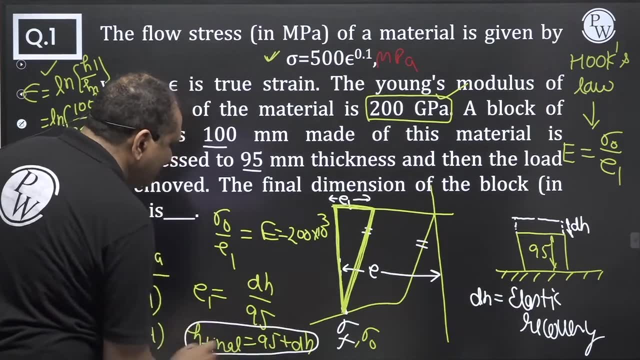 This is a curve in compression. So E1 is nothing but dH by 95, And final height will be 95 plus dH. So tell me what is the final answer. Its answer: What is the final height? Can you tell me now answer? This is the answer. 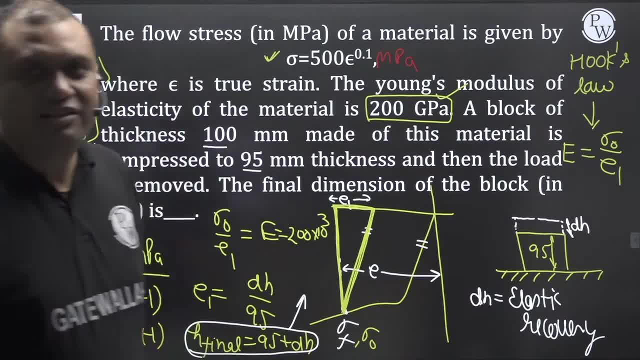 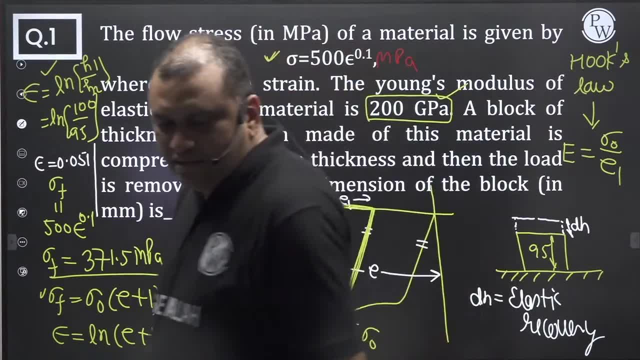 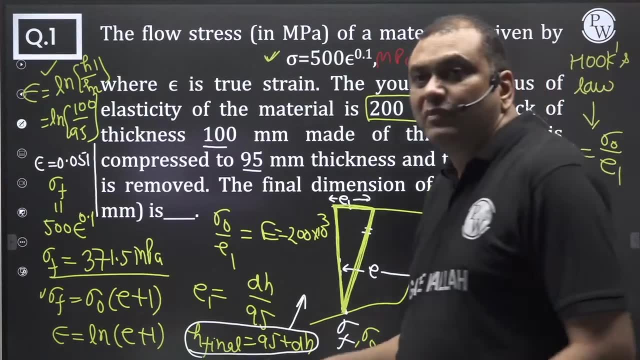 Do it Now. do it. Did you understand? Sometimes it takes a lot of effort. It takes a lot of effort. Now tell me Already 7. Now tell me what is the final answer. Do it quickly. But the lecture which we will start tomorrow, We will do it with questions. 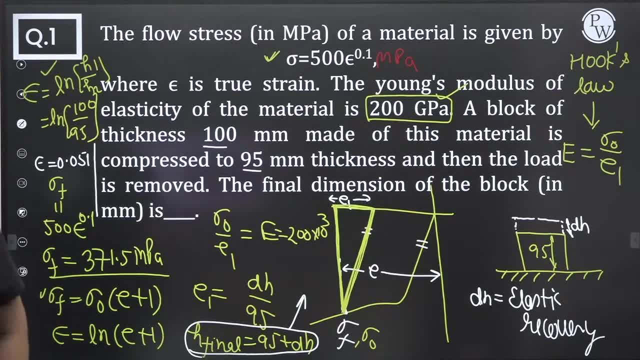 I have 5-6 questions, Very good, So we will start with that. Aman Kant, Very happy to see the answer, But Give me 3 decisions. I would have been very happy Because sometimes in IIT Very good, Very good Ashok, Very good Rishabh. 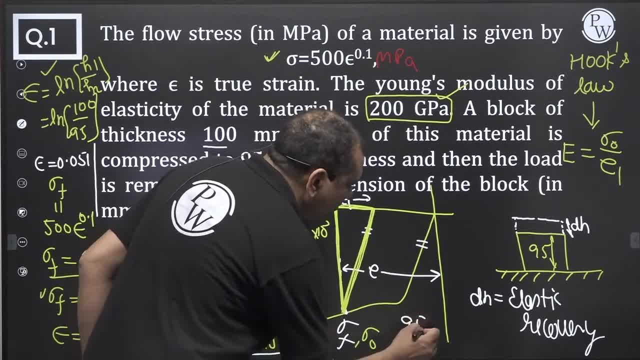 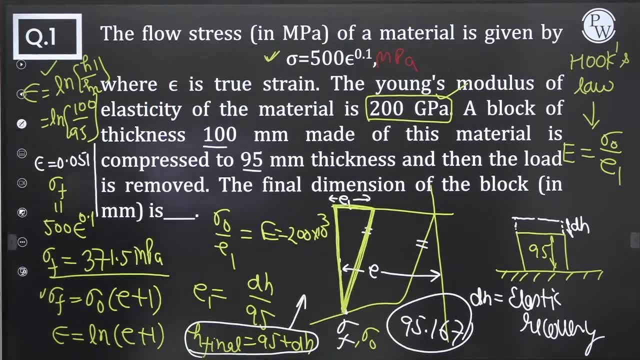 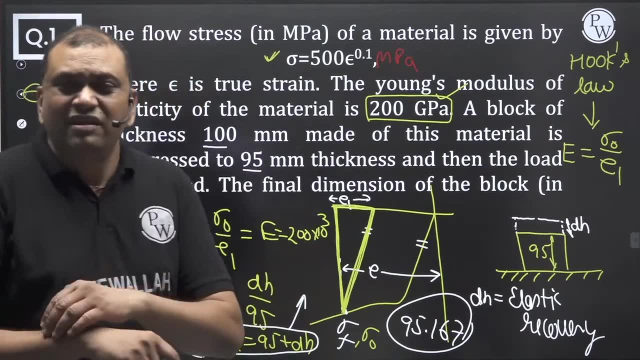 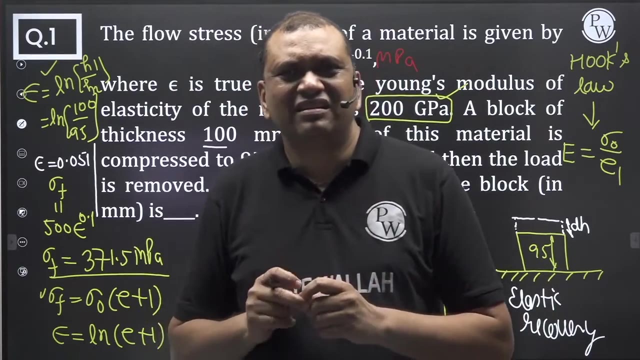 Very good, 95.167. That is the correct answer. Very good, Animesh Nanda. Very good Bashir. Very good See, It is very important to understand this question. That is why I have spent my time on this. I was planning to do at least 10 or 12 questions.